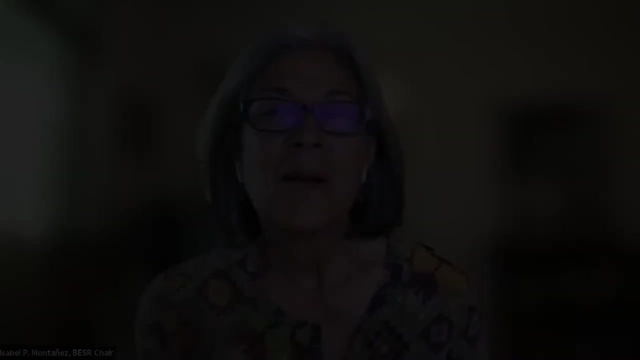 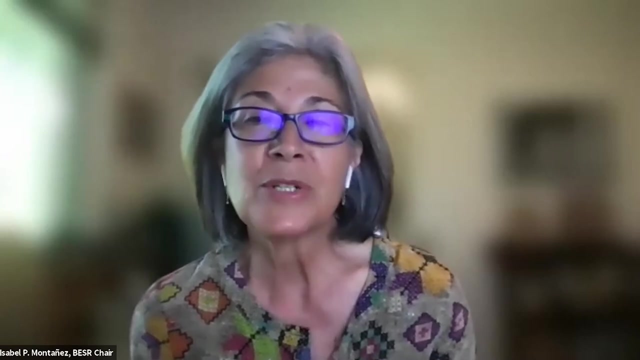 Welcome. Good day everyone. I'm Isabelle Montanez, Chair of the Board on Earth Sciences and Resources, or what I'll refer to as BESER, And I'd like to start by thanking you all for attending today's meeting. 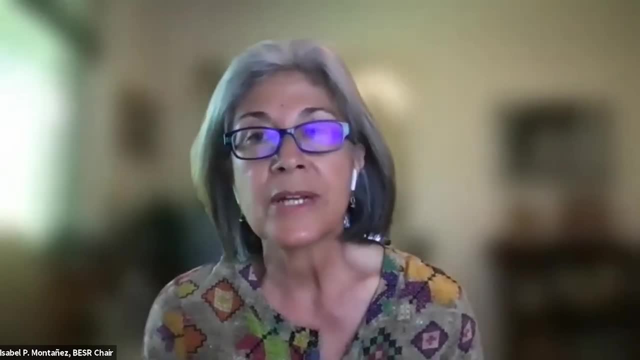 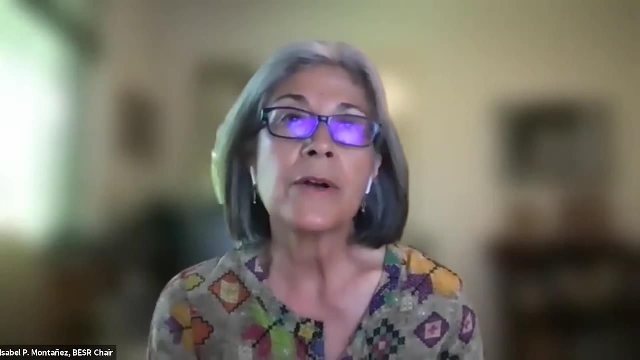 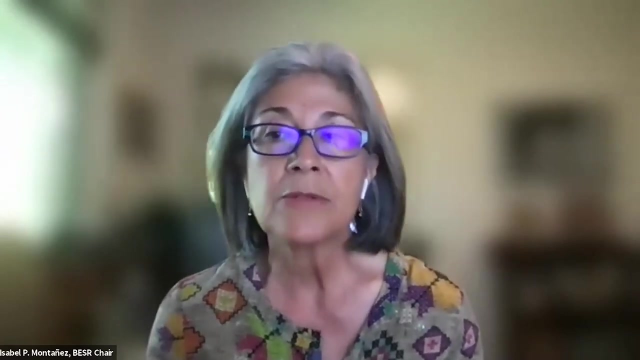 Today's focus is energy and resource needs for a nation in transition. We seek to learn more about the current energy and earth resources research priorities and how these priorities are positioned or evolving to address changing societal demands, to mitigate climate change, and to decrease adverse social inequities and environmental impacts. 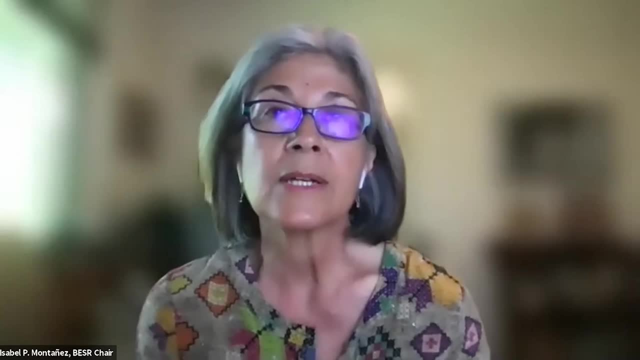 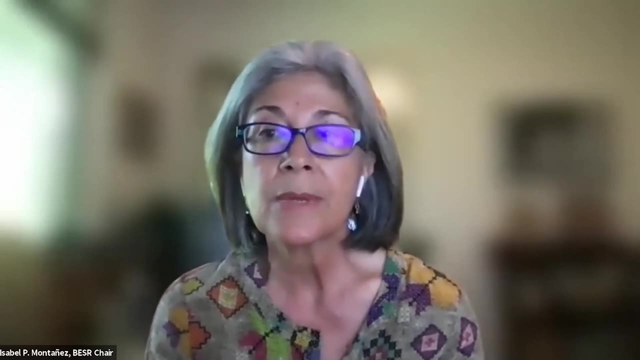 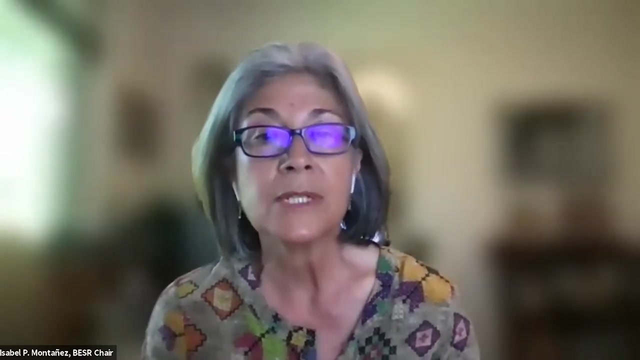 So, after I give a brief overview of the BESER mission and discuss the meeting protocols, we'll be hearing from our keynote speaker, Brian Anderson of the National Energy Technology Laboratory, as well as three panelists: Nicole Saunders from the Environmental Defense Fund, Rebecca Hernandez from UC Davis and Ben Holton, the Ronald P Lynch, Dean of the College of Agriculture and Life Sciences at Cornell University and co-chair of the California Collaborative for Climate Change Solutions. 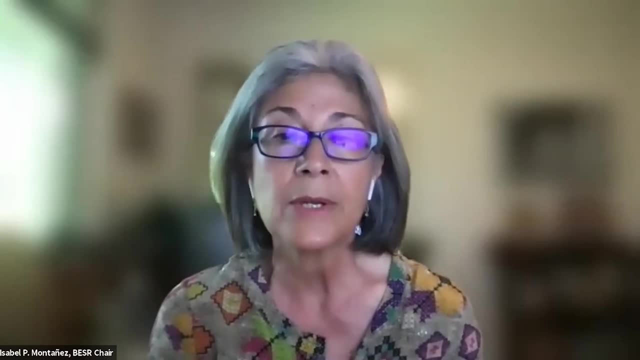 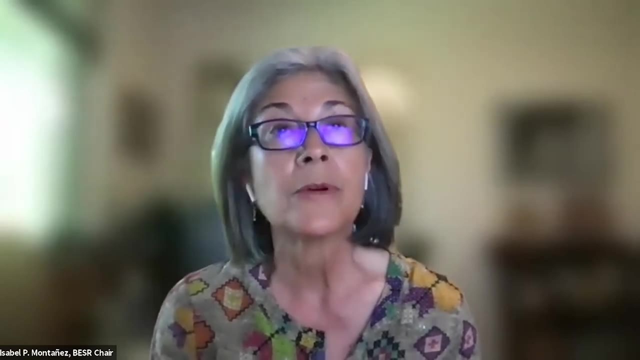 After each presentation, there'll be time for questions from the board and the audience, And we'll be taking a 15-minute break at 2 pm Eastern Standard Time, after which we will return for a presentation. Thank you for joining us for this panel discussion. 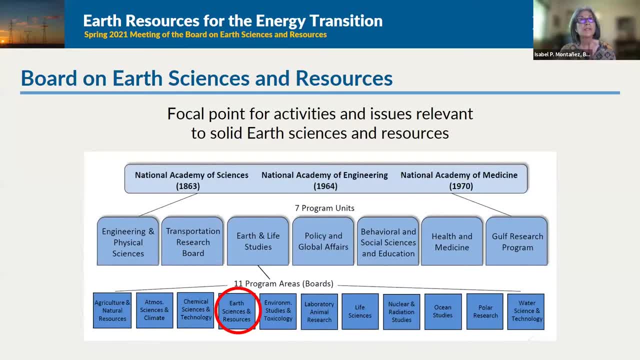 Can I have the next slide please, Eric? The Board on Earth Sciences and Resources is the National Academy's focal point for activities and issues relevant to the solid earth sciences and resources. It's one of 11 boards in the Division of Earth and Life Studies and together these boards comprise most of the national science portfolio of the Academy. 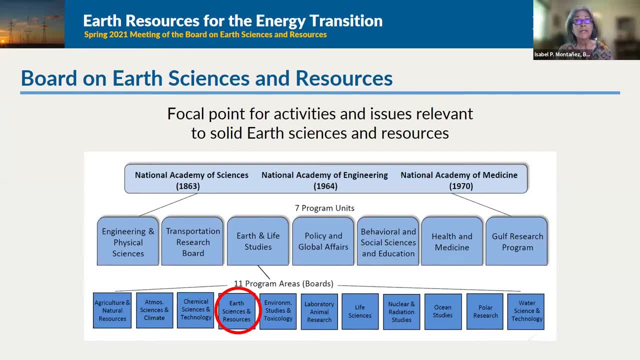 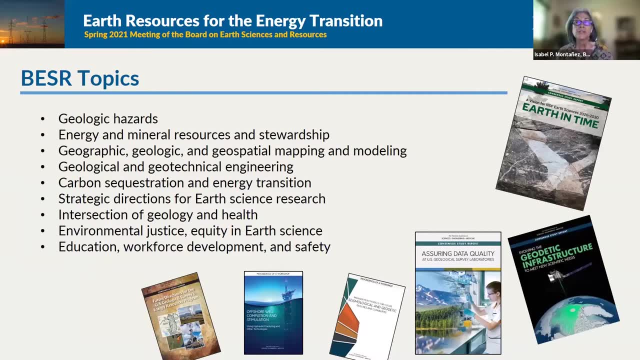 Other divisions cover engineering policy, global affairs and social sciences. Next slide, please. We cover a broad topical space including a range of geologic hazards, energy and mineral resources and stewardship. geographic, geologic and geospatial mapping and modeling. 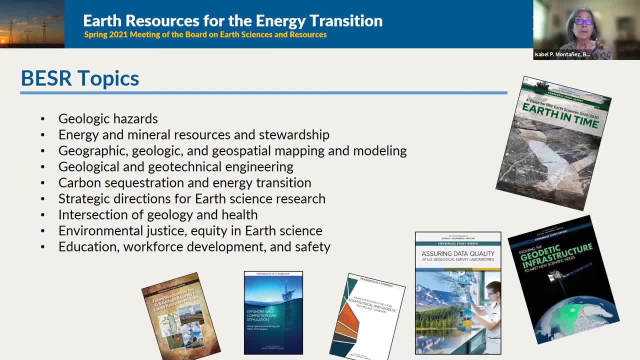 geological and geotechnical engineering, carbon sequestration and energy transition, strategic directions for earth science research, the intersection of geology and health, environmental justice and equity in earth science and education, workforce development and safety. So clearly much of our work has important societal implications. 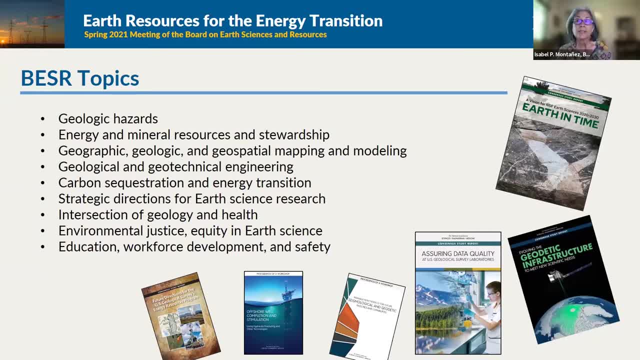 These earth funding sources are diverse and showcase the breadth of earth sciences. Our core funding is currently supported by NSF's Division of Earth Sciences and the Geoscience Directorate, NASA's Earth Surface and Interior Focus Area and DOE Basic Energy Sciences. USGS is a traditional sponsor with pending support. 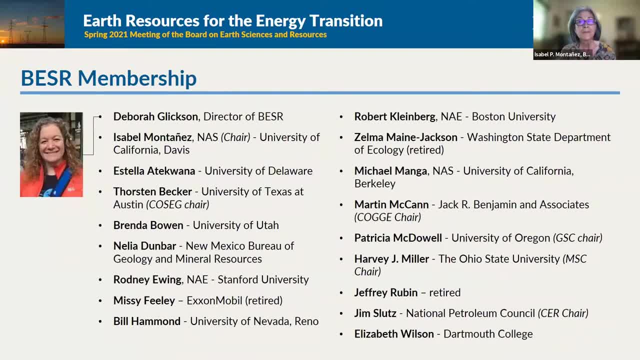 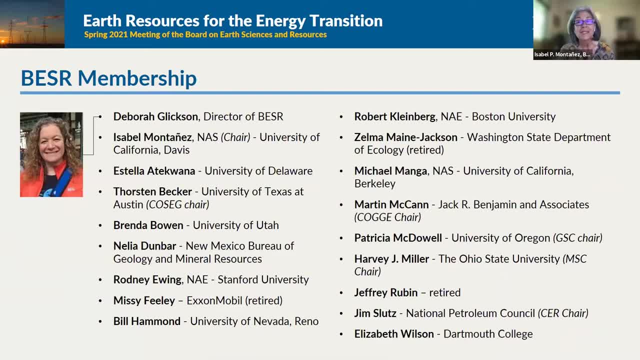 Today, in the interest of time, I'll not be introducing the members and staff, but we present them here to acknowledge their contributions to the board, And I also invite you to look through the agenda booklet for more information on our members. I'd like to mention that we also have a new directorate. 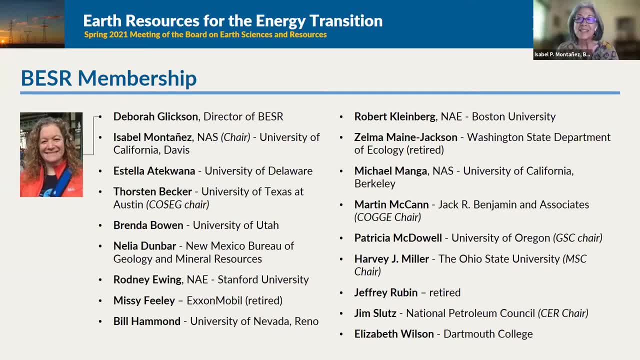 who is the Director for Energy and Geoscience at the University of Northern California, Director Dr Deborah Glickson, who you see here, who oversees both the Board on Earth Sciences and Resources and the Water Science and Technology Board. Deb is a marine geologist who brings 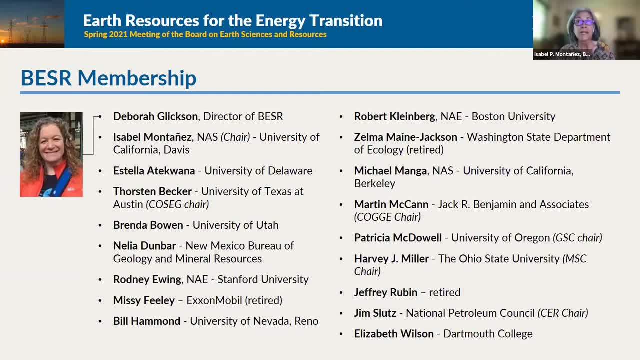 considerable experience to the board, accrued over her tenure at the National Academy since 2008.. And board members, please introduce yourself when asking questions. So just a little bit about our Zoom logistics. Board members, please raise your virtual hands to ask a question. We'll be monitoring the virtual hand-raising and we will call on you. 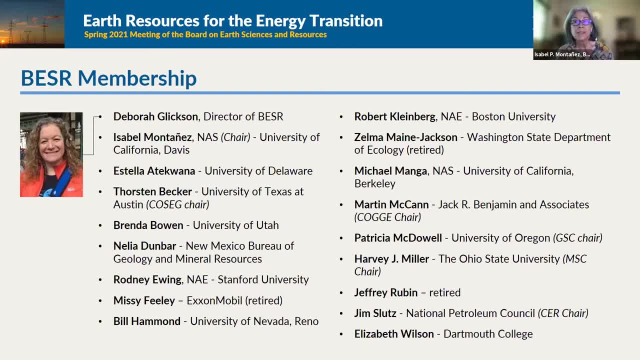 Audience members will be taking questions through the Q&A box located at the bottom of your screen. Please type your questions into the box at any time, click send and staff members will be monitoring the Q&A and passing these questions to the moderators. Please note that this webinar is 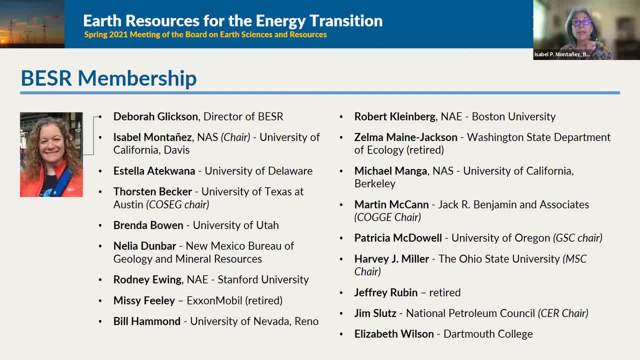 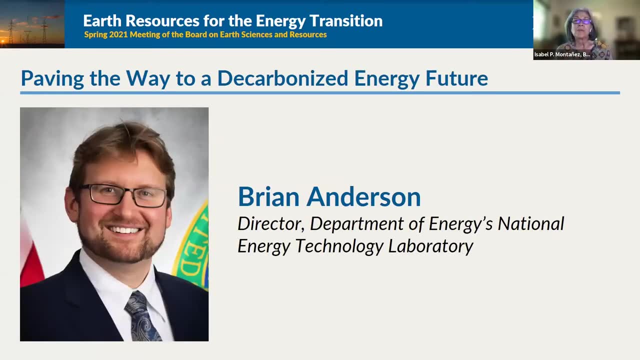 being recorded. Any questions you submit may be read aloud and include in our recording, And a link to the recording is in the description. The recording will be posted on our WIPS. So we're really next slide, please. We're pleased to have Brian Anderson as our kickoff speaker, who will be presenting: 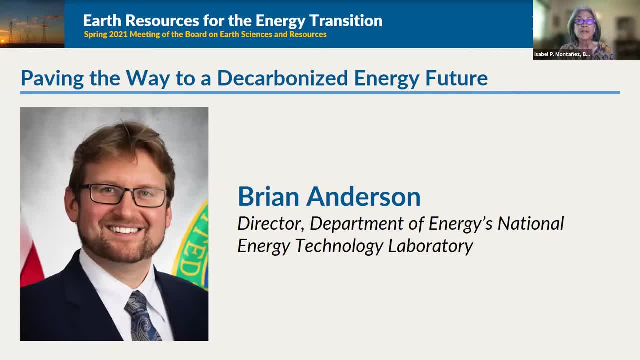 Paving the Way to a Decarbonized Energy Future. Brian is the director of the Department of Energy's National Energy Technology Laboratory And during his tenure at NETL he initiated critical technology development and development of energy technology. He has been a member of the Department of Energy's National Energy Technology Laboratory, And during his tenure at NETL, he has been a member of the Department of Energy Technology Laboratory. He has been a member of the Department of Energy Technology Laboratory And during his tenure at NETL, he has been a member of. 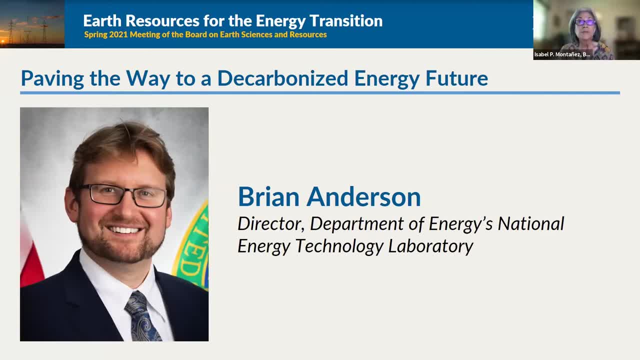 The National Research Association for Sustainable Development and забula projects, including direct air capture technologies for decarbonisation, chemical looping, combustion- with the potential to reduce greenhouse gas emissions, and nonvariable renewable energy for future low-carbon power systems. Brian's also guided the development and maturation of key technologies that are having 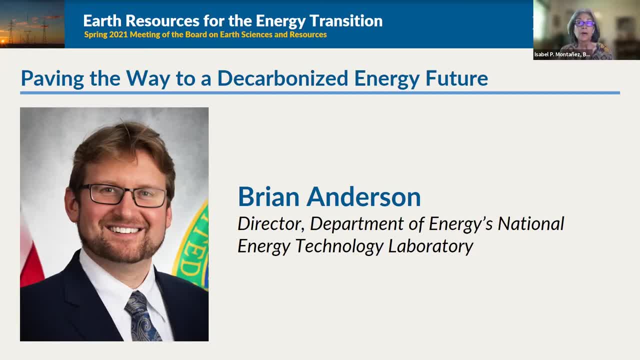 significant industry impact, including microwave ammonia synthesis and carbon nanomaterials. materials manufactured from coal And Brian has just been named executive director of the White House Interagency Working Group on Coal and Power Plant Communities and Economic Revitalization. Jim Slutes, a Beezer member, will be moderating questions. 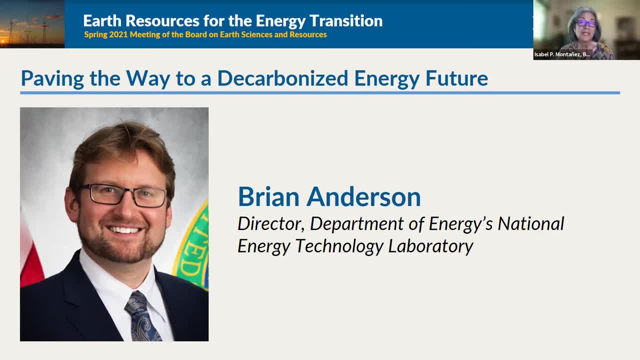 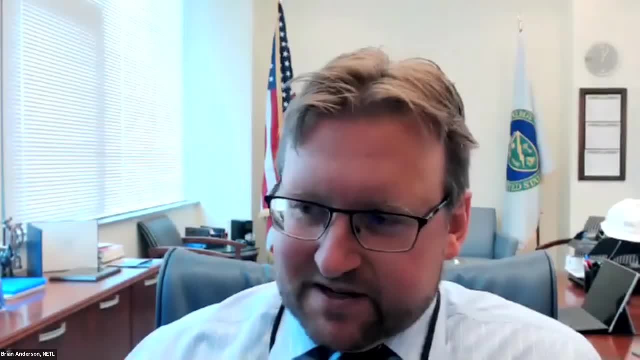 after Brian's talk: Thank you so much for joining us, Brian, And I turn the screen over to you now. Isabel, thank you so much, And the Beezer board: thank you for the opportunity to speak a little bit today about at least. 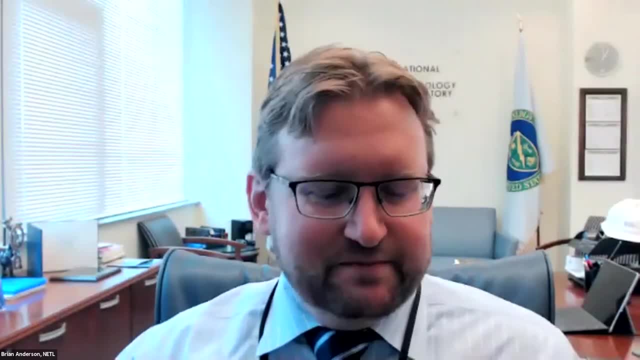 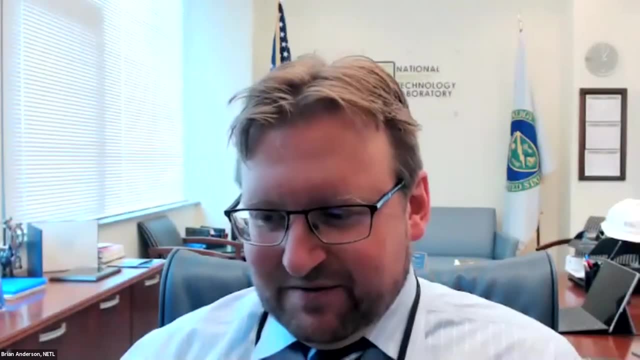 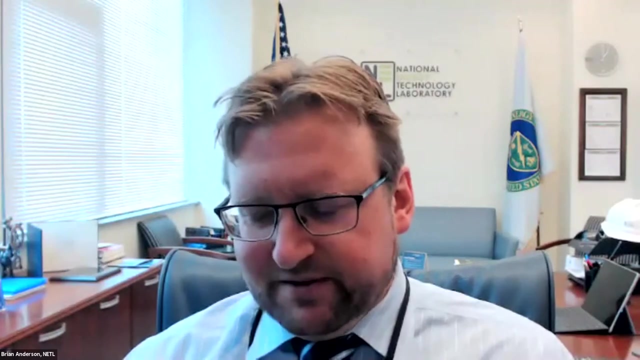 NETL's role and a pathway toward decarbonization. As Isabel noted, I've also, even very recently, been asked by the White House to lead an interagency working group in Coal and Power Plant Communities- Economic Revitalization. This is an 11-agency interagency working. 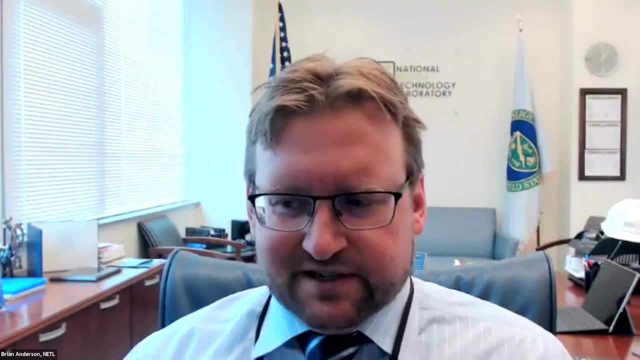 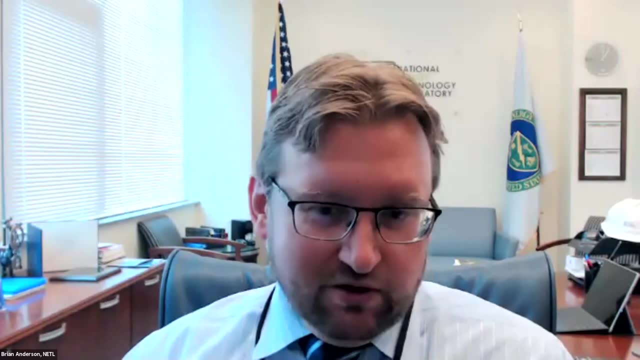 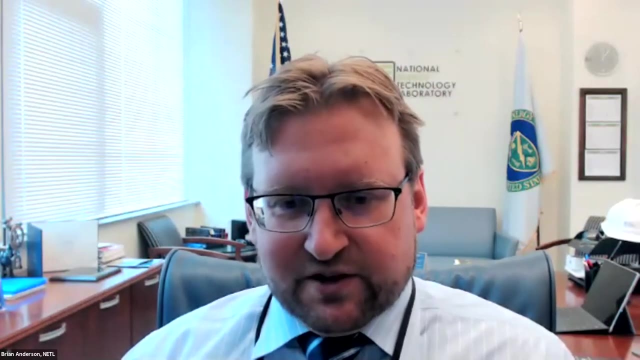 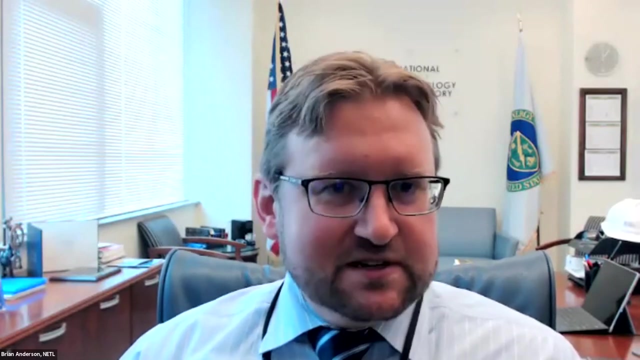 group spanning the entire federal government, because of the acknowledgment of the fact that, as we manage the energy transition, we have relied heavily on coal and natural gas and oil for more than a century in the United States, And those communities have built their economies around the earth resources that they have. 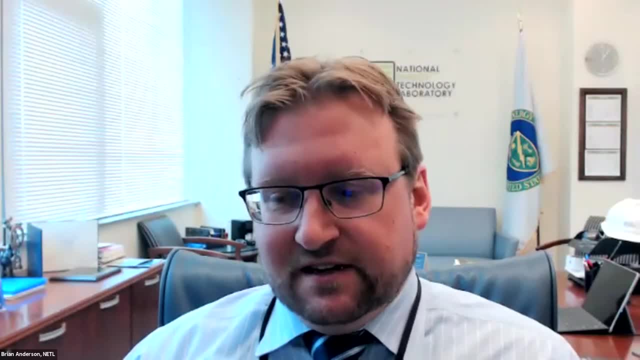 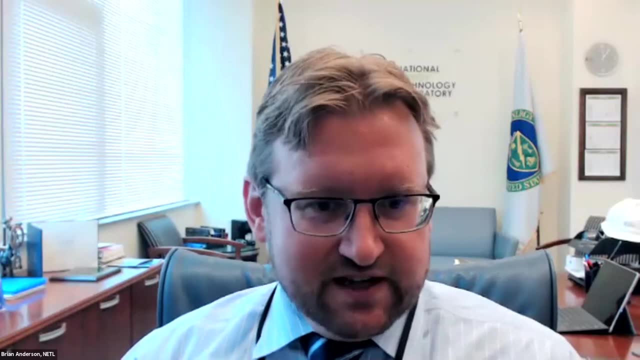 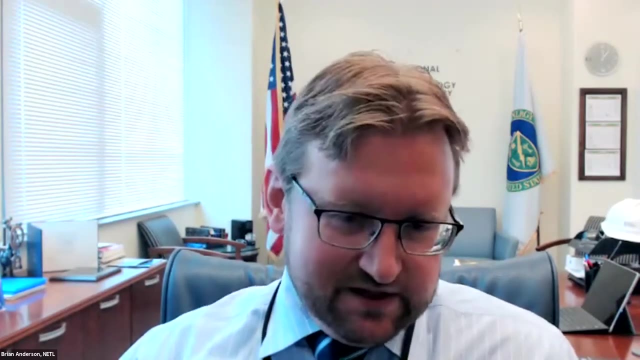 And so, when we think of the transition of the energy, our energy system, into the future, being able to manage the pathway and transition of these communities that are reliant on the earth resources themselves, how do we craft a pathway forward? And so that's part of the role of the interagency working. 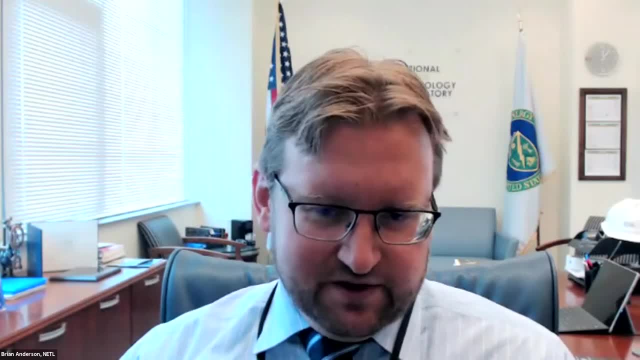 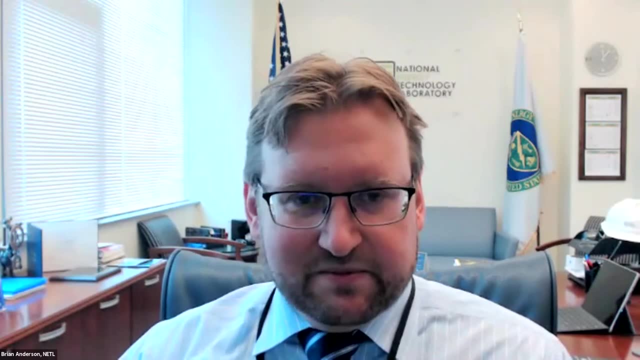 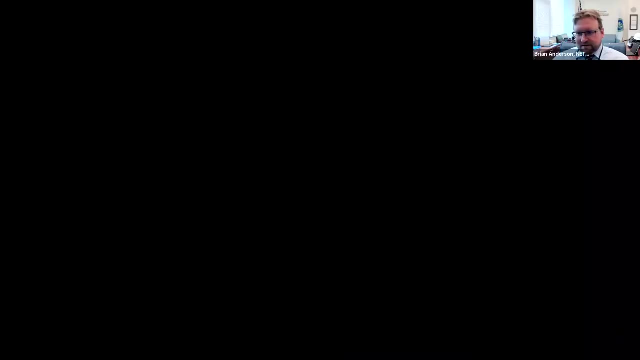 group is to try to identify the pathways and opportunities for those communities, And some of them may in fact be technical solutions like I might present today. So I'm going to go ahead and share my screen now and jump into the talk. I think it's great to speak to the Board on Earth Sciences. 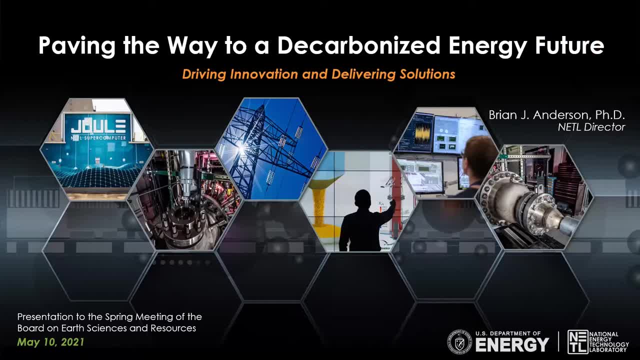 Resources, particularly because of the breadth and depth of the focus areas of Beezer, And I think that there's a real opportunity for us to rethink our energy resources into the future, knowing that today, 80% of our primary energy comes from the earth. 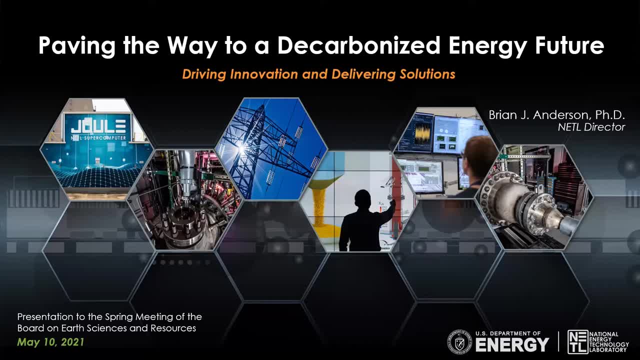 primarily. Well, 80% comes from fossil energy. Even higher number comes from the earth when we consider uranium as a primary energy source for nuclear generation, And so when we consider how we're going to pay the path for a decarbonized energy future. 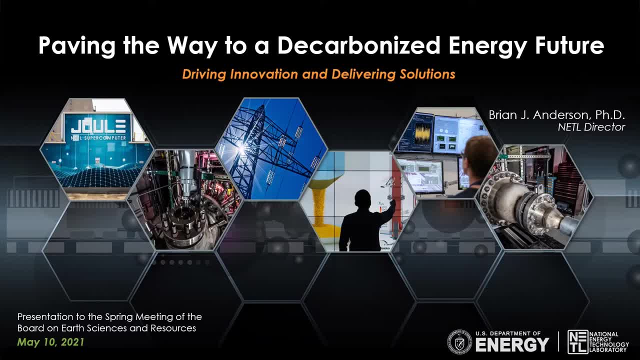 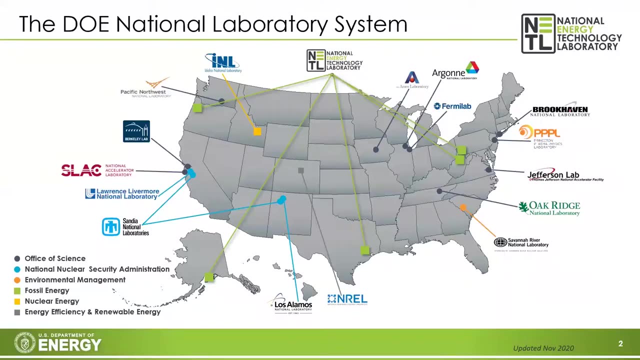 we have to include the subsurface- And it's really inherent to all of us- All of the various pathways that we might envision of getting to a decarbonized energy future, To set the stage for the role of NETL and the federal government. 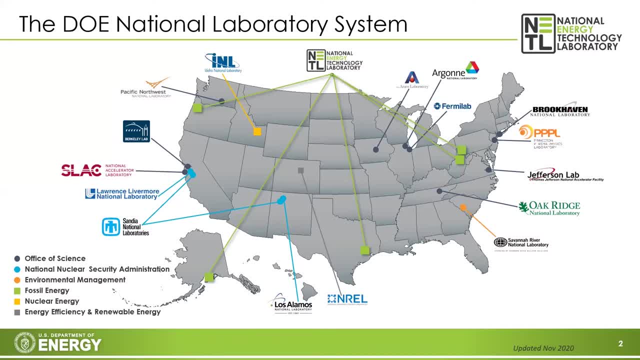 at least the Department of Energy. understanding that we have the Department of Energy National Laboratory System is important, that we have our 10 science laboratories, all shown here in the gray circles. These have our big user facilities, many of which have deep expertise And in our sciences and resources. 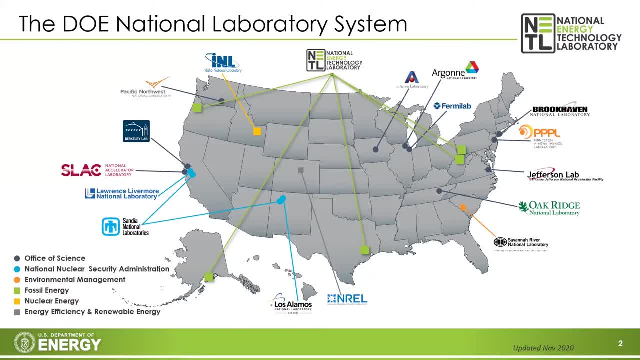 we have our three applied laboratories: The Idaho National Laboratory, focused on nuclear, The National Renewable Energy Laboratory in Colorado, focused on renewable energy, And NETL. as you can see, we have laboratories in West Virginia, Pennsylvania and Oregon, with field offices in Alaska and Texas. 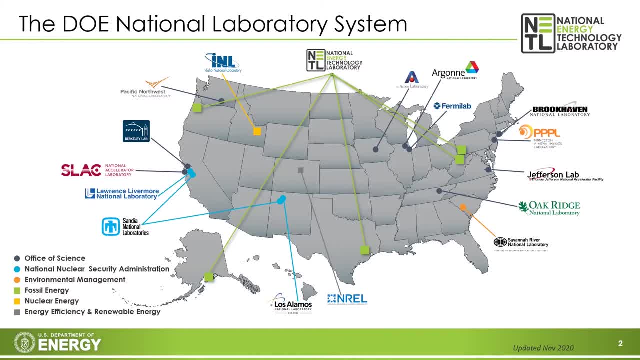 Historically we focused on fossil energy, But I would also add that for 25 years we've been developing technologies for carbon capture and sequestration. So in fact, we are the fossil energy, and carbon management laboratory is really our key focus area. 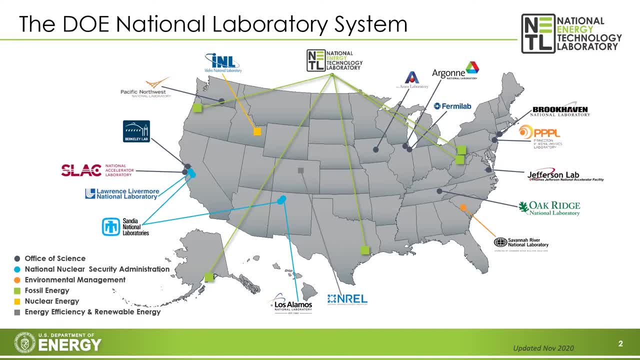 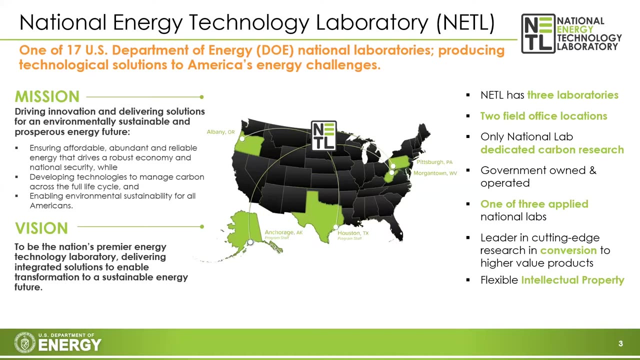 And one thing to note within our portfolio is not just fossil energy but as the Department of Energy's lone government-owned government-operated laboratory, we also steward some programs across the board. So our mission, which is actually recently revised mission of NETL, is to drive. 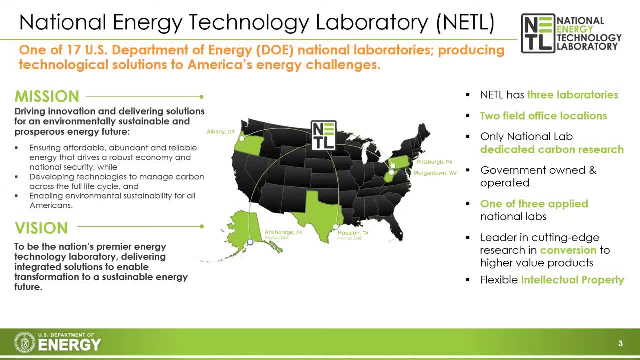 Innovation and solutions for an environmentally sustainable and prosperous energy future. And it's right at the nexus of environmental sustainability and a prosperous energy future where what we are focused on at NETL is to set out the goals of decarbonized energy system of the future, and doing it. 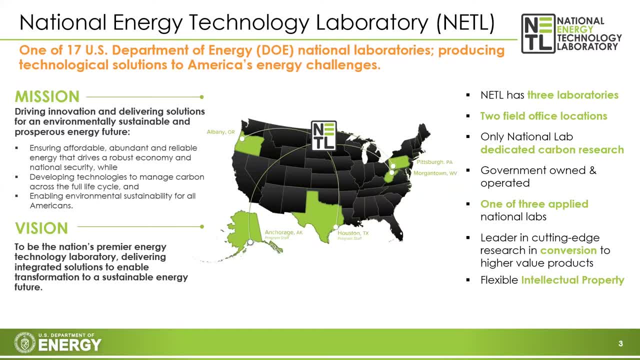 in a pathway that provides the optimal solution for the country, doing it as fast as we can and in a way that Decreases economic dislocation, increases energy justice and environmental justice in communities that have been impacted and will continue to be impacted by an energy transition into the future. 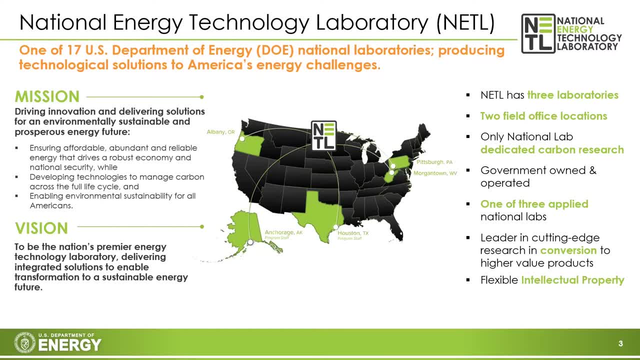 This is a really tough challenge to try to manage all of those goals simultaneously, And so we do it by developing affordable and abundant reliable energy through technologies that manage carbon and energy production, and that includes energy production and energy production across the full life cycle. 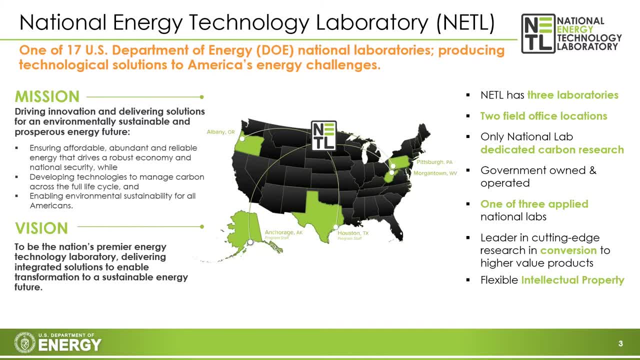 And that is a really important component- is to understand the full environmental impact costs of all energy production and being able to then manage and minimize environmental impacts, the negative environmental impacts, so that we can ensure environmental sustainability for all Americans, And this includes environmental justice in communities that have. 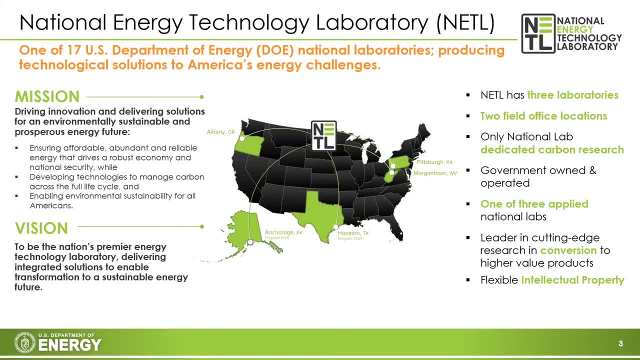 been adversely impacted by energy production In the past. Energy justice and energy jobs moving, moving forward into the future. And so the administration and in the national laboratory system that set out some really aggressive goals and constraints along our energy transition pathway so that we can- we can try to have a just transition. 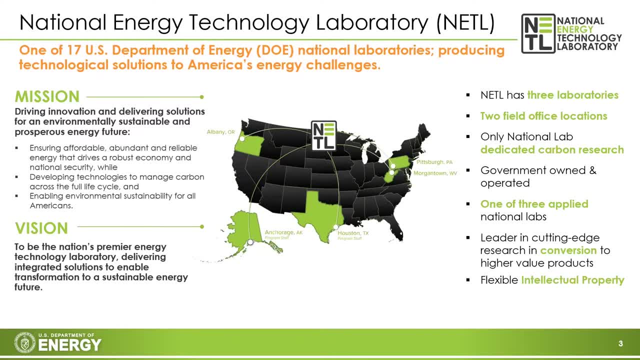 and many of you have heard that terminology and really to dig into what it means is that we have integrated, looking at our vision, that we have integrated solutions. That includes the transition of an economy, the investment of infrastructure, as well as the development of technologies that can achieve those missions of environmental sustainability. 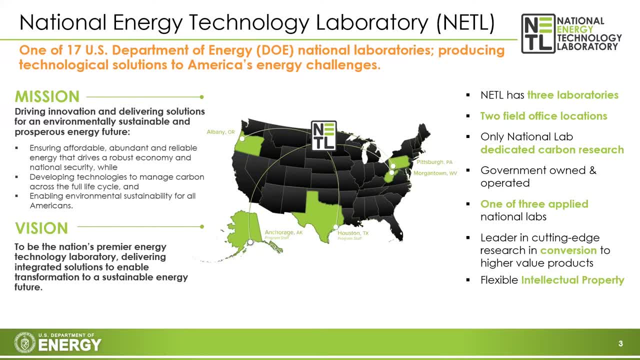 and a prosperous energy future. And so in ATL, you know I say here we're the only national lab dedicated to carbon research, And so that's carbon in the full life cycle through historically a lot of work in production of natural gas and oil, including work in the 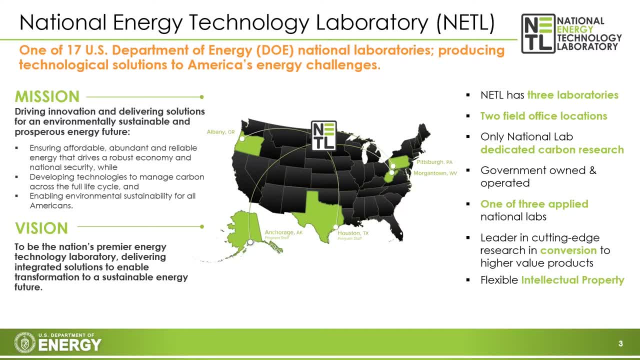 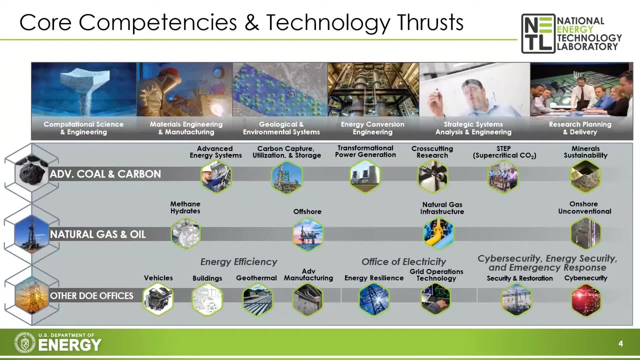 environment, to increase the environmental sustainability of shale gas production And how we can convert our carbon resources into higher value products and and then provide opportunities for for resource rich communities so that they're not stuck with a resource curse. I think that's really important in terms of adding value. 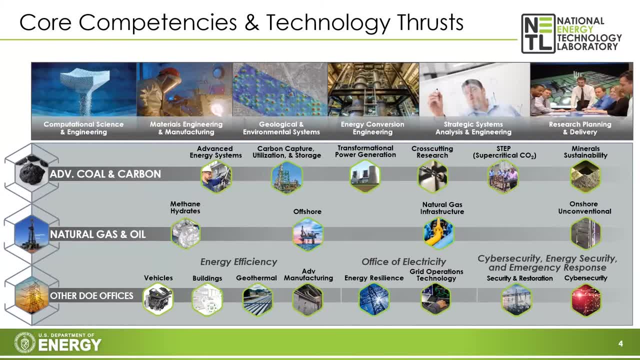 So to get to know any TL and in case you know- I know many of you already know that we're going to be doing a lot of research. We're going to be doing a lot of research. I know a lot of you on the on on the webinar today are familiar with us. 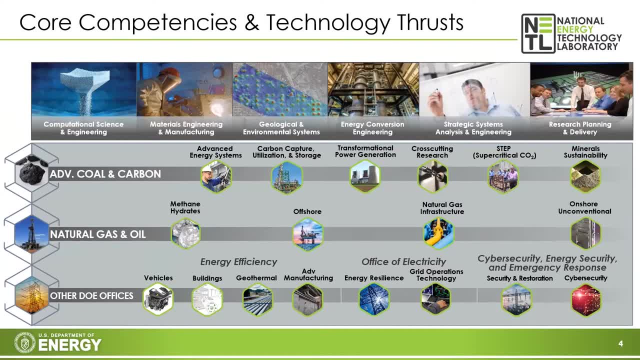 But to get to know us a little deeper, we have five core competencies in the Research and Innovation Center, which is our research arm. These are in computational science and engineering, materials engineering, geologic and environmental systems, which one would say is our BESER arm. 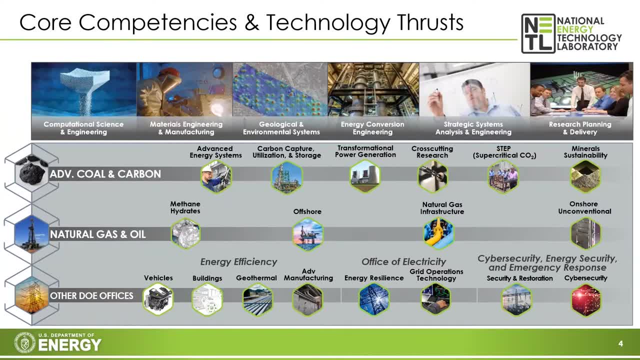 But in fact, our BESER work, work that's related to these are, is computational science and material science, energy conversion, engineering, and also in our strategic systems analysis. That includes the light cycle assessment work that we do, as well as energy systems modelling. 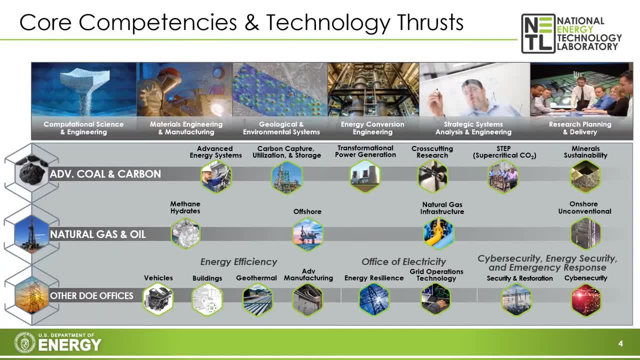 across the whole whole spectrum And the certainly the top two horizontal lines and coal and carbon and natural gas and oil are what we've worked on in our portfolio for over 100 years at our Pittsburgh facility and over 75 years and more in Albany. 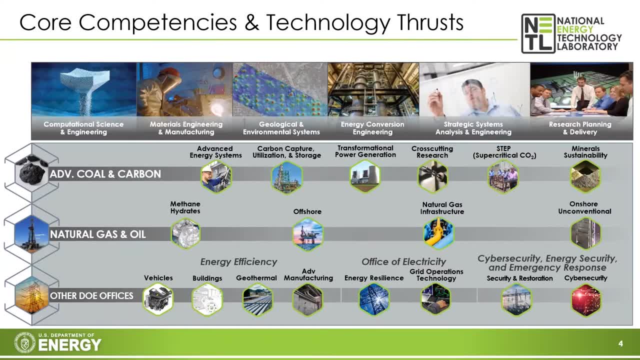 But we also work very closely with energy efficiency and renewable energy, energy managing a significant portion of the vehicles program and geothermal and advanced manufacturing and buildings, the Office of Electricity and CSER, Cybersecurity, Energy Security and Emergency Response. So when you package all this together, we really try to take 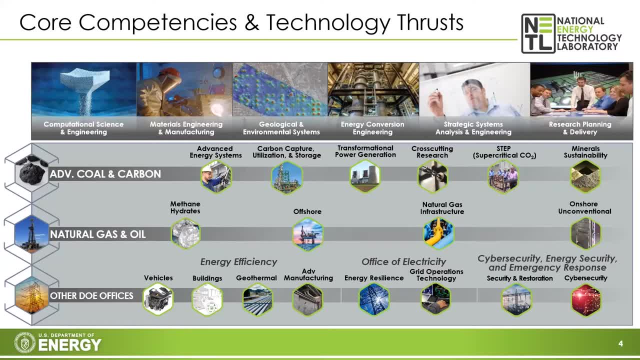 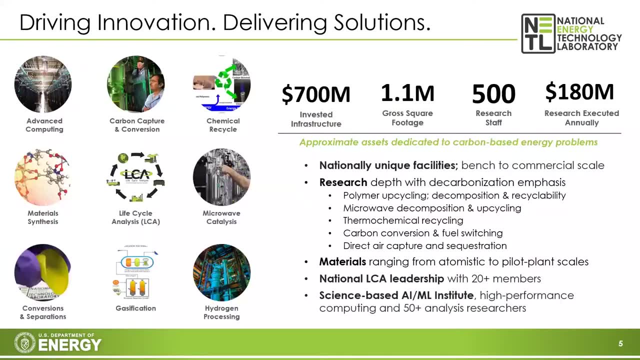 a holistic, systems level approach to the energy system as a whole- integrated energy systems- and then how we can manage the pathway of the energy transition to a decarbonized energy future. And so, when we look at the specific application areas, I brought up life cycle analysis, which is 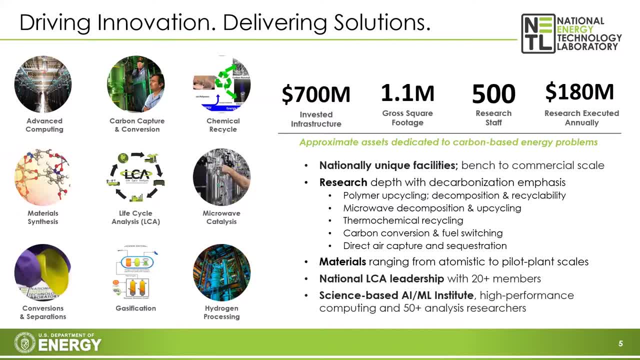 the middle of the nine boxes here, which really is core to how we evaluate the energy transition, how we evaluate new technologies that will come on to be able to manage not just carbon across the life cycle, including all of its potential emissions and greenhouse gases as a 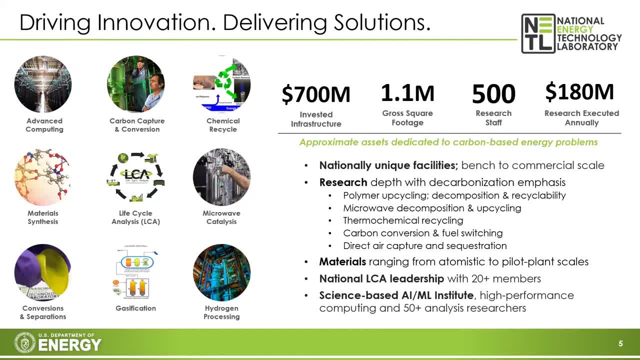 whole, but also the full environmental impact associated with energy production, of all energy technologies- And therein comes some of the things we'll talk about later today in critical materials, critical minerals, rare earth elements and things like that, And then another whole suite of technologies that we work on in chemical recycling. It was 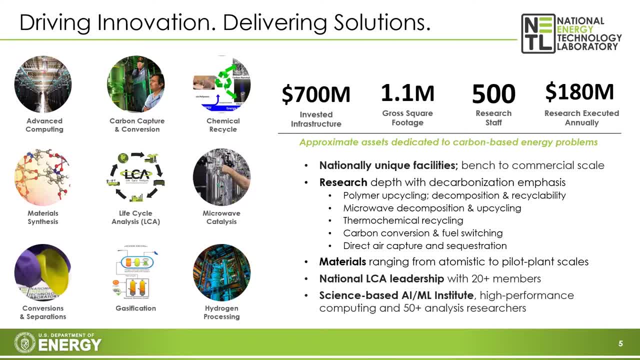 mentioned in the intro, microwave catalysis being able to lower energy barriers to even manufacturing processes- material synthesis, gasification, hydrogen processing and hydrogen distribution, And so we really have to do a lot of work to do that, And then we also have to do a lot of work. 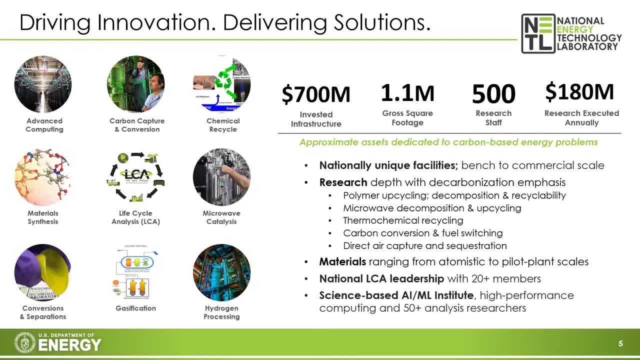 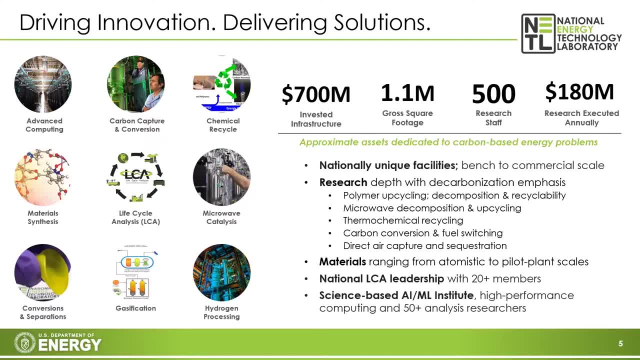 decarbonization as an energy carrier down the future. And so, again, our leadership and life cycle assessment really drives a lot of our decisions and investments in research, of technologies, of how to decarbonize our energy future. So this comes in. I mentioned the strategic systems. 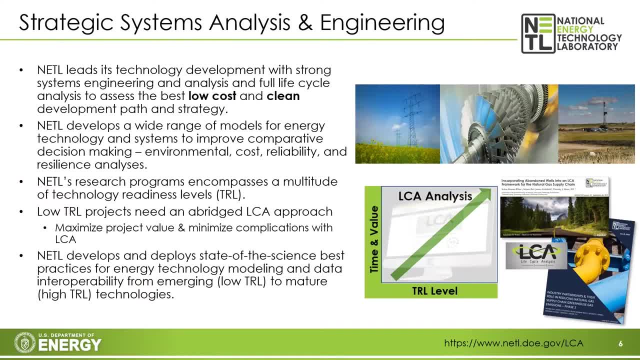 analysis and engineering When it comes to the life cycle assessment, techno-economic assessments and then the impacts of research investments on the goals that we've set forth for the aggressive targets of decarbonization. understanding the pathways that we can move along the entire energy system portfolio to again aggressively tackle the climate crisis. to develop technologies to reduce the carbon impact and full greenhouse gas impact of our energy technologies. 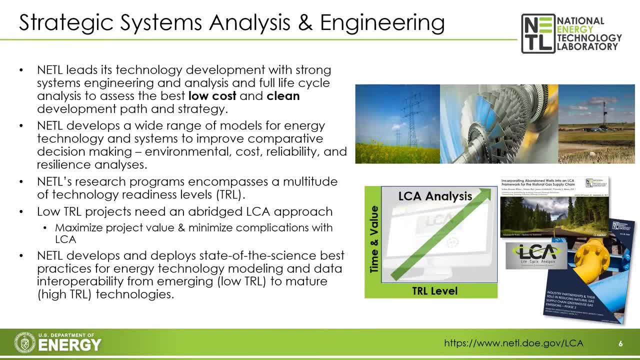 and doing it in a way that one can imagine a multivariable optimization process where a consumer constraint might be the goal of decarbonized electricity sector by 2035, fully decarbonized net zero economy by 2050,, but doing it across a set of decisions over these next 29 years that minimize any negative economic impacts. 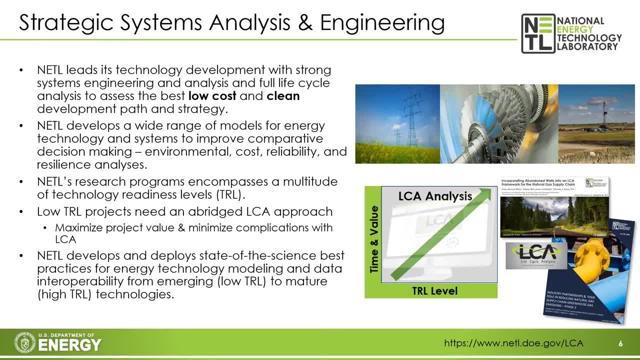 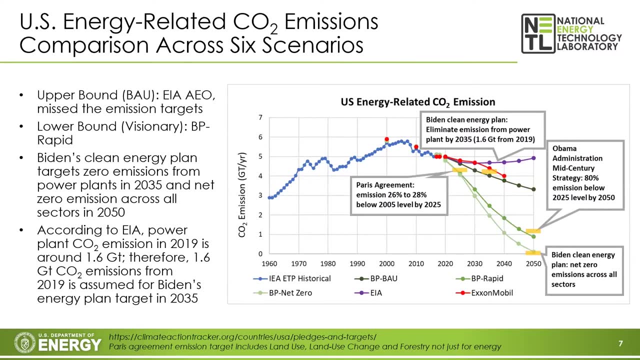 as well as optimizing the opportunities of energy communities, is really the grand challenge that we're working on, not just at any MTL but across the entire national laboratory system. So we think of the pathways to decarbonization. Here's just a sampling of some of the scenarios for CO2 abatement and mitigation and minimization of the energy system globally. 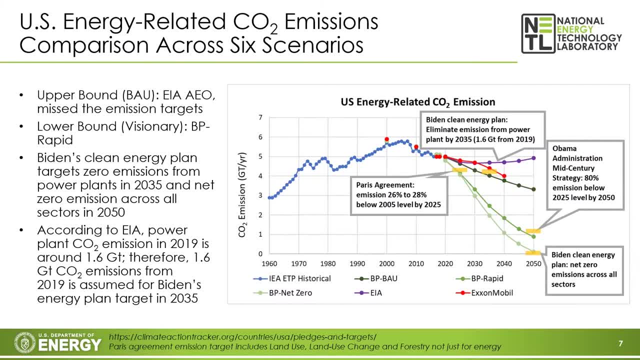 We look at the International Energy Agency, BP's net zero pathway, BP's business-as-usual pathway- there in green EIA's examples, ExxonMobil's scenarios And then the rapid decarbonization example from BP, And if we look at these particular targets, they all require very aggressive and very near-term action. 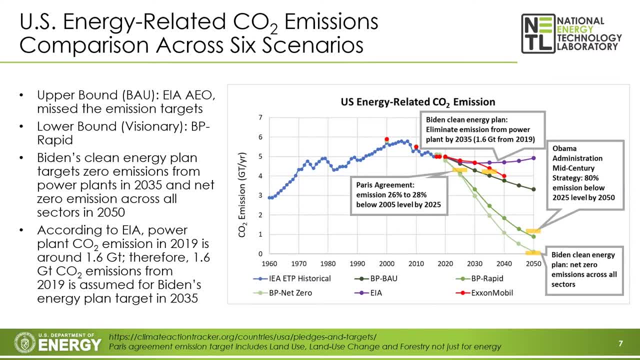 And certainly those actions have been taken. If you look at the trend line from 2000 down to 2020, there's US-related CO2 emissions that have been decreasing and, frankly, in large part to simultaneously deploying zero-emitting renewables. 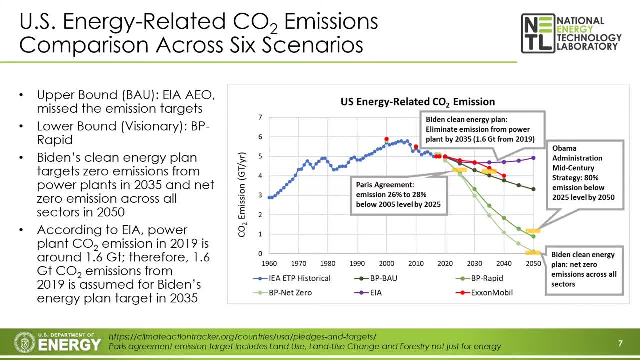 As well as a tremendous shift in the power generation fleet from coal into natural gas. We know that, you know, back just over a decade ago we were producing about 52% of our electricity from coal. Today it's 24%, with a large part of that shift going into natural gas and decrease in the emissions. 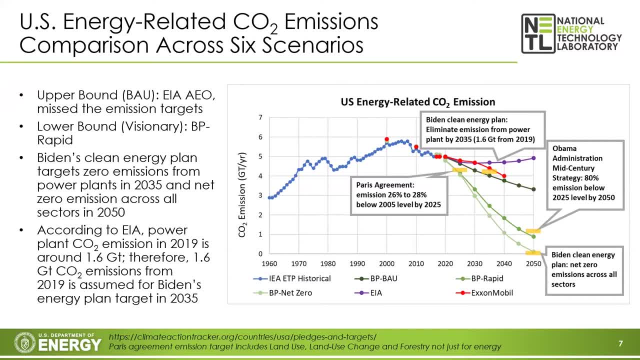 But that certainly opens up, as the folks at EDF have focused upon and thinking about equity and compliance, seeing how that may improve. but to run 10t-formum of factory power average, is that 50%, 40%, ch? What's going on? 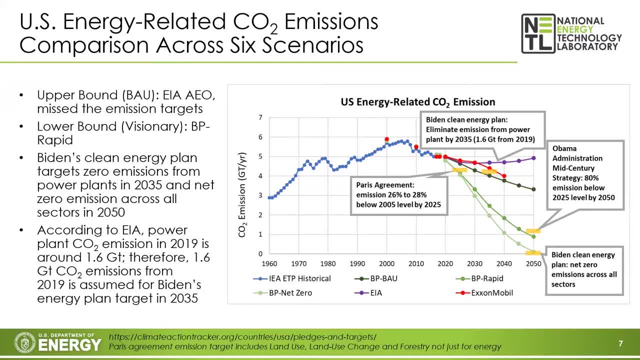 $50K ch. have very capably examined that has the potential of leading to methane emissions through the transportation and distribution of natural gas, which is again a major challenge. that's part of our portfolio is the methane emission estimates as well as mitigation targets. So anyway, you put. 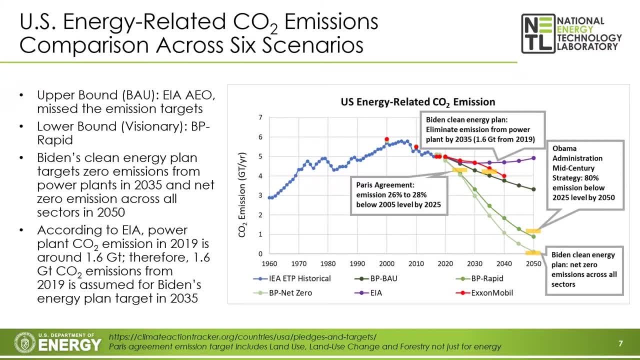 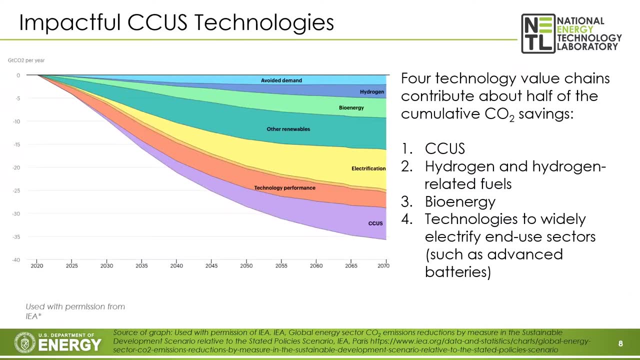 it all together and we need some very aggressive pathways to decarbonization to get to a net zero economy in 2050, shown only by the BP net zero example here on this particular set of six scenarios. So when we look at how we're going to build those decarbonization scenarios again, 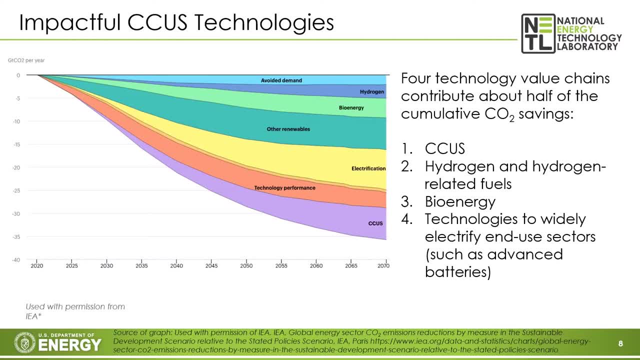 just one example of the pathway: the set of wedges of decarbonization as illustrated by the International Energy Agency, which very graciously allowed David Turk to step away from the IEA and join us in the Department of Energy as the Deputy Secretary recently. But the IEA has. 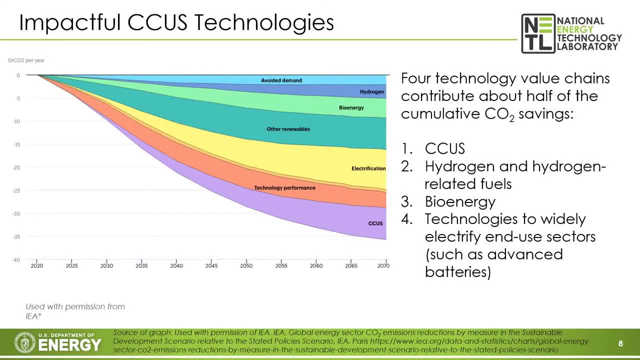 shown. all of the pathways include and certainly lots of electrification of the transportation sector, as well as the industrial sector, which is often overlooked when we talk about decarbonization pathways. Other renewables in addition to hydrogen. well, hydrogen is an energy carrier, not necessarily a renewable, but the bioenergy, wind, solar technology. 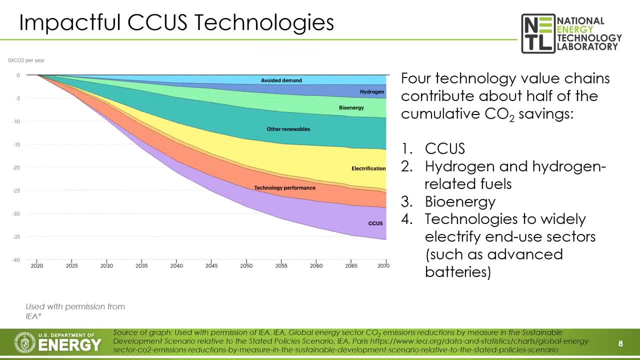 performance, to drive down or drive efficiency. they all require the onset of carbon capture, utilization and sequestration at some point in onset- and you can see that right now there's a lot of deployment of renewables. and then, certainly, when we consider some of the constraints specific to the electrical grid and increased demand of the electrical grid. 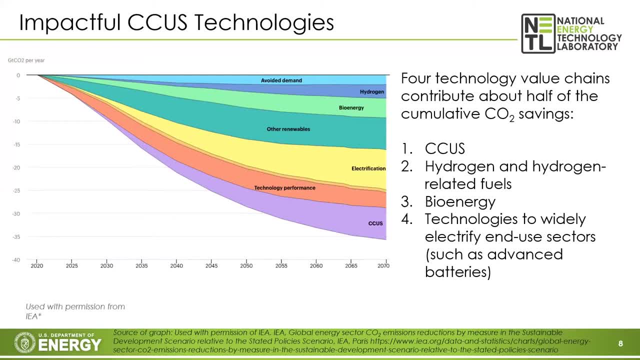 through electrification of industrial and transportation sectors, requires us to be able to deploy- хочешь 그러"- deploy low or zero carbon on-demand power generation, firm power that can provide the resilience of the grid that we so require. Now, certainly, there's been a lot of discussion around. 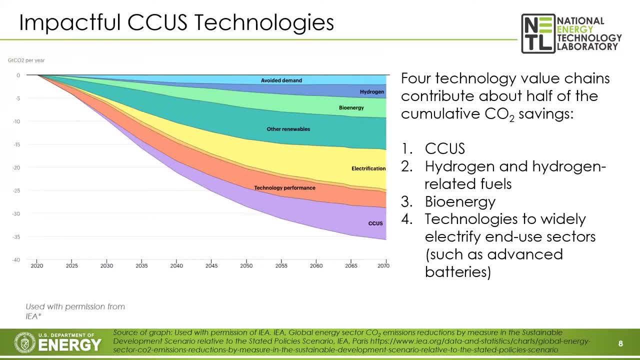 the polar vortex in Texas earlier this year and in regards to the blame or the share of blame that would be borne by all of the different components of the system under a very unique and rare polar vortex in Texas. But it does come down often to the 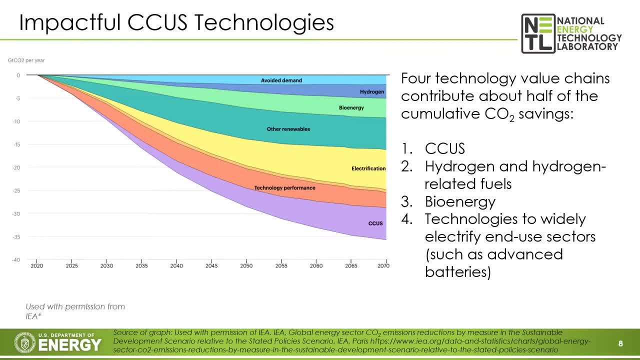 structure of the market. And so when we think of all of the technology solutions that we have at our disposal, be it load following and on-demand power generation, we think of the technology solutions that we have at our disposal, be it load following and on-demand power generation. 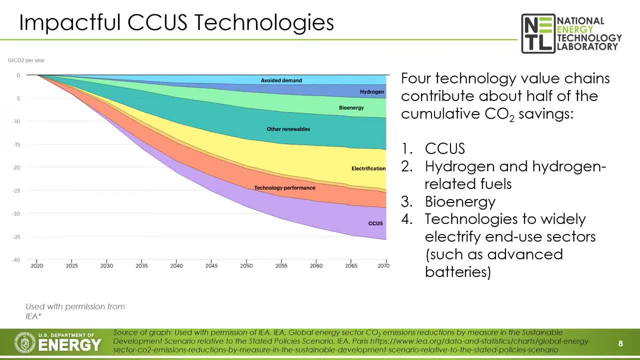 we think of the technology solutions that we have at our disposal, be it load following and on-demand power generation. in fact, a lot of the postmortem on the Texas incident comes down to the fact that there is a reserve margin that was low and the structure of the market and the lack of a capacity market. 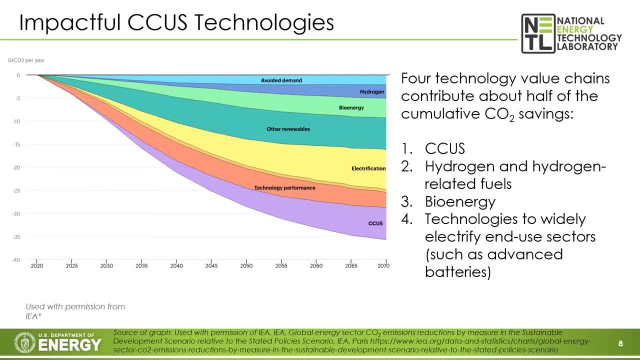 And so we can come up with all of the technologies that can solve many of our energy problems at low cost, but they all require some policy drivers or market solutions and market structures that are often not driven by technologies, in fact. And so again, when we look at the various 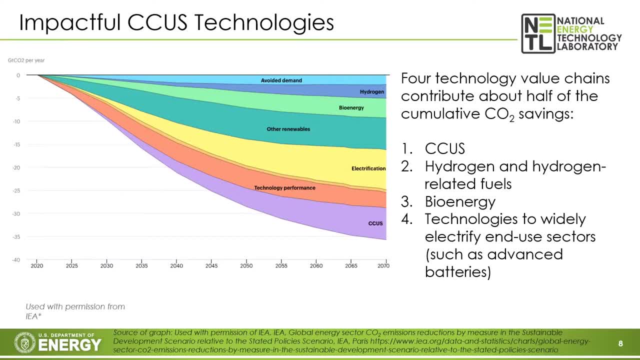 decarbonization scenarios, we do see a very strong need for the entire geosciences community to step up, not just in CCUS, for sure, but in the sustainable pathways of producing critical materials, producing the rare earth elements that we need to power the renewable economy, and then also, certainly, advanced batteries and the great 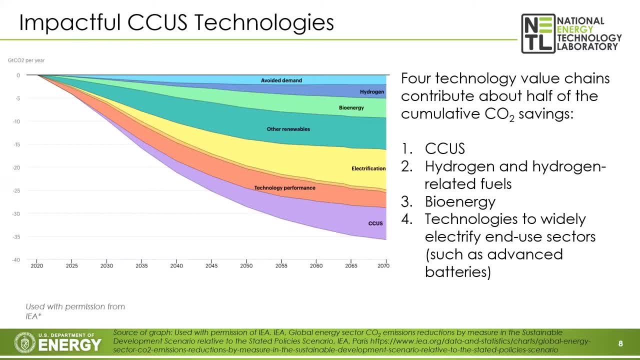 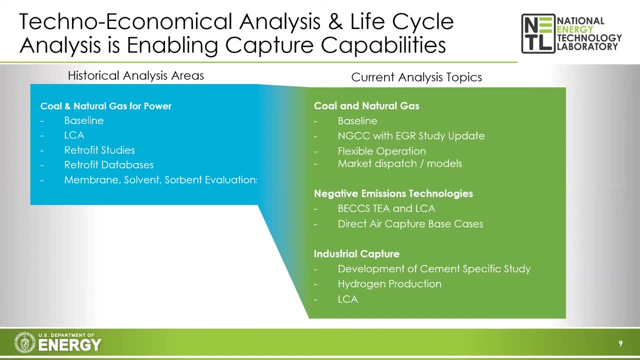 geologic needs associated with materials and driving sustainability across all of the sectors including, say, cobalt production in the Congo as one example. So, when we consider all of the different technology pathways, as we mentioned, we historically at NETL have 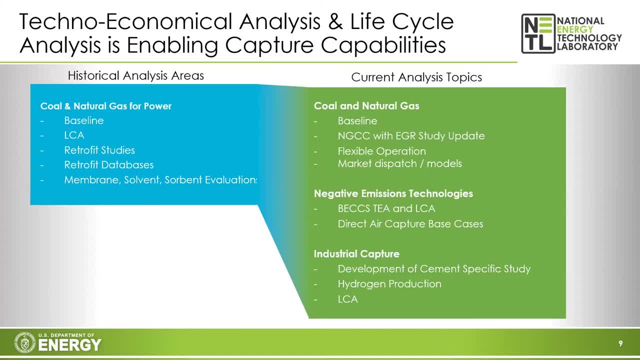 done baseline life cycle analysis, retrofit studies for coal and natural gas for power. But as we're moving into a rapid decarbonization of our energy system, we are now expanding our analyses to include certainly negative emissions technologies. It was mentioned in the intro about 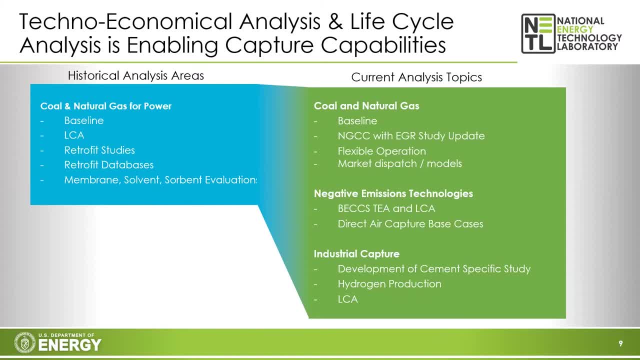 direct air capture as one of the levers that will need to be pulled when we get to deep decarbonization of those hard-to-declose energy systems. So we're going to have to do a lot of out. ain't all right when we start getting don't know? 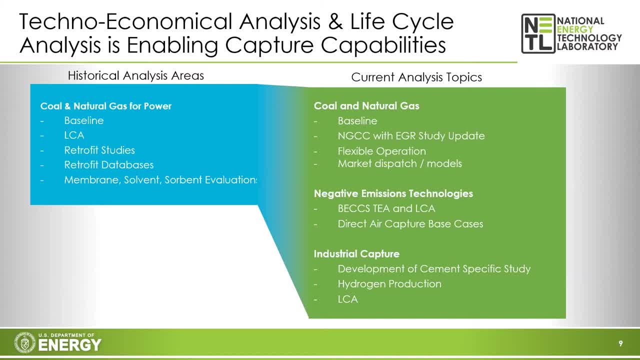 I think that also limits the way in which we'll decarbonize segments of the economy, particular around the industrial sector, where there are really difficult components of our economy to decarbonize. that we will need negative emissions technologies, including biomass energy with CCUS, that's, the VEX- and direct air capture. 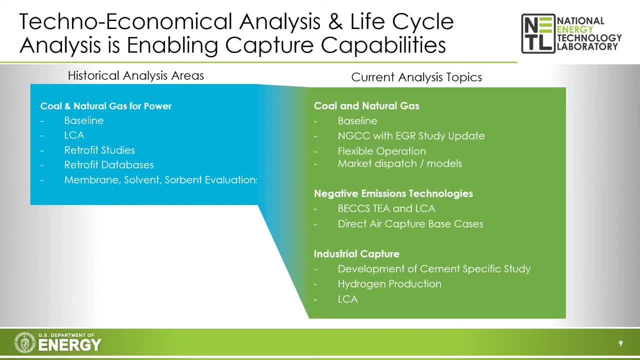 as levers to pull for us to get to a full net zero 363 00R sleeping coal fleet with accelerating retirements in the near future, as well as natural gas that is currently being deployed at a very high rate in the United States, and how we can retrofit or even 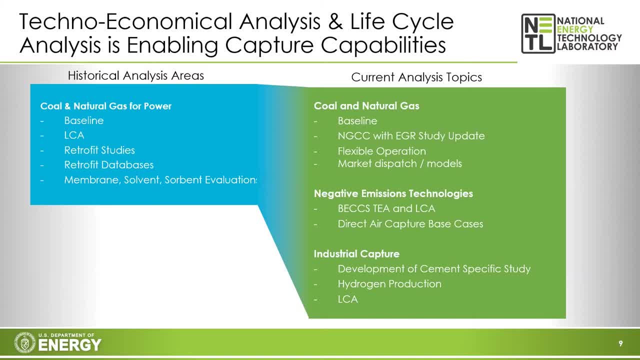 develop technologies that would be deployed in real time on the coal fleet and the natural gas fleet, so that we understand how to navigate the decarbonization pathway. And then, when we're targeting decarbonization of the entire economy, we must look at the industrial sector particularly. 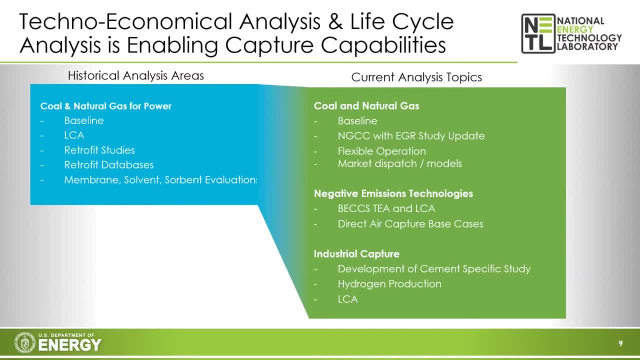 some of the heavy industry that has a very large CO2 footprint, like cement. I'm glad to see we're going to have some enhanced weathering discussion later in this meeting today, as well as some of the other issues that we're going to be discussing later in this meeting. 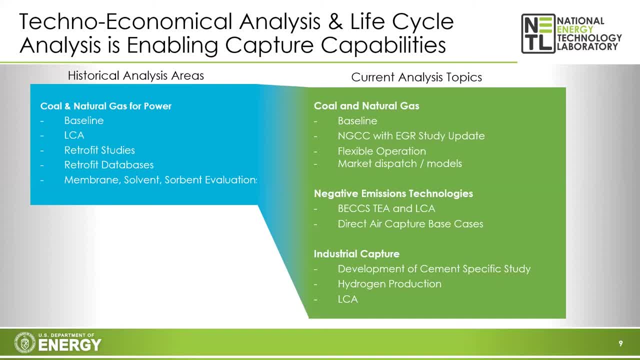 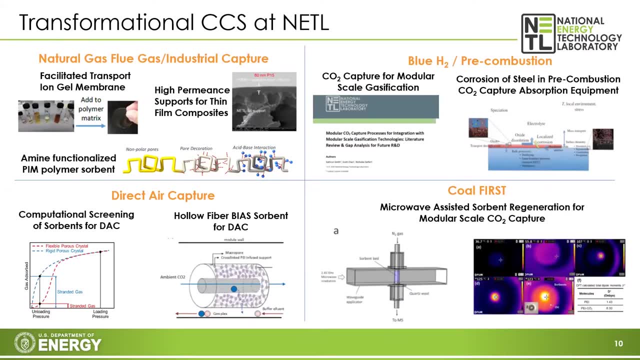 The opportunity for hydrogen production and then again, life cycle assessment. As you can see, there's a theme, So to give you an update of where we are in terms of carbon capture and sequestration technologies, looking across the spectrum from natural gas and industrial capture. 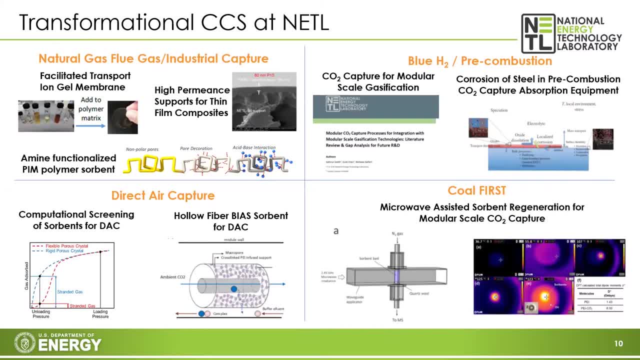 there's a lot of advances beyond the traditional deployed amine, amine sorbent and solvent processes that have been matured through the chemical industry or have been deployed on a demonstration basis from coal burning power plants. But when we look at some of the challenges and opportunities for 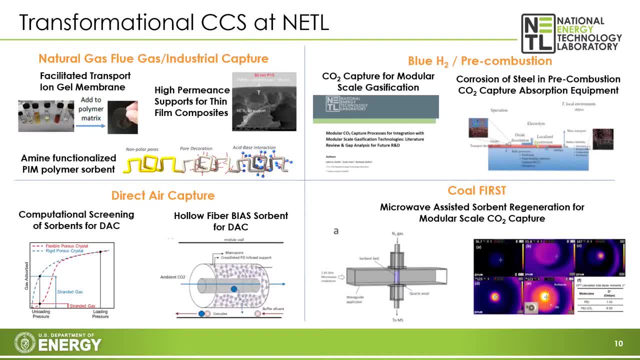 capture of different CO2 rich streams, like in industrial capture- often we do- we have high compositions of CO2 in the streams, not like in natural gas, where we might have 7% CO2, coal being 14%. We may have 50% CO2 in some industrial streams, And so a whole suite of 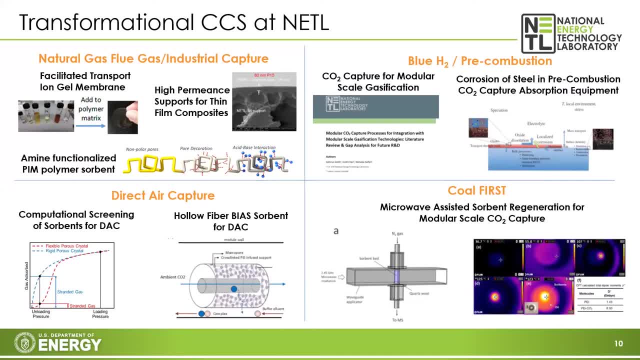 technologies to be able to capture carbon at low cost has been our focus. In the direct air capture space, we have started work in computational screening. This has been ongoing. As a matter of fact, one of our projects: we were able to screen carbon at low cost. We were able to screen carbon at 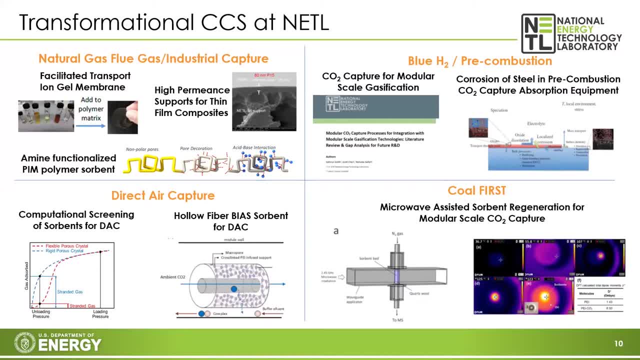 low cost. We were able to screen carbon at low cost. We were able to screen over a million combinations of a polymer organic framework with molecular organic framework. in a composite material with polymers. We screened over a million different types of materials, identifying four out of a. 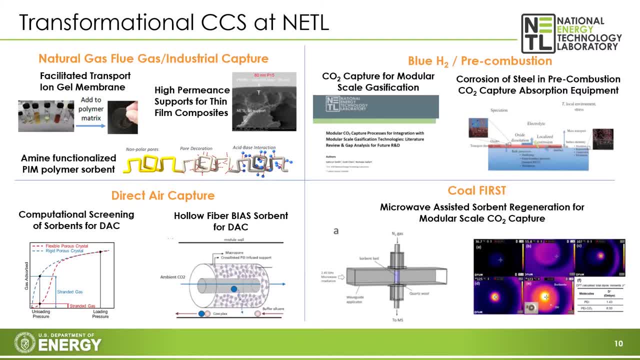 million- talk about a needle out of a haystack- to identify four that showed great promise and decrease in cost of capture using a hollow fiber sorbent, And we've also been developing this bias sorbent, which, in fact, is a particular type of material. 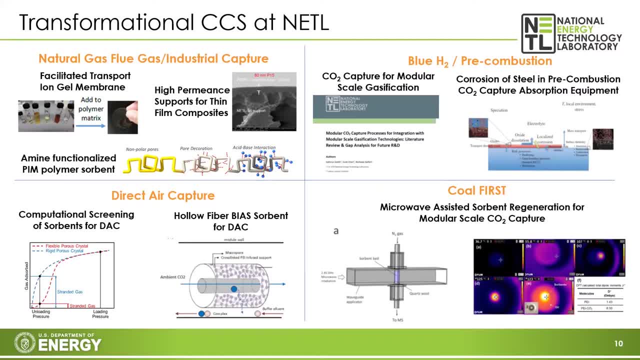 that can not only absorb CO2, but, as a matter of fact, is pretty useful to absorb things like lead and drinking water and even rare earths, as it turns out. And so in the direct air capture space, it is about capturing from a very low concentration- 400 parts per million- But we see a. 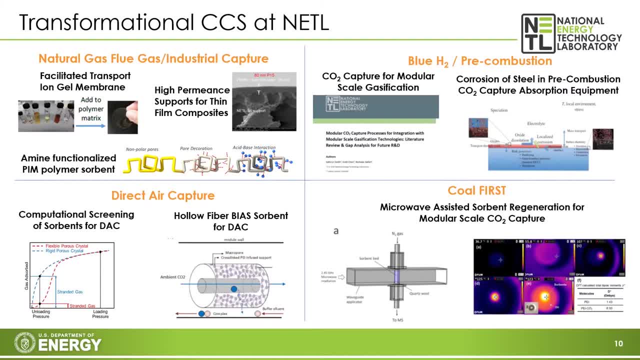 glide path for some of the costs of carbon capture and direct air capture not to reach the low levels of $30 per ton- That's our target for capture from industrial sources and coal and natural gas, but still some lower costs of capture that can come on again to offset some of the hard. 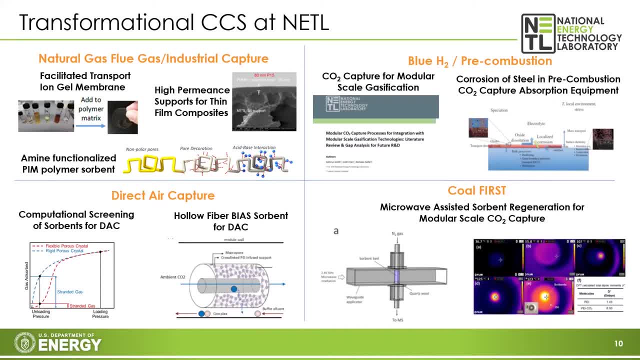 to decarbonize parts of the economy. Another big area is in using hydrogen as an energy carrier, where today the bulk, the vast majority in the 90 percentile of hydrogen that's on the market today, is produced from fossil resources, most of it from. 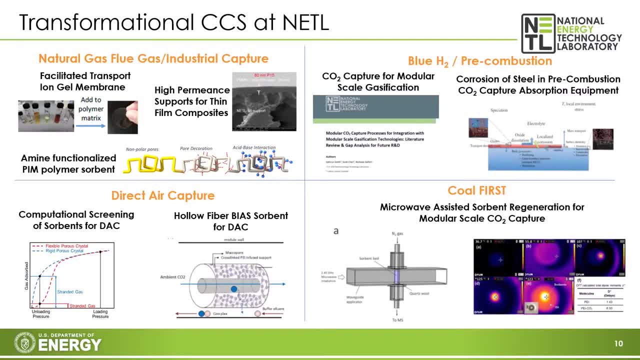 natural gas. If we can drive down the cost again of carbon capture for hydrogen, creating blue hydrogen, then we have an energy carrier that's not carrying carbon with it And again a tremendous potential to not only have hydrogen as an energy carrier and possibly a transportation sector. 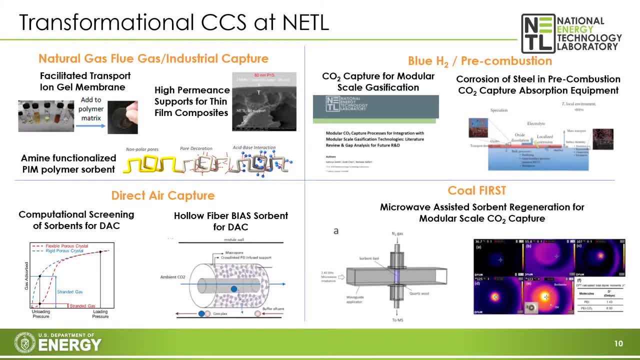 but certainly parts of the hard to decarbonize industrial sector, like steel manufacturing. for instance, there are options at the disposal of substituting hydrogen in for carbon-rich steel, for iron ore reduction, And then a program that was kicked off a couple of years ago in Coal First, 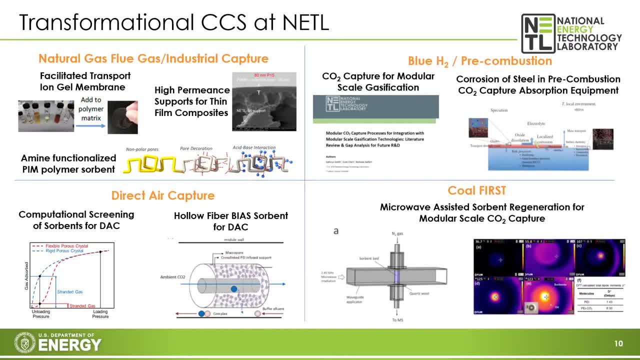 Coal First is about flexible, innovative, resilient, small and transformative technologies that are net zero CO2 emissions or even, in some instances, net negative with biomass. that are driving toward a modular, small energy production with modular CO2 capture that could possibly be deployed in the coal and power plant communities replacing CO2-emitting energy generation. 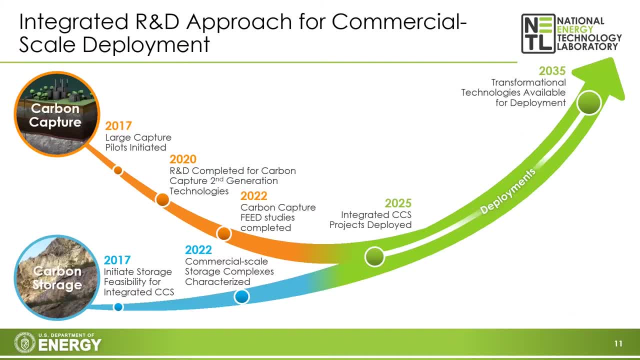 So as a goal for our whole integrated CCUS program, carbon capture and carbon storage. as you see on the timeline, we are rapidly approaching integrated CCUS projects to be deployed And these are the second-generation CCUS technologies that have been demonstrated at the laboratory scale, scaled up at a test facility called NCCC, the National Carbon Capture. 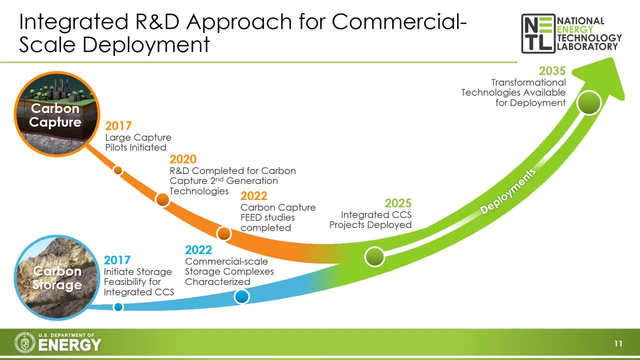 Center in Wilsonville, Alabama, sometimes deployed in Mondstadt, Norway, for scale up. And then again going back to the need for policy drivers. 45Q, as the tax credit for CCUS projects is providing a bit of the market pull for technologies to then be deployed by 2025. 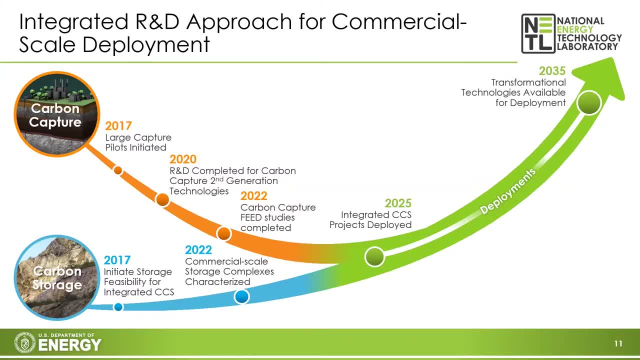 Now we, then, are driving toward transformational technologies deploying over the next 10 years. These transformational technologies have cost drivers driving down the cost of carbon capture to $30 per metric ton of CO2, or even lower, And one of the real challenges is understanding. 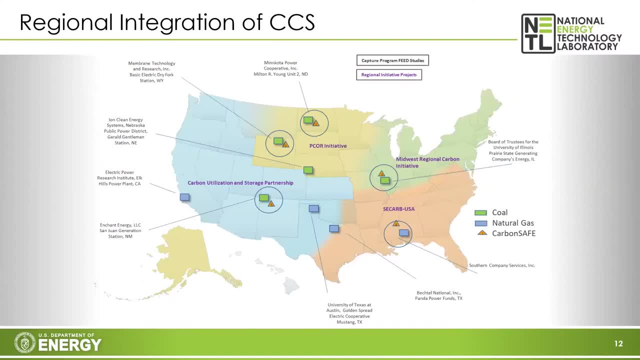 how the CO2 will be sequestered in the subsurface, And we have spent many years with partnerships across the United States to first, characterize the potential for CO2 sequestration in the subsurface. Secondly, the potential for permanence of the CO2 in the subsurface. Third, to reduce the 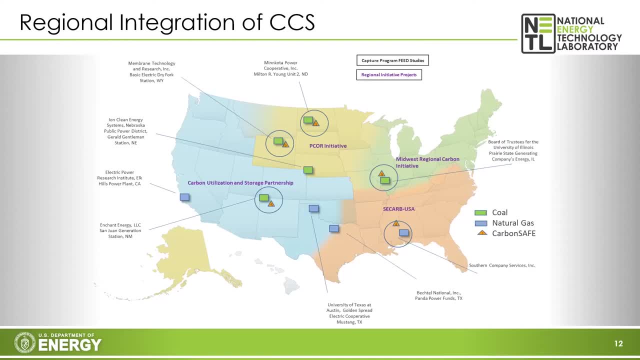 risk, that risk being a risk of leakage, risk of induced seismicity for large-scale carbon capture and sequestration. And, as we see, we're integrating the CCUS projects regionally. We have the regional partnerships, as well as programs called Carbon Safe, which is about the safe storage, long-term storage. 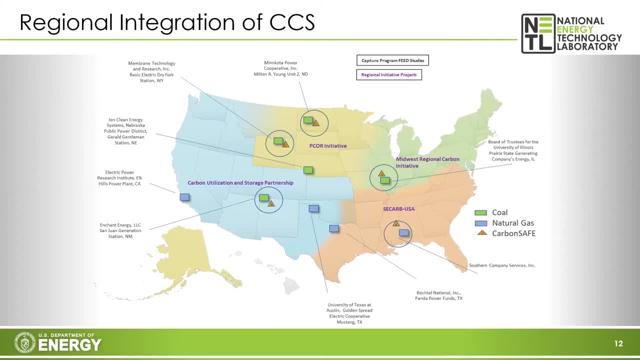 permanent storage of CO2 in the subsurface And we really are starting to have a great understanding of how these technologies are going to be used in the future. And we have a lot of understands of how these technologies are going to be used in the future And we really are starting to have a great understanding of the potential in the subsurface. And now we would need all of the surface infrastructure in place via CO2 pipelines and the carbon capture. 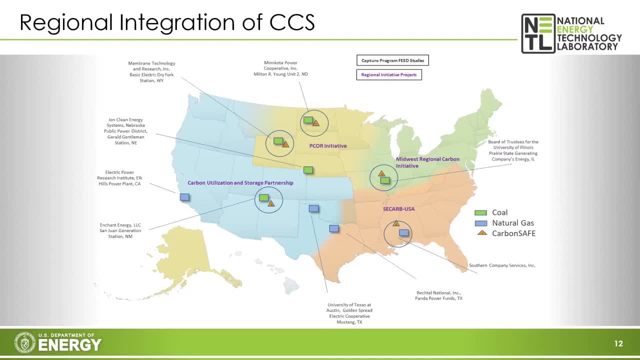 system as a whole. N- Here's the last one, n- here's the last one- d, p, a, y, f, c, i, l, y, n, s, nd, n, d. the constraints around resiliency and reliability and the ability to have firm net zero power on the grid. we do need to deploy CCUS in the subsurface. 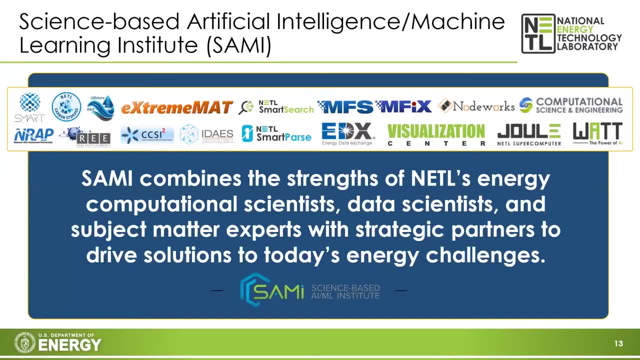 All right. so changing slightly, changing the focus, but the application still being the same, we have kicked off an institute called the Science-Based Artificial Intelligence and Machine Learning Institute, which its focus in SAMI is really. it's about physics-based- or here you can say science-based- artificial intelligence and machine learning. to where 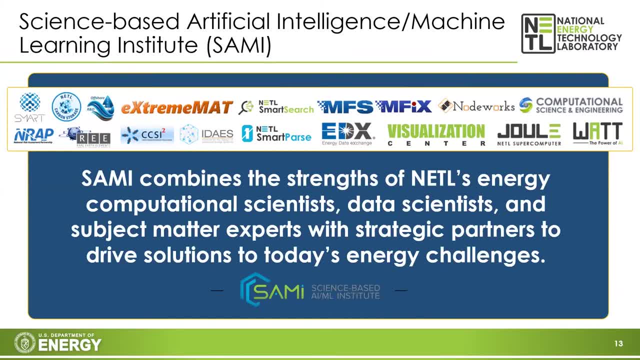 instead of historically, and this is not a knock on data science or artificial intelligence or machine learning, but to date, most of the algorithm development in AI and machine learning and large data analytics have been focused mostly around empirical models and using the structure of the algorithms and the learning algorithms and the computational 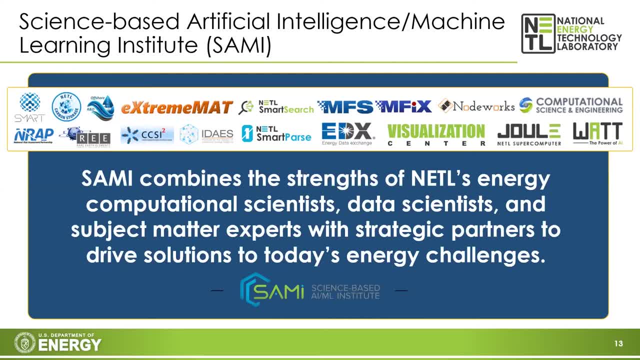 science space focused on empirical models, even using neural networks and smart learning algorithms that are not always driven around science-based models, And so our focus is to bring the science-based models and subject matter experts on the physics of a system, the data scientists and computational scientists to have this focus on physics-based models coupled. 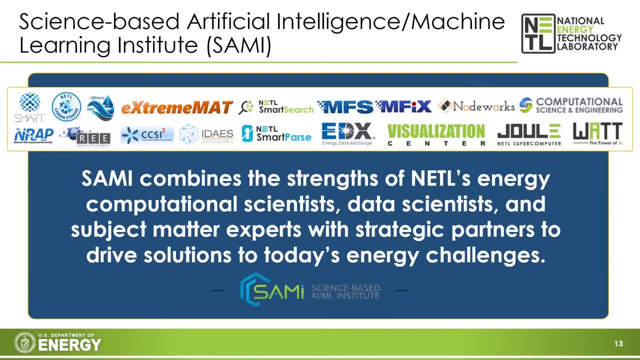 with the artificial intelligence strategy And so the whole logo soup. around the top are a number of the different projects or platforms that we have used, or across the national lab system have used to try to drive towards physics-based and science-based artificial intelligence machine learning. The top left one see there is SMART. That's specifically on the subsurface. I'll talk. 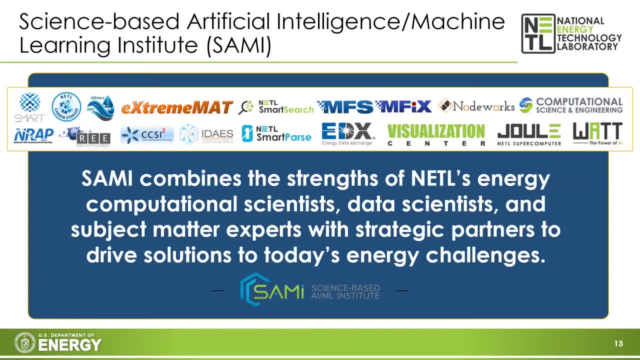 about that a little bit more. But then other examples. one in particular right in the middle bottom, EDX, the Energy Data Exchange, is a data platform with SMART algorithms built into it for how the data come in and adding metadata so that these data-rich environments are informed. 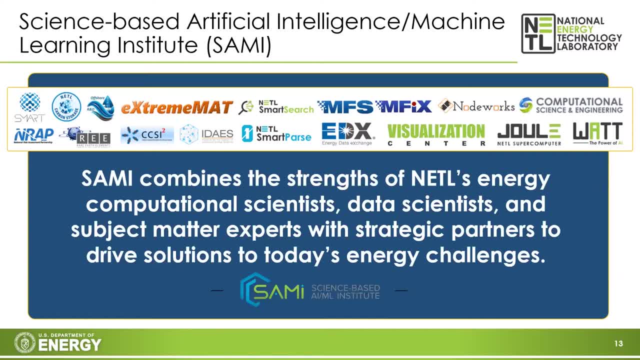 by SMART, By the situational awareness of data collection, And then one other particular example, IDEAS, which is on the bottom row. the fourth one over IDEAS is our Institute for Design of Advanced Energy Systems And, like the others, like SMART and EDX and XtremeMAP, this is a collaboration of multiple. 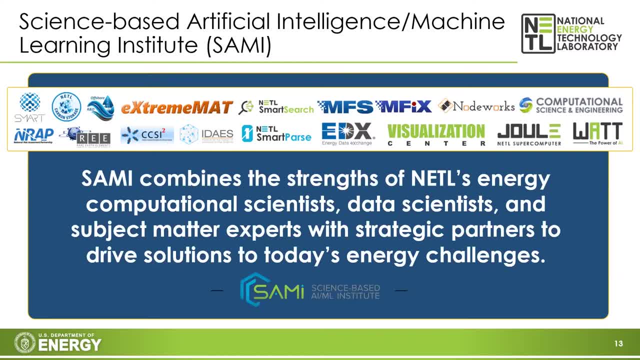 national laboratories. It's Berkeley National Lab, PNL, Sandia, Los Alamos, NETL and this and some activities, And then we have other academic institutions like Carnegie Mellon University. This is an entire platform built to be able to bring in science-based models, couple it across time and link scale and 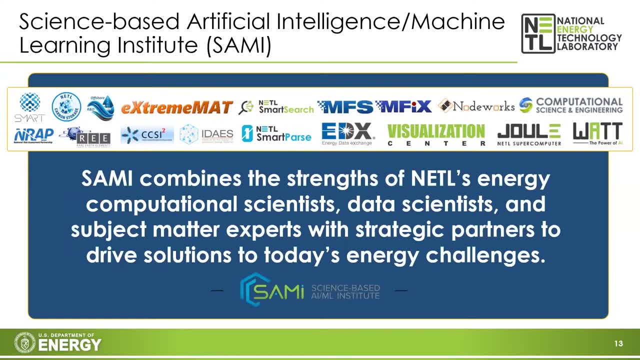 IDEAS can in fact simulate all the way down to a material in a power plant, up to how the grid works on a day-to-day five-minute-ahead grid market. so we can understand the effects of cycling on the grid, on the materials themselves within a power plant, And so to move from those time and link scales, 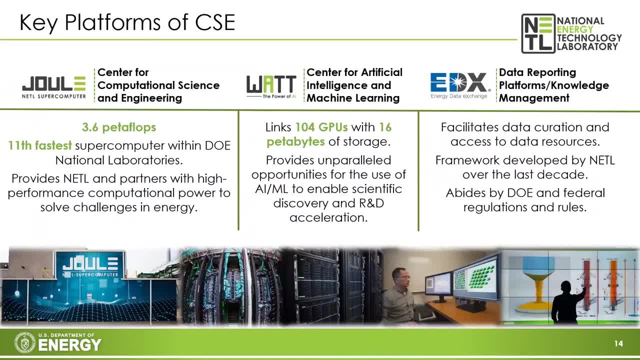 is really a tremendous, tremendous breakthrough. So we have some platforms. I've mentioned EDX, We have our Joule supercomputer and our Watt Center for Artificial Intelligence and Machine Learning. Watt's actually the name of the computer itself That is focused on data science. 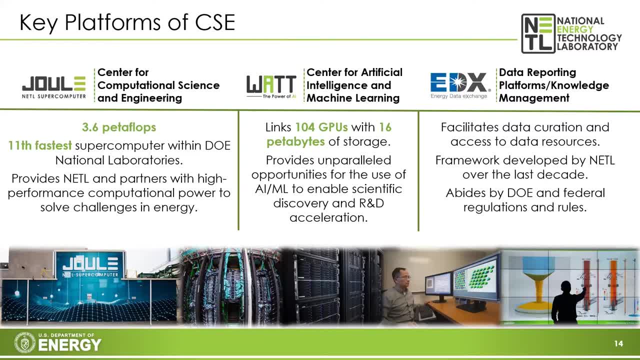 And, in particular, on the next slide I'm going to talk about data science and subsurface. It is specificWatt is specifically designed for very fast ingestation of data and the ability to analyze across huge data sets in rapid time. And we're at the point in human computational 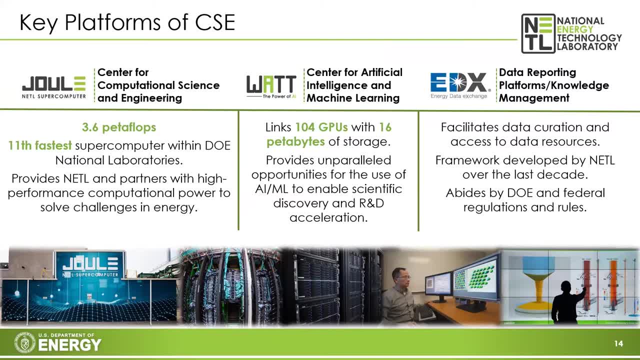 systems that we don't understand how big 16 petabytes are. In fact, 16 petabytes would store the Library of Congress, the world's largest data collection. would store the Library of Congress 1024 times And the speed at which we can ingest that data. if you took the Library of Congress. 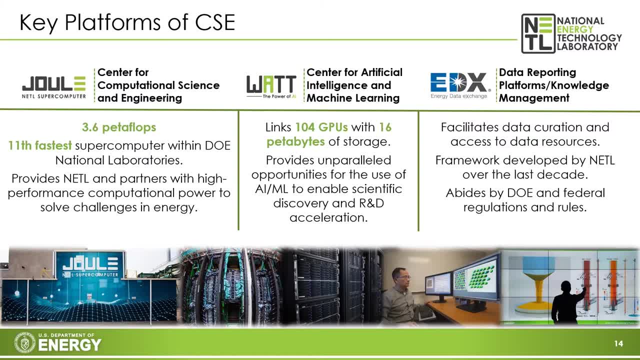 printed it out on eight and a half by 11 sheets of paper, one-inch margins, 10-point font, double-sided and cheap paper. it would stretch from Washington DC to St Louis and we can read it in about four miles per second is how fast we can read and analyze, not just read. but 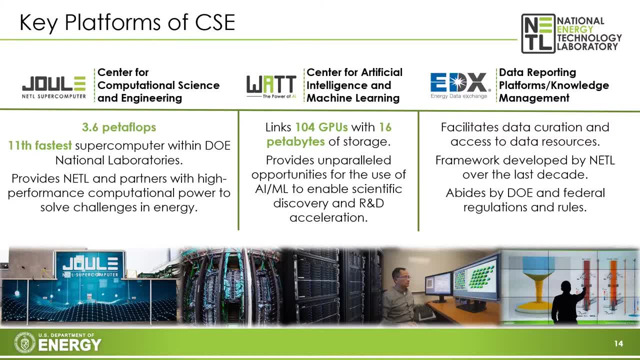 analyze that data, And this is important because the data sets we're facing in the subsurface are becoming very large. We're going to have to do a lot of work to make sure that we're getting the data and the ability to ROA and the ability to do the actual analysis of the data And so, within the 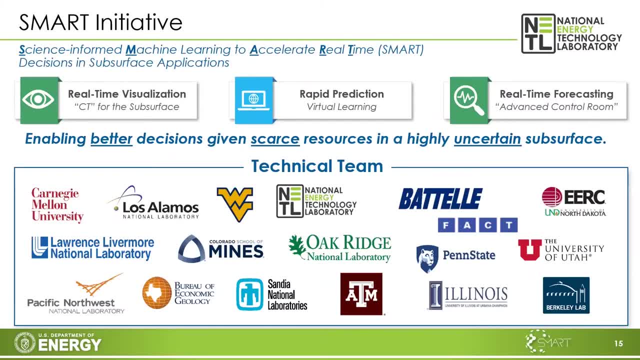 large, very large, yet often sparse, And so that presents some interesting computational challenges that we're trying to attack in the SMART Initiative. So the SMART Initiative is how we can use science-based artificial intelligence and machine learning to accelerate an understanding of subsurface processes, And so you can see we have a pretty broad technical team all focused on 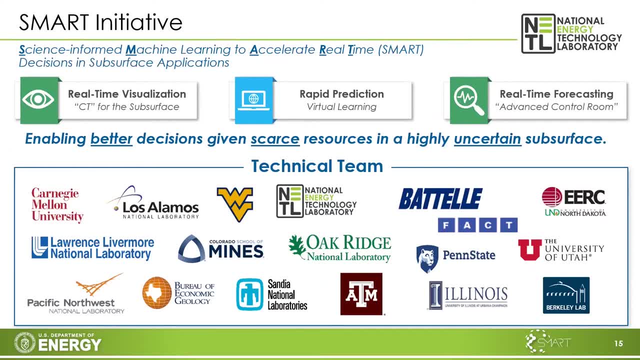 how we can better adapt our understanding of processes that happen in the subsurface chemistry to fluid flow, even to the propagation of hydraulic fractures, and the application space is in carbon sequestration as well as oil and gas production and the long-term ramifications. 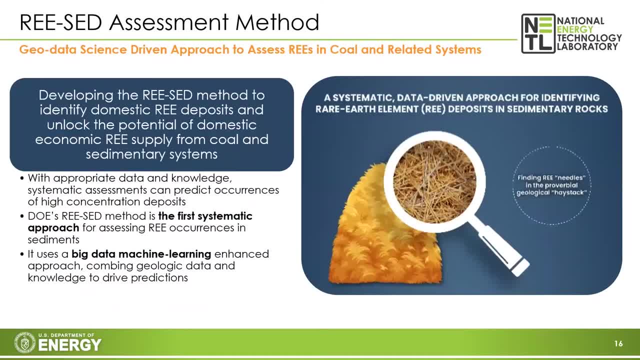 of CO2 storage. Another area of unlocking the potential in the subsurface by using data-driven assessment methods- and this is largely driven out of our Albany laboratory with our pretty deep geospatial data analytics capabilities- is a new method to assess the rare earth element. 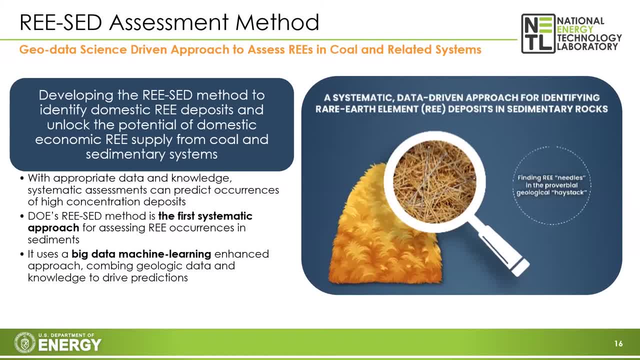 potential within sedimentary environments. so that's already said, And so it's this geodata, science-driven approach so that we can assess rare earths and coal and other sedimentary environment systems, So that we can Understand and identify the potential for extraction of rare earths from our existing. 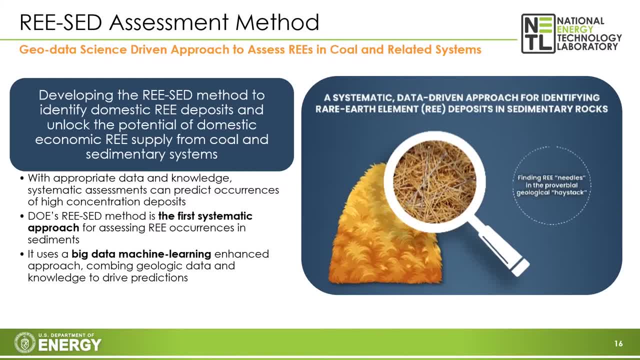 resources as well as our environmental remediation opportunities, be it acid, mine, drainage sludge or ash ponds that contain a significant amount of rare earth elements that could be driven into our US supply chain of rare earths that are so critical to everything from the. 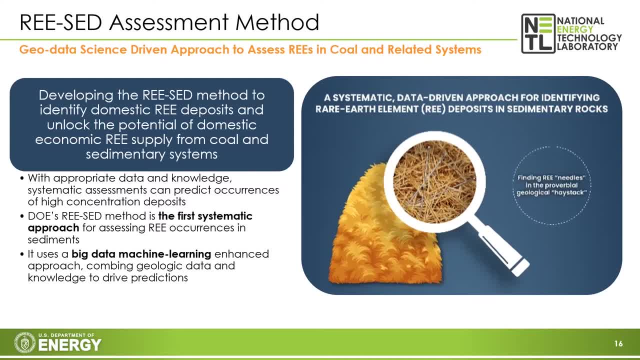 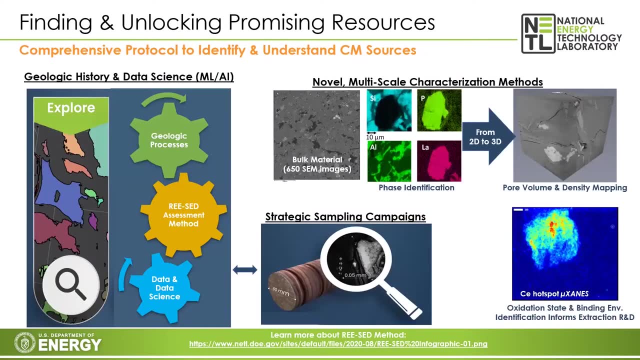 permanent magnets And we tend to talk about. you know this whole issue of the ecological energy is so instilled in many. you know we have to know about that and we have to have a good understanding of what that means. but we also have to have a good 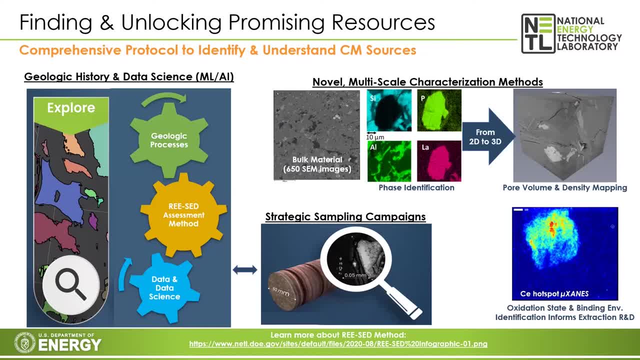 understanding of the artificial intelligence in our systems and what it means for our green sea plants, And so this is also a real challenge given the current status of the supply chain, And so we're trying to unlock the promising resources using artificial intelligence and machine learning from historical and geologic data, understanding not just the current status. 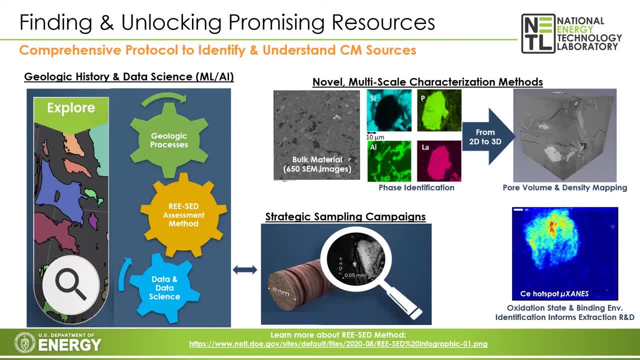 but geologic processes that would have led to the green sea plants, and so this is another real, one of the key points that we're trying to explore. Are there any particular problems that are going to come up in the future concentration of rare earth elements in the subsurface? so the geologic processes at the 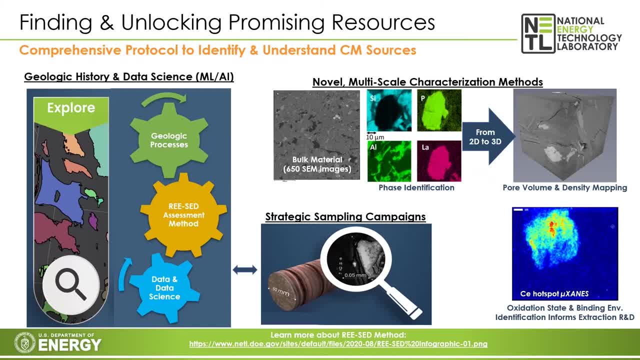 basin scale all the way through the, the mapping of the sedimentary environment, through geologic history to today's state and then confirmed by sampling. and we we've just entered a partnership with usgs where we are sharing all of our data that we have across the entire entire federal 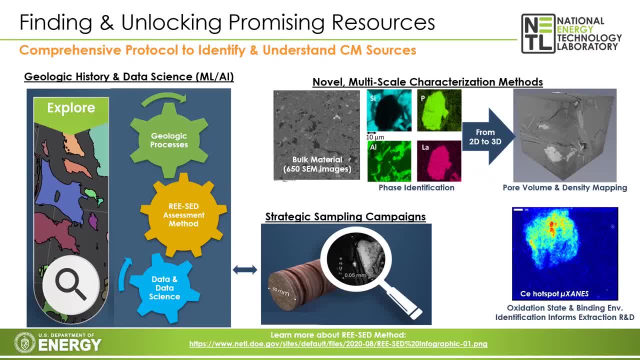 government in in the subsurface to understand how we can unlock new resources for rare earths and other critical materials. and so it scales all the way from the you know sem scale. you can see from the micron scale up to basin scale, mapping and modeling of the geologic processes in the 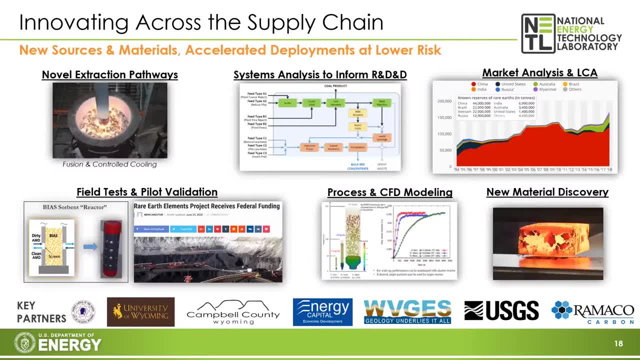 sedimentary environments. so our portfolio in the rare earths space spans across really the entire chain: extraction pathways of extracting rare earths and other critical materials, critical minerals, as well as field tests and pilot validation, scaling up and understanding the possibility of moving, moving the market in the united states and and the life cycle. 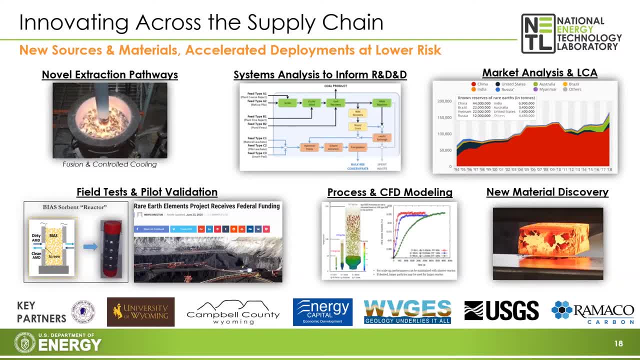 assessment again, not just, for this is not just co2 emissions. this is the full environmental impact cost of the production of our rare earths and critical, critical minerals, so that we can ultimately build into the potential for new material discovery, new alloy development and and certainly opportunities for demand growth in rare earths and critical elements. these are some of the 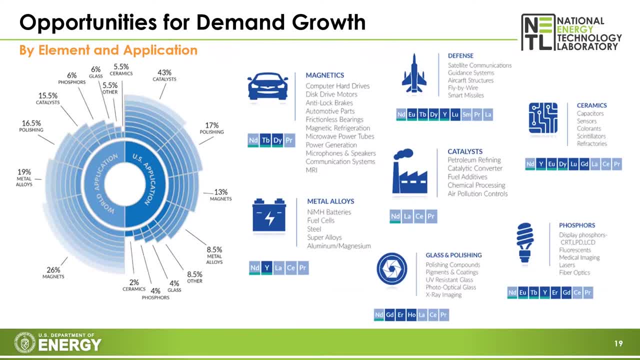 examples of where we use these rare earth elements across the entire supply chain and certainly as we drive down the decarbonization pathway over the next 29 years, as i, as i said, we are going to continue to look at some of the kinds of types of decarbonization methods that we can typically use. 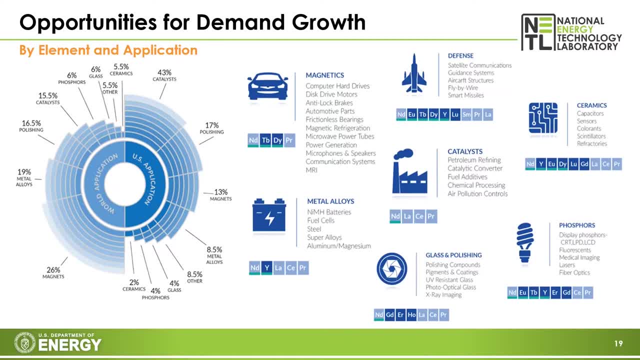 for decarbonization, to understand what we need and what we want to do with it. we do not use decarbonization, as this is always challenging, but we do need to work on it. we need to understand the types of environmental laws and the type of environmental solutions we need to use. 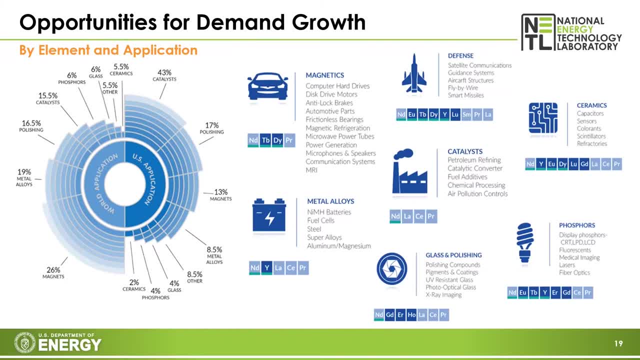 we need to know the type of rock quality. we need to know the different types of mining methods. we need to know the quality of the lakes. we need to know the type of soil. we need to know the type of exercise. if there are any dark areas, can we click on these and see if we can jump off the? 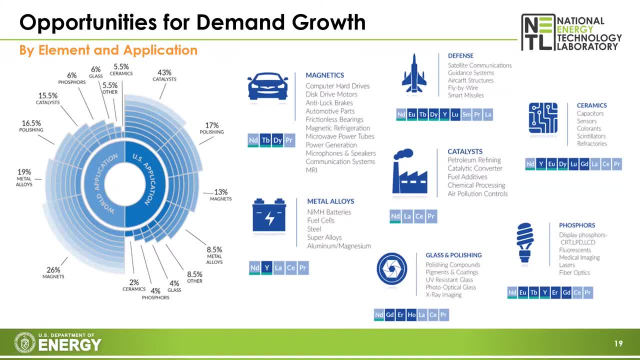 cliff and get some heavy water, we can get some of the most expensiveENELECTRICS. anything you'd like to talk about. that's a great question. again, the first thing we have to do is we have to that. I hope we have a really, really good discussion, And so I'm just going to close. 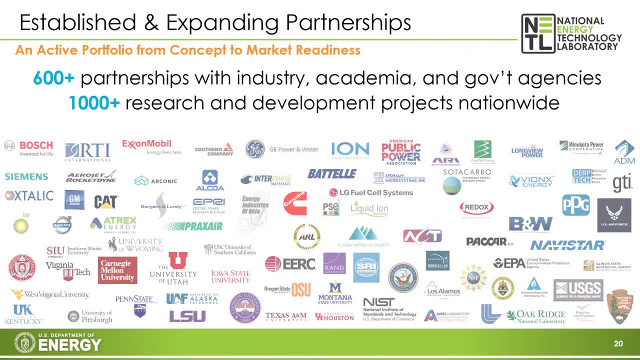 with the fact that we can. we cannot do any of the work we do at NETL or the interagency working group across 11 agencies without a robust portfolio of partnerships. We at NETL have over 600 partnerships and 1000 different R&D projects across the country. It is in every 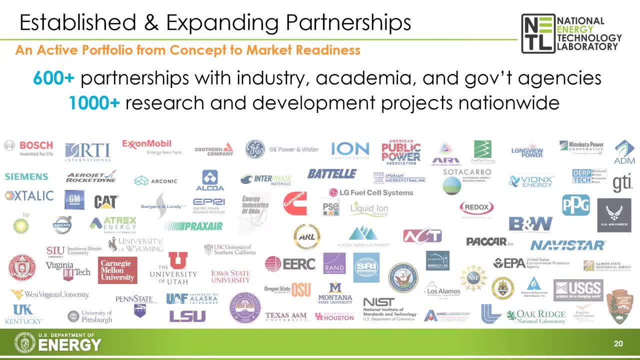 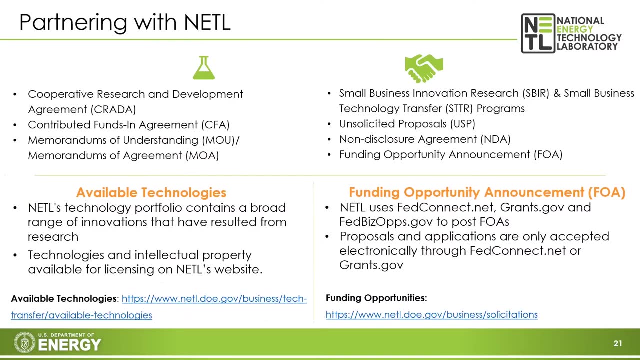 all 50 states, And certainly it is the benefit of all of these project partners that we have the opportunity in front of us to decarbonize, And so I'm glad that we have such a robust partner set And there are many different ways because, I mentioned, we're a go-go laboratory. 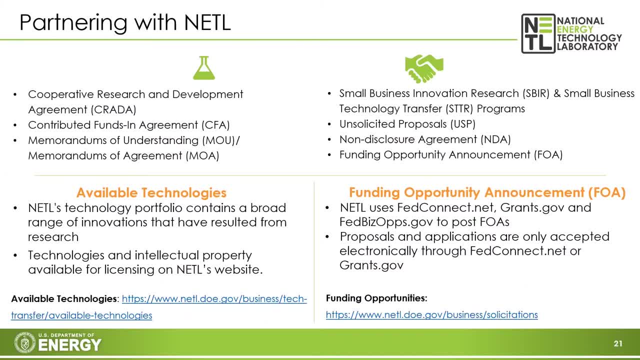 We issue funding opportunity announcements. We also partner in cooperative research and development agreements and small business innovative research agreements, And so there's a whole plethora of ways that we want to get engaged with partners across the country, And so, with that, I'm going to thank the organizers for. 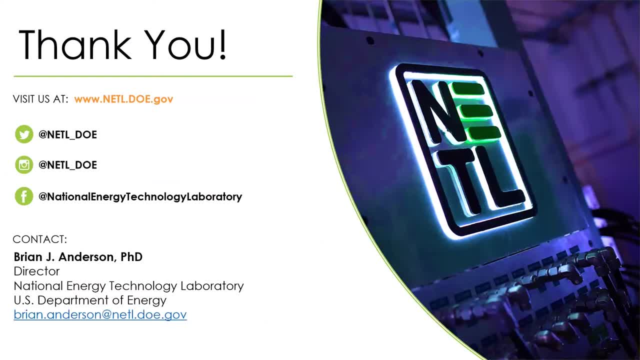 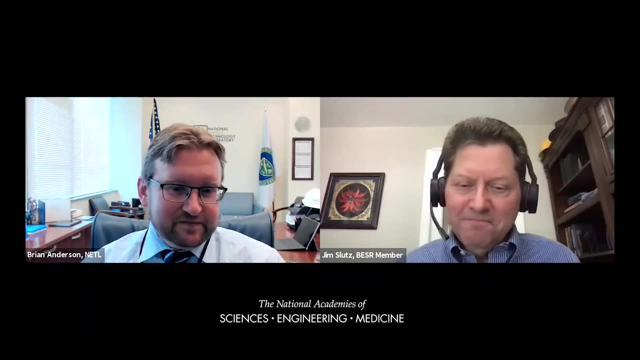 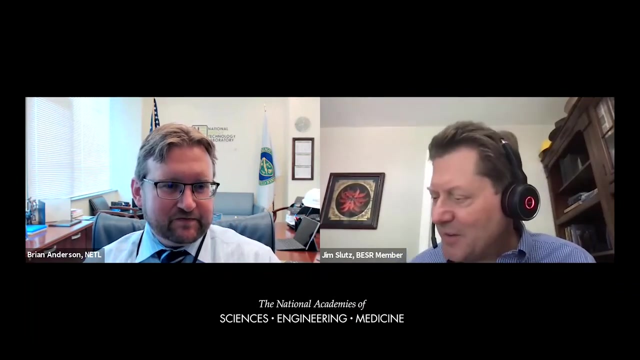 the opportunity for me to speak about what I wanted to talk about today, But I really look forward to engaging conversations so we can see where we go in the conversation and open it up to questions. Thank you very much, Hi, Brian. This is Jim Slutes, a member of Beezer, And thanks so much for that great opening. 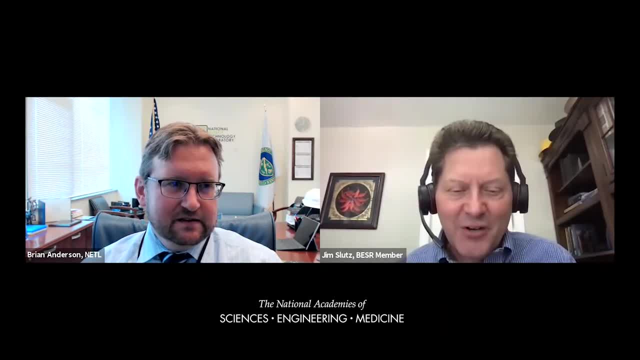 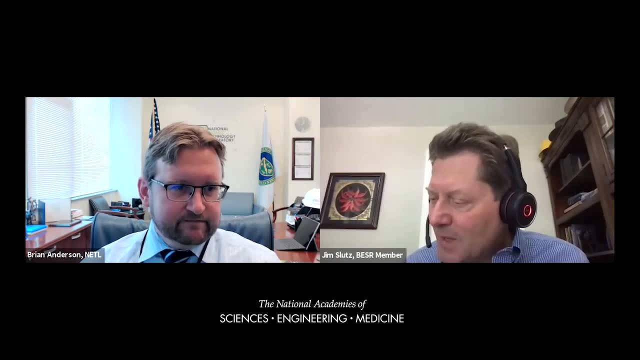 and really great stage setter for this whole discussion on research and the energy transition. So a quick reminder to folks- the members of the board that are on the that we can see. you can use the chat box, You can raise the hand and we'll call on you if you have a question to ask, And those on the webinar. 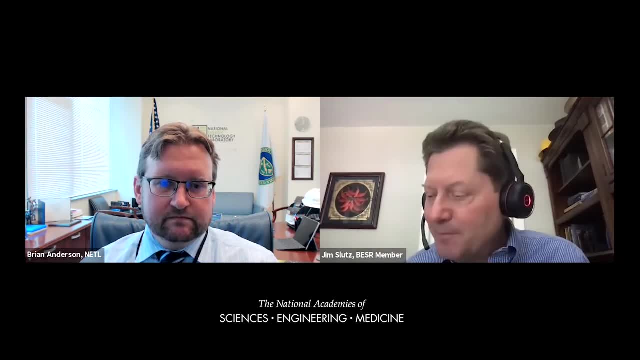 if you would just type your question into the Q&A box, we'll get to as many questions as we can. We have a nice set of time here for discussion, So this is great. Just while we're getting kind of things lined up. Brian, let me kick us off. You kind of did quite a bit of discussion there. 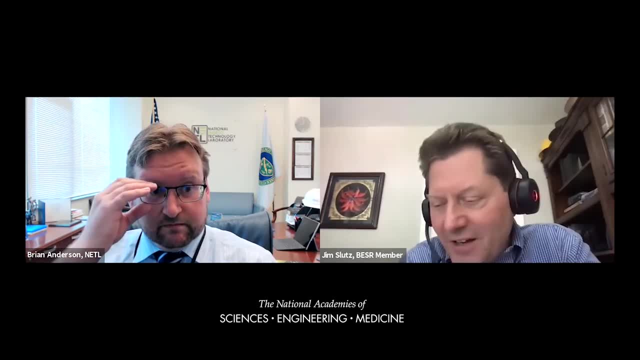 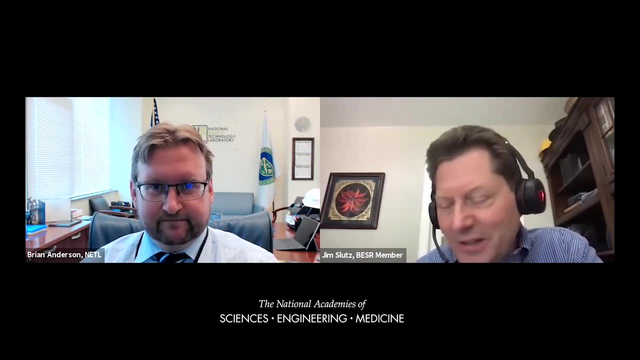 on the end on critical minerals And that's great. So thank you so much for that. Thank you, And that's kind of a and materials, that's kind of a. key current issue within this board is our Committee on Earth Resources. We're in the middle of a webinar series on critical 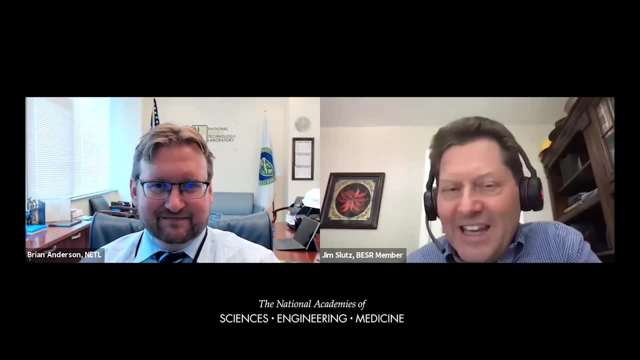 materials, And I saw recently that NETL issued a significant funding announcement for critical minerals related to coal mine waste and recovering minerals from coal related issues, And so I was wondering, because part of the thing as we look at this, and I'd be remiss without 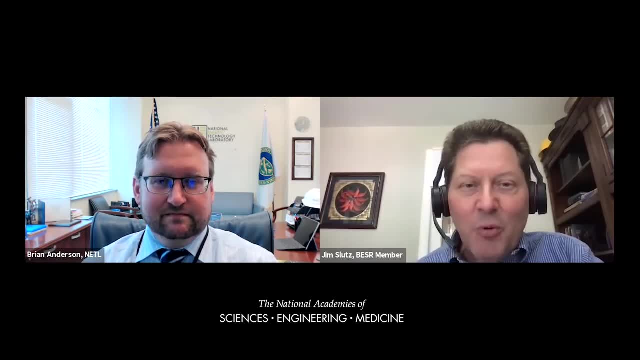 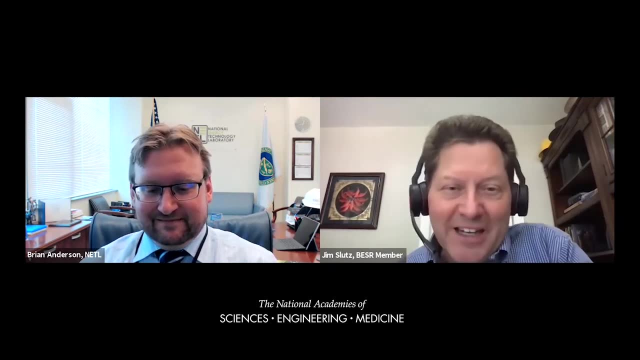 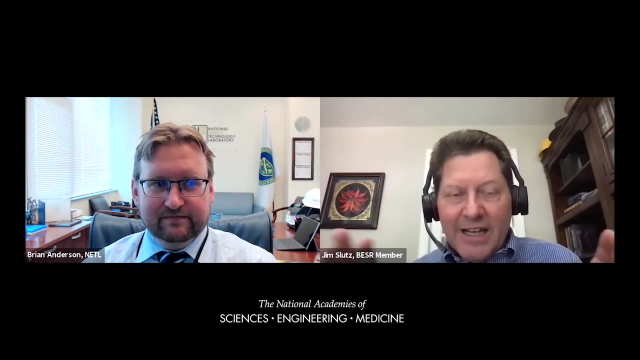 mentioning you mentioned IEA. IEA released a new report on critical minerals- which is quite eye-opening for those that haven't seen it- on the challenges of what is the demand in the future and how do we meet it. But it raises the issue because we know there's- and NETL does- a 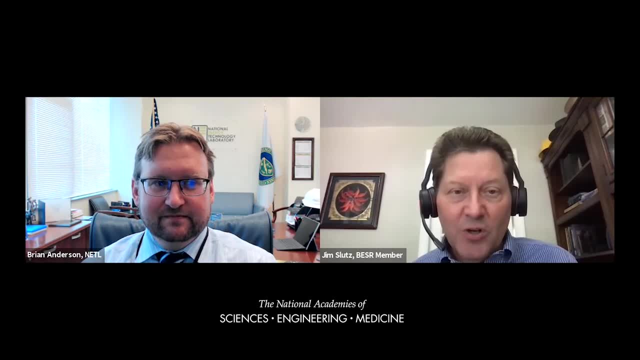 lot, but it's not always clear for those of us that work on this where in the federal government this critical minerals issue both is managed and looked at. We know USGS tracks, kind of current, you know a lot of information, But from a research perspective, because it's going to be, 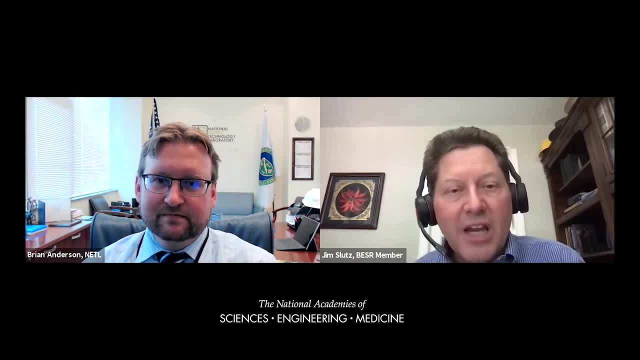 more and more important. is this going to be a? is this an evolving area where DOE is expanding broader, beyond just some of the traditional areas? Do you is there more of a government-wide initiative on this? Is there stuff you can share on how we might look at this from a US government? 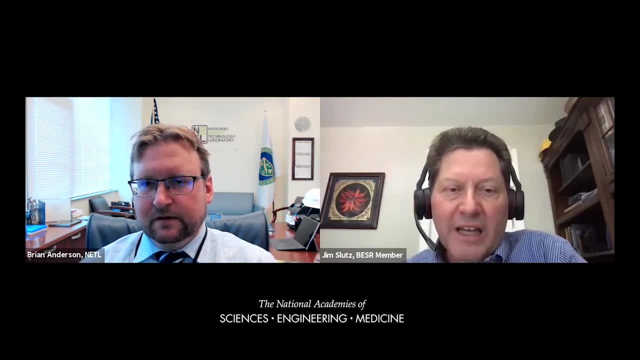 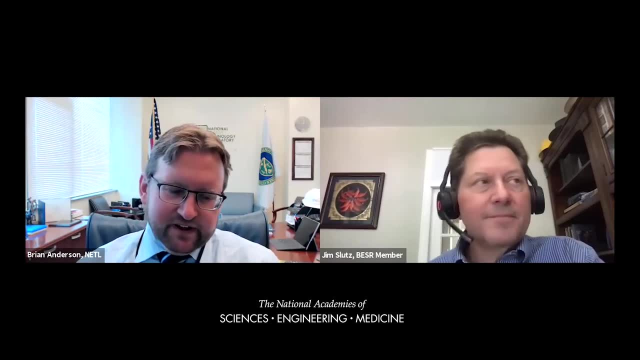 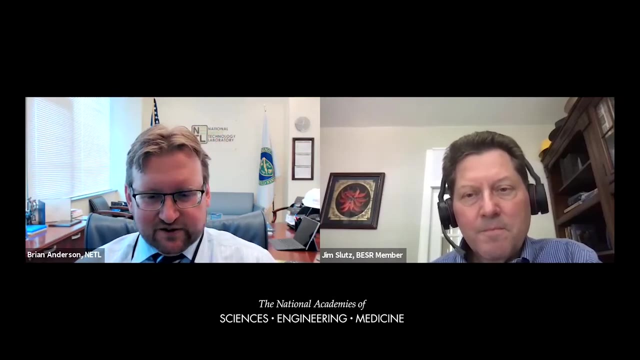 management perspective, And how do we look at managing the critical minerals and particularly research? Jim, that's great And so in. so the Department of Energy interests are twofold. I mean one within the fossil energy space as well as geothermal. so this is the earth resources space. 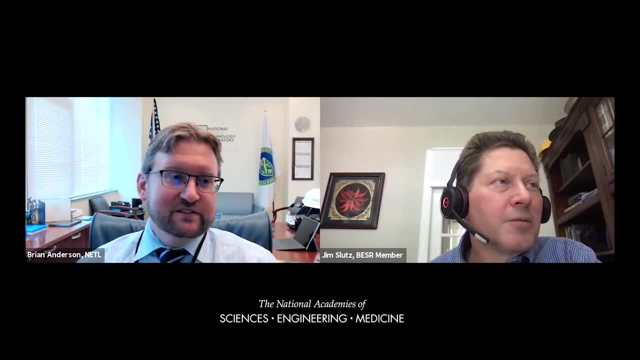 within the department we have identified that there is an opportunity for a resource base of rare earths and critical materials, And so the geothermal technologies office has had a had some efforts in the past that they've funded for extraction of critical minerals from geothermal brines and things like that. 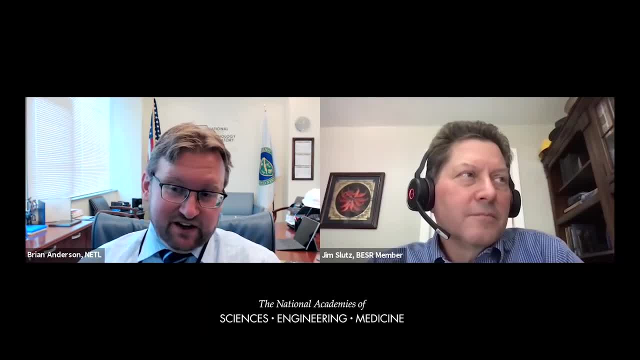 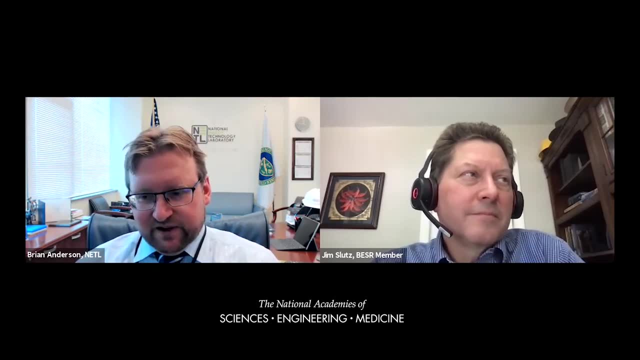 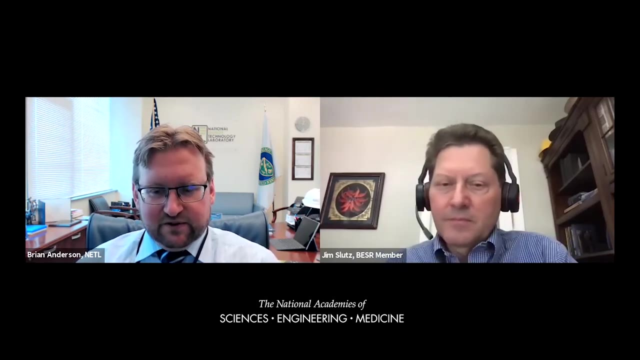 We identified within the fossil energy space that these sedimentary environments of coal have some increased levels, particularly the heavy rare earths, And so our focus has been of being able to leverage the resources side. But then, when I say that the critical minerals effort of the department- 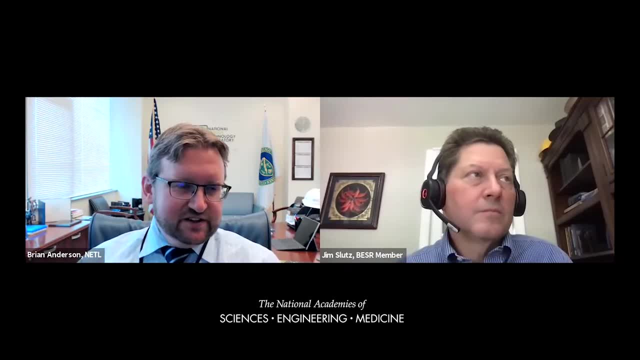 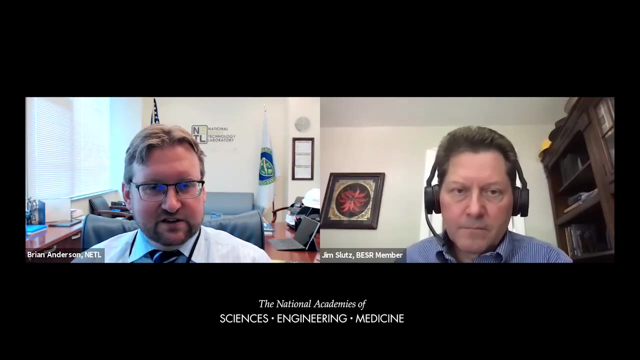 is twofold. It's because, within the energy efficiency and renewable energy space, knowing that the demand for critical minerals in in the renewables development is so high, there's also a real focus on how we can increase critical minerals and rare earth elements into that supply chain for for renewables deployment. 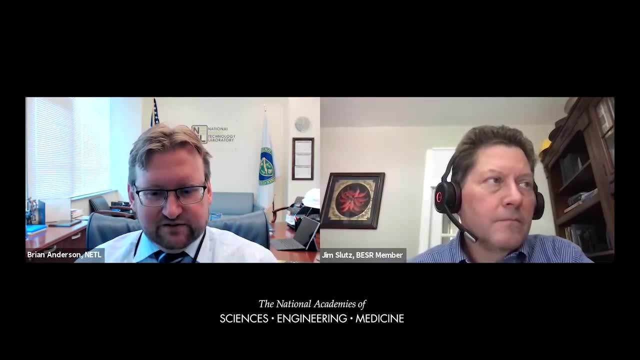 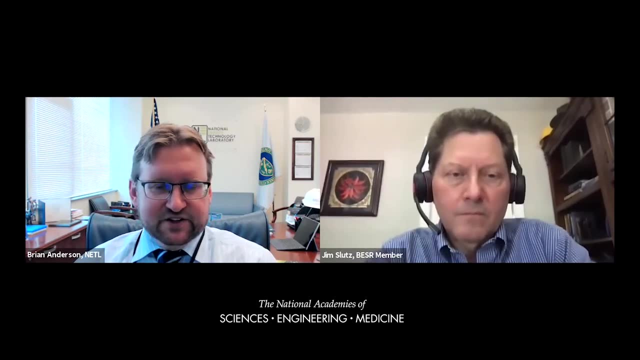 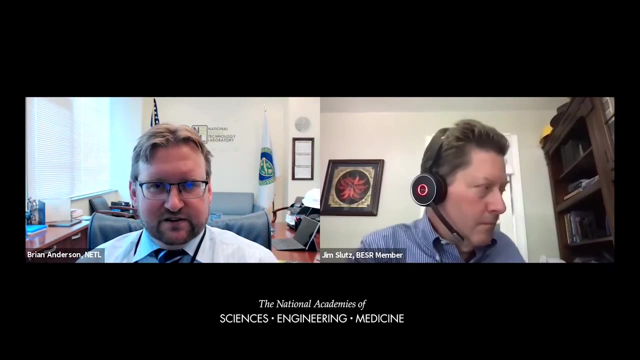 And so that's really the the breadth of rare earths and critical minerals As a focus within the Department of Energy. we did just stand up the Division of Minerals Sustainability within the Office of Fossil Energy. There's also a lot of work over in the EERE. 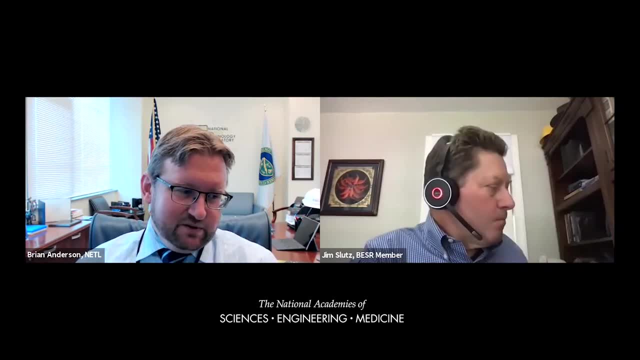 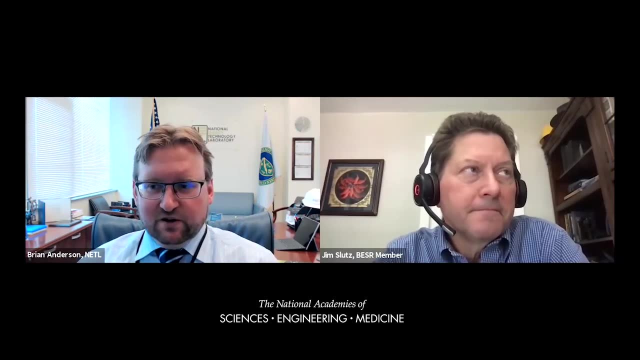 Now the whole government approach. we have worked with some of our partners, certainly in in Interior and USGS, as, as I had mentioned, understanding the resource base as a whole, and in in Department of Defense. frankly, because of their efforts, 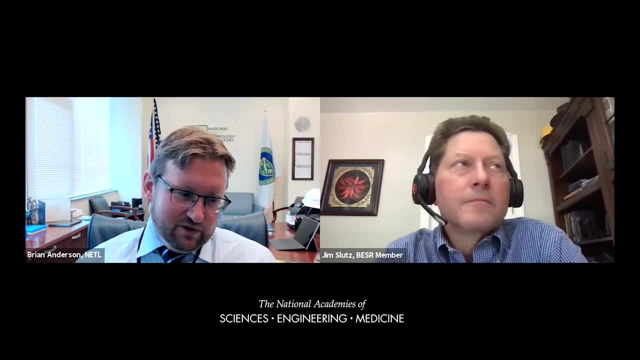 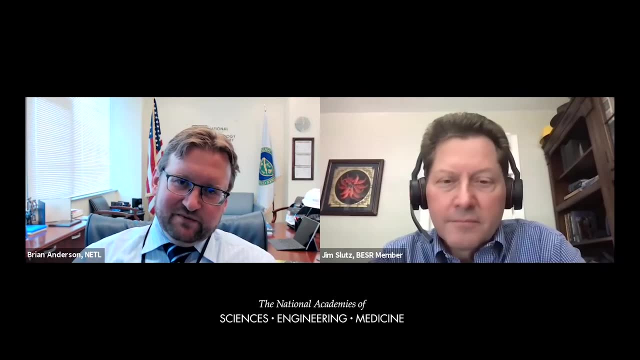 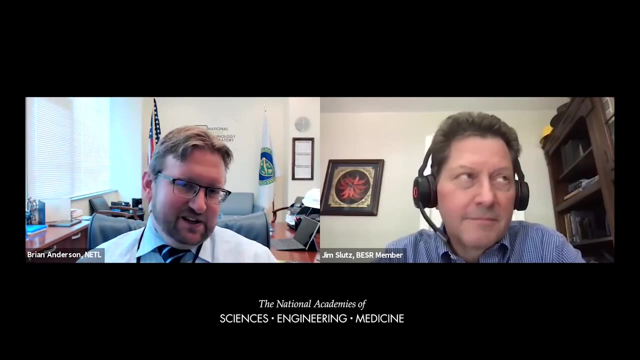 They are a little different from our supply chains, But the technologies that we are working on are: There's a merge point within a supply chain of moving it from a resource- say an acid, mine, drainage sludge- You make a rare earth oxide and then, once you have a rare earth oxide, the supply chain really converges. 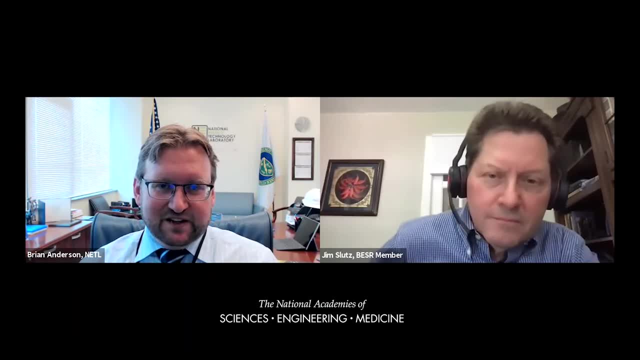 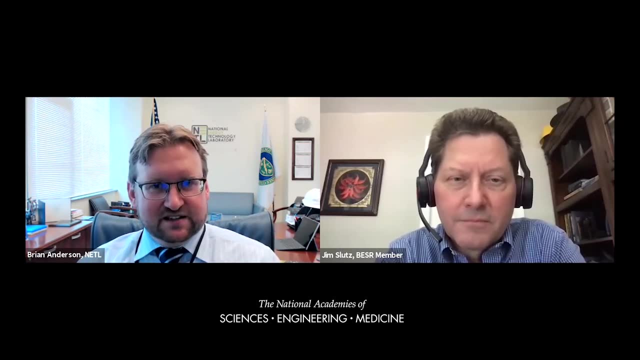 with almost any any source of rare earths that you would. you would have, be it Mountain Pass, a historical rare earth mine, And our focus then is on the environment, is on the environmental sustainability of the process of purifying and alloying into the final. 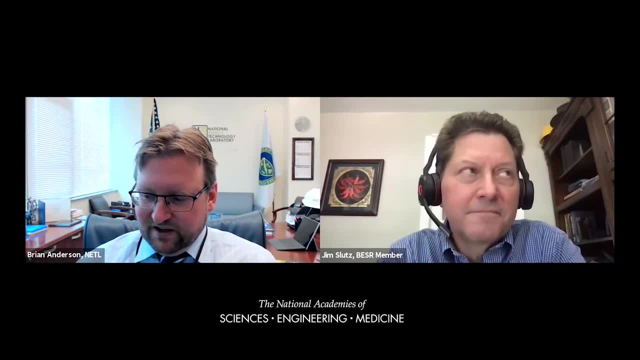 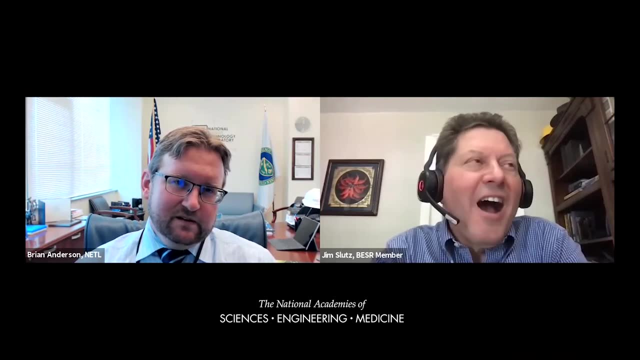 metal. So I think we're doing quite a bit of work across the whole supply chain in that respect, but it's not covering the whole federal government. Okay, thanks, Brian. Hey, one of the questions that came in. we have a couple board members to go to and I'll go to them in just a second. but 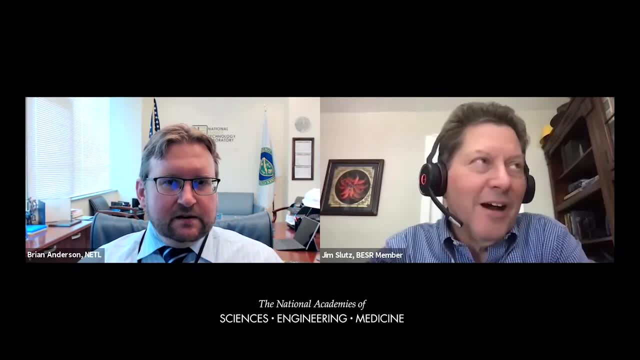 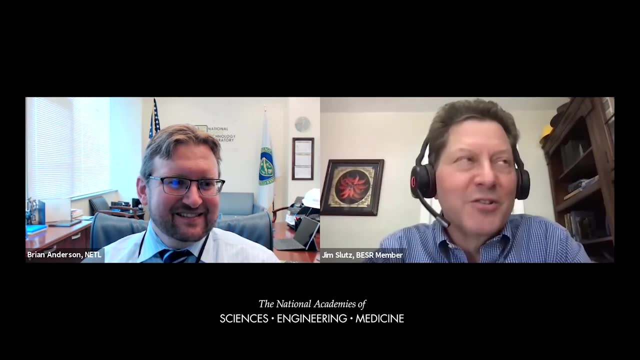 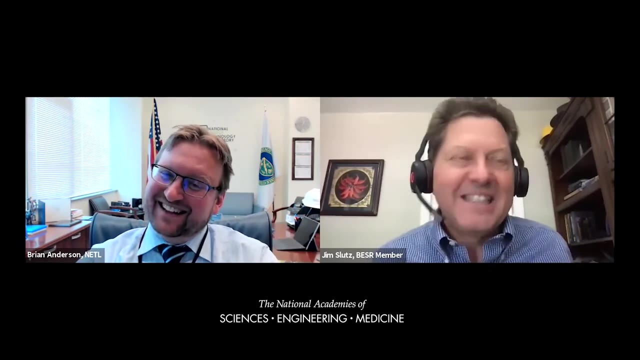 I see one of the questions is a personal favorite that particularly resonates with me that someone's asked because, Brian, you and I, and probably very few others, have been to Albany Oregon, and realized what a jewel that facility is, And so can you share a bit more about the? 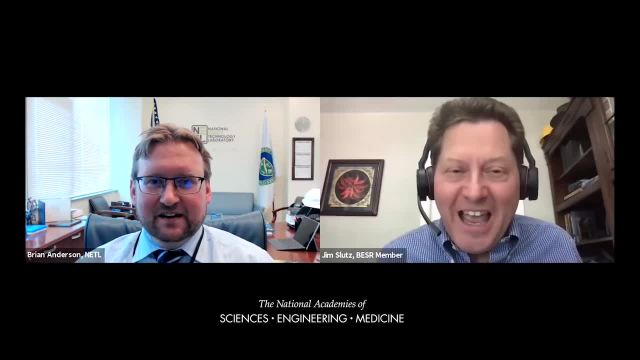 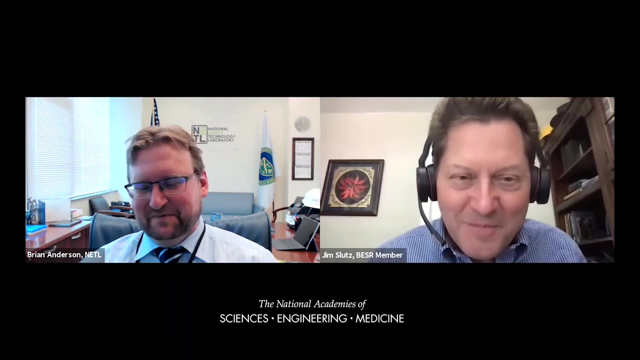 focus and efforts taking place at the Albany Oregon lab, And I think this is a great opportunity for you to share. I want to champion a little bit of that because it was one of my favorite field visits when I was at DOE years ago. Yeah, thanks for teeing that one up. So in Albany, historically, I'm not going to. 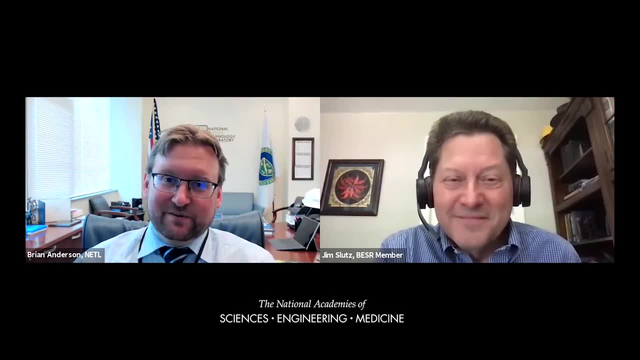 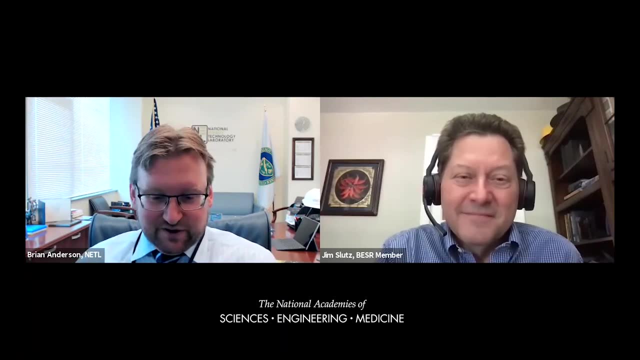 go through the whole history, but during the Second World War the Albany Research Laboratory was founded to work on new metals, metals and metal alloys. Over the course of the last 75 years the Albany Research Facility has spun out a whole specialty metals alloy industry in that part of West Central Oregon, And so our focus is. 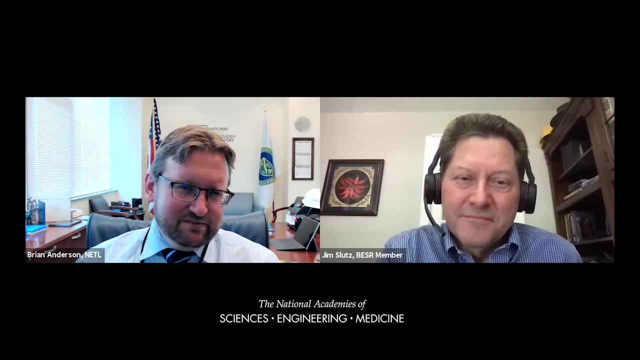 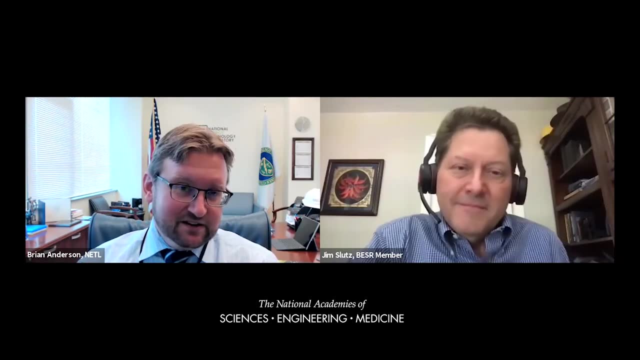 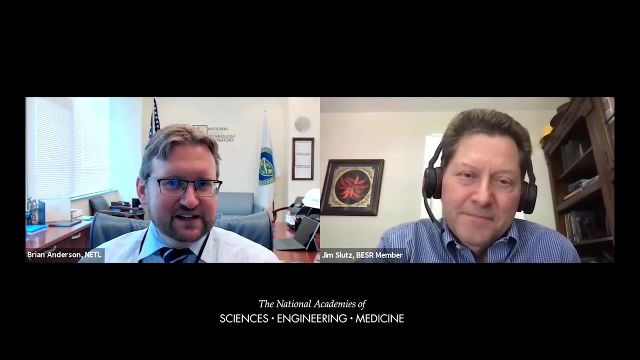 still on advanced alloys, advanced alloy processing. We have really unique facilities to be able to scale up and develop new materials and new metals, in particular in the alloying. But more recently we've expanded a lot of the research we do in Albany to include that: geospatial data analytics. 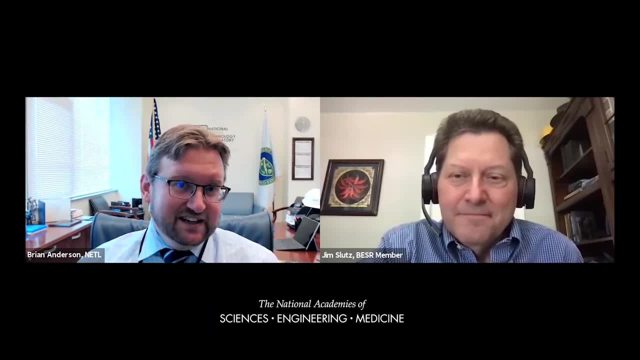 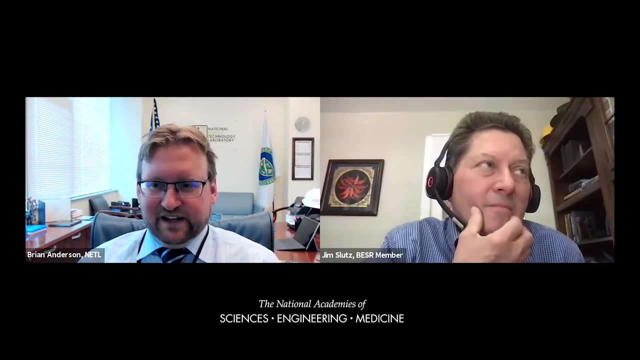 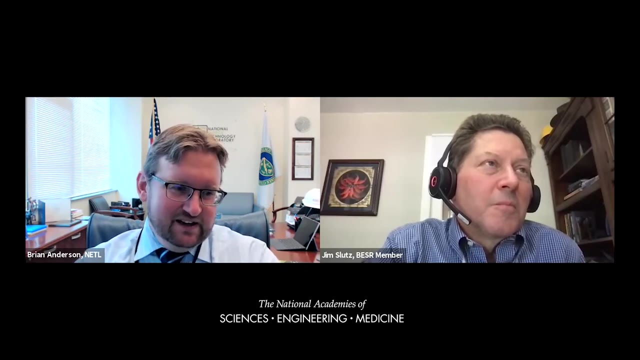 So we have this great team, huge team called Gaia, which is a geologic, a geospatial data analytics team. They're focused in Albany and just tremendous assets there. So while Albany is the smallest of our three laboratory facilities, it does have still. continues to have great impact, And one of the great inventions out of the Albany Laboratory- in addition to lots of metals over the course of the years but was actually- is a biocompatible metal heart stent that is in use All across the world- patents in Japan and the United States and is credited with saving many. 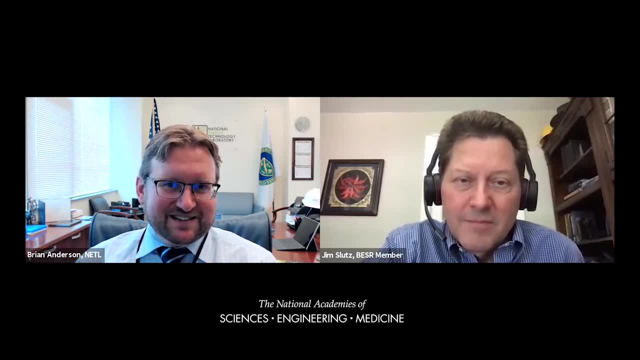 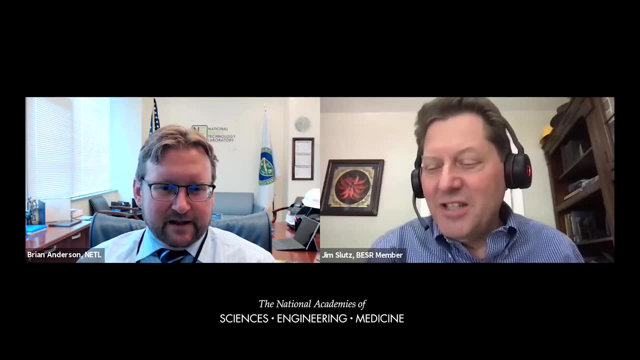 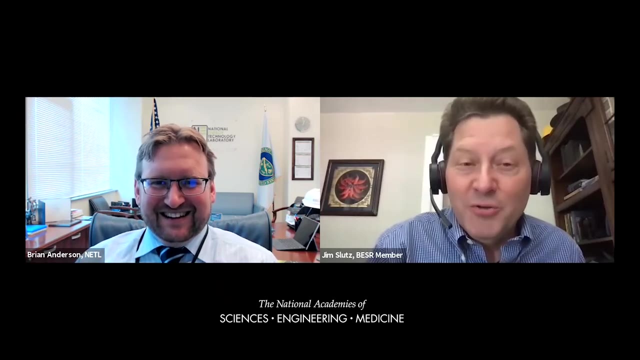 many hundreds, if not millions of lives as a biocompatible metal heart stent. Thanks, Brian. Yeah, And just if I could just add one thing, because it's the other lives they've saved- is the current state of the art body armor used by the US military, which is a huge national. 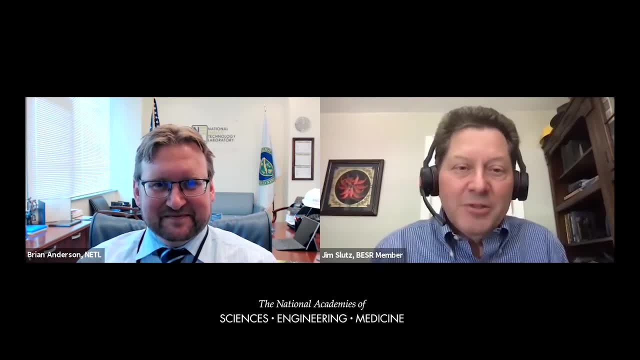 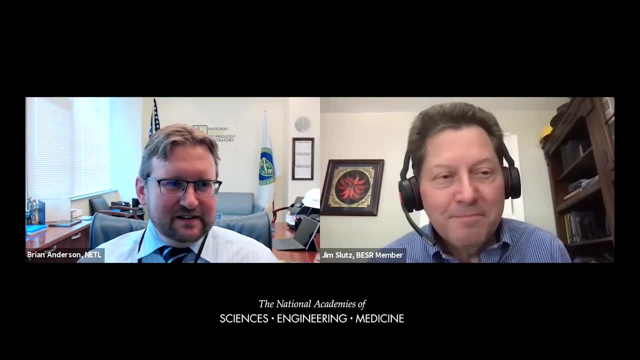 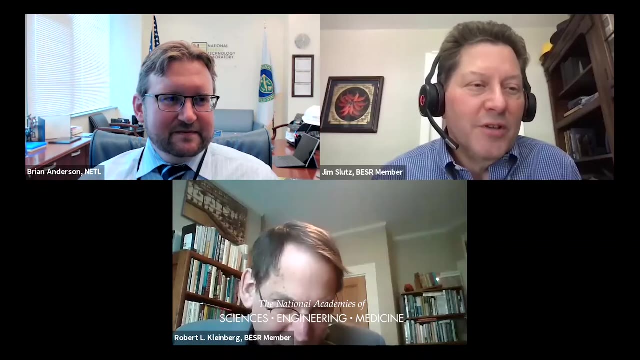 defense and and accomplishment. So let's go to a couple board members. First we have Rob Bob Kleinberg. Bob Bob, you need to unmute there. Okay, there we go. Hello Brian, Very nice to see you again. 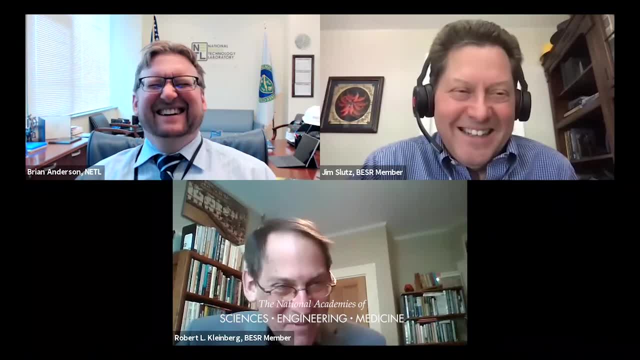 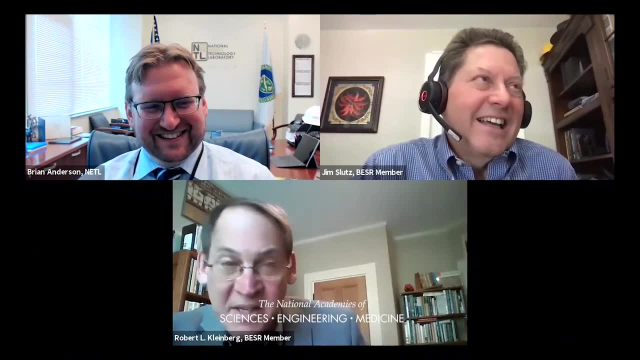 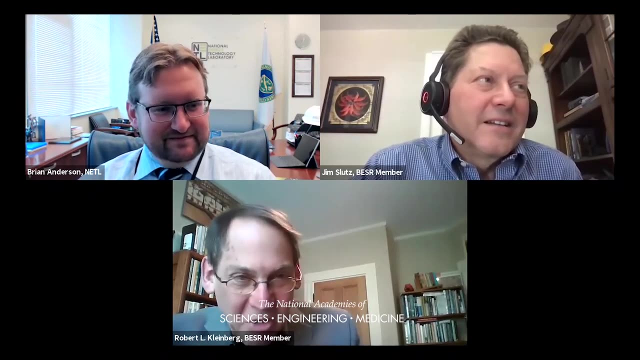 And now I understand what 16 petabytes is. I never really quite was able to visualize that. But the question I want to ask is about seasonal energy storage. Right now the United States uses something like 5% of its natural gas production to sort of level the load between summer and winter. 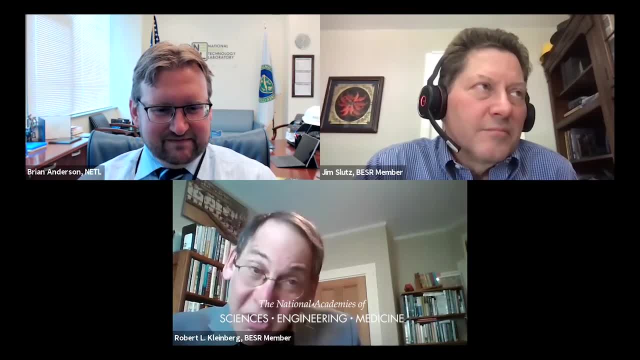 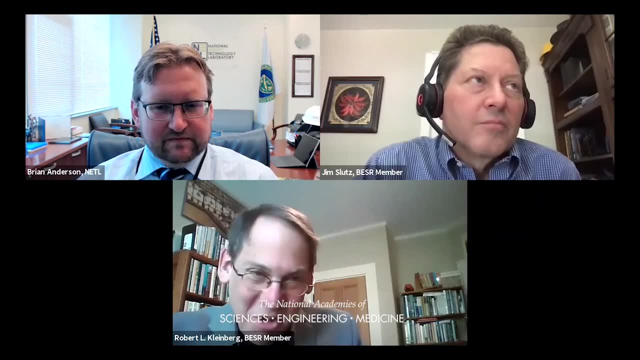 consumption of energy. It seems to me that that's only going to grow as renewables become more important. We don't get much solar energy here in Boston during the winter, So do you have an outlook as to how we're going to decarbonize and maybe expand our seasonal energy storage? 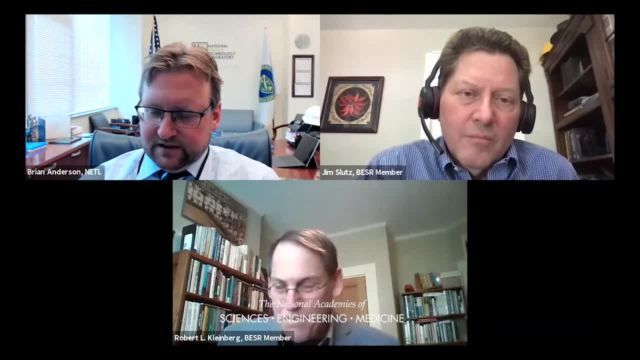 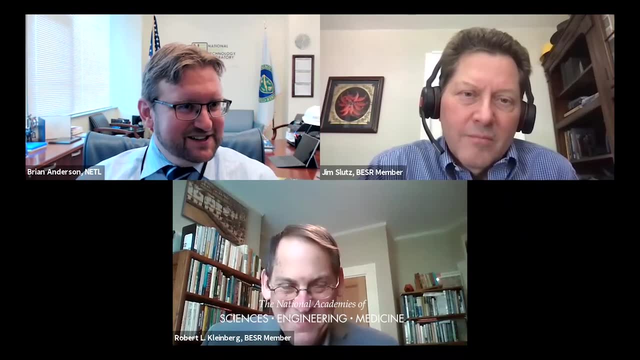 I think that's a really good point, Bob, And not only Well. so the quick answer is no, I don't have a great handle on it at the moment. We're still working on it. That's the short answer. 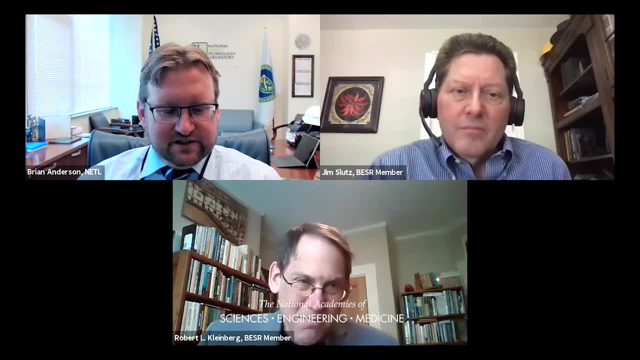 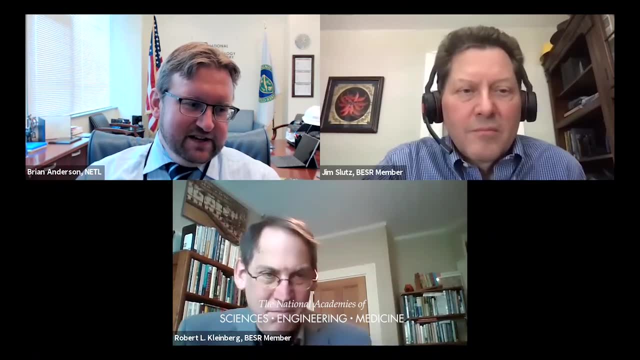 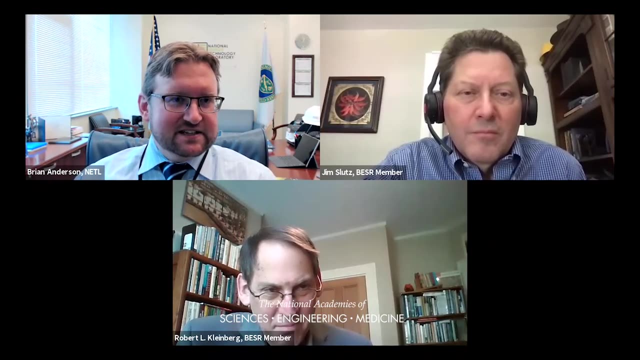 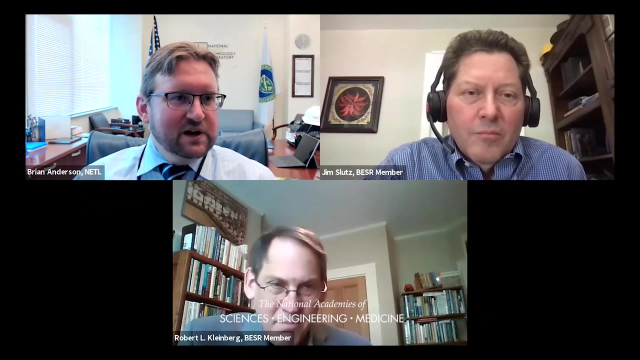 But one additional complexity is not just with seasonal energy storage that would be enhanced and an increase in local environmentalimanagement by deeper solar penetration on a seasonal basis, But then on a daily basis. as that big trend line grows, then the daily variation will grow as well. 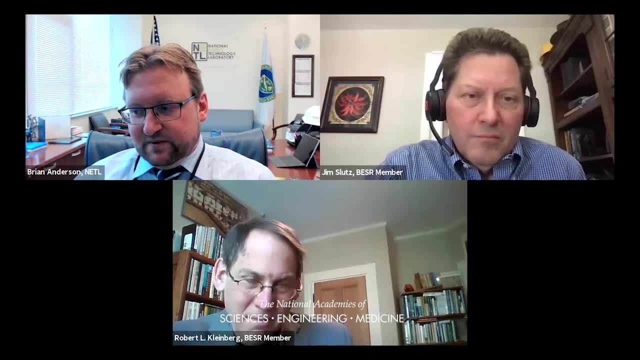 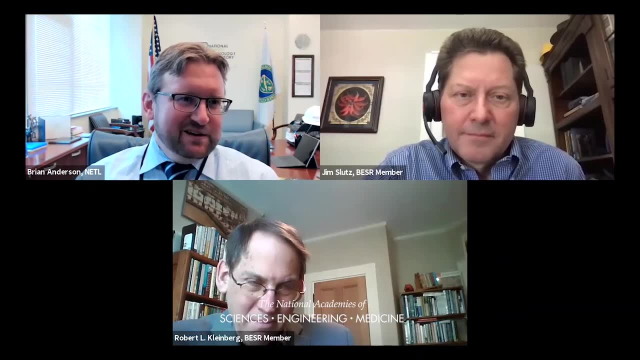 and so even higher variations, And so that is one thing that we still have to manage, And so right now, I mean not to paint a bleak picture, but the natural gas infrastructure, particularly in the Northeast, is operating on a pretty fine edge. 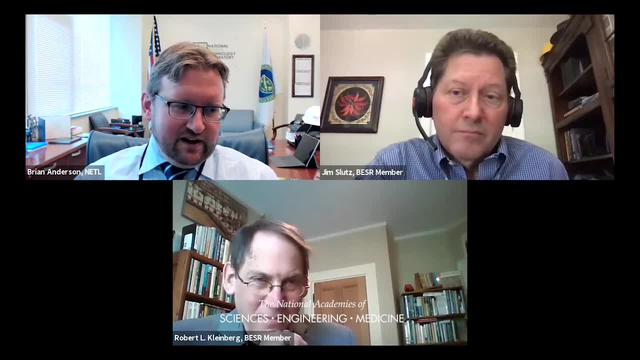 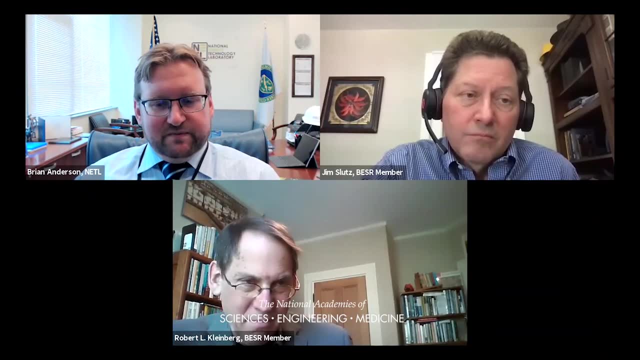 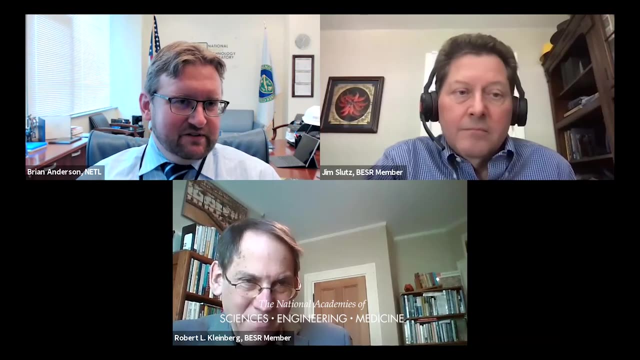 when it comes to delivering natural gas on demand in the wintertime, when power plant needs increase, but yet homes are heated with natural gas, And so it's all part of a very complex problem which any imbalance creates. you know possible problems. 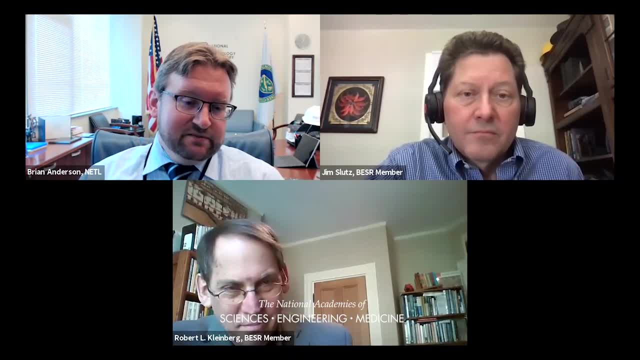 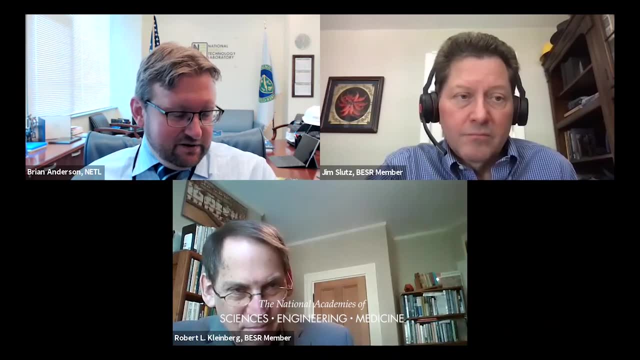 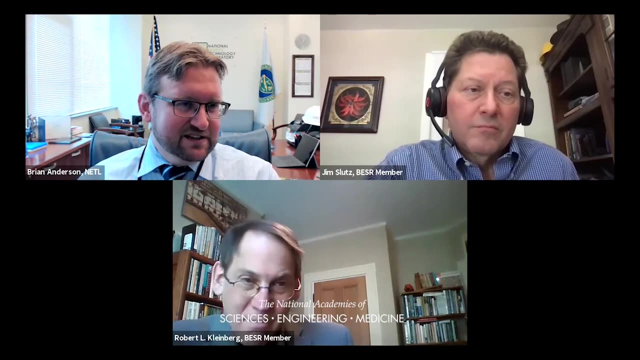 That we saw just a couple of years ago in Michigan, in MISO, when one natural gas compressor plant went down, or compressor station went down. that ended up resulting in about 12 automotive facilities shutting down because it knocked out power, And so we operate the energy system at very tight margins. 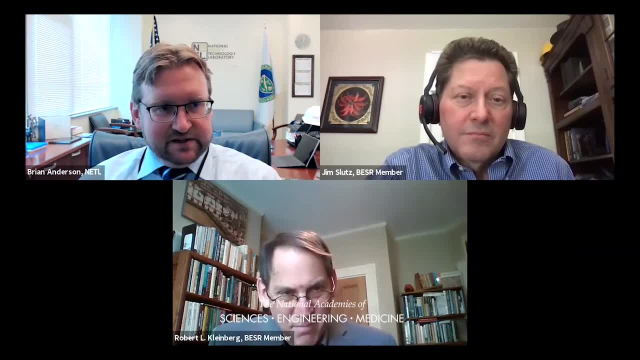 and as we drive aggressively to decarbonization, it's going to throw off a lot of the balances that we have to just manage. We have to be out in front and have to manage them very actively in order to maintain the resiliency that we require. 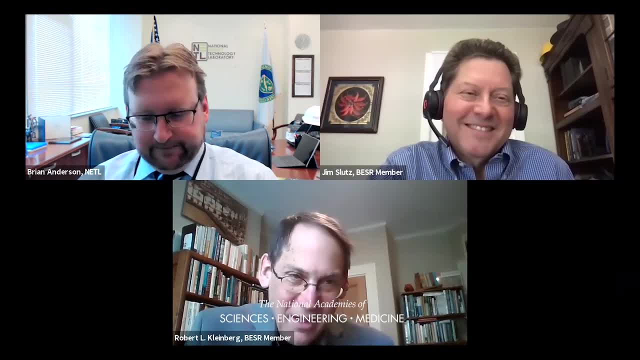 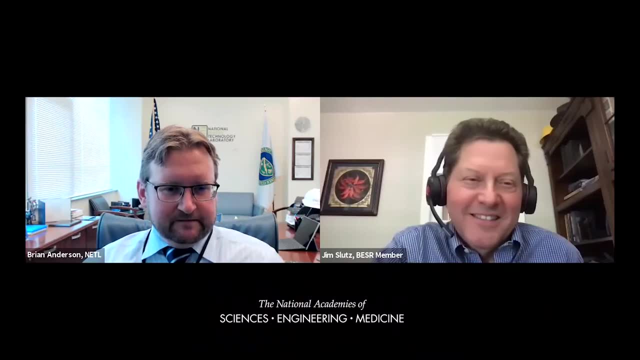 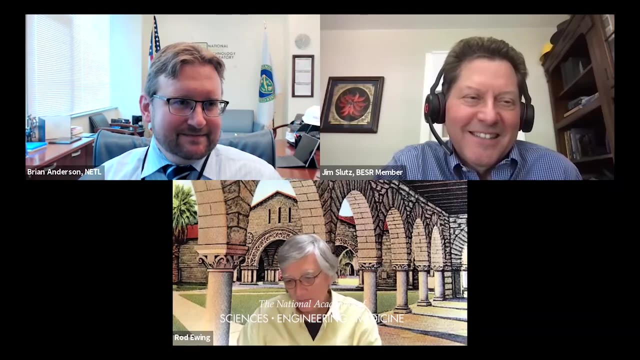 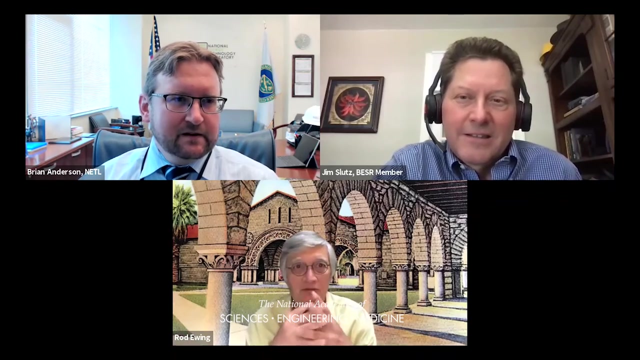 Right. Well, I certainly urge you to keep that in the forefront of your mind. Thanks, Bob. Rod Ewing, Rod Ewing Right Brian, thank you very much for the interest, the interesting talk and the comprehensiveness of the presentation. 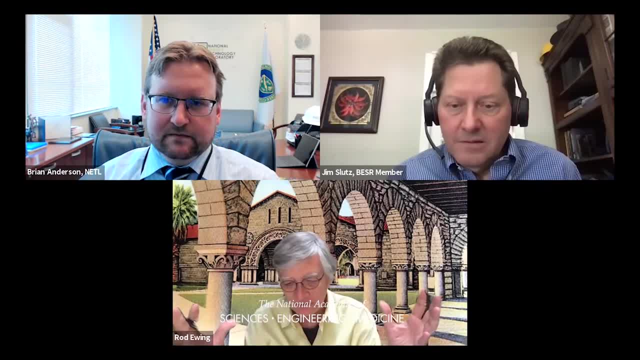 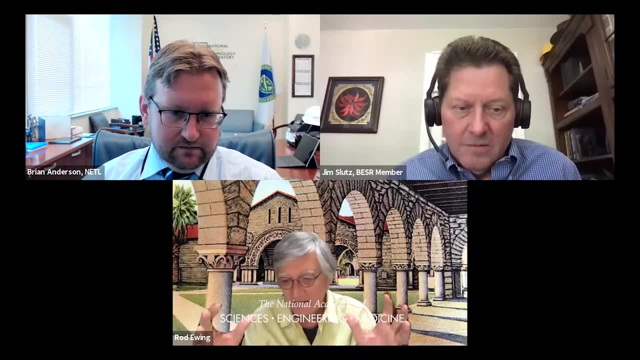 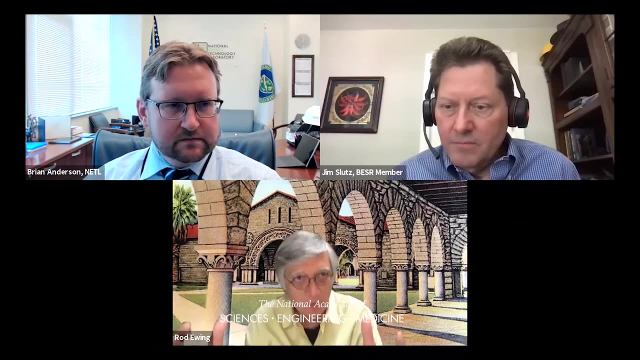 That said, and even though what you've presented is a pretty sweeping portfolio of research topics and charges, how does NETL interact with other sources of renewable energy, their support within DOE and, in particular, I'm interested in the absence of any mention of nuclear energy? 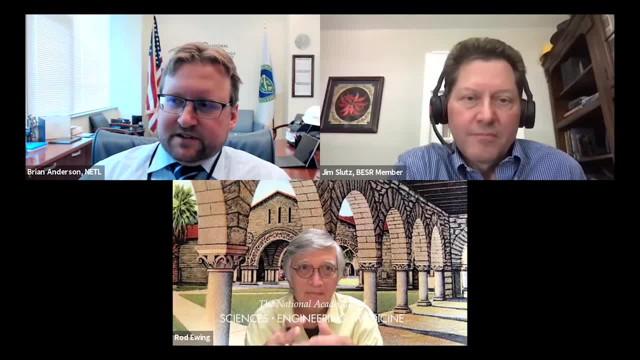 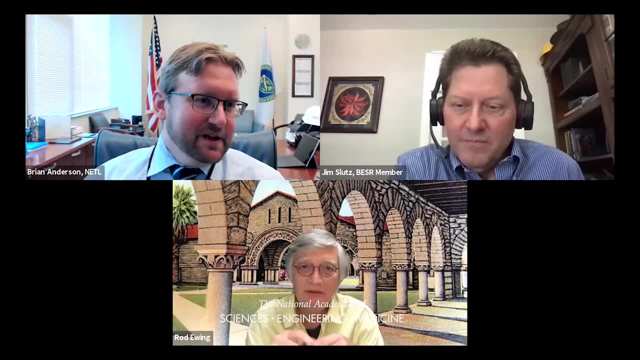 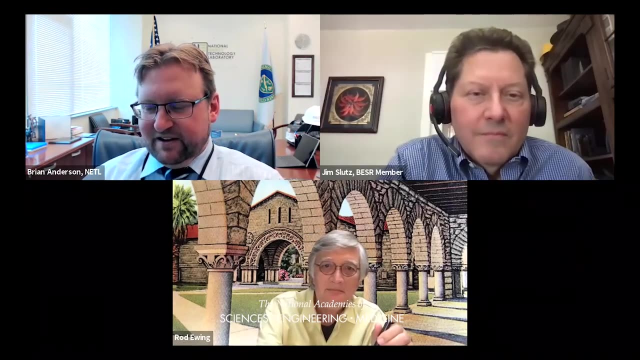 Well, the absence of mentioning a nuclear is just simply that we don't manage any of that portfolio. It's all out of the Idaho lab, But the nuclear is, you know. I just I may have absolutely not mentioned it, but it has to be a critical part of the portfolio. 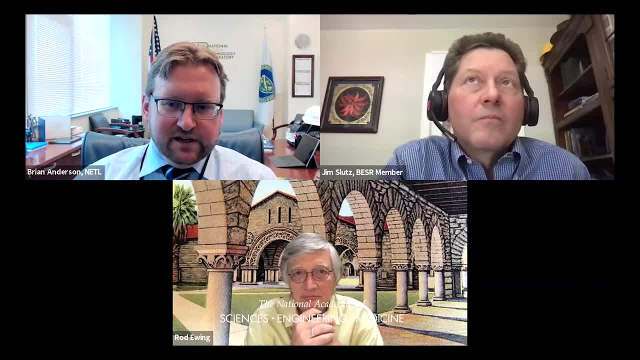 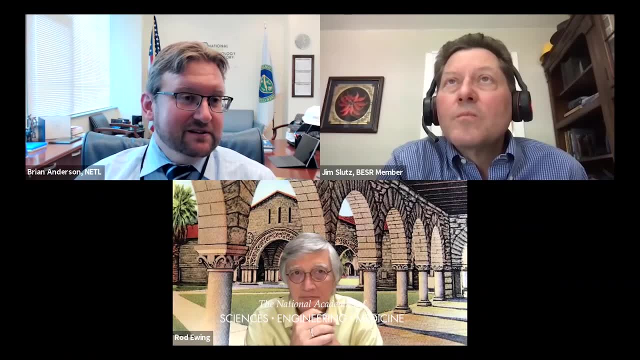 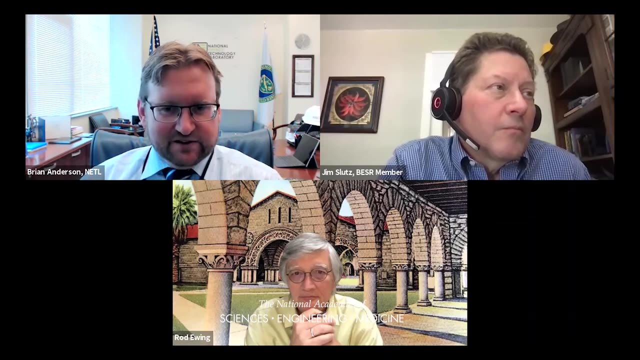 Under, you know, zero carbon scenarios. it is. you know it's a very important part of the portfolio. It is the one no zero carbon-emitting firm power that's on the market today, And so it certainly advances in small modular reactors to allow some flexibility. 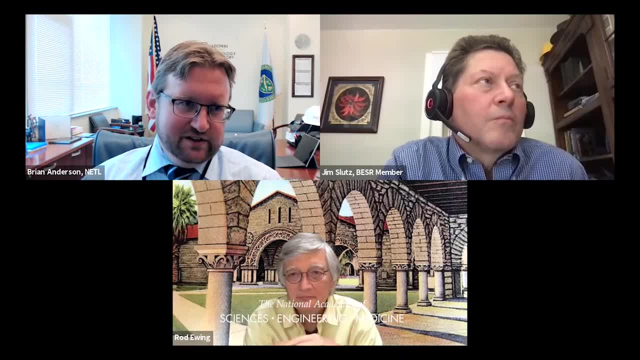 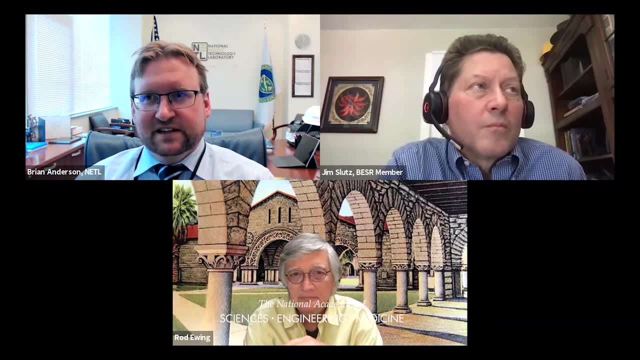 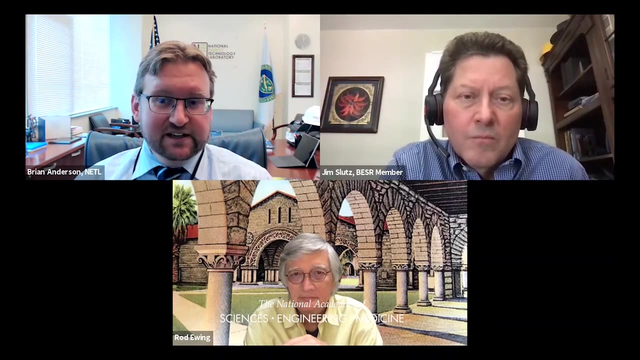 and the possibility for load. following is a huge direction of the Office of Nuclear Energy to contribute to the portfolio and then driving down costs and inherently lead time for permitting and building new technologies Right. And then the social acceptance to come along with that as well is critically important for us to. 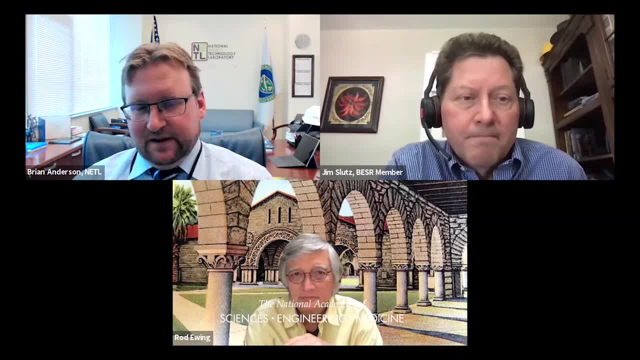 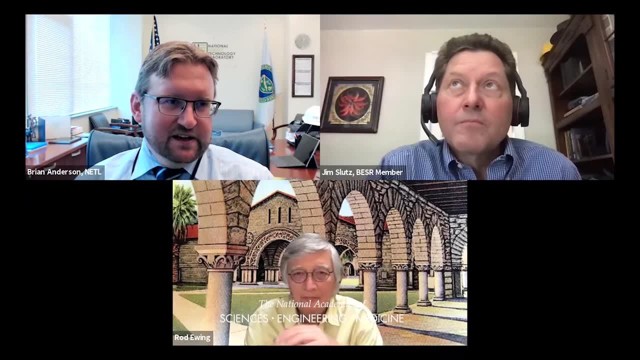 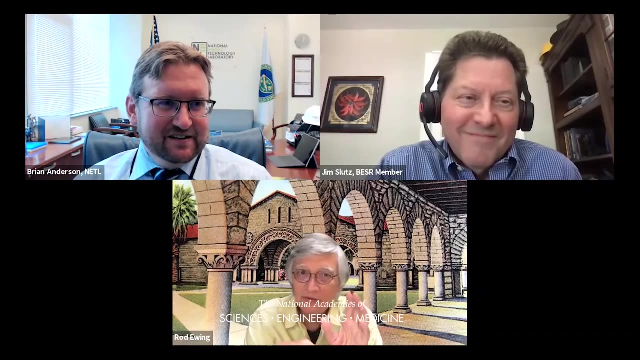 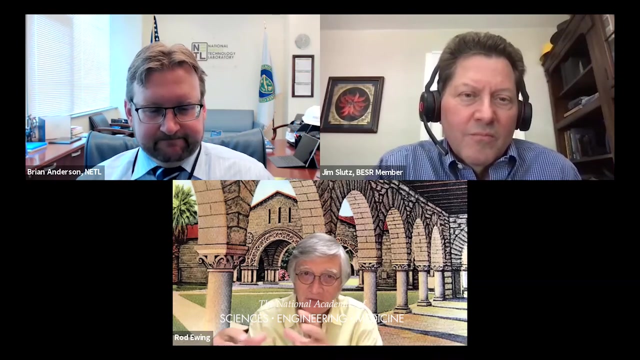 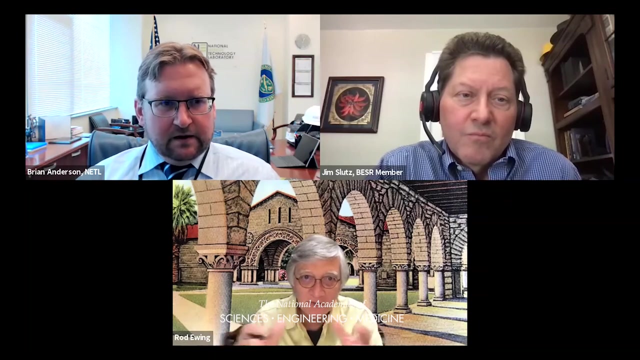 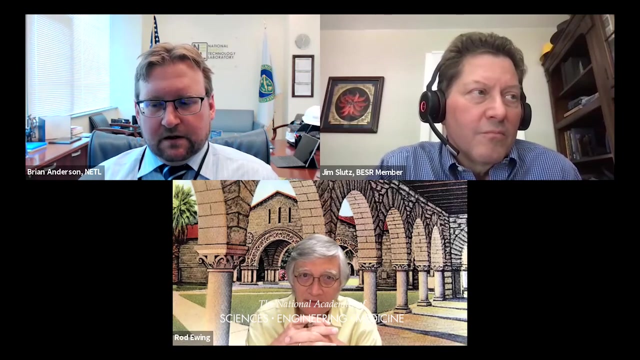 as a part of the portfolio to decarbonization. That's kind of an opinion. The facts are there's a huge portfolio in the nuclear space in the Office of Nuclear Energy. My apologies, I didn't touch on today, Just just a quick follow up. One of the centerpieces of what you're doing is the life cycle analysis And of course, within nuclear energy and DOE that's a big question. Is there a process by which the life cycle analysis for nuclear and other energy resources is compared and developing policy? 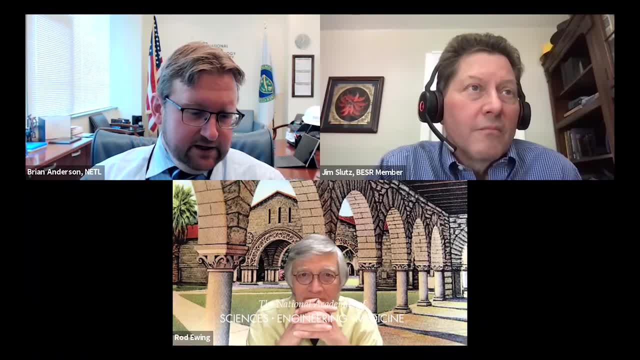 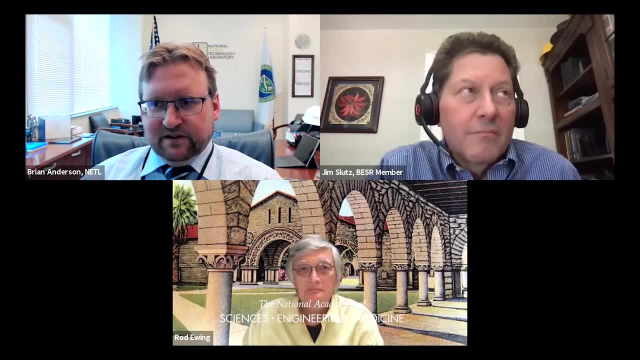 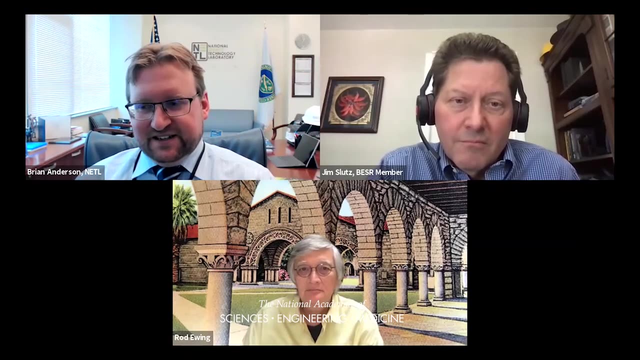 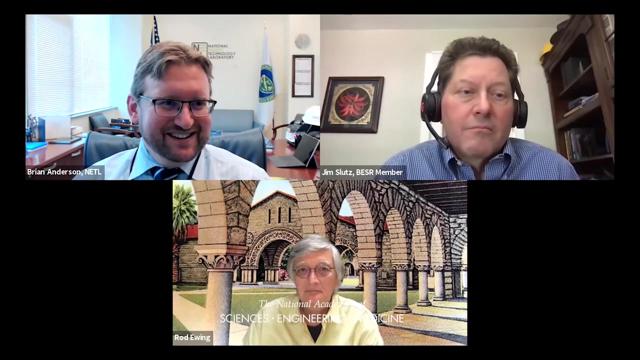 So, in short, yes, And so a major part of the portfolio in the Office of Nuclear Energy is the stewardship of the life cycle of the nuclear material, the fissionable material, and particularly waste. And it does get into very sensitive topics around political topics, around the storage of waste in places like Yucca Mountain and the like. 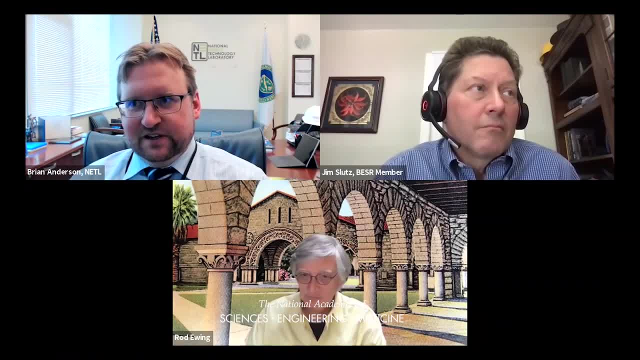 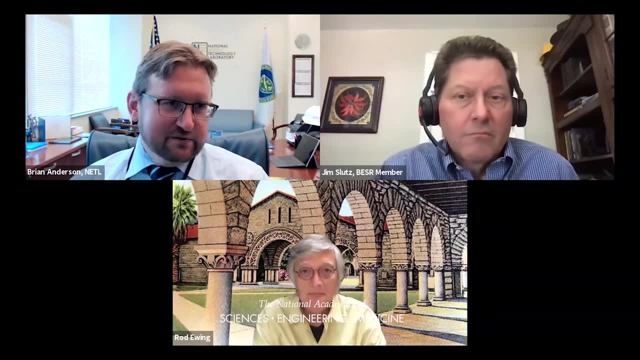 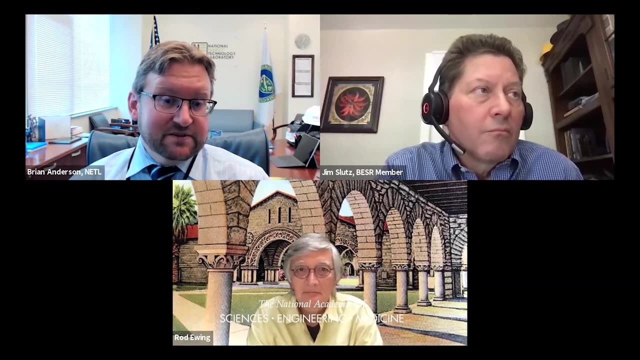 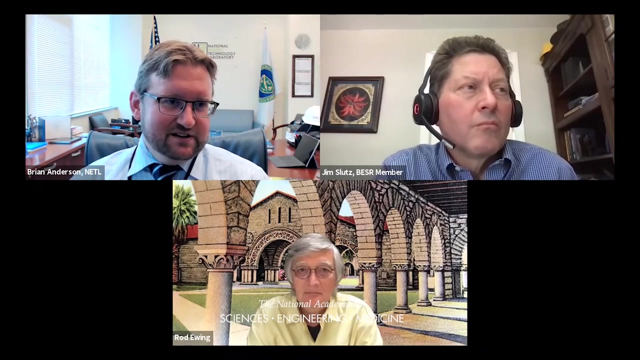 And so it is a critical part of the assessment And the department department as a whole under the undersecretary for science and energy, where fossil and renewables and nuclear all sit. And so it is a it is a critical part. Now it becomes different, difficult, because there are some apples to oranges when it comes to, you know, managing nuclear waste over its entire life cycle, to managing carbon over its entire life cycle. 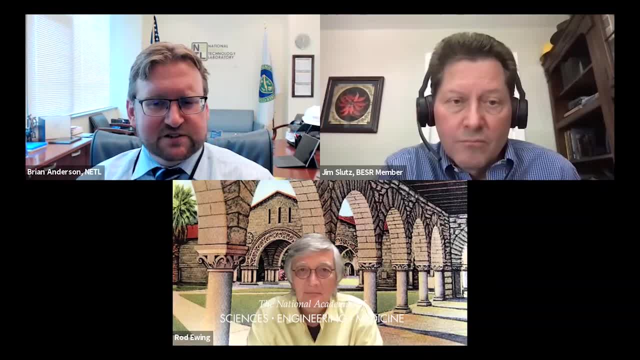 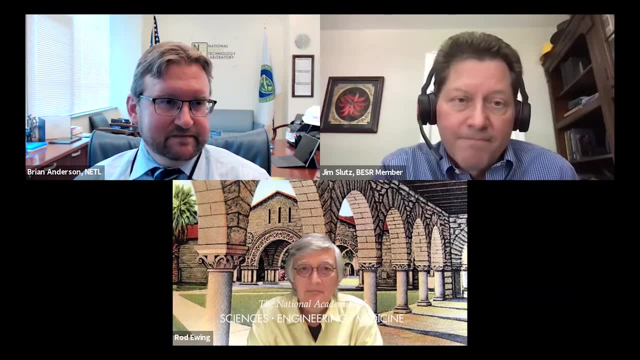 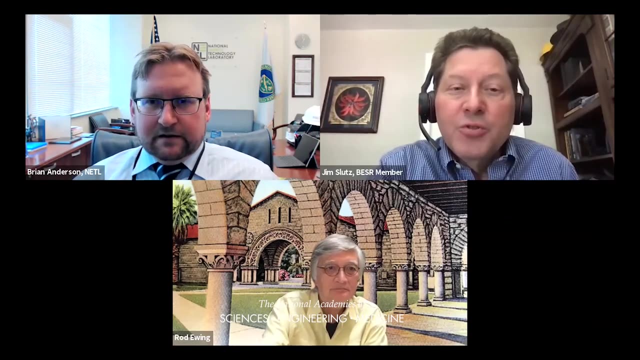 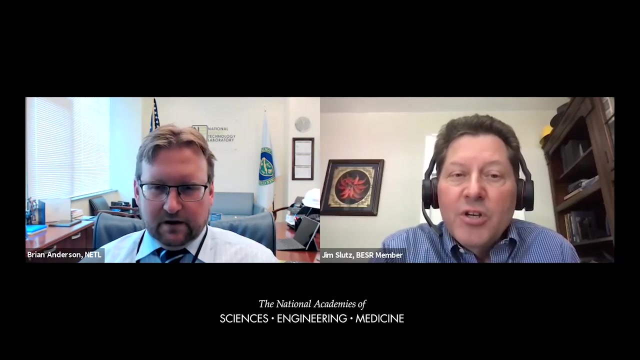 They're different to difficult to compare one one to another, And that's where there's a lot of social policy and, You know, social equity questions that come up. Thank you, Thanks, Rod. Hey, hey, Brian, we just have a few minutes left. So what I'm going to do, if you're okay, we'll do some of these questions more like a lightning round. I'll just I'll touch on a few different questions and then maybe you can do some wrap up comments to try to address those. 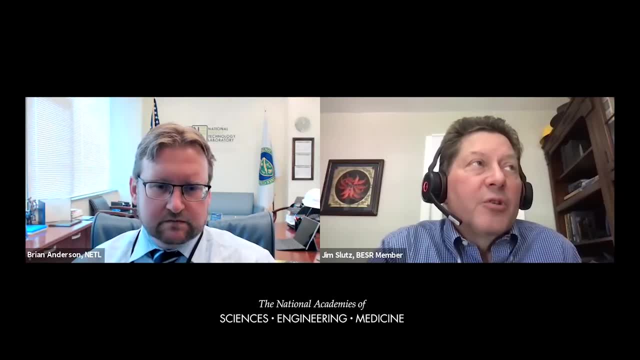 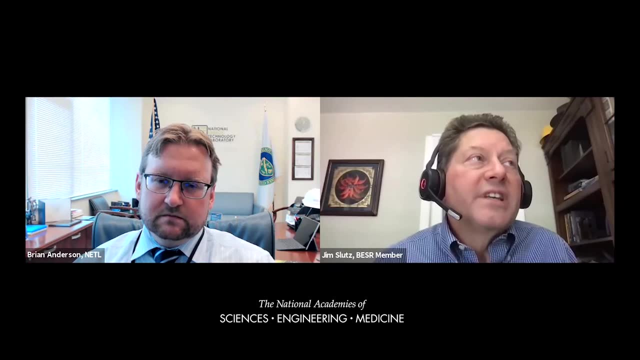 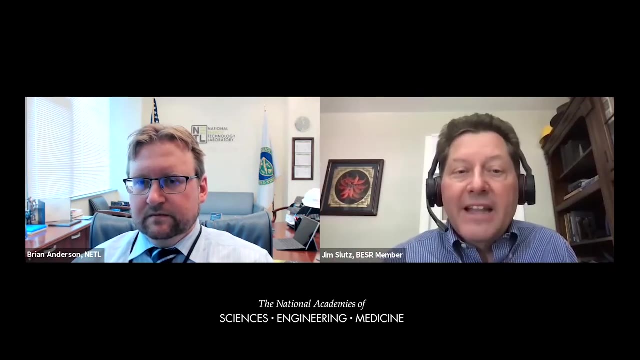 And so we'll. there's one about efforts to decarbonize over, you know, over a 30 year period, and and are there? What do you see as as kind of critical policy actions that might be needed to implement those? Let me, let me add to that. or what are some of the critical path items in research? maybe as well, I think, would be of interest to people that you're seeing. 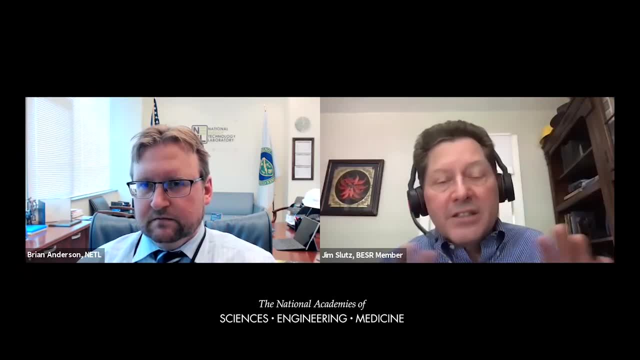 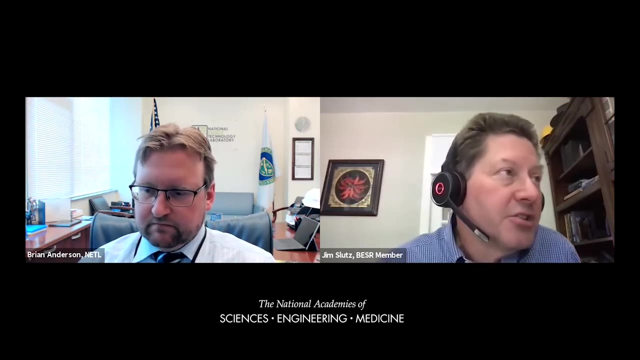 And then there's a question about it's. it's under methane sequestration. but I think the broader, you know methane is getting a lot of attention. the UN issued a report last week about it. You know what, what? You know what, some of the little bit more on your, you know, methane reduction and some of the technology areas, and and then the. the final issue is the broader than than is these transformative technologies and sometimes government, the government regulations. 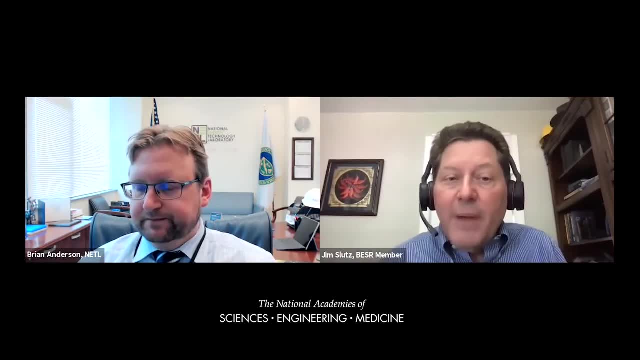 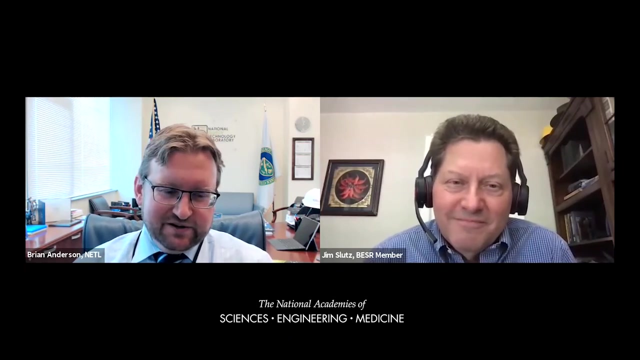 don't really accommodate new technology well, so kind of a pathways on regulation that may be that interface between technology and regulation. so three things, kind of critical, critical policy, end and regulation. So I'm going to lump the policy and regulation together. is that we needed it? we? we do need a comprehensive energy policy framework. that you know right now. 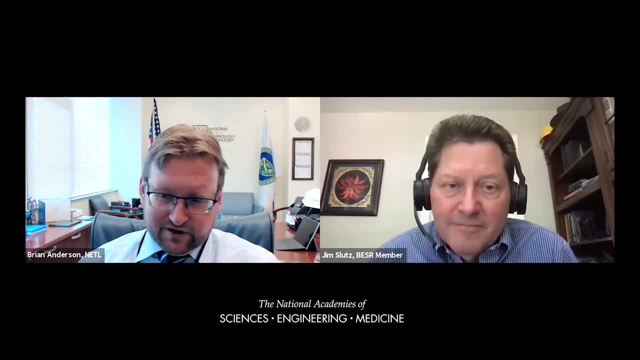 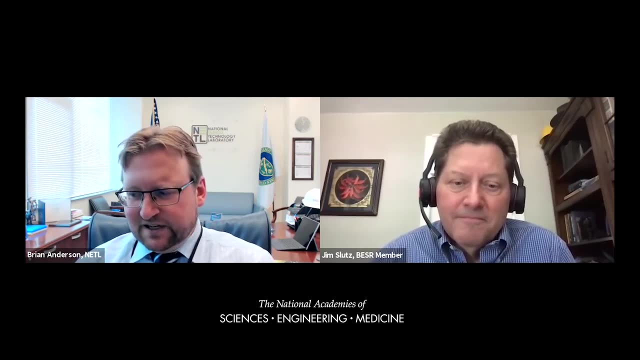 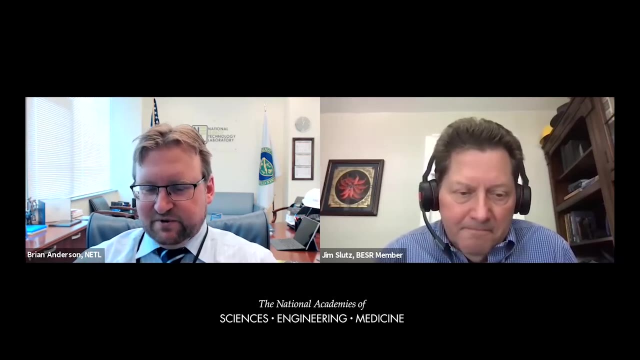 So we have a combination of investment tax credits and production tax credits. 45 Q looks kind of like a production tax credit When you compare it to the PTC- is on on wind and solar. And then we have a transition to a real comprehensive policy portfolio that touches on investing in technologies to move them over the barrier. but then we certainly don't have a policy framework for the pathway of reduction of co2 as a whole. 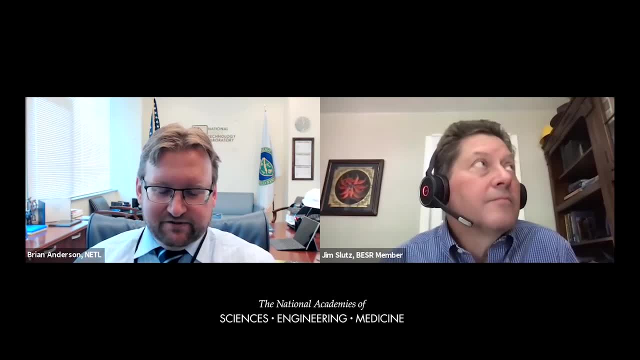 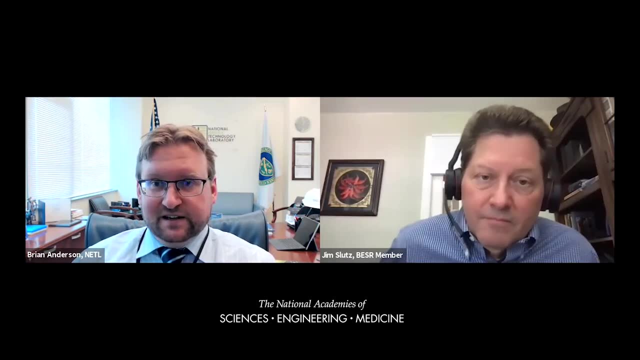 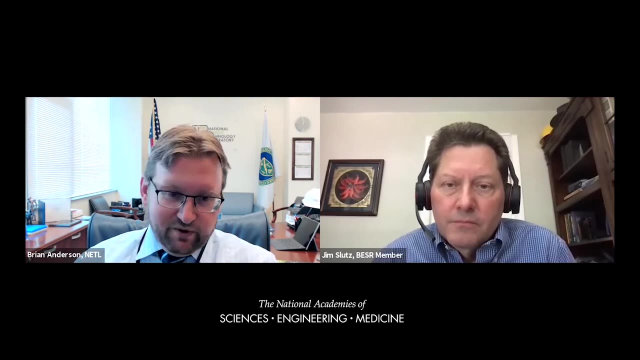 So we need that. That includes that policy framework needs to include the ability and the regulatory environment to be able to permit new, new projects More rapidly, particularly if we see that co2 sequestration is necessary, necessary. we will have interstate pipelines of CO2 and the ability to permit that and move it. 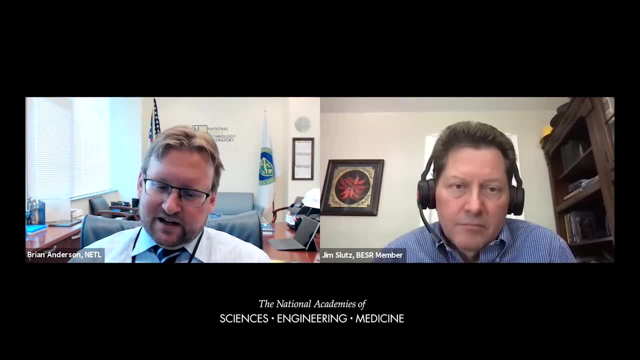 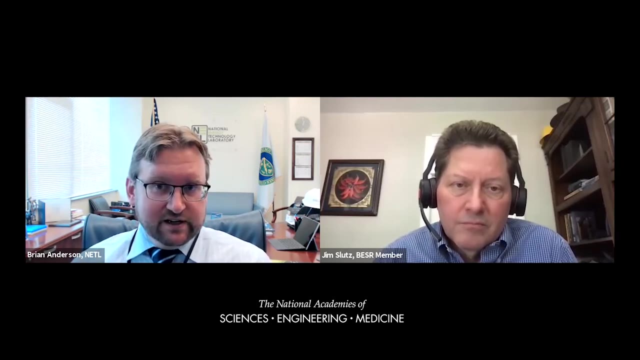 forward using existing rights-of-way technologies that we need. Certainly, grid-scale storage remains one of the big issues to be able to handle the hour-by-hour variability of increasing variable renewables onto the grid. In addition to you know, I think that CCUS is a critical 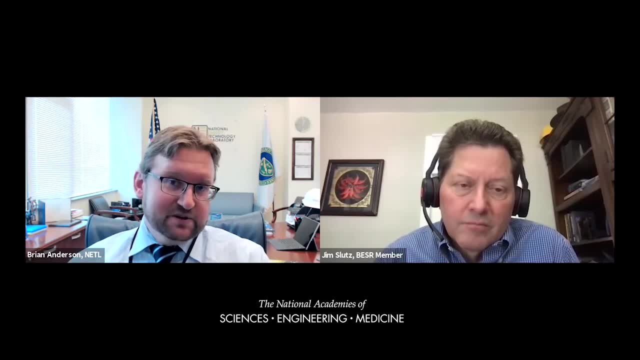 pathway. Once we get to 60 or 70 percent decarbonization, we really must have CCUS technologies ready to go. So then we have long lead-term items in order to be ready for that, and that includes a lot of the infrastructure that needs to get out front. And then 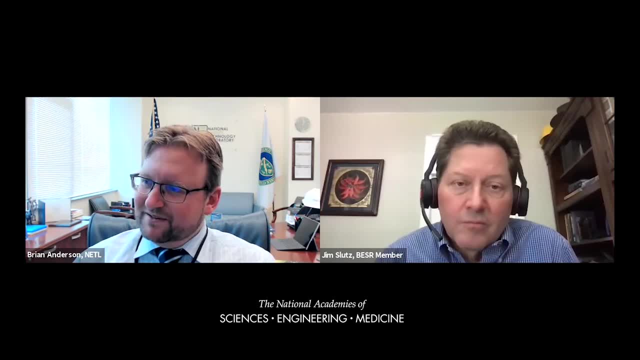 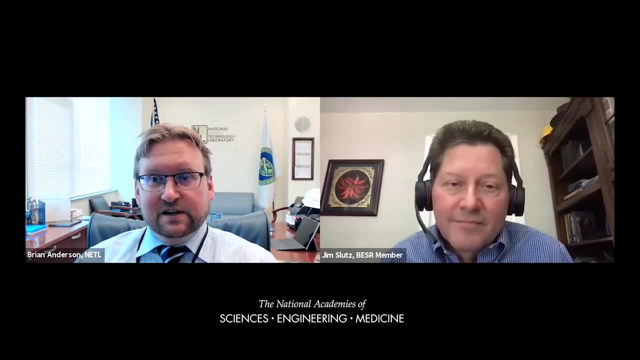 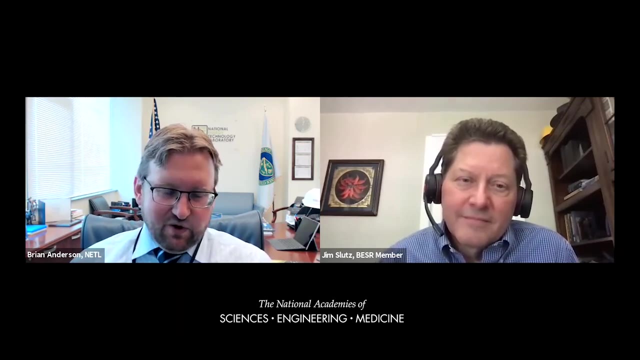 oh shoot, I missed the one in the middle. Oh, methane, Methane. you know we have a pretty robust portfolio in detection of methane, So across the entire infrastructure portfolio to be able to detect where it is, categorize and measure and quantify methane emissions, as well as new. 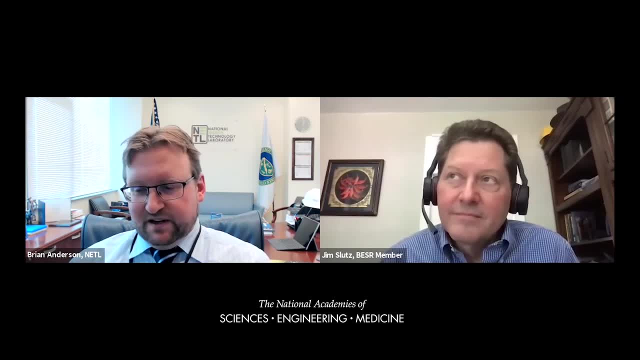 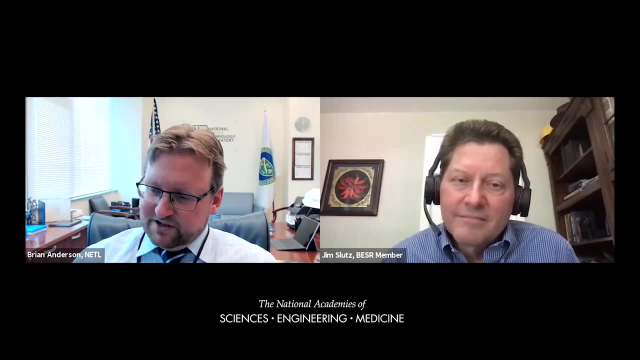 technologies for even converting a natural gas compressor stations, as well as new materials to mitigate methane. Now, in terms of- you know the question of sequestration of methane, we store, as Bob mentioned, we store methane natural gas underground, as it is today. 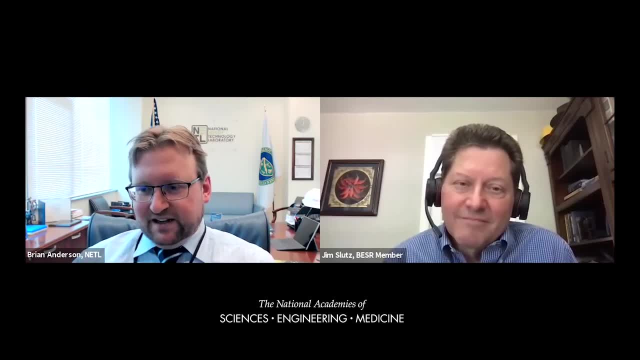 But in fact, if you capture the methane, you would end up using it. you know if methane is a climate-forcing gas much stronger than CO2, so it's actually better to burn it, burn it and capture the CO2 and get the energy out of it than perhaps sequester it. 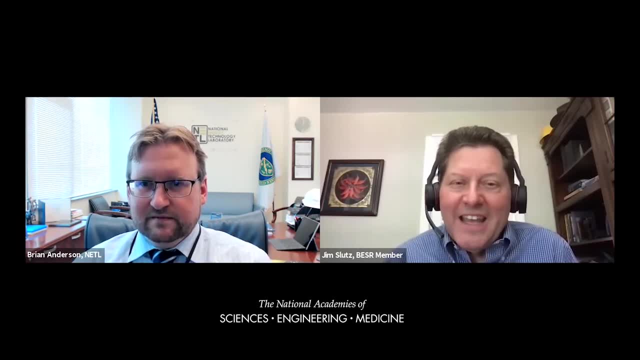 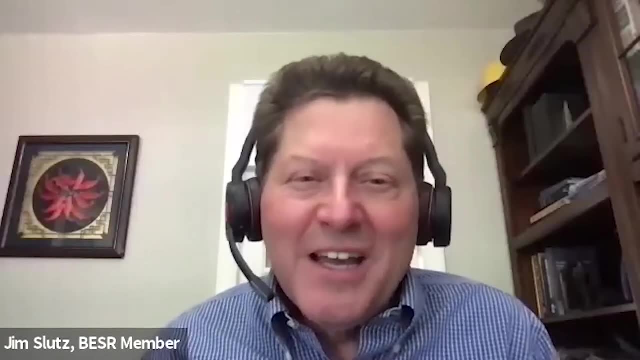 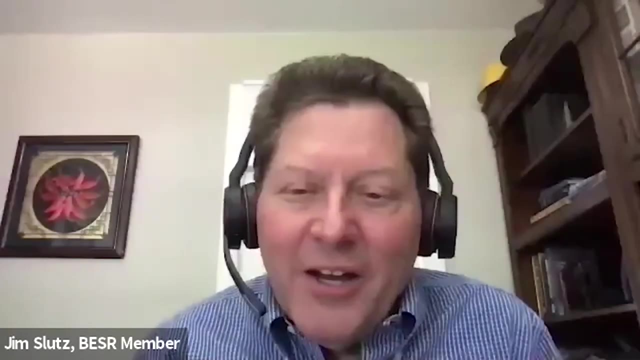 Well, Brian, thanks so much for joining us today, Thanks for this great kickoff And let's all give Brian a virtual round of applause for this great opening. Appreciate it. We'll look forward to staying engaged with you, Brian and NETL, And I know the board is going to be very, very, very. 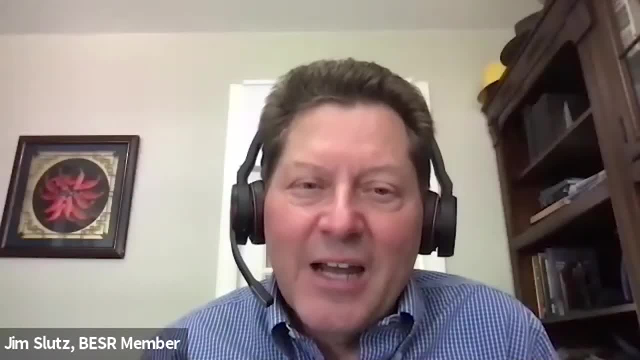 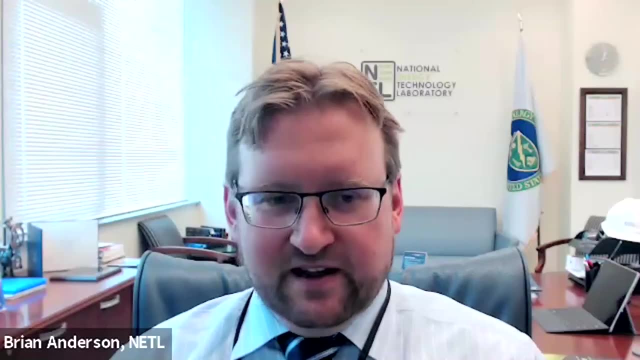 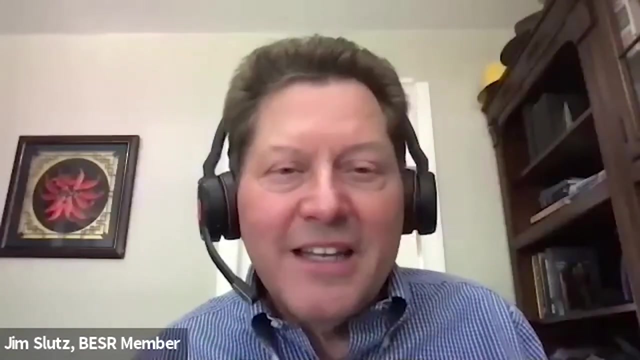 very excited about this And I think the board and all of our committees, as well as other places in the National Academies of Science, Engineering and Medicine, really consider the NETL relationship critical. I thank you for the opportunity And with that, let me hand the mic over to. 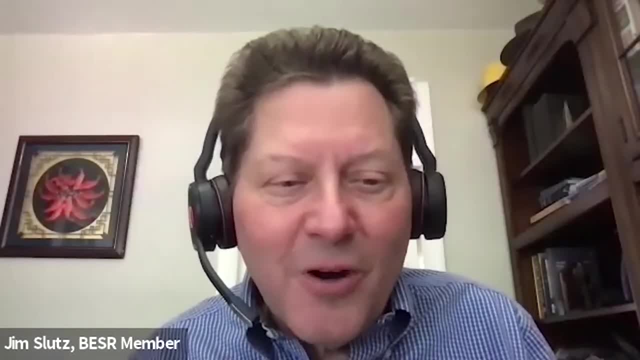 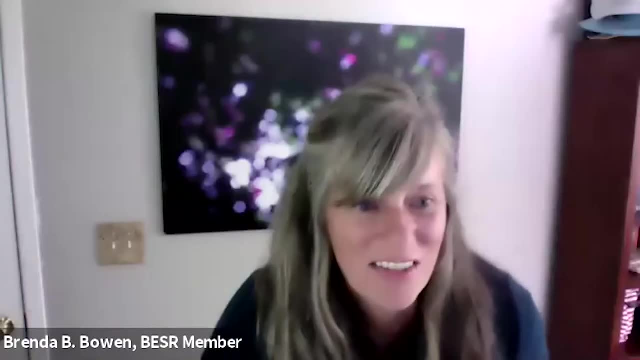 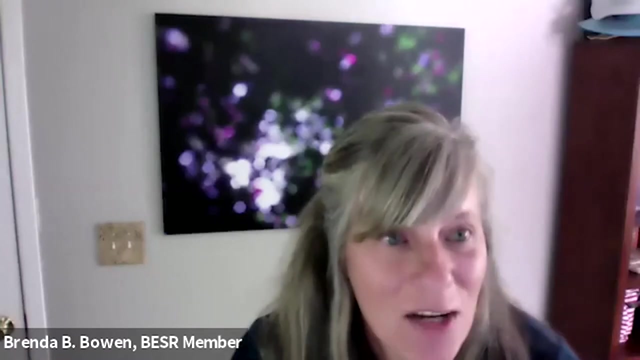 Brenda Bowen, who is going to moderate our next panel today. Thank you Great. Thank you, Jim. So we have a great panel lined up for today where we'll be exploring the land and water impacts and trade-offs of the energy transition that we've been talking about. 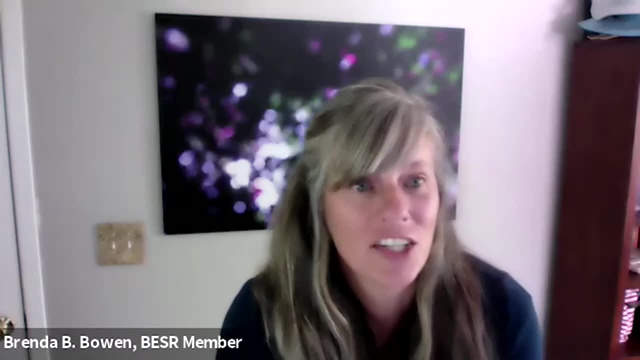 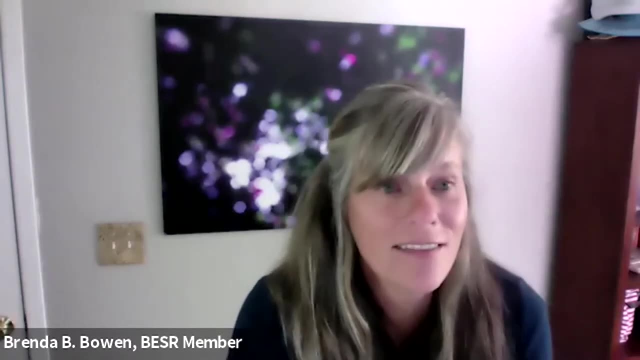 We'll hear about produced water, about renewable energy, sustainability and enhanced weathering. Speakers will touch on resource needs, industry relevance, environmental impacts and connections to communities. After each speaker, we'll have a few minutes for questions, And so please feel free to enter your questions into the. 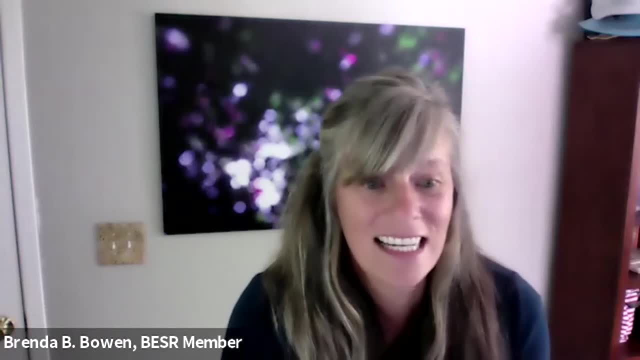 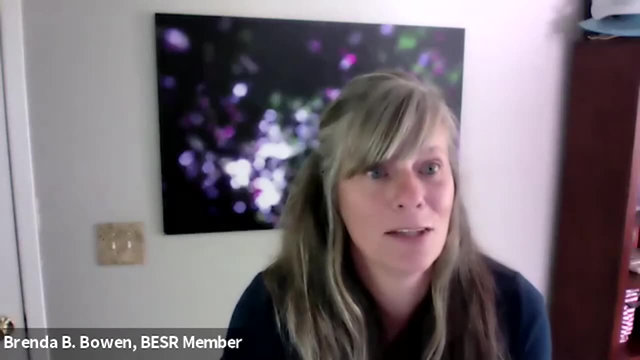 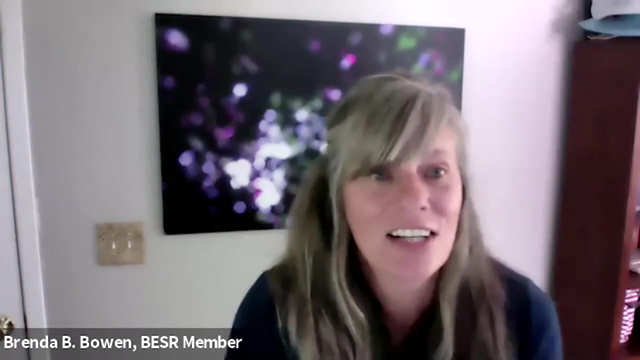 Q&A as we're hearing their presentations And then we will take a short break and then come back together for a full panel discussion with the whole group. So we'll begin our panel with Nicole Saunders. Nicole is a senior attorney with the Environmental Defense Fund in their energy program. 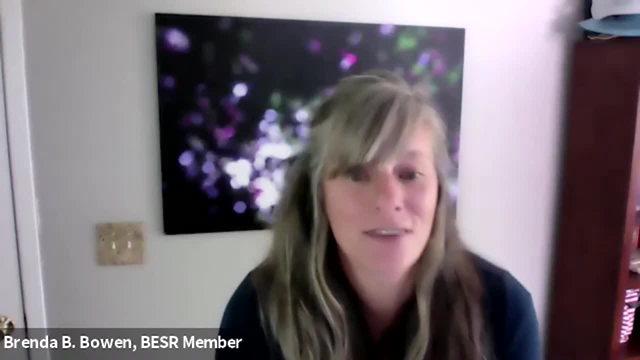 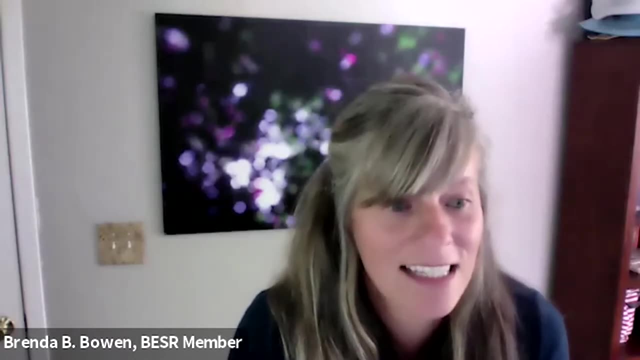 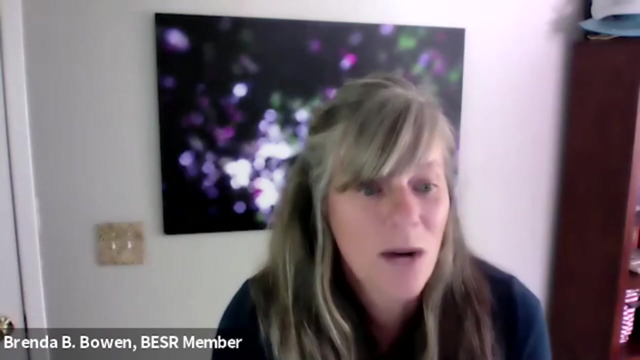 Her work is devoted to ensuring that science-based regulations, policies and industrial practices are in place to reduce human health and environmental impacts from energy development. She focuses on the management and disposal of oil and gas wastewater, as well as policies to ensure environmental integrity in emerging carbon. 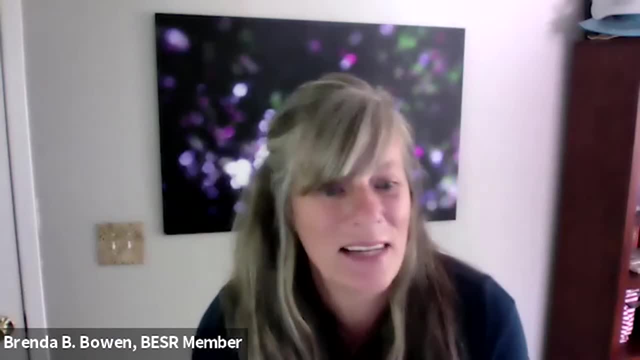 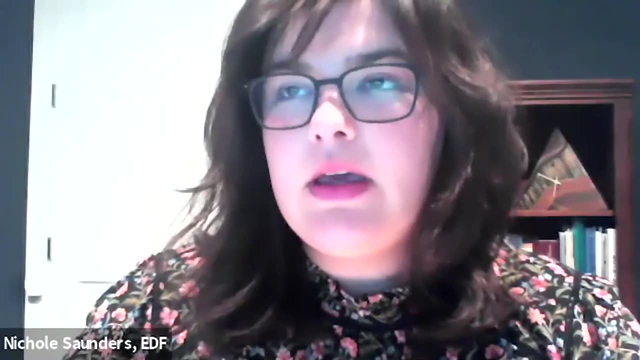 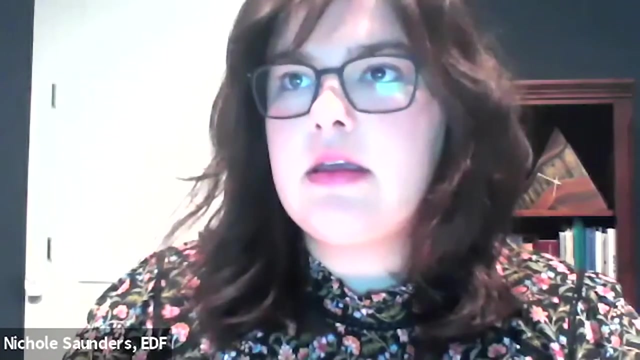 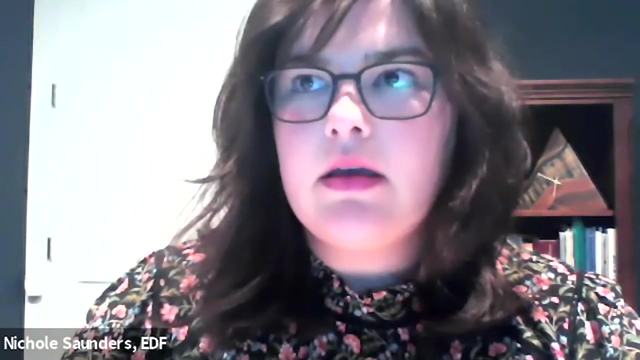 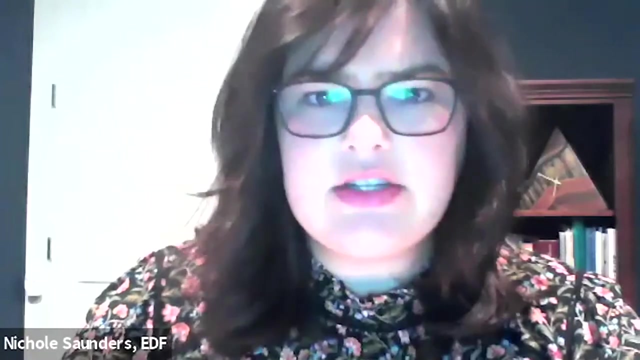 capture and sequestration projects. Nicole, thank you for being with us here today And I'll pass it over to you. Great, Thank you so much. I'm going to um share my screen quickly. Can you all see slide one of my presentation? 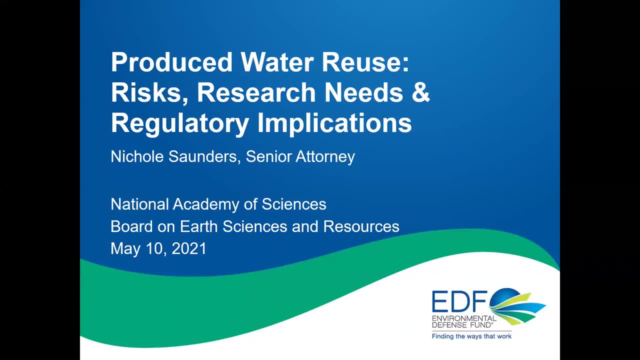 We're not seeing it yet. Here it goes. Yep, Great, Took it a little second, but we're there, All right, Thank you so much, So I'm going to kick it off. I just want to thank the national academies and this board for having me. 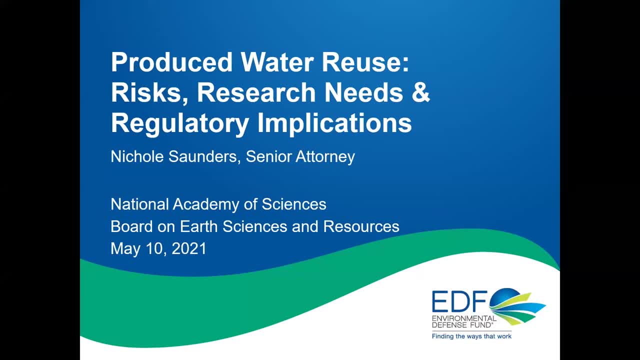 today to have this great discussion as we speak on the theme of transition. I'm actually really glad to have this opportunity to talk to you about a more of an emerging issue in the energy water arena, which is the growing interest in looking at oil and gas wastewater or produce water for its reuse potential. 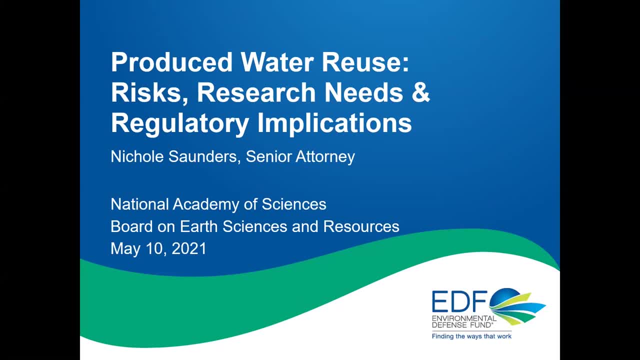 So for many years now, EDF has been collaborating with academics, industry and other experts to better understand the science of produced water and its chemical character, treatment and toxicity. all of that towards being able to inform policy and regulatory decision making as this question evolves. 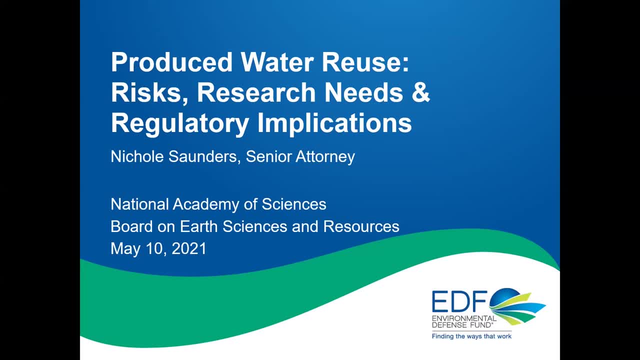 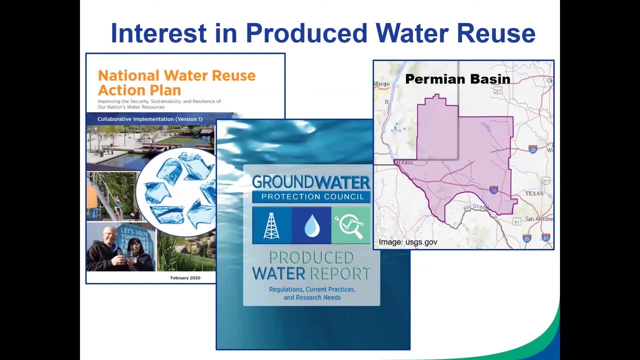 And so please bear with me as I try to move through some of our most recent findings and data for your consideration at kind of a quick pace. to stay on track. Today produced water. as I'm sure most of you all know, is a mixture of formation, groundwater, chemical and fluids used in production and anything that results from the mixture of these two things. it returns to the surface with oil and gas. 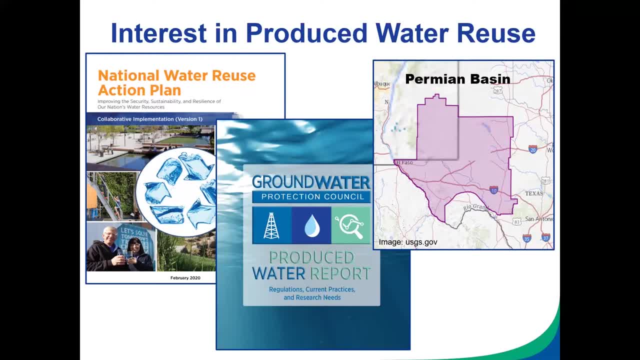 And in many places it returns in much larger volumes actually than the hydrocarbon itself. Nationally, a little over a trillion gallons of produced water surface annually, And the predominant method for managing this waste Stream, both historically and today, is the reinjection over 90% of produce waters managed this way. 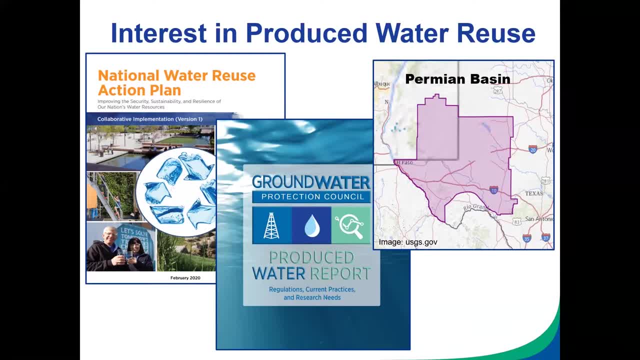 However, as regions grapple with the effects of climate change, drought, disposal challenges like seismicity, and other business and economic streams, many are beginning to look at this waste stream as for its potential as a resource, And so there are numerous recent publications and plans that identify this issue. 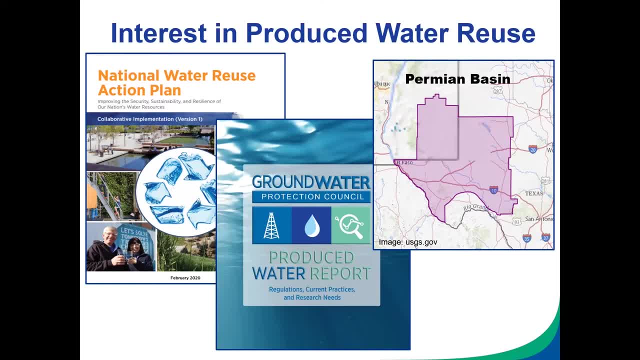 that you could look to for broader discussion. One of those is EPA's Water Reuse Act, Which includes produced water and one of the five major sources of water for potential reuse. The Groundwater Protection Council's report on produced water is arguably the best existing primer on the multiple facets of this issue. I'm somewhat biased, I should disclose. I was one of the authors and on the leadership group for this. 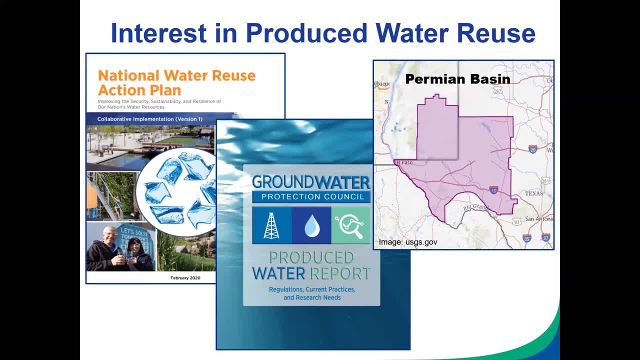 But it really is a fantastic resource and includes multiple modules on things like research needs, technical considerations, regulatory considerations. I just want to highlight a couple of things. I just want to highlight that the Permian Basin, which is kind of a hot spot for this issue- no pun intended, necessarily, but New Mexico is in year two of a research consortium aimed at addressing some of these questions related to reuse. 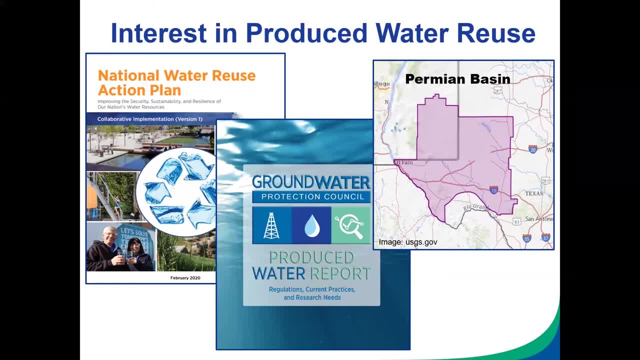 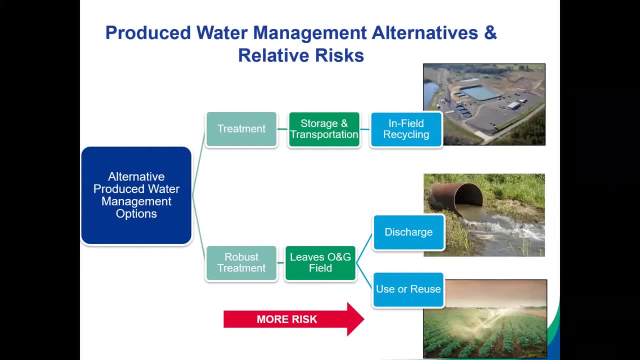 And Texas is moving towards likely passing a bill that will set up a similar stakeholder group. So what are we really talking about when we talk about produced water reuse in this context? So there are two main buckets Utilizing produced water to supplement or replace freshwater use for oilfields. 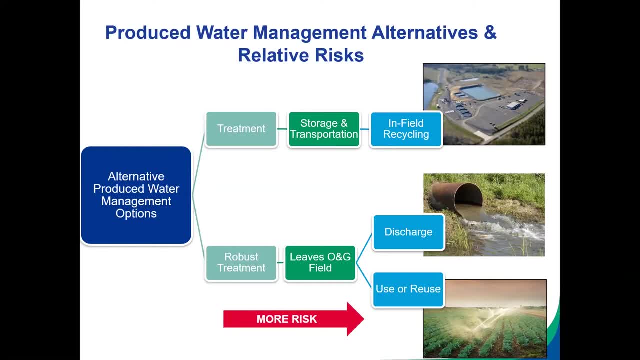 Utilizing produced water to supplement or replace freshwater use for oilfield operations is chief among these alternatives, And if it's conducted in a manner that really reduces spills and leaks, this is this is a really good forward momentum opportunity. It's a positive move away from putting pressure on local freshwater resources for development. 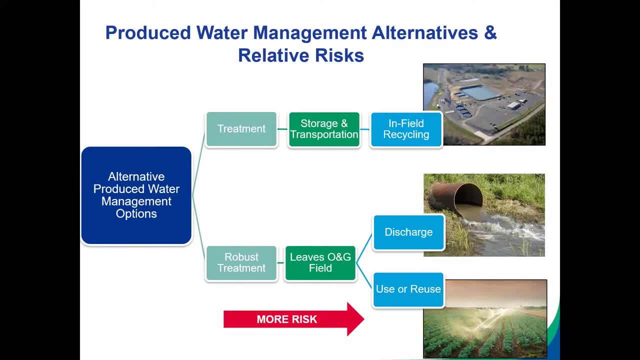 I'm actually not going to spend my time talking with you about this option for reuse today. What I want to spend more time about are these alternatives to look at the release or reuse of treated produced waters. What I want to spend more time about are these alternatives to look at the release or reuse of treated produced waters outside of the oil and gas environment. 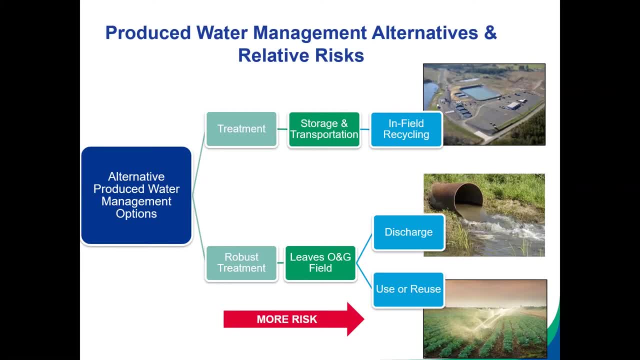 These are come with much more complex considerations surrounding identifying and appropriately managing risk. A chief among these challenges is a really a foundational limitation in our knowledge regarding the more comprehensive chemical and toxicological character of produced water, Combined with a present lack of really updated regulatory programs that are designed to manage this. 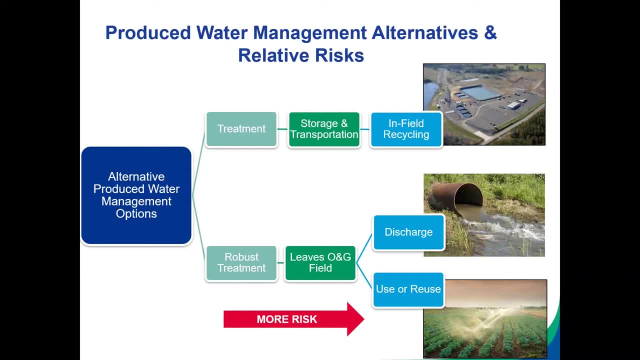 wastewater in these new ways, And that's primarily due to a lack of a historical need for this kind of research around produce water because of the tradition of managing produce water through underground injection. So with the time I have today, I want to give you a really high level overview of these issues and better and EDF's work to better elucidate the challenges ahead. 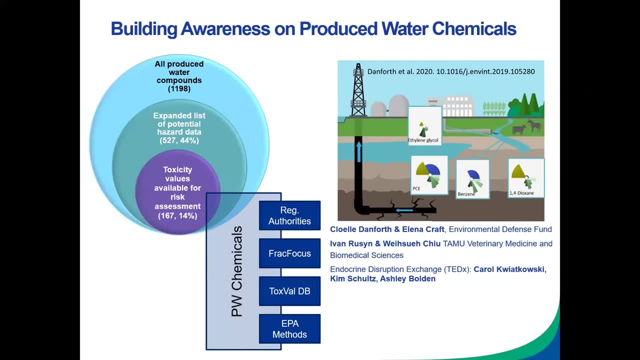 So a key area of work for us has been focused on trying to tease out what we know and don't know about the chemicals in produce water itself, Because we've identified this as a as a real challenge. So our health scientists worked with Texas A&M and the Endocrine Disruption Exchange to review the literature and identify studies on produce water. 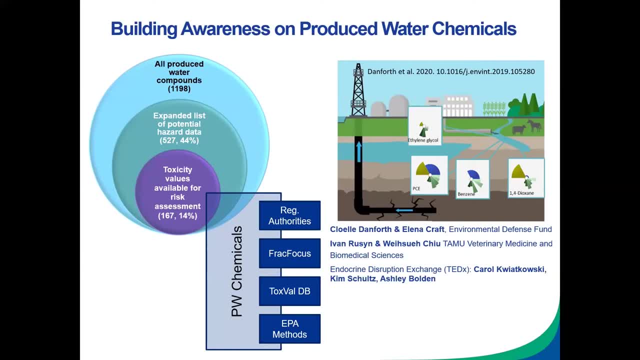 And we use that to develop a comprehensive database and a framework to prioritize those chemicals. That paper and the database are available in an open source journal. that DOI is on your slide. So in this first review we identified a little under 1200 constituents in produce waters nationally. 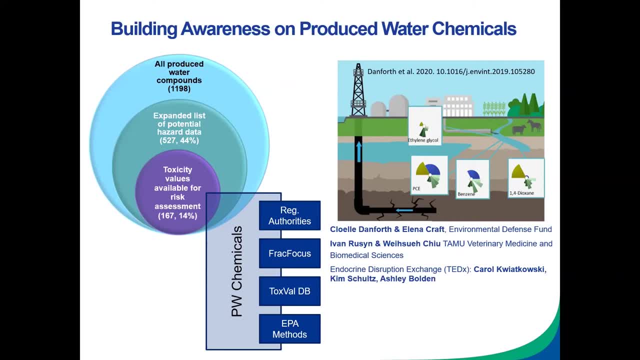 And so using that, Using this database, we were able to do things And across research, across other forms of information. So, for example, we were able to take our database and crosswalk it with available toxicological data And see what we have for these produce water constituents, and it turns out the answer is really very little. So less than 14% of the constituents in this database have the type of toxicity you would need to conduct really a good risk assessment. 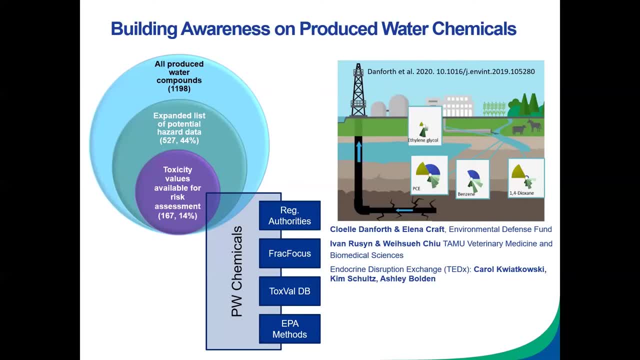 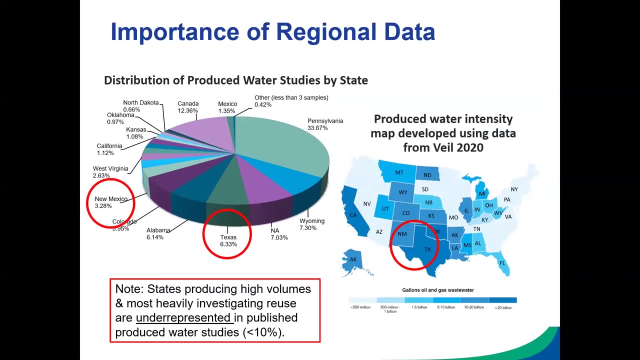 And we were also able to look at how these chemicals were represented on other lists or databases like regulatory programs that might apply if you look to discharge or reuse, And I'm going to talk about that more here in a moment. One key point I want to make quickly about the database is a really a notable limitation in the data set. We are limited. 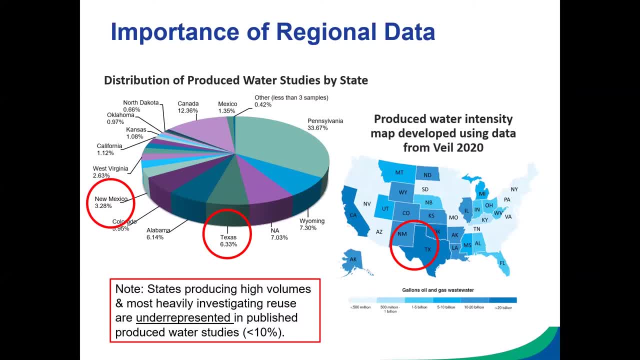 To gathering data only where produce waters have been tested and studied and only on what was actually looked for. So that common issue of you're only going to find what you're going to find. So that common issue of you're only going to find what you're going to find. 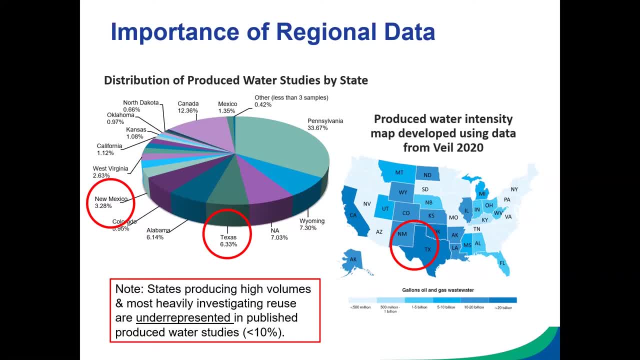 So that common issue of you're only going to find what you're going to find. So that common issue of you're only going to find what you're looking for. and so regional variation is a really important example. on this slide I have two graphics on. the one on the right represents the latest compiled. 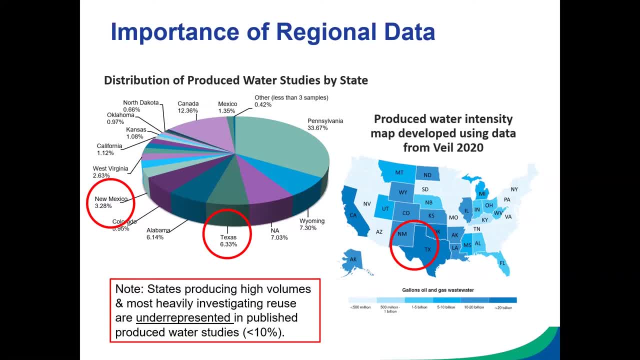 Data in a report form on produce water volumes alone and it's kind of an intensity map. So I've circled the area in the southwest, whereas the Permian Basin where we see large volumes and where there's this growing interest in Alternative forms of reuse. and on the contrast, on the left is a distribution of our produce water studies. 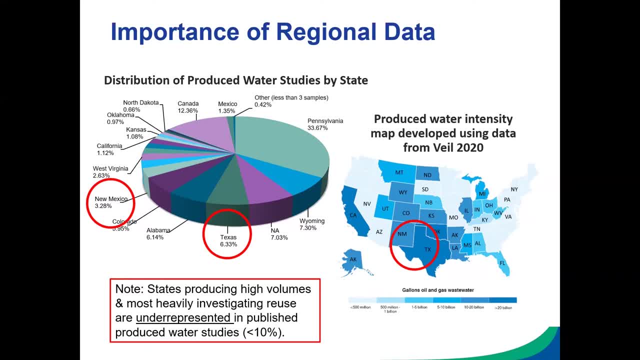 That we compiled by state, and you can see that these two things don't overlap. So the states producing really high volumes of produce water and investigating its reuse are really drastically underrepresented in the published literature. So, generally speaking, we don't have enough data about produce water. but a more important point is that decision makers, especially regulators- 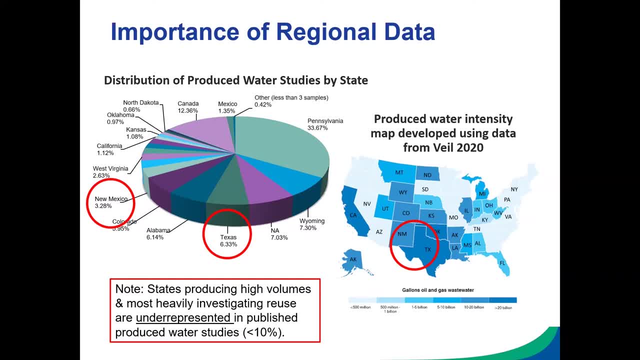 Really need information about their region, specific produce water, and that's because produce water is highly variable. You know, if you look at Geography, geology, time, operator to operator, well to well, day to day, we can generalize, yes, but the regional data will be really key in making informed and protective decisions. 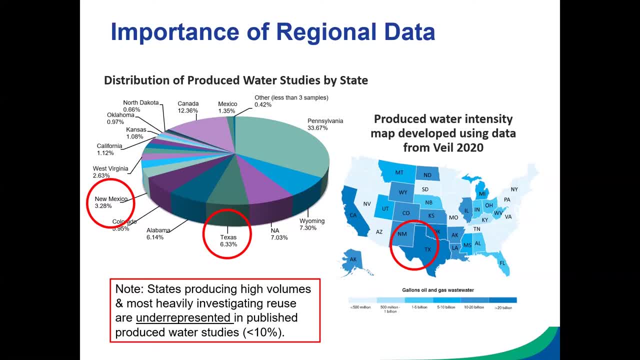 And we don't necessarily have enough of it where we need it. So I want to turn now to share a little bit more specific data and talk about what these research challenges and knowledge gaps might mean in a regulatory context as we think about the potential for expanded reuse. 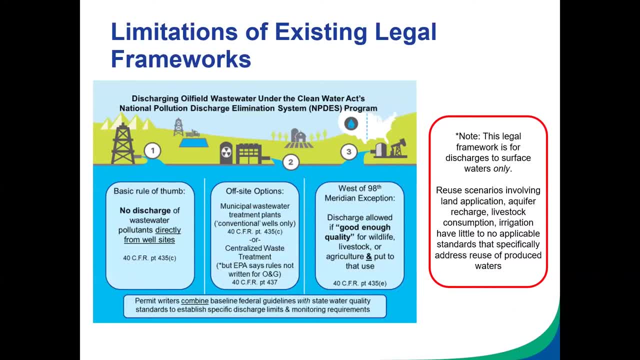 So really quickly from a regulatory framework. simply put, the frameworks for produce water, discharge and reuse are pretty limited. They really weren't written with the idea of widespread discharge and reuse in mind and don't usually specifically address the constituents of concern we find in the literature on produce water. 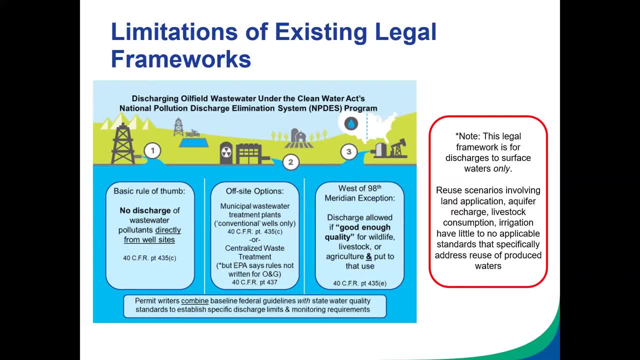 And because it represents the most comprehensive existing framework. I'm going to focus on surface discharges in the Clean Water Act today, But a huge big difference here is that this framework that I'm talking about in this initial analysis that we've done is not for discharges outside of the Clean Water Act. So other scenarios that are considered, like land application, irrigation, aquifer recharge. 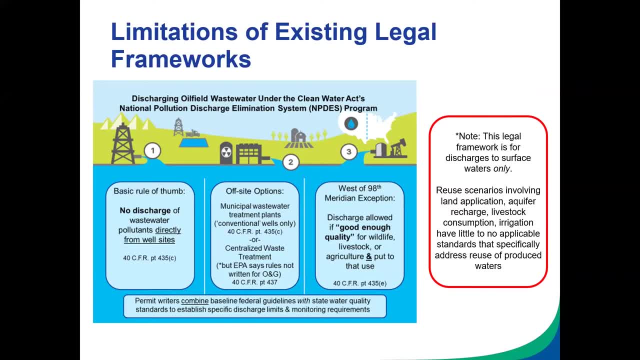 they really have little to no applicable standards or regulatory programs that are specifically equipped to consider and apply to reuse of produce waters and the constituents were concerned about there, So I'll put that on as a a major gap. that's worth further research, But in the NPDES program under the Clean Water Act, 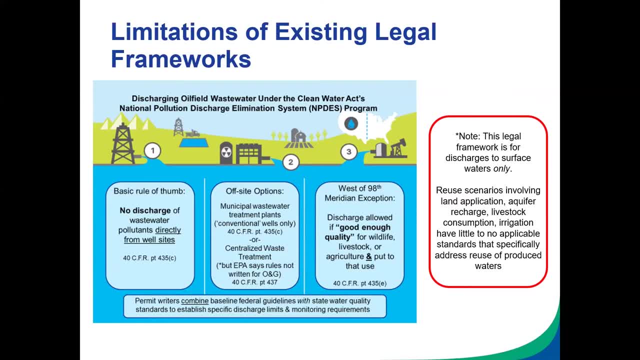 the basic rule of thumb is that no discharge of produce water is allowed direct from an operating site, with two key exceptions to know about. First, an operator can transport their produce water offsite to a POTW or a CWT. These are two types of treatment facilities. 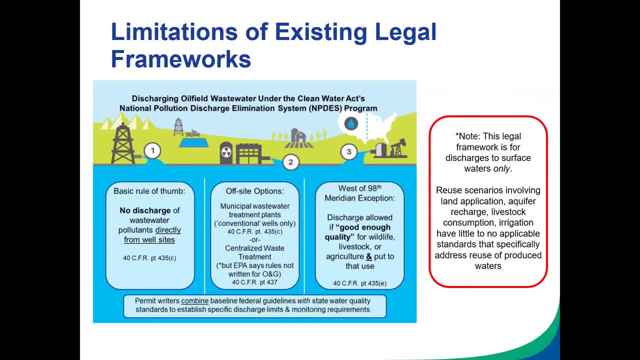 Treatment and discharge via a municipal facility or a POTW is allowed for only for conventional oil and gas facilities And usually occurs in really limited areas, predominantly in the Marcellus region in the Northeast. Treatment and discharge via a CWT or more centralized industrial treatment facility happens at a handful of facilities, again predominantly in the Northeast. 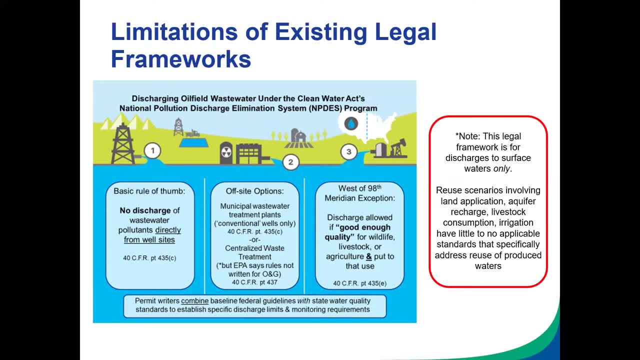 But that has been recently studied by EPA, who identified a number of concerns about the applicability of the program to produce water. And finally, there's an important consideration to the no discharge rule, where, if you're west of the underneath meridian, 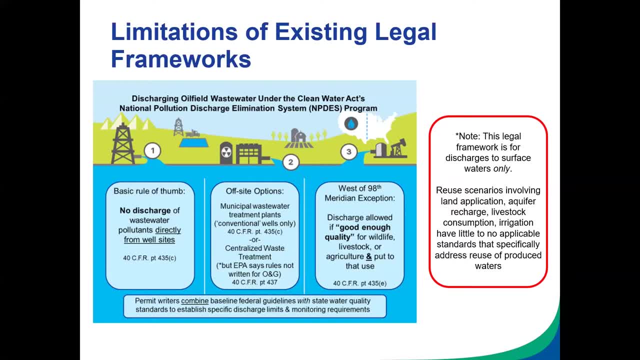 discharges from well sites are allowed if they're of good enough quality for wildlife, livestock, ag and are put to those uses. So the question really becomes here: how do we define good enough quality or define what the appropriate regulatory program for reuse really looks like? 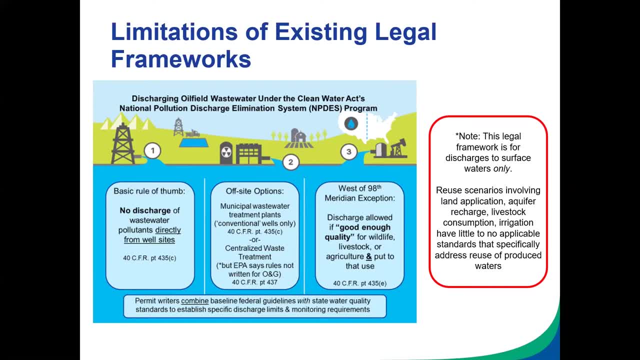 And permit writers are left to answer these questions, and doing so is complex. So when we're looking to establish or regulatory permitting program, there are a number of basic questions that we were thinking about when we started to think about how we could use our database to help. What constituents are we concerned about? Are 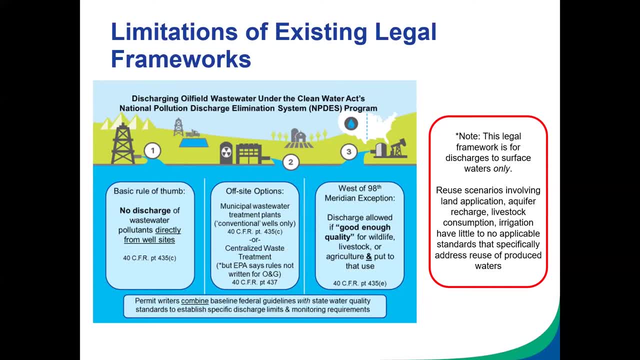 there approved analytical methods, meaning methods that can detect and quantify a constituent and be used in a regulatory environment that's legally enforceable? Are there existing standards we might be able to look at? Do we have the toxicity information? we need to understand what, who. 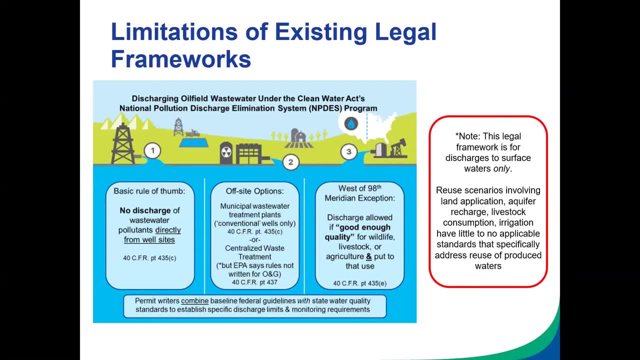 and at what levels these pollutants might come into contact with and might they cause harm. So EDF has recently updated our database and used the tool to start breaking down some of these challenges, And so this presents at a really high level some of our findings, So basically, our new. 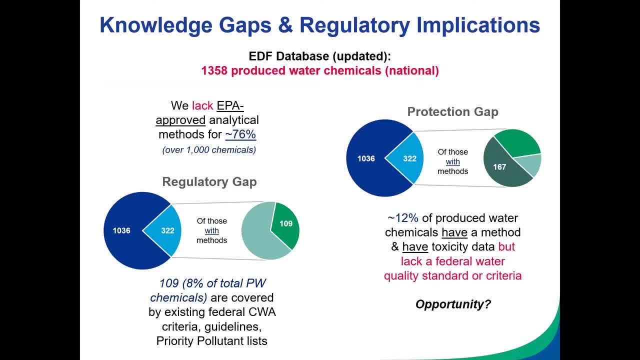 database has a little over 1,350 produced water constituents. So if you look at the EPA-approved analytical methods- the kind of methods you'd need in a regulatory environment- we have a detection challenge. Not only are there limitations in what's disclosed as being put down whole, but we're also 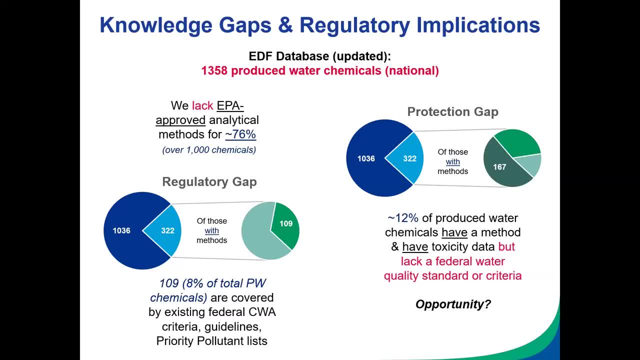 dealing with a lot of things that are not disclosed as being put down whole. We're also dealing with a large number of chemicals that really haven't otherwise been incorporated into programs and needed a method. So less than 25 percent of these constituents have approved analytical methods. 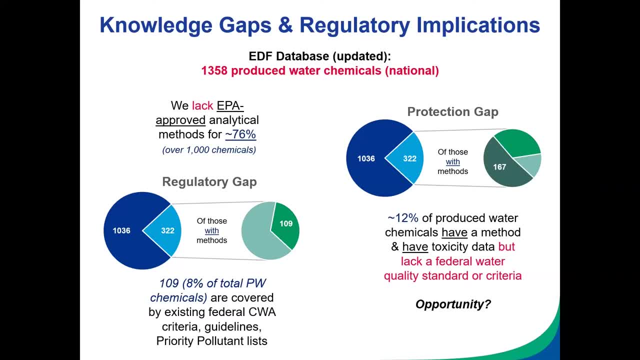 So if we want to look at what we have available today in the world of standards- we want to. we want to, first and foremost, look: okay, where can we assess a constituent and know that we have a standard if we wanted to incorporate it into? 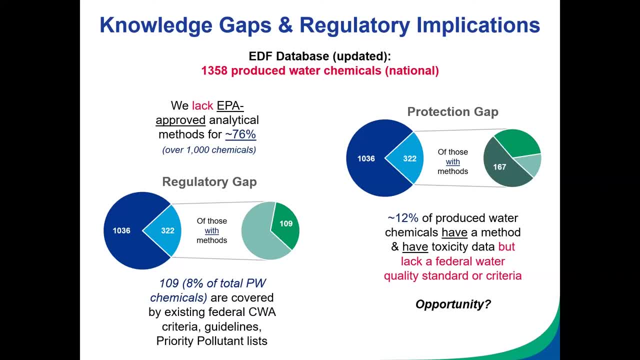 a regulatory program. So right off the bat we lose about coverage for about a thousand potential constituents because we don't have the analytical methods today. For those that are left, are there opportunities? Am I at my time? Brenda, You can go for another another minute or so. 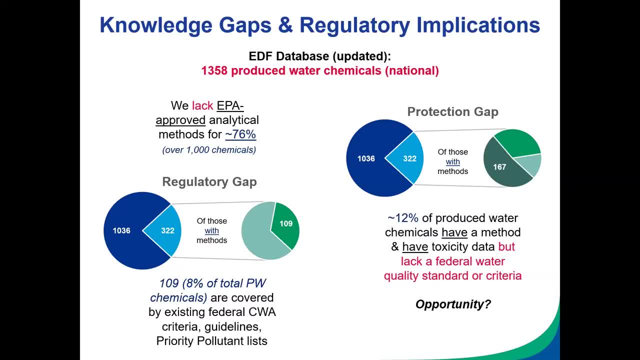 Great, okay, So of those, there are about a little over a hundred that are already covered in the Clean Water Act, And of those, there are about 167 that actually do have comprehensive toxicity data, And so what I? what I'm moving through here is there are some opportunities to 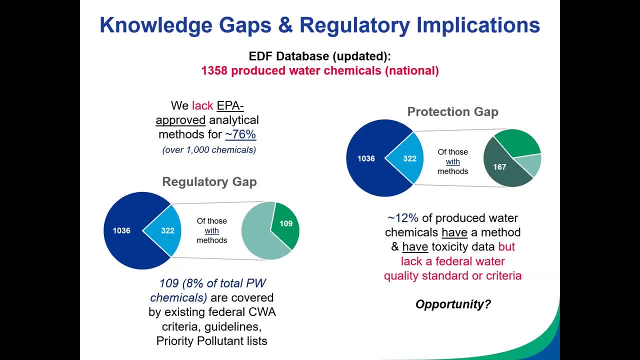 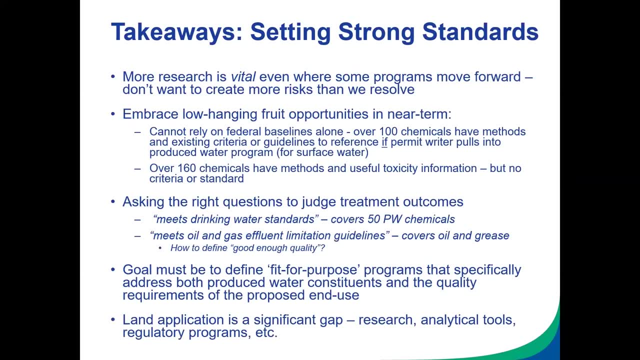 look at standards that we have today that are covered by that. constituents are covered. So really quickly, I'm just going to put this slide up and I'll move through it so I can. If the interest in looking to produce water as a resource really holds, it's vital that necessary. 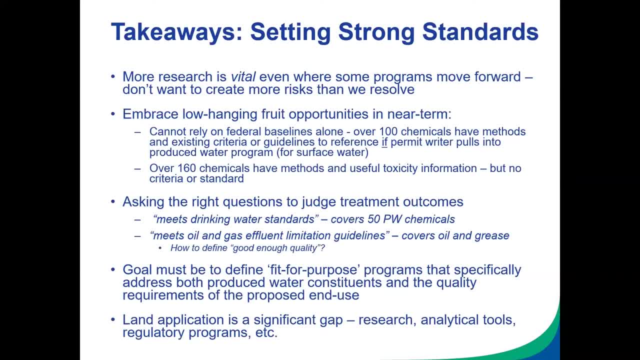 research and regulatory development is done to ensure that we can write the appropriate protective permits that don't inadvertently allow for beneficial research. So I'm going to start with the first slide. So there are some standards that we need to be able to use to inform our existing freshwater ecosystems, wildlife and public health. 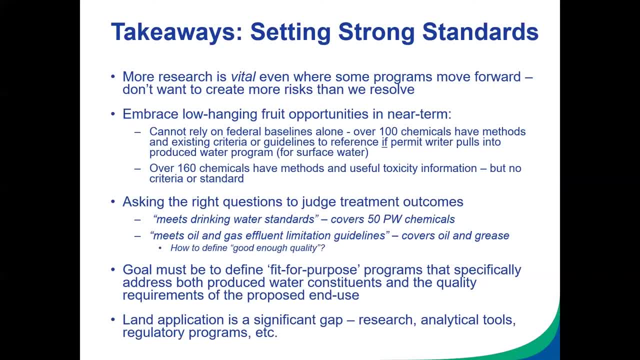 So more research is really key And there are some low-hanging fruit opportunities, like I mentioned, where there are standards on the books that we might be able to use if we incorporate them into a permitting program, And we might need to look at where. 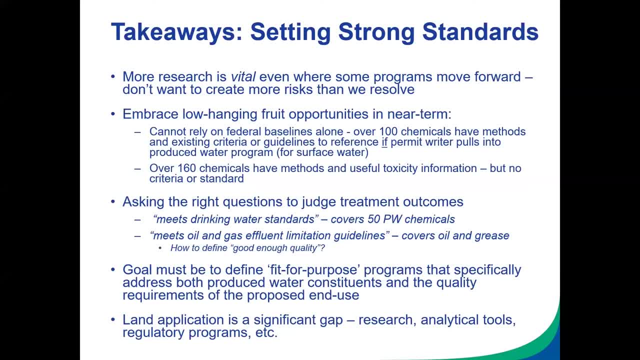 we have toxicity data and could use that to develop new standards or inform more appropriate research, And all of this is really to ensure that we're asking the right decisions as society, as regulators, as researchers. how are we judging the viability of this practice of? 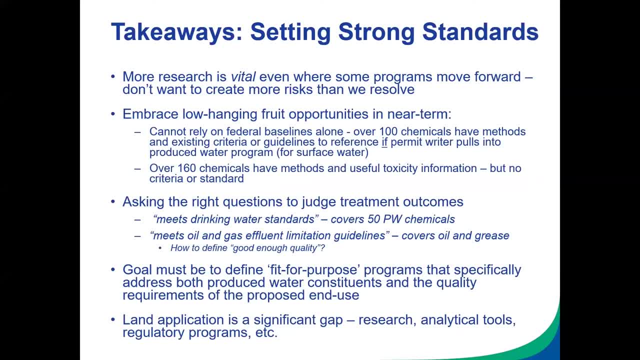 produce water use. So you'll often see a question like: see a position that produce water can be treated to meet drinking water standards but that really only covers about 50 produce water constituents and may not be really the constituents we're most worried about. 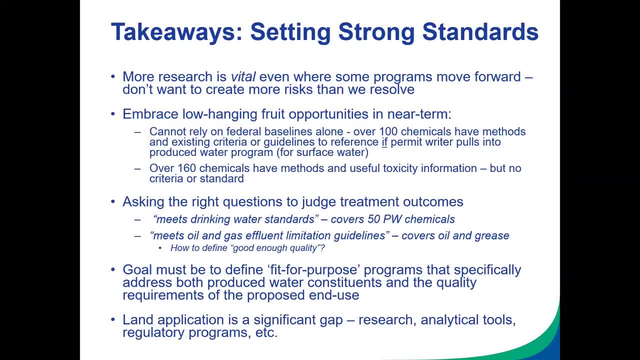 Or it might say: this meets the oil and gas effluent limitation guideline, but that has only one standard for oil and grease. So the end of the slide answer is really: how are we defining good enough quality And are we asking the right? 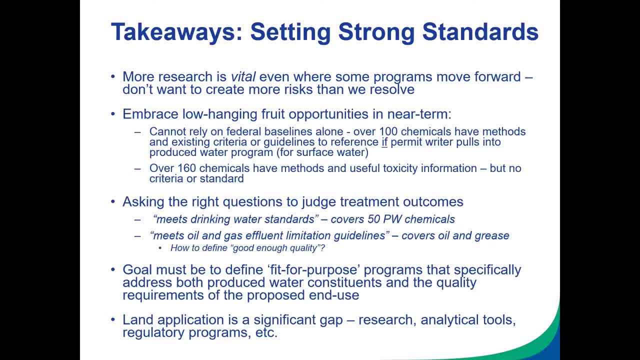 questions about produce water to look at this opportunity for reuse. We really want to design these fit for purpose programs that we know are based on an understanding of produce water, knowing what the requirements for your end use are, based on those constituents that are concerned in produce water, and design a program that meets those targets. And there's just a. 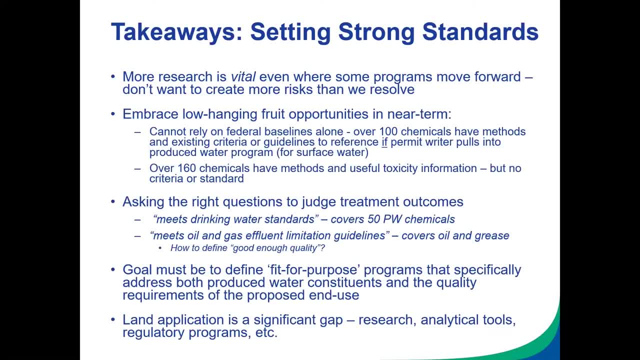 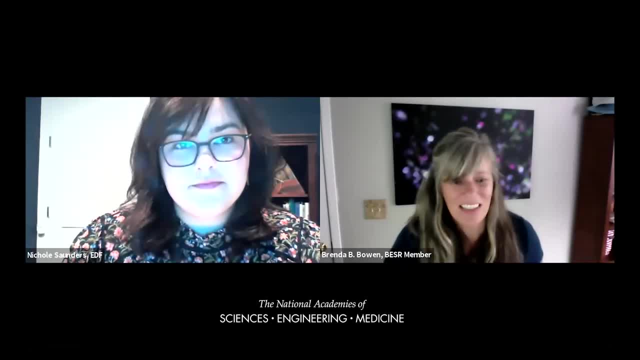 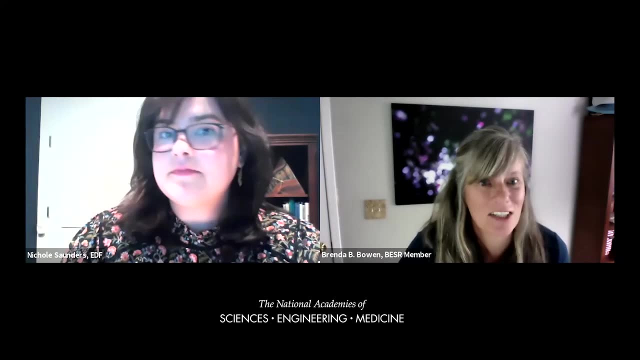 lot of research that we need to do if we want to get there. So I will wrap up there. Great, Thank you, Nicole. Really interesting to think about: produce, water reuse and where we need to go with research and priorities there. Want to invite any board? 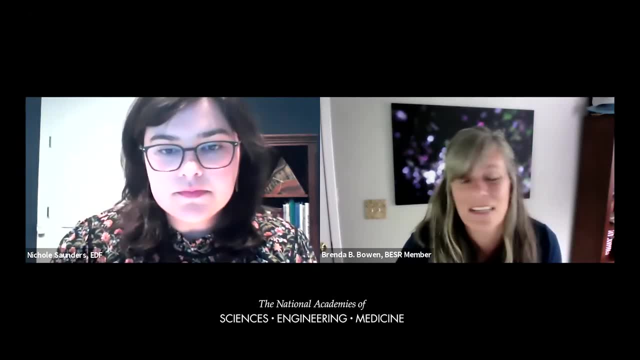 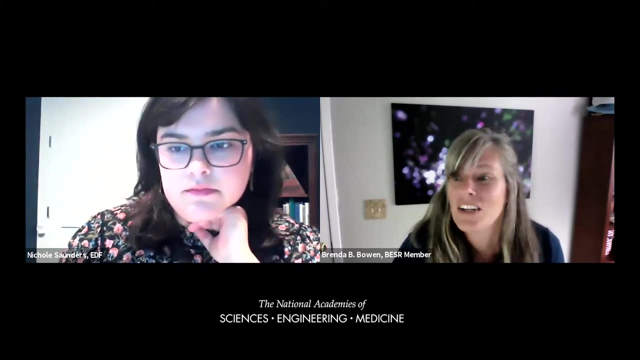 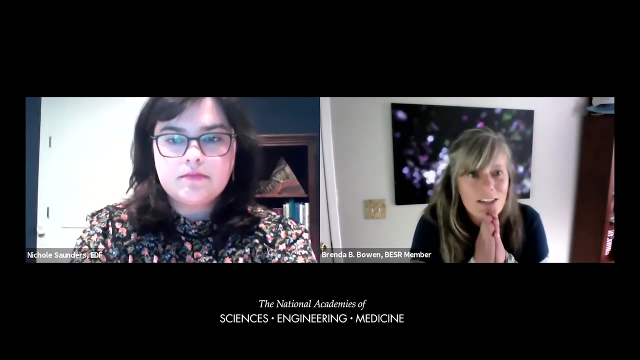 members with questions. We just have a couple of minutes for questions here to please raise your hand And, while you're thinking of those, just to get us going, if you had to choose a single direction for what you see as the highest research priority from sort of the earth science? 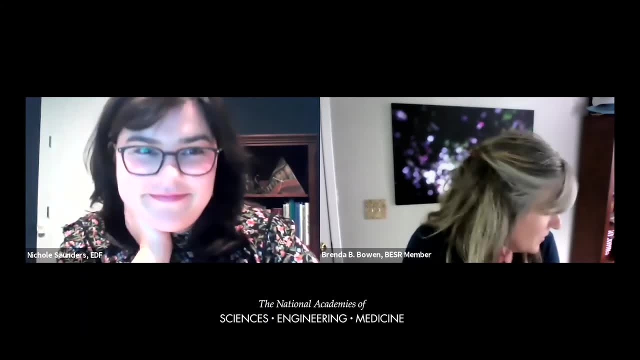 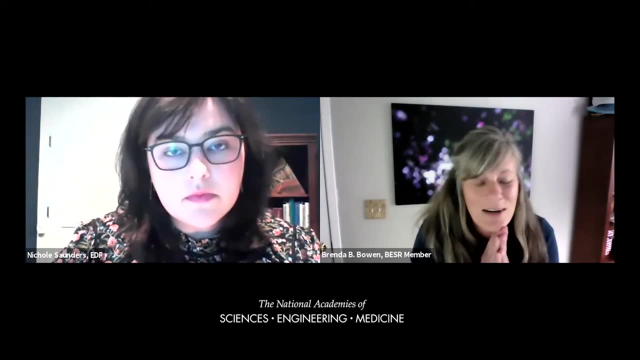 community to help advance where we need to go in kind of this legal framework to better utilize these produce waters. where would you say that that priority is from the science community? For the science community, I would say one of the biggest gaps right now is 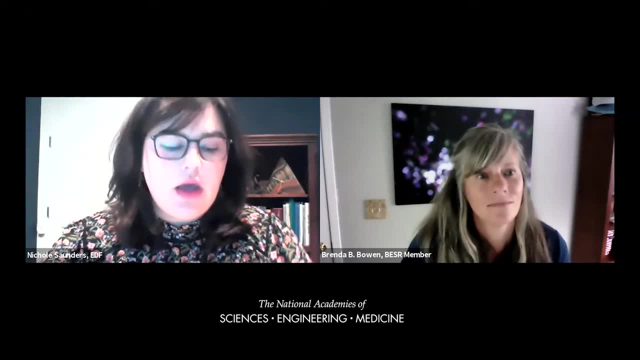 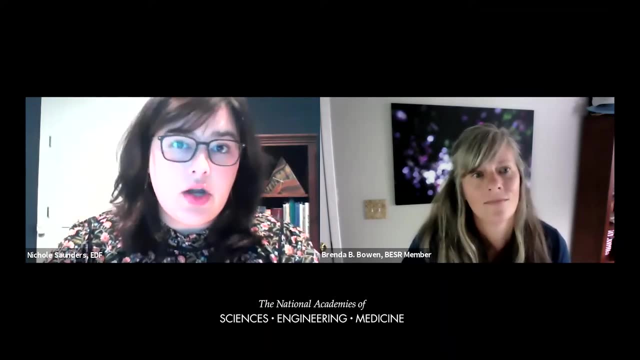 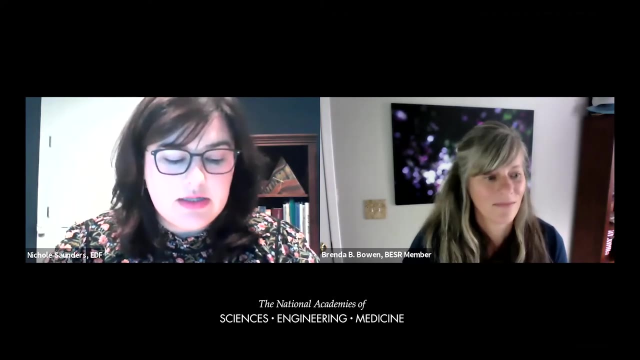 that land application component that I really couldn't get to. So, really diving into what the hazards are, what the exposure pathways are, how might we take what we know and don't know about produced water and think about the proper criteria or guidelines in a land application context? A good example in the 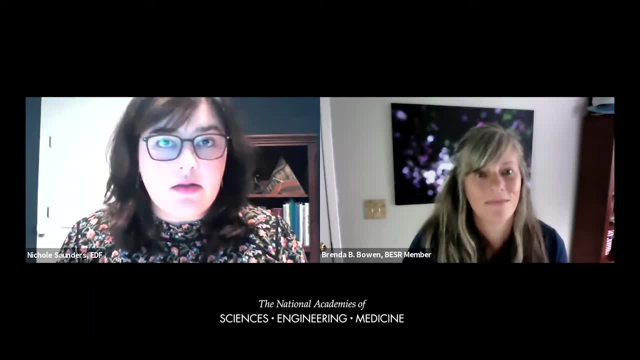 Clean Water Act context. we have the HoloFluent toxicity test or the wet test that can look at high throughput, comprehensive, like the complex mixture, and identify at least that there's a toxicity red flag. We don't have a fantastic equivalent for that in the land application. 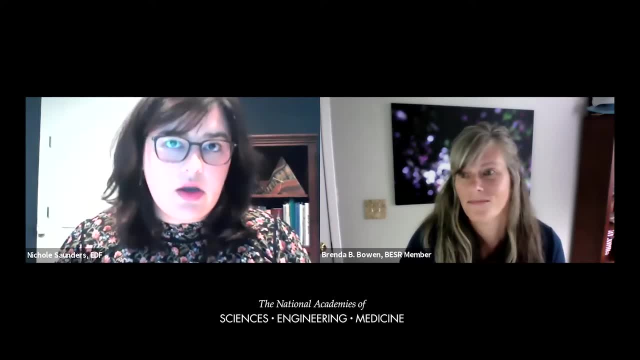 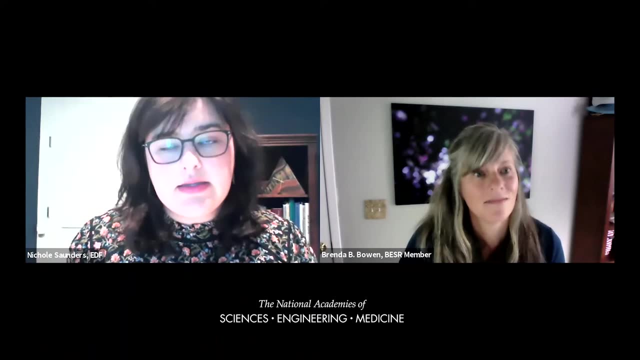 context. So there are some challenges in knowing what are the standards. what are we concerned about in produced water if we think about crop uptake, soil impacts, runoff wildlife or livestock consumption? Those are some questions that I think often fall through the cracks because we do focus. 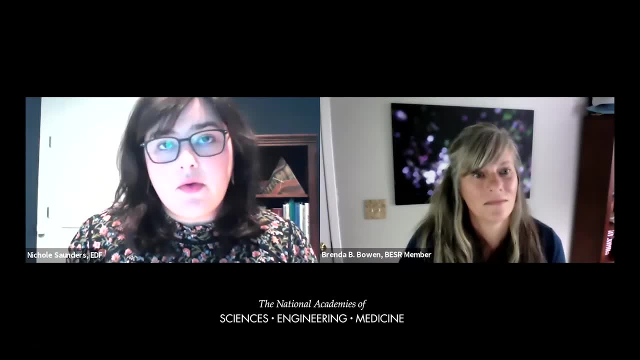 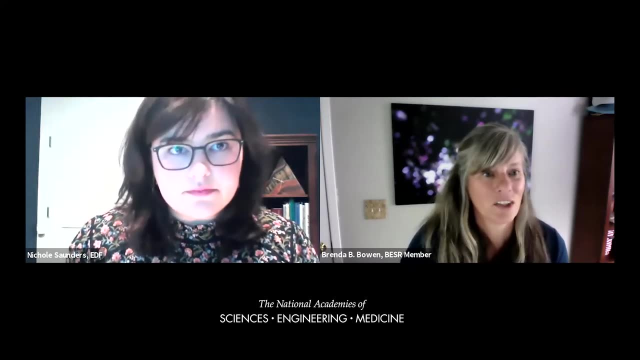 on the Clean Water Act side, It would be important if we're going to actually think about using this water in the land arena. Great, Thank you. Thank you so much, Nicole. All right, In the interest of staying on schedule, we're going to move. 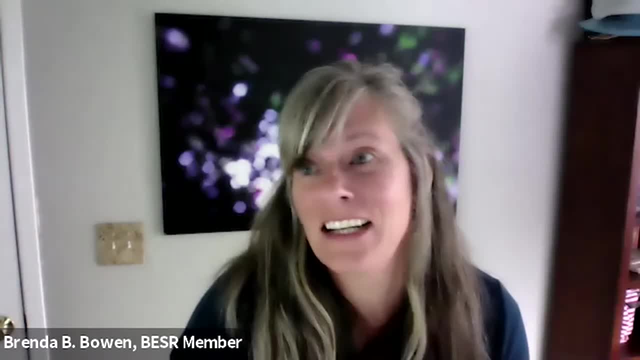 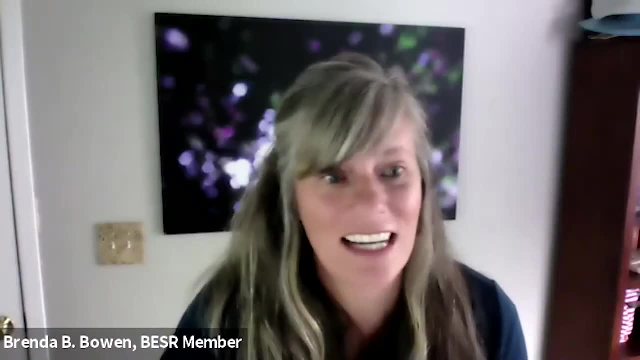 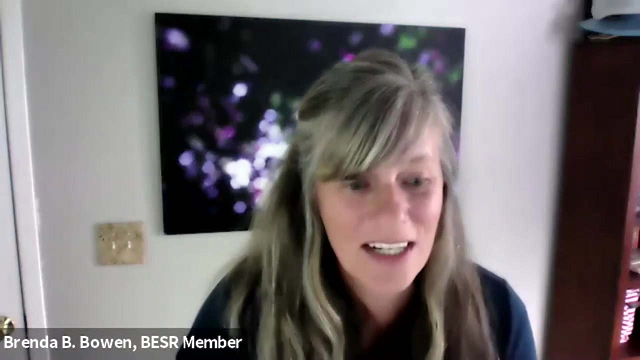 on Panelists, board members and audience members. as you have questions, do keep them in mind, as we'll come back to a full panel discussion after we hear from our three speakers, So we'll move on here. So next we will hear from Rebecca Hernandez. Rebecca is an assistant professor of earth system. 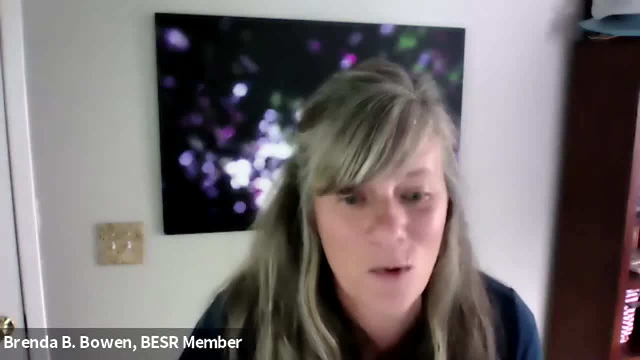 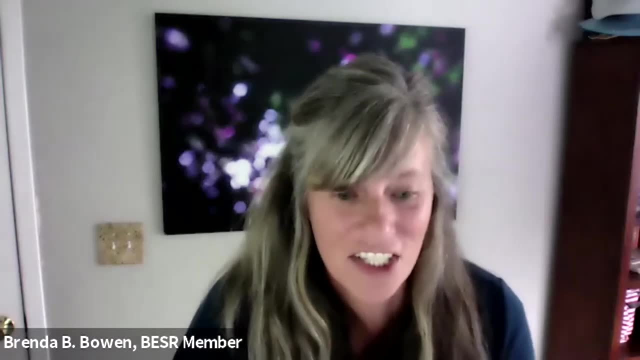 science and ecology in the Department of Agriculture. She's a professor at the Department of Land, Air and Water Resources and co-director of the Wild Energy Initiative at the University of California Davis. She directs field-based, data-intensive and technology-supported research. 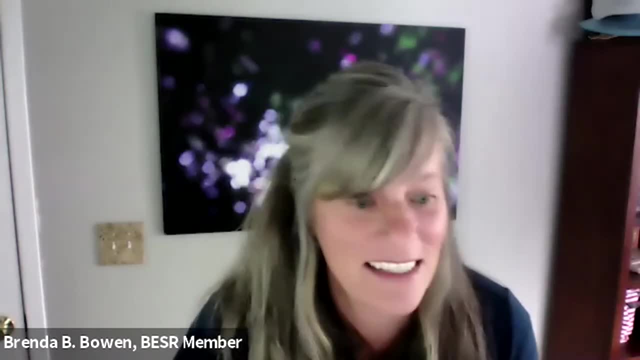 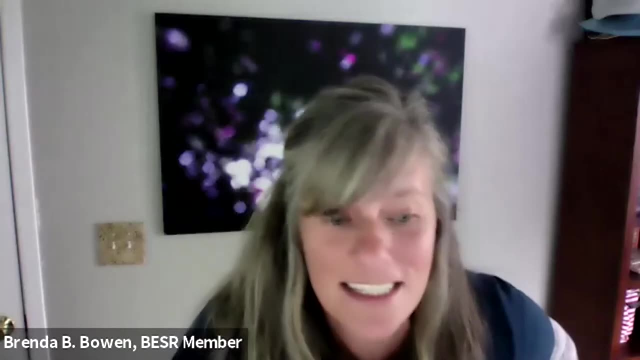 at the intersection of energy development and the environment. Her work on energy ecology has been featured in the Washington Post, National Geographic, NPR, Forbes and Scientific American. Rebecca, we're excited to have you here with us today and look forward to your presentation. 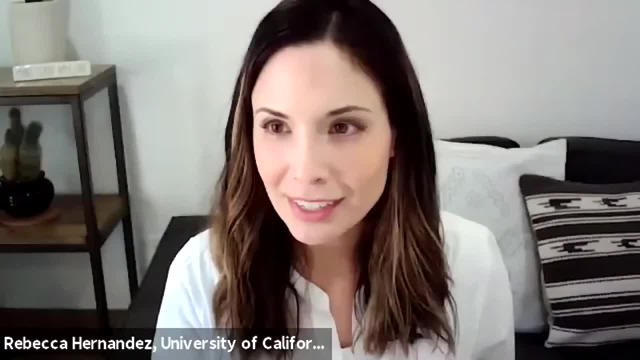 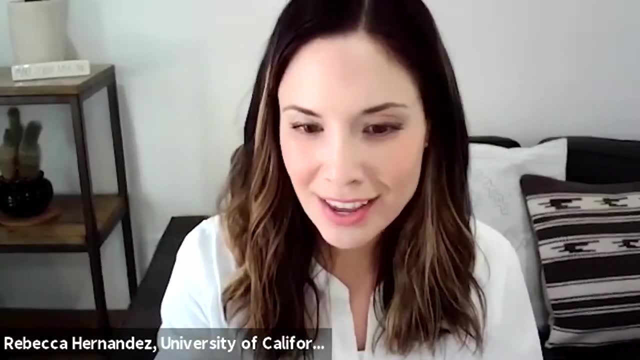 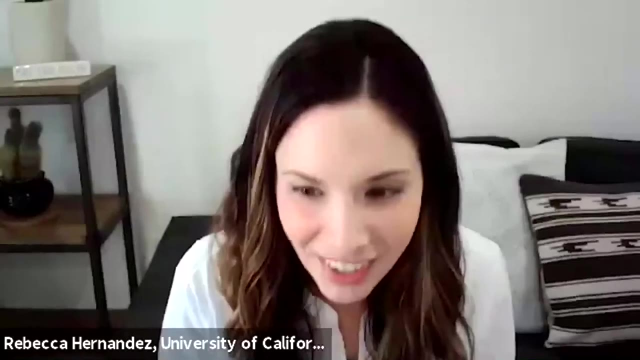 Thank you so much. I'm just setting up my slide deck. There we go. Can you all see that? Yes, looks good. Oops, Oh, we lost it. Oh no, Okay, one more time, Let's see. 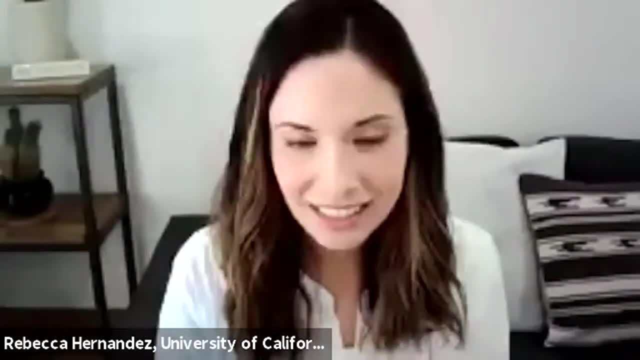 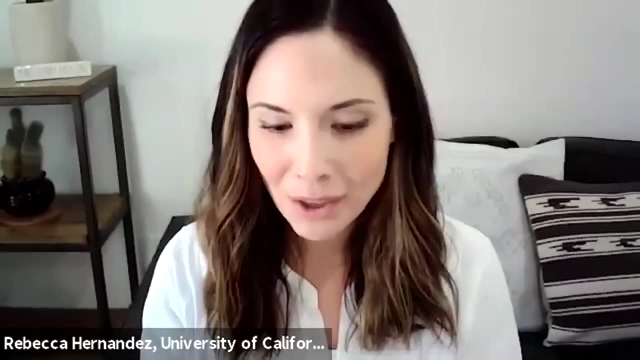 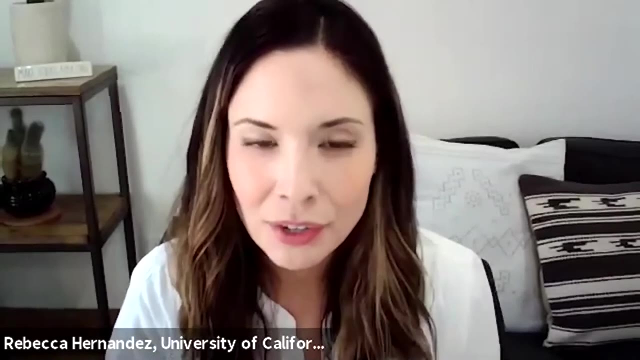 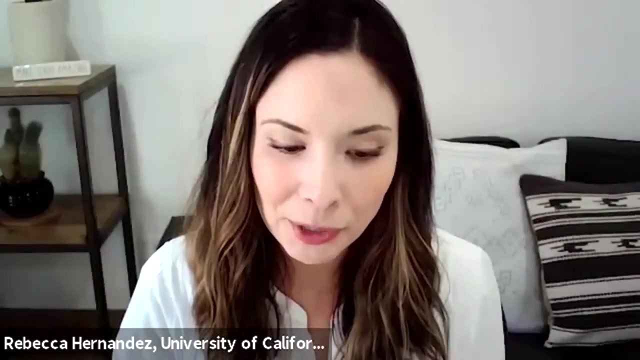 There we go. Okay, you can see that. Okay, you can see that. Yes, All right. Well, thank you so much to the Board on Earth Sciences and Resources for organizing this event and for your leadership on this topic. I'm just really pleased to be here. 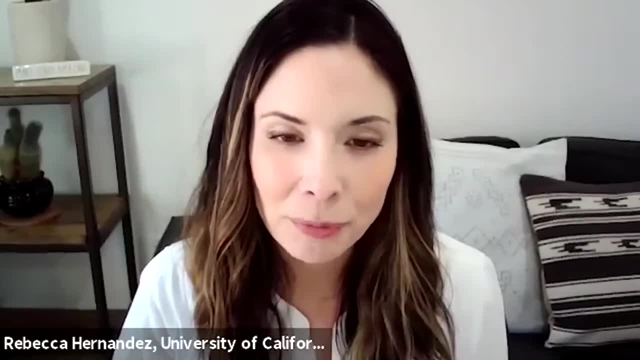 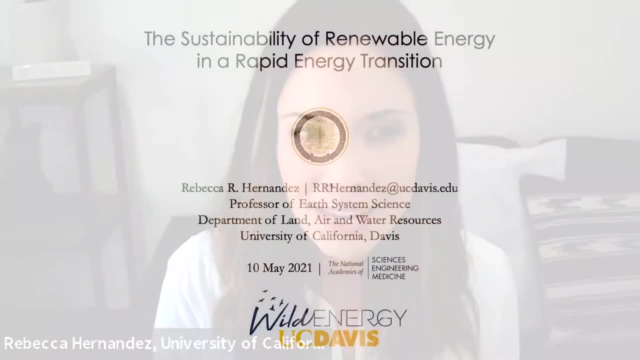 with you all. One question that I really enjoy asking my students at UC Davis is: how much land have you used today? And often I'm met with confused faces and a few hesitantly raised hands, and I typically follow this up by saying: 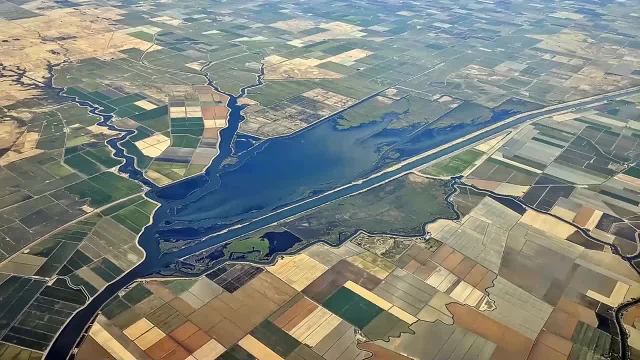 how many of you have turned on a light, a laptop or an iPhone? So many of us here today might know that turning on a light, a laptop or any appliance that uses fuel or electricity that uses land And, in fact, all energy supporting human activities, requires land. 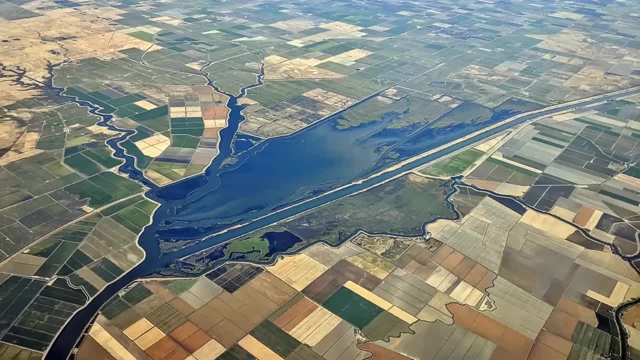 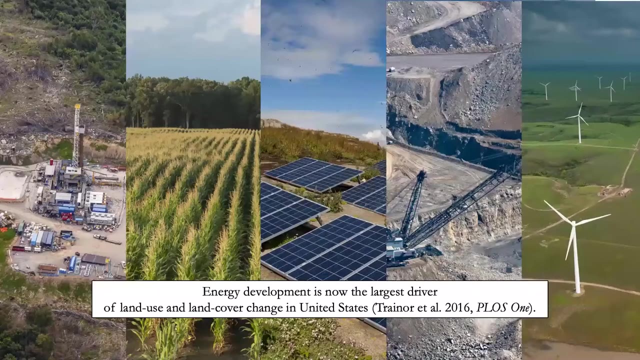 land, both directly and indirectly, But how much and to what end? Many of us here know that this is something to be true. So even in geographically large countries, this reality can and is becoming a problem of great ferment. So, for example, in the United States, energy development is now 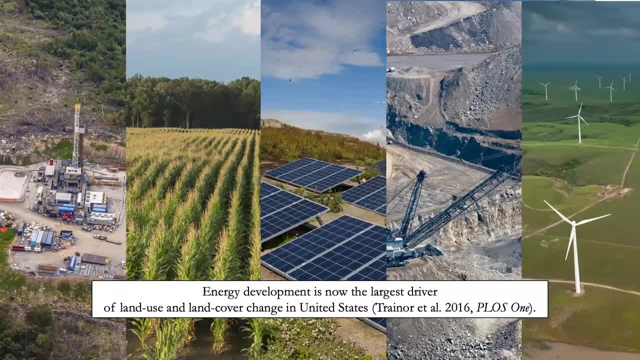 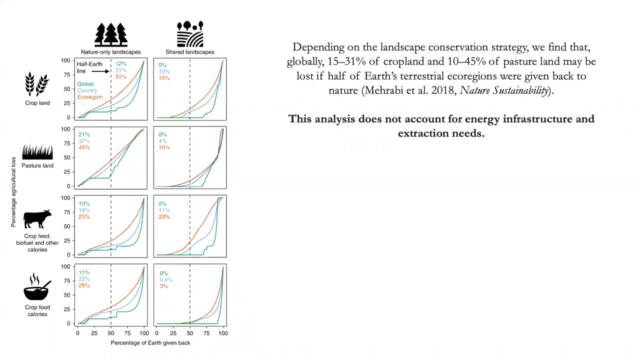 the largest driver of land use and land cover change. And here in the US, an area larger than the size of Texas, about 800,000 kilometers squared, is expected to be impacted by energy development and infrastructure by 2040.. So the need to account for land and ecosystem impacts. 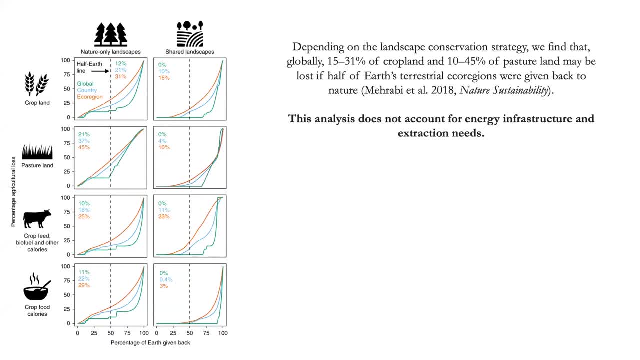 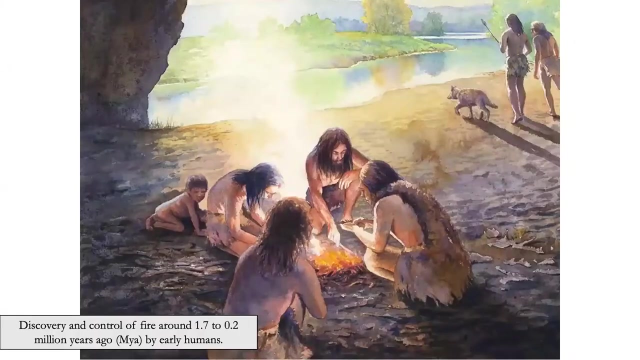 for energy becomes more probative amidst a global call by scientists like myself and conservation groups that we need to save half of Earth's ecosystems for nature, and where loss of crop, lands and pasture under such scenarios are really substantial. So how will we fit everything in Now? in the beginning, humans used wood. 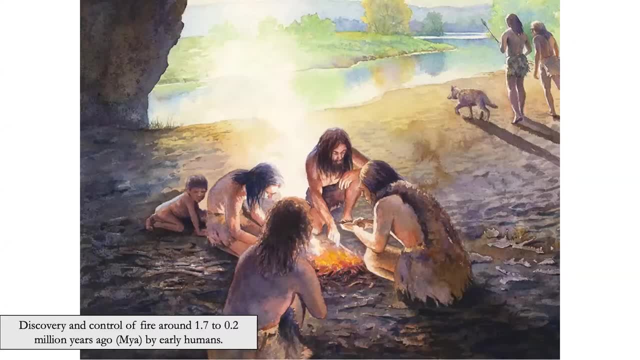 for energy right from the biosphere, These pre-industrial or organic economies. they relied on biomass That drove, deforestation and required large areas of tree plantations to support really small local energy demands for populations that were much smaller than today. Now the 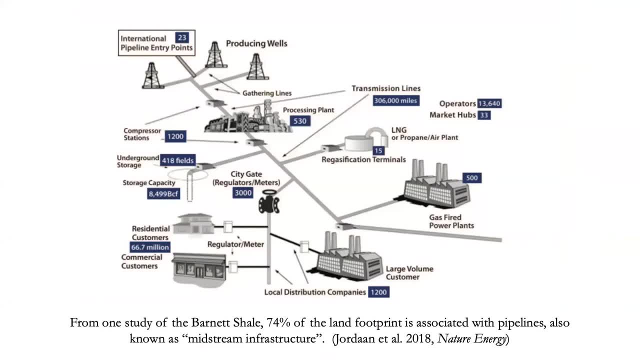 20th century was noteworthy for three transformations, all generating novel ecological impacts of energy on the planet Earth. First, in the rise of total energy consumption, which is an order of magnitude greater than pre-industrial times. Secondly, in the use of hydrocarbons, coal oil and natural gas for electricity. But 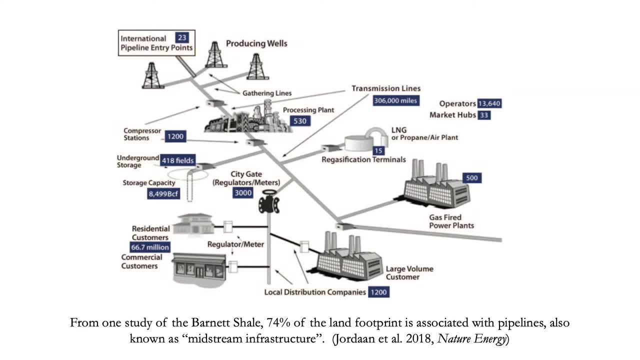 last and certainly not least, in a greater separation across landscapes from where energy was being generated to where it was being consumed. No longer were we restricted to the distance we could walk to carry firewood. We were no longer able to walk to the distance we could walk to carry firewood. We were no longer able to walk to the distance we could carry firewood. We were no longer able to walk to the distance we could carry firewood. We were no longer able to walk to the distance we could carry firewood Instead, we could. 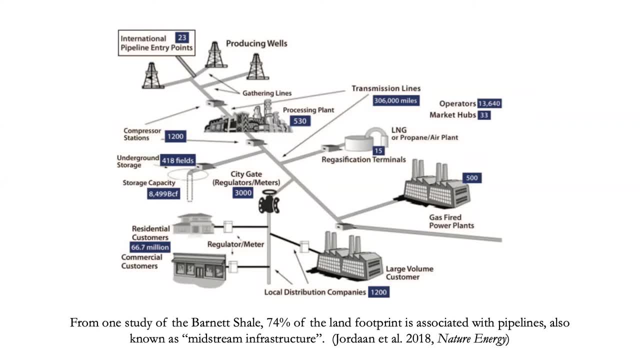 site energy infrastructure away from our viewsheds, often into marginalized minority as well as indigenous communities, And we could transport that energy as electricity along extensive transmission lines And this is what I've defined as what's called outsiding, And you can read about that in a study on local energy in front of disability. 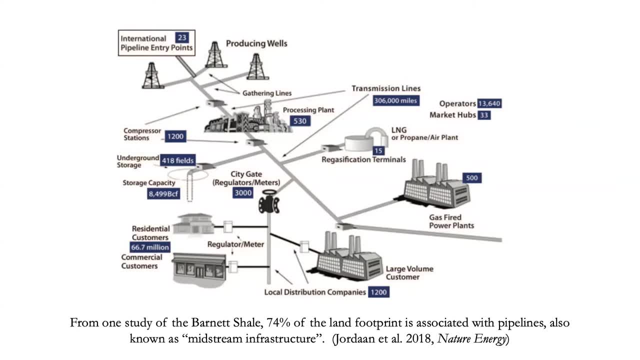 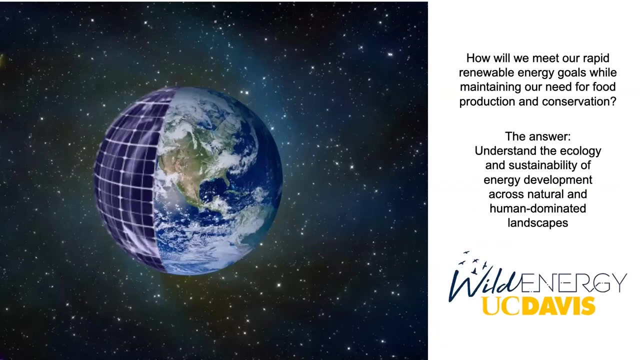 But for the first time impacts of energy on land. they really manifested in these direct, indirect and latent modes along these very expansive and intractable supply chains. So in my group a motivating question for our research is: how will we meet our rapid renewable 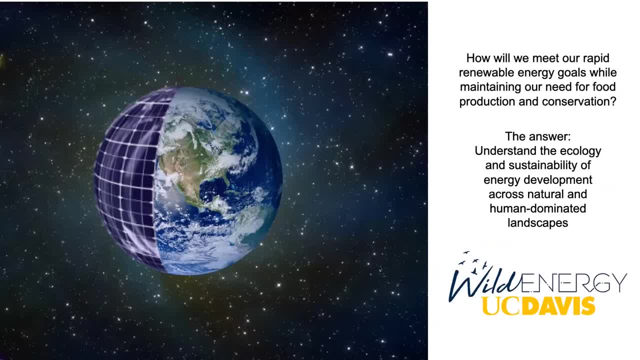 energy goals. Speaker. 1. for conservation and food production. And although we study diverse energy technologies, we often use solar energy as a model energy type to study these relationships because it dwarfs the potential of other renewable energy technologies, including wind and biomass. 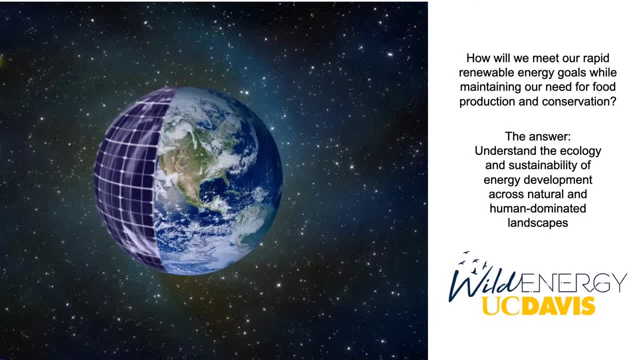 by several orders of magnitude, And it's so modular and cosmopolitan in its accessibility. Irina's remap case shows that PV may grow over the next 10 years, reaching a cumulative capacity of approximately 3,000 gigawatts by 2030, and almost 9,000 gigawatts by 2050.. So this is. 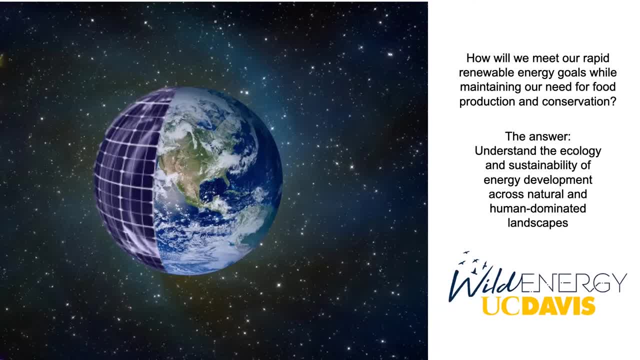 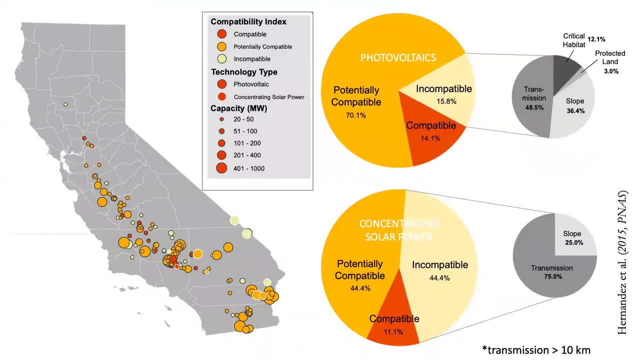 18 times higher than installed capacity in 2018.. So in 2015, we developed the Carnegie Energy Energy System, or the Carnegie Energy System or the Carnegie Energy System- Environmental compatibility model. This is a satellite-based decision support tool. 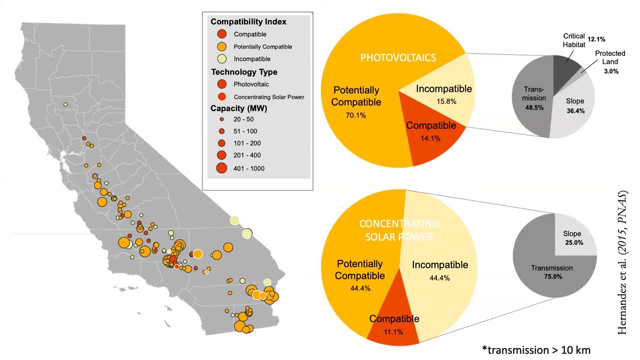 And we use this tool to evaluate how well we are citing ground-mounted utility-scale solar energy, specifically installations greater than 20 megawatts. So these are super big installations And we focused on the state of California in the United States, which has really been at the vanguard of global development for 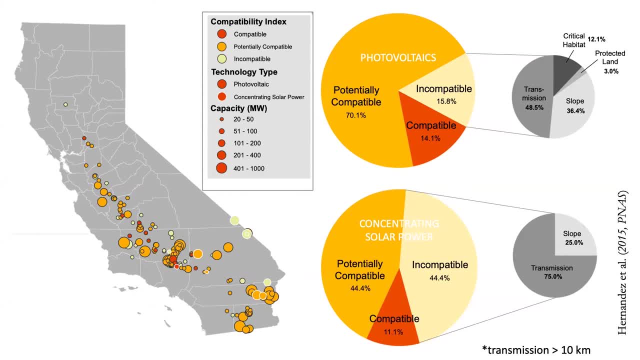 several decades Now. the map on the left that you can see here. this shows all solar energy installations, colored according to their sustainability index and sized by capacity, And we used a three-tiered ranking for power plant sites. So compatible, potentially compatible. 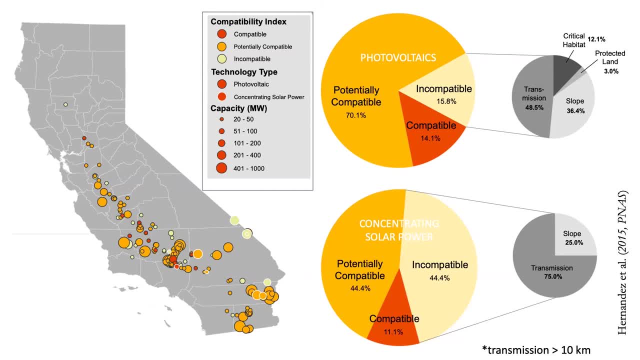 and incompatible. Now if you look at the pie charts, you can see that we found that less than 15% of PV and CSP installations were cited incompatible areas And many were cited in incompatible areas owing in large part to extended distances to existing transmission, And some were marked 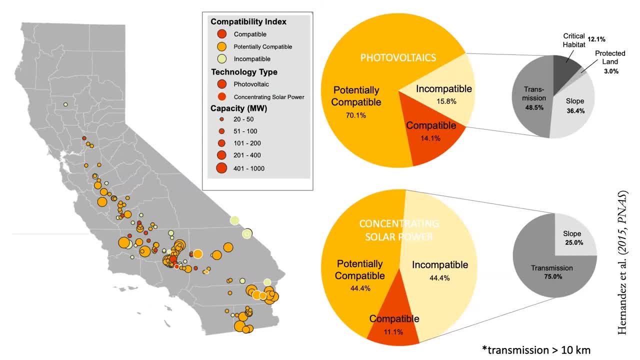 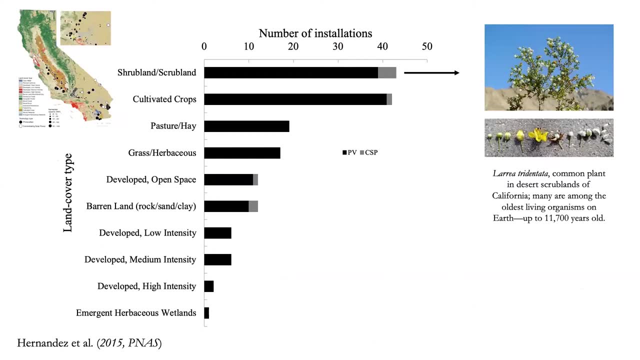 as incompatible because they were cited in areas of endangered and threatened species habitat. So we also explored the siting of these installations by land cover type And we found that PV-powered solar energy installations were more compatible with land cover type installations. So that's really what we found, And in the report on the left I also showed a. 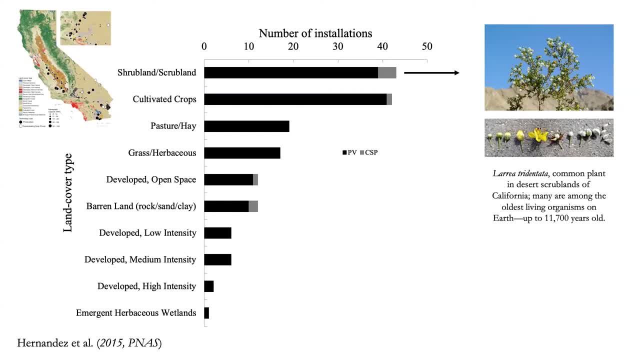 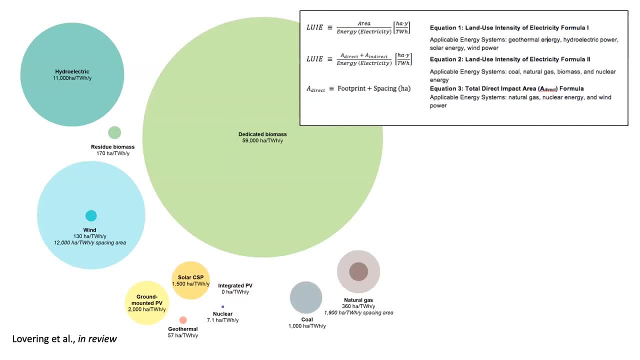 couple of versions of the results of these investigations. And we also found that just in the 50 to 60% of the PV-powered solar energy installations, the very largest and the least the impact of energy on land across all major electricity sources And to date all of them have had. 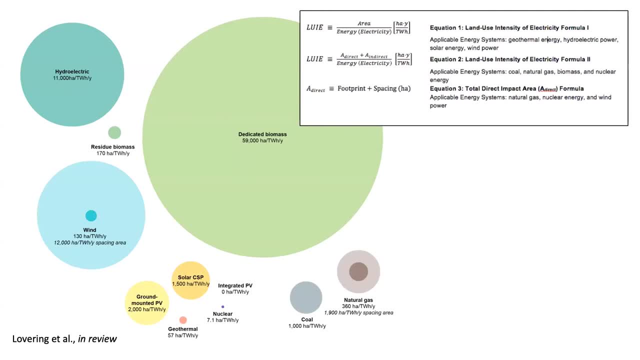 some methodological limitations or weaknesses. So here, in work led by Dr Jessica Levering, we calculated the land use intensity of energy for real world sites across all major sources of electricity, integrating data from published literature, databases and original digitizing and data calculation. 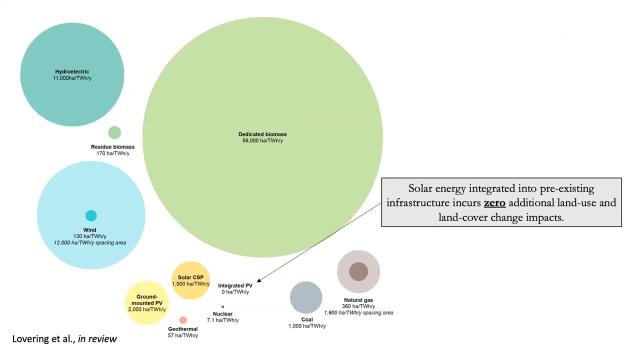 And this is what we found. We found that ground mounted solar energy, including both concentrating solar power and photovoltaics. this is an order of magnitude lower than hydro and dedicated biomass, but requires more land than coal, natural gas, residue biomass, wind, geothermal and nuclear. 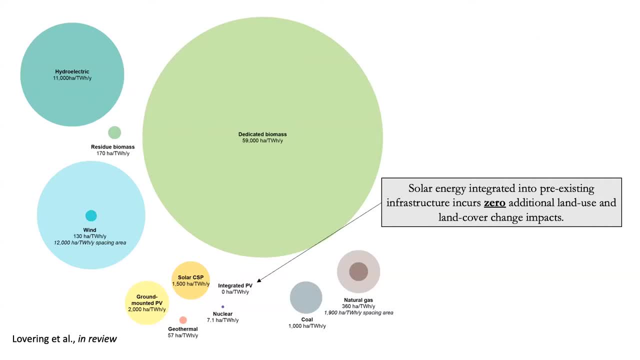 But in terms of land use and land cover change: solar energy integrated into pre-existing infrastructure. this is our one free pass, or free lunch as we could call it. This incurs zero additional land use and land cover change impacts, And our work in our lab is currently focusing. 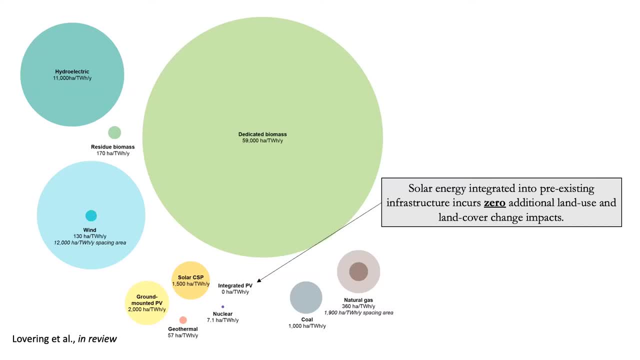 on calculating opportunities within the commercial building stocks to serve as recipient environments For solar energy, especially large commercial buildings. So our preliminary results have revealed that the 30 largest commercial buildings in the US embody rooftop footprints that average about 275,000 kilometers. 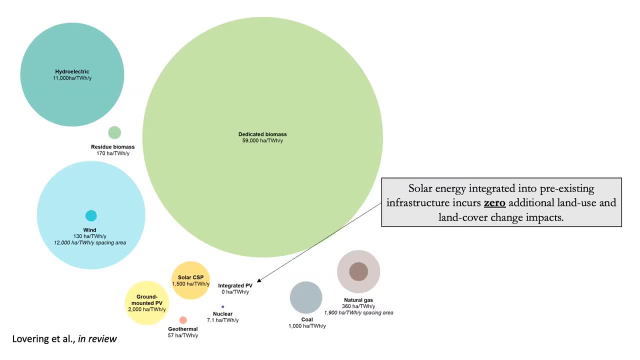 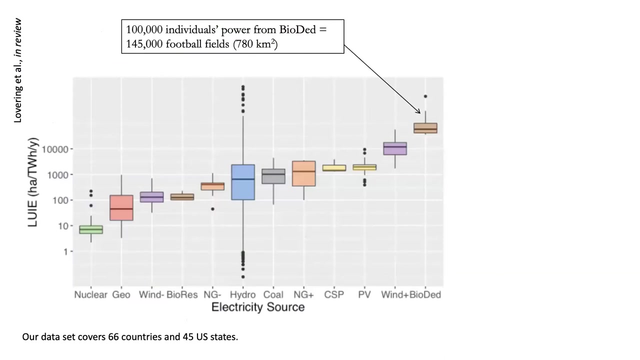 sorry, 275,000 meters squared, And this is an area that is equivalent to approximately 50 American football fields. These are very large buildings. Now one more thing. this is that same data on a log scale, And I wanna point out to put dedicated biomass into context. powering an average US city of about 100,000 individuals for one year. I would require about 78,000 hectares with dedicated biomass, So this is about 145,000 football fields, which might make us all feel a little bit uncomfortable. 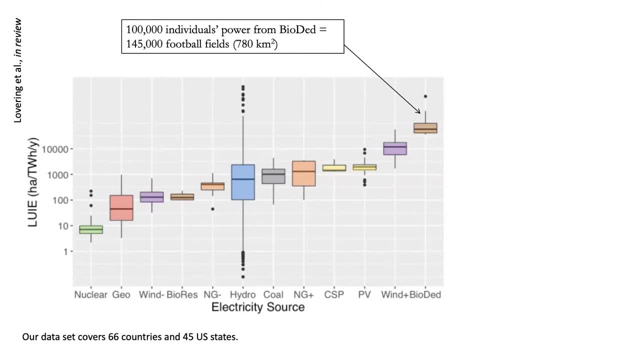 You're right. You can remember from Brian's slide that large green bioenergy wedge for achieving cumulative CO2 savings And indeed most global decarbonization pathways now emphasize dedicated biomass, some for which biomass is greater than all other sources combined. 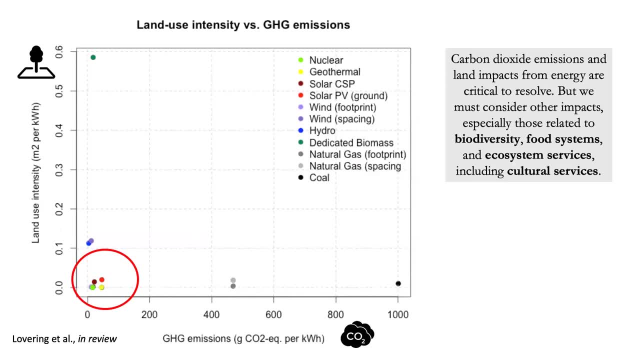 But using these data, we can then consider both the environmental impacts from direct emissions and from land together And this really confers a more comprehensive comparison of total environmental impacts. So that area encircled in red here on your slide, this is really the sweet spot. 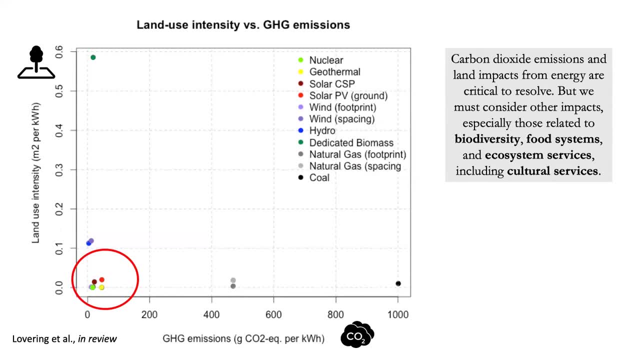 geothermal, nuclear, solar and wind, in that these sources of energy are optimized in terms of their CO2 emissions and impacts on land. But we need to consider other impacts too right, Especially those impacting biodiversity and ecosystem services, Even cultural services. 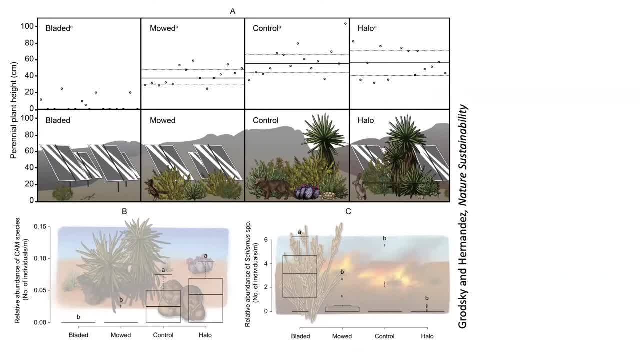 In California. my work shows that deserts are prioritized right as recipient environments for solar energy development. But deserts globally embody these longstanding ecological, economic and cultural resources for humans and especially to indigenous land rights holders. Here my colleague Dr Steven Grodzki and I 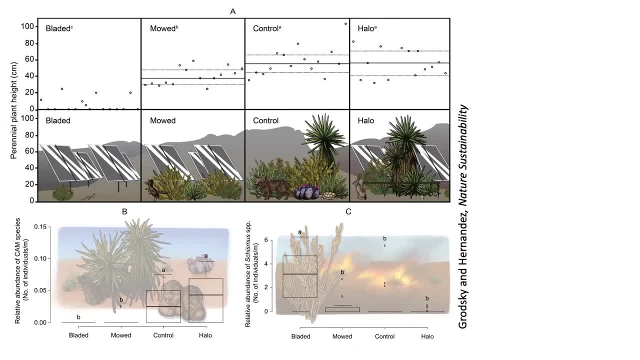 we measured the effect of solar energy development decisions on desert plants at one of the world's largest concentrating solar power plants in Ivanpah, California, And we found negative effects of solar energy on this desert scrub plant community. Specifically, we found that perennial plant cover 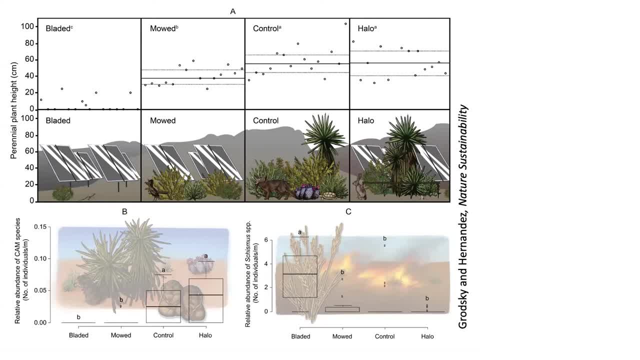 and structure were lower in the bladed treatments- which is often what happens with these power plants- than in the mowed treatments, And we determined that cacti species and Mojave yucca are particularly vulnerable to solar energy development. that is, blading and mowing. 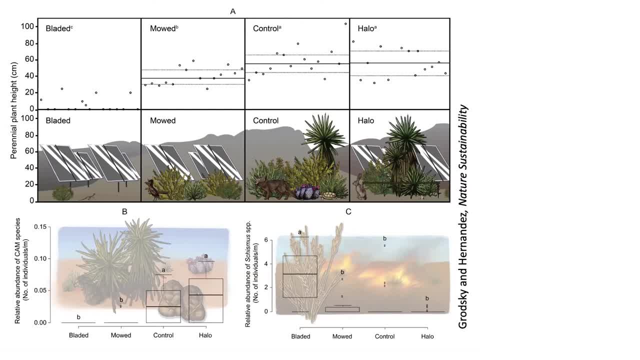 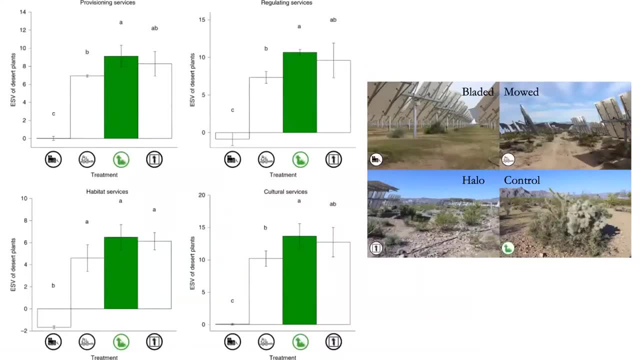 Whereas schismas, which is an invasive annual grass that often promotes desert fires, is facilitated by blading. We're also interested in elucidating impacts of solar energy development decisions in this system on ecosystem services. So here we found the desert scrub plant community. 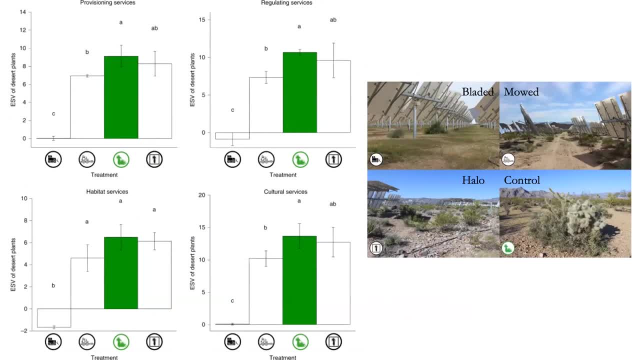 confers 188 instances of ecosystem services, including carbon sequestration and pollination, and cultural services like sense of place and indigenous tools to 18 Native American ethnic groups, And we found that bladed and mowing treatments reduced cultural provisioning and regulating ecosystem services of desert plants. 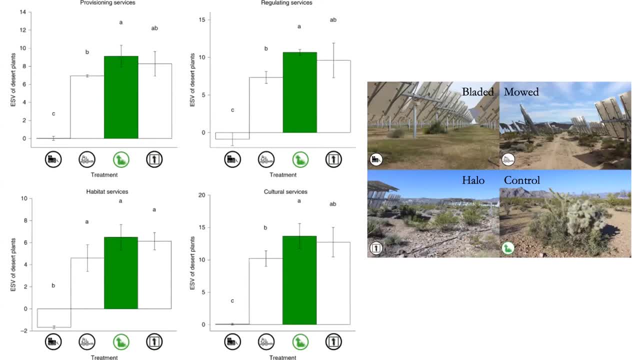 compared to the undeveloped control. So overall it demonstrates the potential for ground-mounted solar energy development in deserts to reduce biodiversity and socio-ecological services and emphasizes resources. sorry, but it also emphasizes the value of integrating renewable energy infrastructure locally. 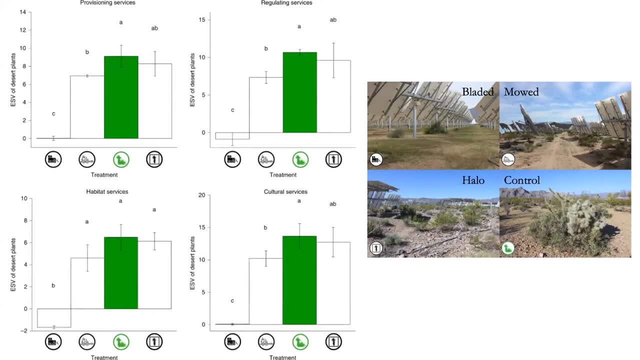 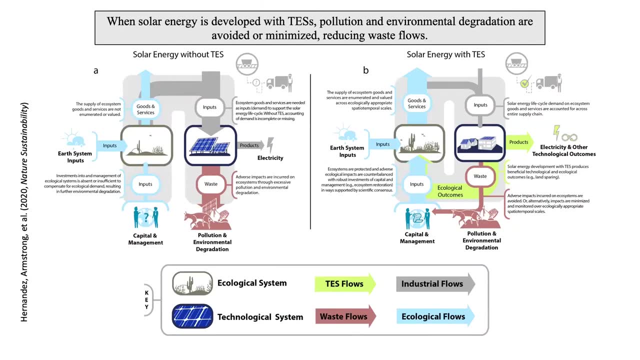 and into the built environment. Now moving forward, my colleagues and I have proposed a new model, and one that builds upon the excellent work of Dr Bakshi at Ohio State University for engineering solar energy systems and renewable energy systems broadly, in a way that maximizes both technological 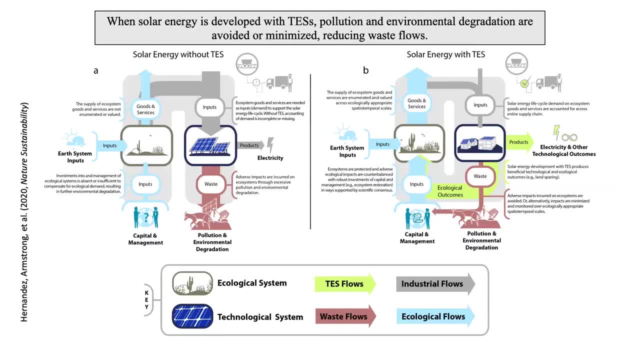 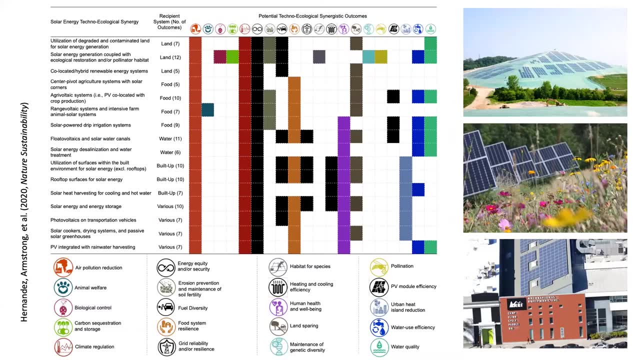 and ecological benefits. So we identified over 15 different types of these installations that can be developed, known as techno-ecological synergies of solar energy, And this includes installations over land, over water and, importantly, in cities, even within agriculture, agricultural areas. 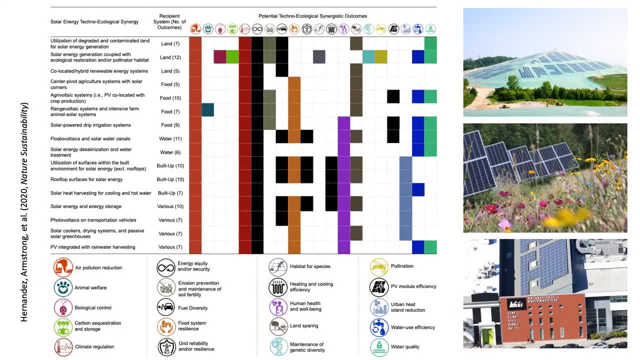 And all of these produce about. we found 20 unique beneficial techno-ecological outcomes from this type of engineering and design. So examples include the utilization of contaminated land for solar energy generation. That can include land related to areas formerly mined for coal. 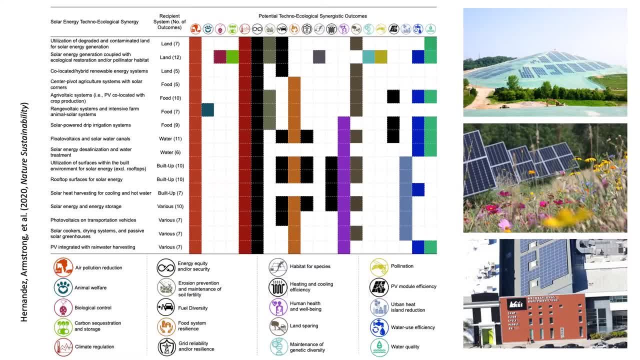 For example, agrivoltaics, rangevoltaics, floatovoltaics, solar energy, coupled with uh ecosystem restoration and pollinator habitat. Rob Davis with Fresh Energy is really making huge gains on that opportunity in the US And our attention in our lab has really turned. 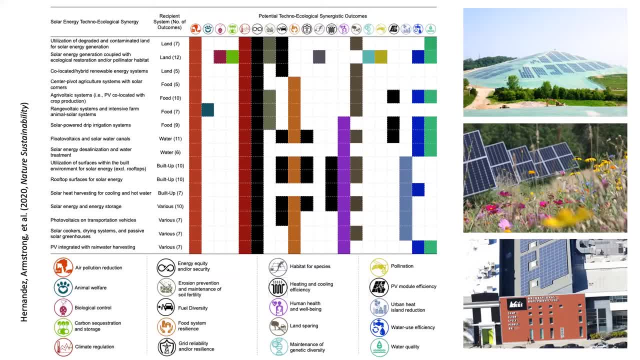 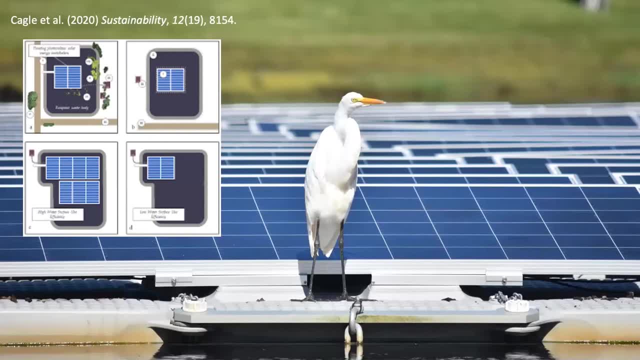 to these novel applications and quantifying the net technological and ecological outcomes of these opportunities. For example, we're conducting a foresight synchronized study of floating solar energy. We're studying relationships between floating solar and PV performance, biodiversity and hydrology, um including water impacts. 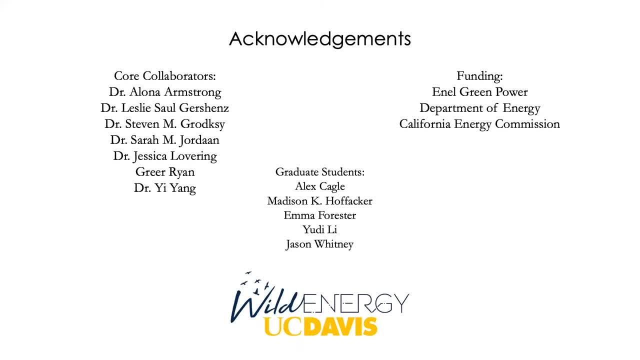 Thank you so much for your time and attention. I'd like to thank my collaborators and my, my graduate students and my funders, without which, uh, none of this would be realized. Thank you so much, Rebecca. Really fascinating to think about all these connections. 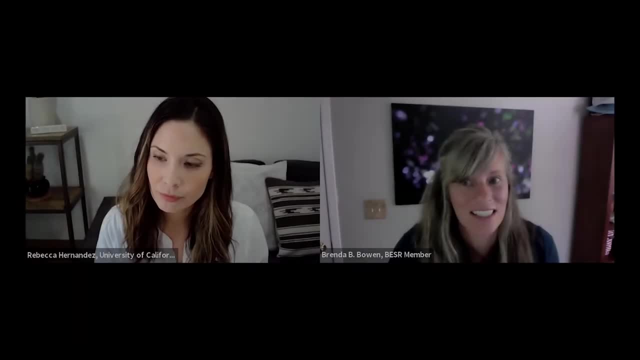 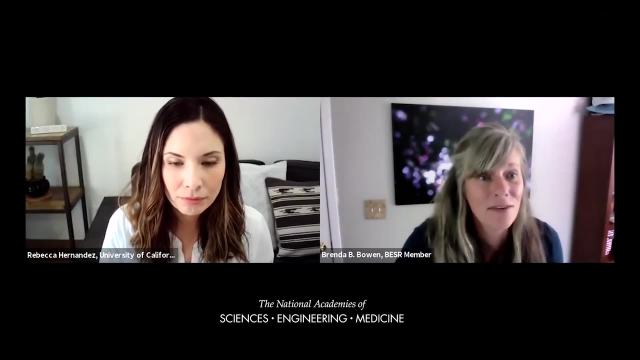 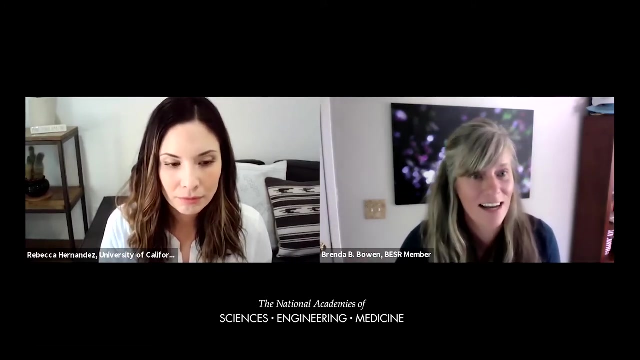 around land use and ecological change as we imagine This transition towards ramping up renewables. So appreciate that And, um, we'll invite folks to note their questions so that we can come back to them for our, for our full panel discussion after we hear our next. 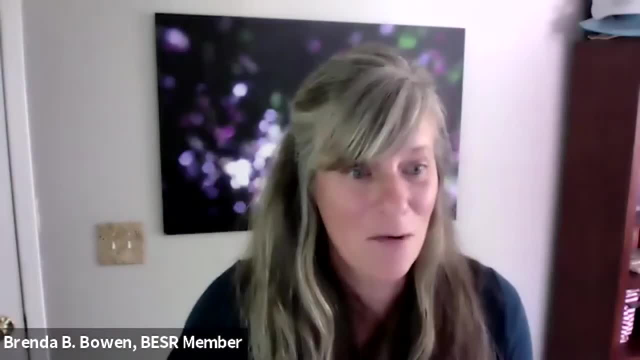 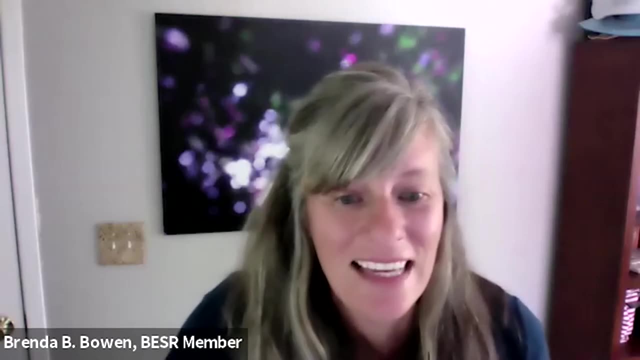 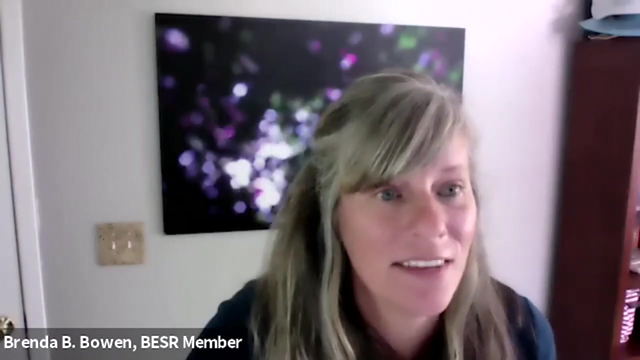 and final speaker. So with that I will go ahead and introduce our our last speaker of the panel, um, Benjamin Holton. Ben is the Dean of the College of Agriculture and Life Science. He's a Cornell university professor in the department of 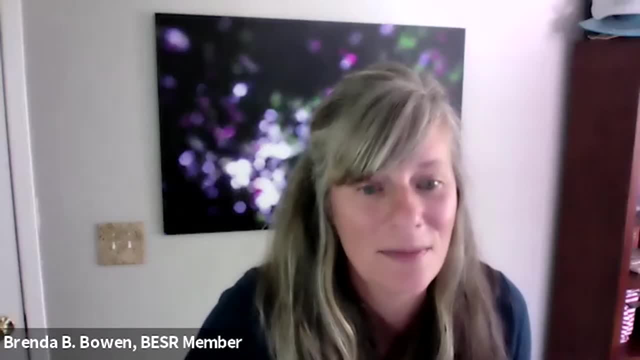 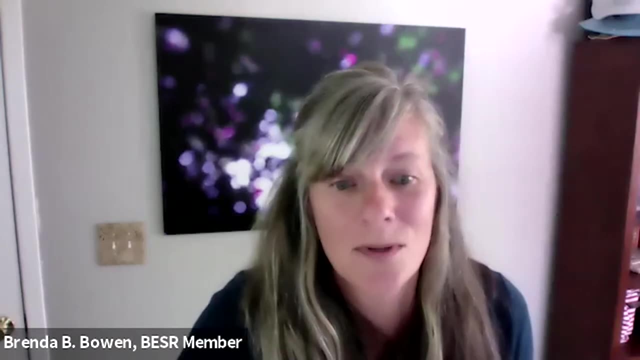 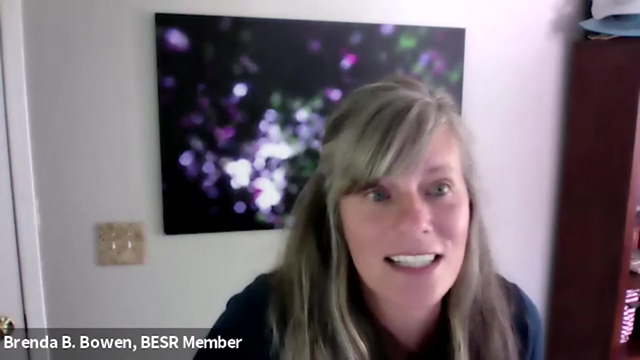 ecology and evolutionary biology, and of global development. Ben is the founding co-chair of the California collaborative for climate change solutions, which works with researchers from key research institutions to accelerate the translation of research findings into practical climate solutions. He also directs over a hundred acres of farmland carbon. 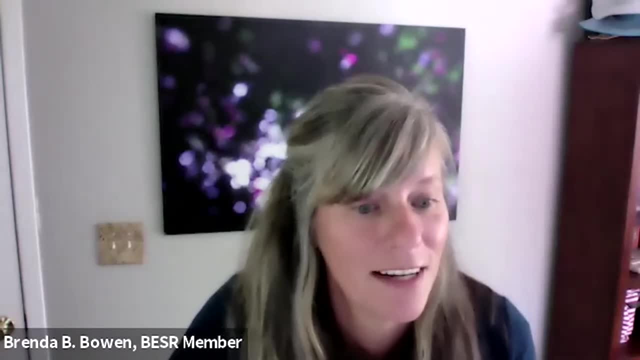 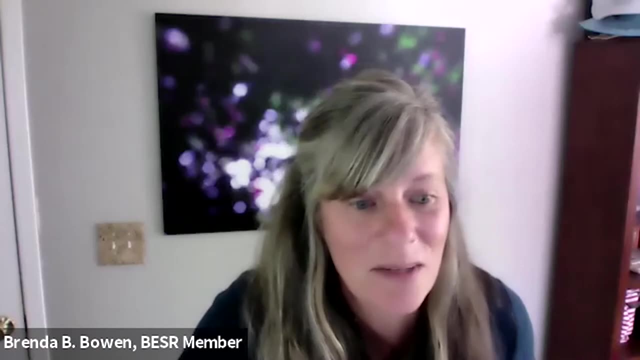 sequestration projects to improve crop yields and create new financial markets For farmers and researchers. unfortunately, Ben uh had an emergency today and is not able to be with us in person. However, he recorded his talk, which we will play. 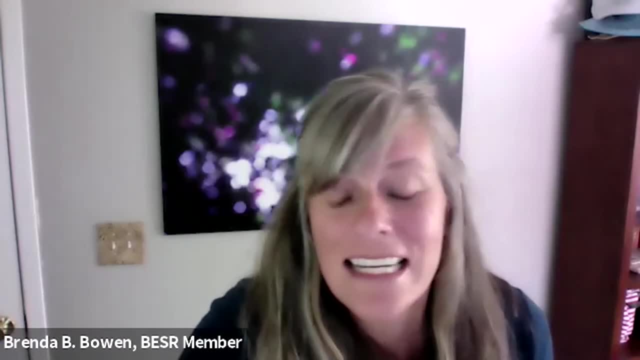 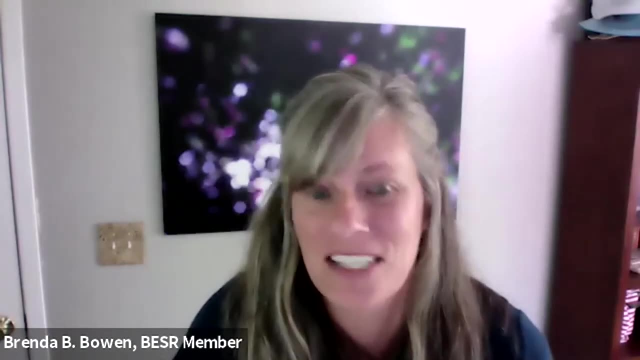 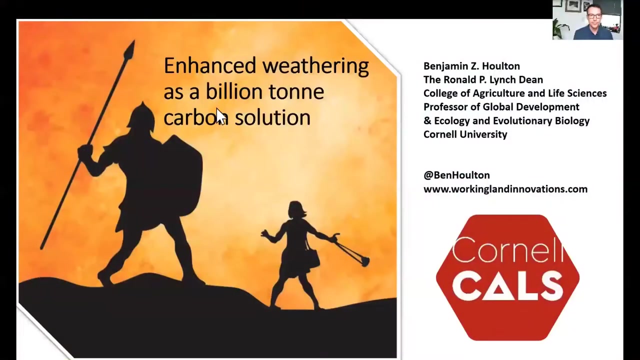 Now um Garrett, who, to know one of his team members, uh, is joined us here today and we'll join for the panel discussion after our break, following Ben's presentation, So we will now show his recorded talk. Thank you so much for this opportunity to. 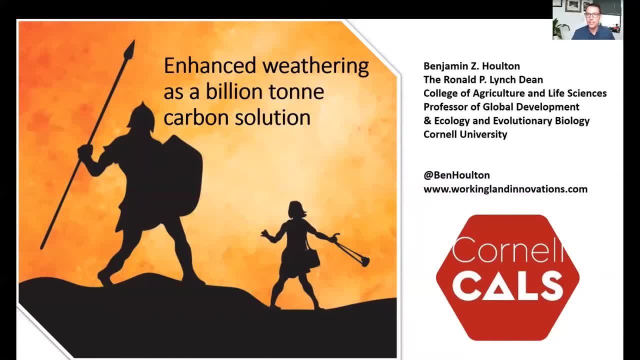 present to you today. I am Ben Holton, the Ronald P Lynch Dean of the college of agriculture and life sciences and a professor of global development and ecology and evolutionary biology at Cornell university. apologies that I can't be there in person. Uh, luckily my research associate, Dr 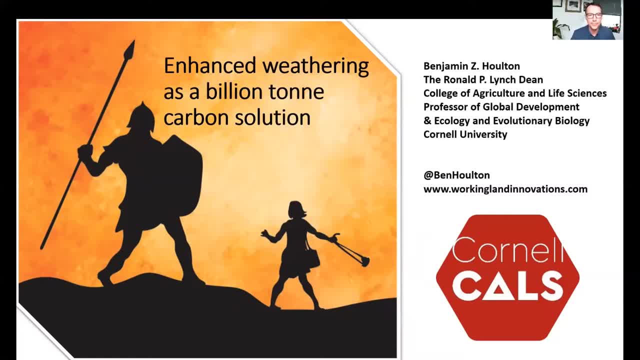 Garrett Bono will be available for the Q and a. I'm going to briefly overview this idea of enhanced weathering, the notion of grinding up rock, applying It to the soil and having that rock break down so that it creates carbonates that securely lock carbon, extracting it from 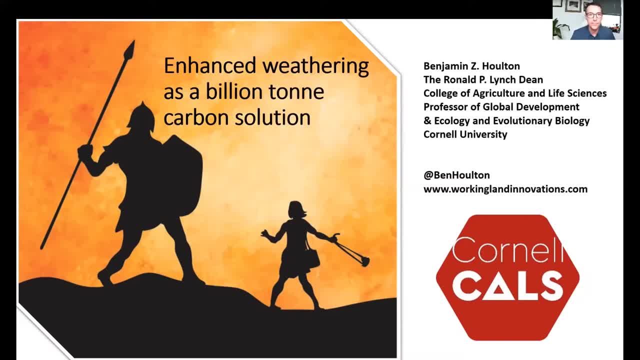 the atmosphere into a form that no longer causes dangerous climate interference. There is a lot of discussion today about enhanced weathering as a possible billion ton level solution, but that capacity and the gap to the science and deployment is very significant, And so what I want to talk to you today is first the idea of 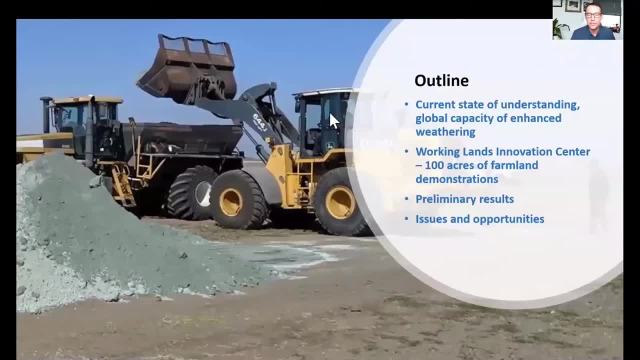 enhanced weathering as a solution to atmospheric CO2 accumulation, including the global capacity for this pathway to operate in agriculture. I will then discuss results from the working land innovation center that I direct with my colleague Dr Wendy silver at UC Berkeley, where we are deploying this technology across more than 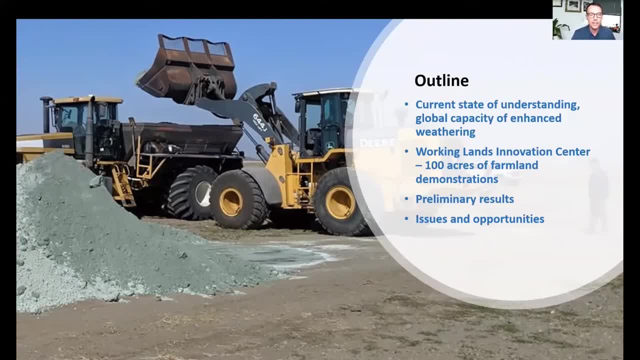 100 acres Of farmland in California, And that includes diverse cropping systems in range lands. I will present some preliminary results from the first year of our study in the working lands innovation center, And then we'll talk briefly about issues and opportunities. 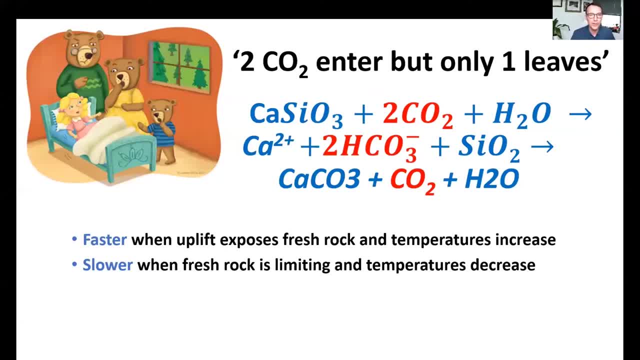 So, taking the big picture perspective, we all know about earth's Goldilocks and the fact that our planet maintains life because of, first, it's distance from the sun being just right. but on top of the earth's Goldilocks and the fact that we have this orientation to the sun, there are incredible feedbacks between 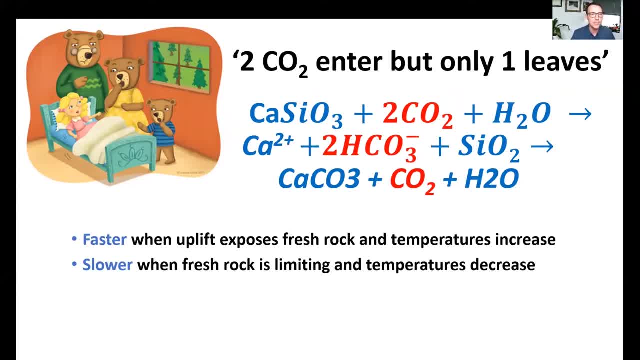 atmospheric to and climate that result in stabilization over time, so that the earth doesn't end up in a runaway greenhouse effect like Venus, or get too cold like Mars, and rather stays just right. The secret ingredient involves silicate rock weathering reactions which consume atmospheric. 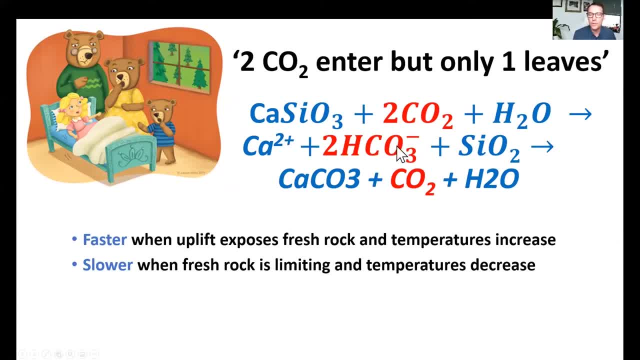 CO2, creating bicarbonate in dissolved form that eventually make their way and wash from the land into the ocean, forming calcium carbonate that can securely lock a mole of carbon dioxide from this initial reaction for millions and millions of years. This set of reactions, Known as the urea reactions, are faster when uplift exposes fresh rock and the temperature rises. 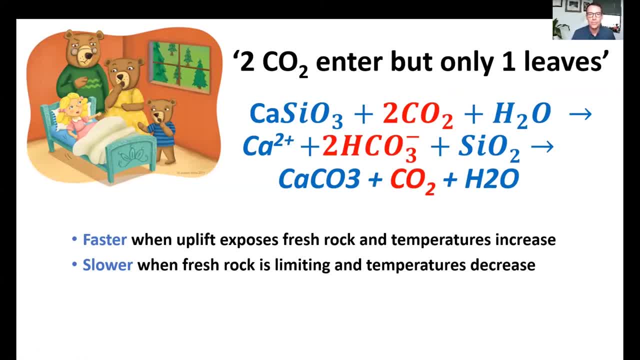 So, in other words, it gets hotter and CO2 rises. weathering happens more quickly, thereby acting as negative feedback on runaway climate change. It also is slower when there is less fresh rock exposed to earth's surface And, as temperature decreases, this allows for natural processes of CO2.. 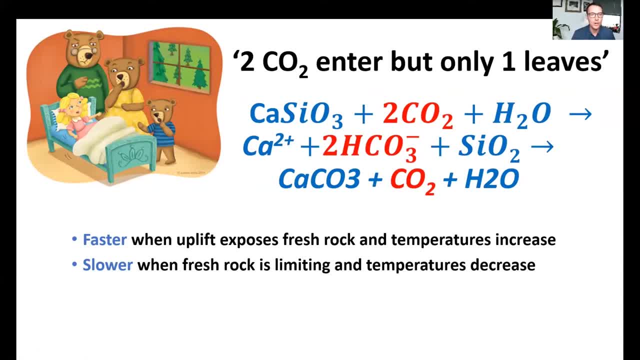 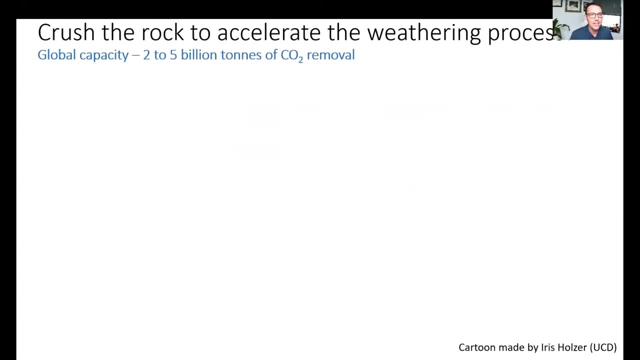 Ventilation from volcanoes to accumulate CO2 at a level that continues to allow for earth's temperature to experience a relatively stable condition. So the question of today is: can this kind of approach, this technology that the planet has invented and been operating for billions of years, be accelerated? 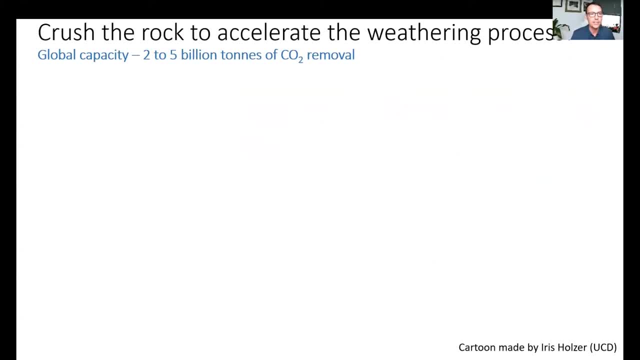 Well, of course there is potential for accelerating this process. Well, of course there is potential for accelerating this process. Well, of course there is potential for accelerating this process. One of the ideas is to take, finally, crushed rocks that are a byproduct of the mining. 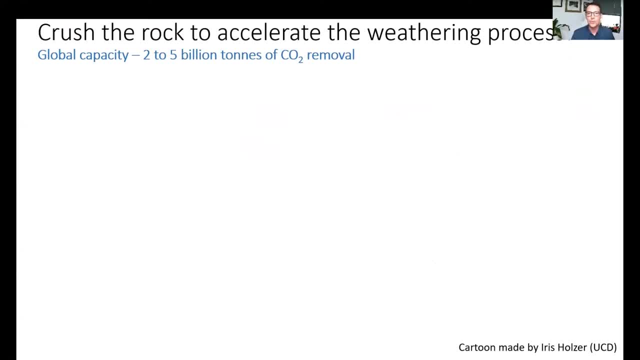 industry and apply them to croupling soils to greatly accelerate what is normally a relatively slow process over time. Current models suggest that anywhere within reason enhanced weathering, if applied this way, could get you to 2 to 5 billion tons of CO2 removal on earth's surface. 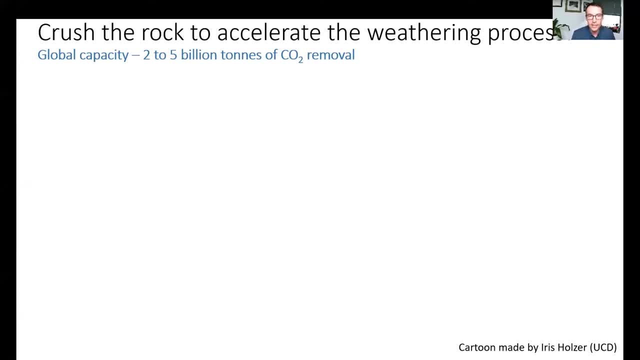 Rob Lemansky croplands. but again, the gap between that capacity in deployment is extremely significant. so just to go through in a cartoon formula what we're talking about here, we take crushed rock, Rob Lemansky, That is enriched in calcium and magnesium silicate. we apply it to the soil where there is CO2 that is being pumped up in the soil environment through respiration. 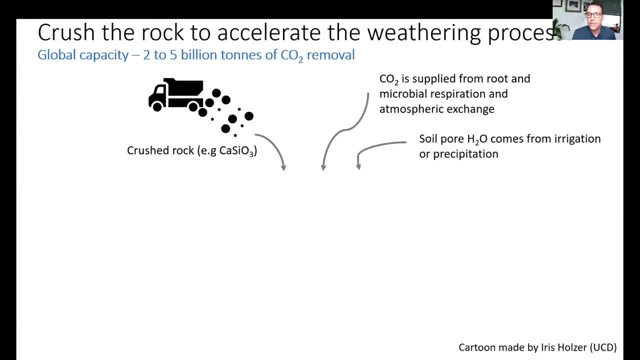 Rob Lemansky, From microbes and roots. the water from irrigation or precipitation comes in contact with that CO2 and it can form carbonic acid which dissolves the calcium silicate, Rob Lemansky, And that initially forms bicarbonate, calcium ions and some silica. so we get two moles of CO2 sequestered for this initial reaction sequence. 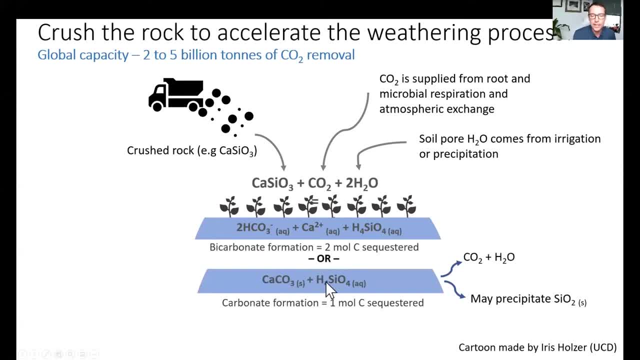 Rob Lemansky. However, if some of the calcium carbonate precipitates back out in the soil, you release one CO2 back to the air, Rob Lemansky, Meaning only one mole is sequestered. so in either. in either scenario, whether we form bicarbonate or carbonate, carbon dioxide is removed. 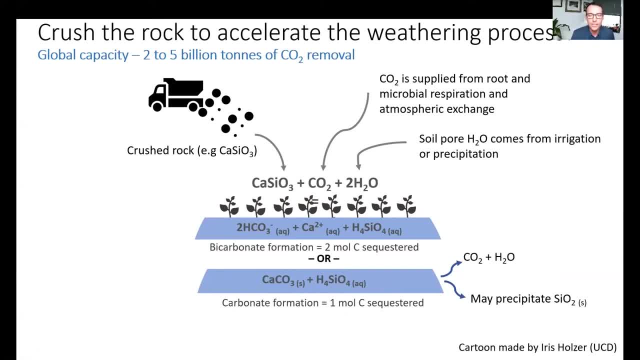 Rob Lemansky And carbonates in the soil have a lifespan of over 77,000 years on average. of course, that is highly contingent on land use change, but it suggests a very learned long term. carbon sink, Rob Lemansky, In the ocean environment. you're talking about a transport time that can get you millions of years. 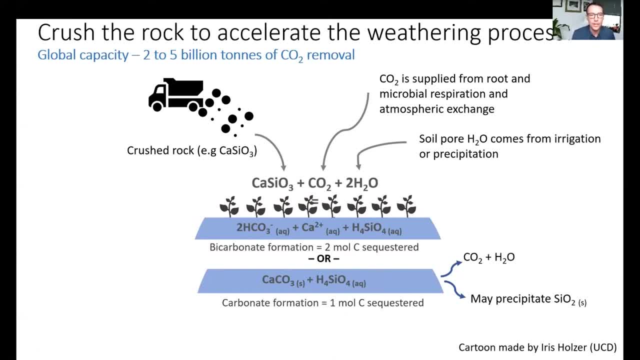 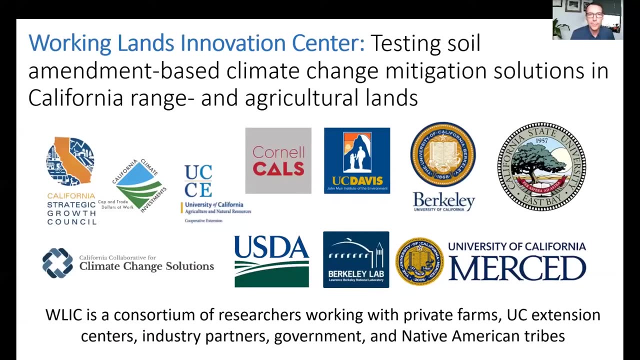 Rob Lemansky. years of CO2 removal, so very secure carbon that is not susceptible to biological reactions in the way that organic carbon might be. Rob Lemansky. In the working lands innovation Center, we are trying to fill the gap between where the capacity is and where the science needs to go to really understand how this technology operates across diverse cropping systems when carbon dioxide is removed. 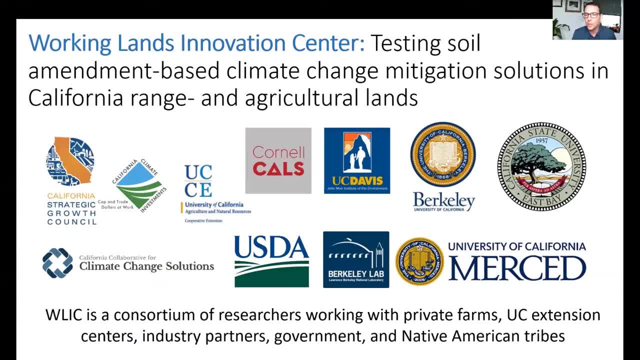 Rob Lemansky- When it is not so efficiently removed and how we can work with farmers, ranchers and industry partners, government and tribes to understand the full potential in terms of barriers to adoption. Rob Lemansky. In the working lands innovation Center, we have created an ensemble of different researchers across California working in combination with the US Department of Agriculture. 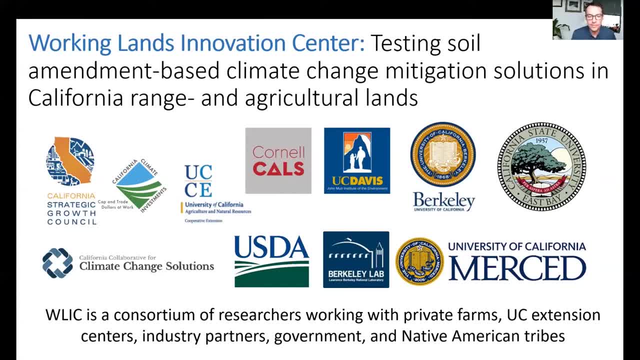 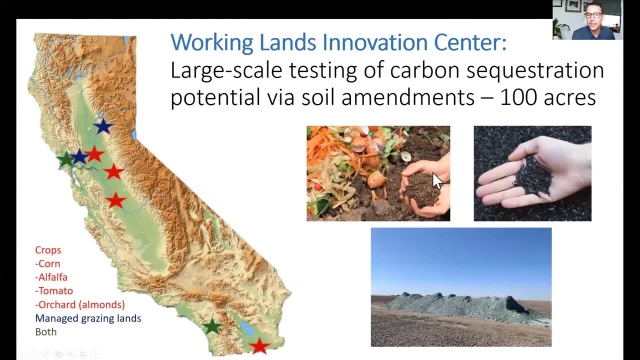 Rob Lemansky and local government agencies, as well as private farmers. Rob Lemansky- And you see extension to examine in an array of approaches dealing with enhanced weathering. Rob Lemansky, In this approach we are also examining enhanced weathering in combination with organic amendments from compost, in this case, working with manure repurposing and green waste. 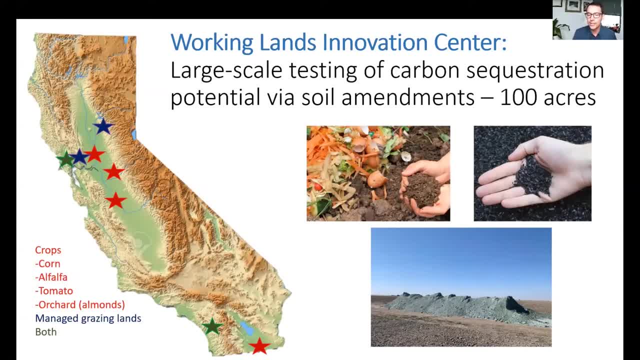 Rob Lemansky, As well as biochar, which is being generated from salvage trees that impose a fire risk. applying these separately in combination along the backbone Rob Lemansky, Of the Central Valley all the way into the imperial valley along the border of Mexico, gives us a bio climactic envelope. 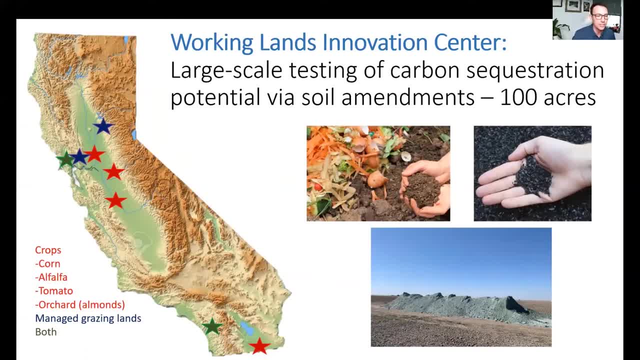 Rob Lemansky. That allows us to really understand exactly how this technology works across a range of conditions. that includes coastal conditions, which are relatively cool, and interior conditions, which are incredibly hot. we are working across corn, alfalfa, tomato and orchards, Rob Lemansky, As well as manage grazing lands in both. in some of our research, 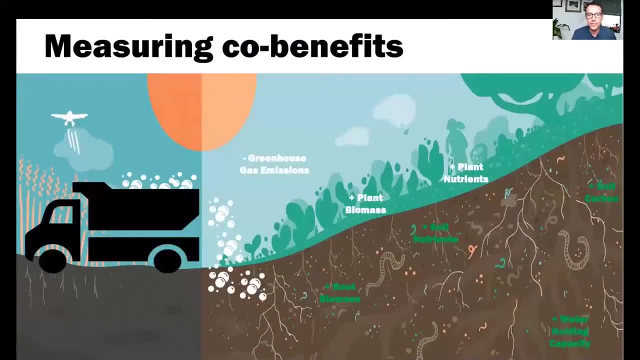 Rob Lemansky sites. Rob Lemansky. we're measuring co benefits in this project. we believe that one of the greatest opportunities for carbon dioxide removal will come when we have what we call carbon capture with benefits. that is, Rob Lemansky, Enhanced yield in our cropping systems, more nutritious food supply and healthier soils, as well as things like water holding capacity. so we are measuring all these co benefits in combination with greenhouse gas emissions, including flux towers. 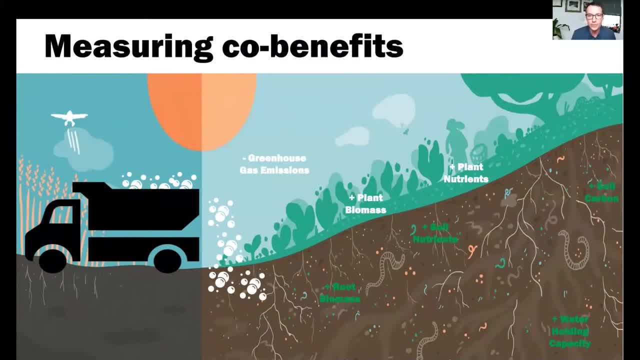 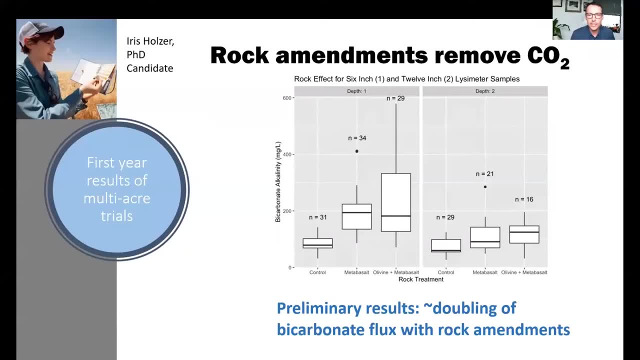 Rob Lemansky, and measurements and techniques to understand enhanced weathering within the soil, Rob Lemansky. So we have observed some incredibly exciting results in only the first year of this study. this is these are results from my PhD student at uc, Davis, iris holzer. iris has been examining enhanced weathering and the byproducts of the weathering reactions in lysimeters that are collecting. 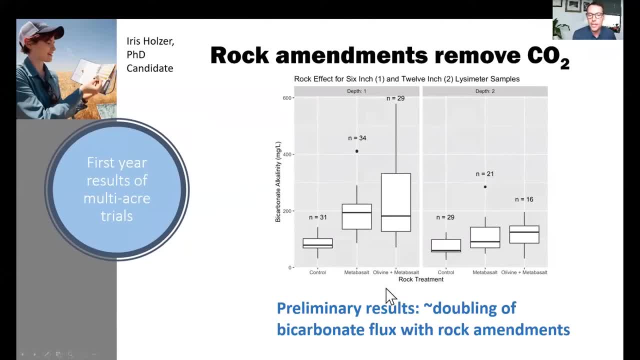 Rob Lemansky soil water. Rob Lemansky Soil water across control, meta basalt and olivine plus meta basalt treatments and she's finding an approximate doubling of CO2 sequestration in the form of bicarbonate in the soil water. 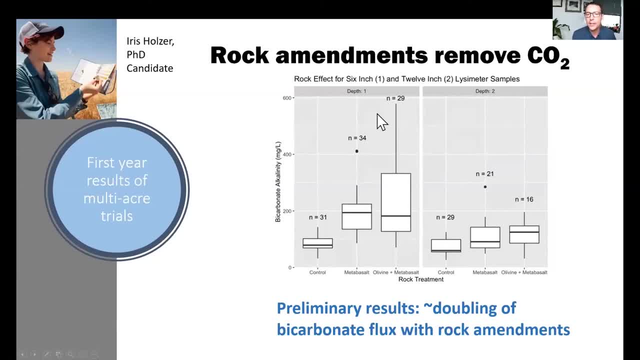 Rob Lemansky. In addition to the surface soils, where she is examining lysimeter water in the top six inches, she's also looking below the till environment and it's starting to, Rob Lemansky, detect a little bit of evidence that bicarbonate is also forming. 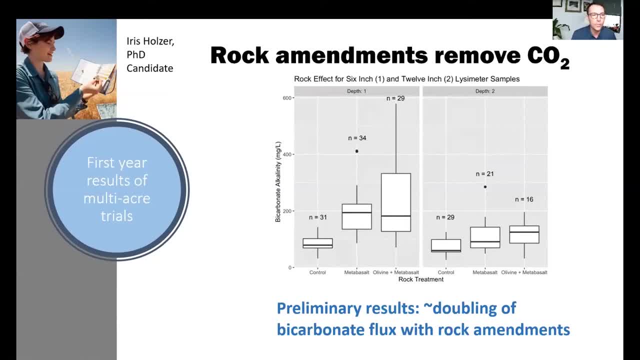 Rob Lemansky. Deeper into the soil, just beneath, where the weather rock material is, is happening in the surface. so really exciting results. we're not sure how well these results will hold, but I would add that these results are actually happening in with a historic. 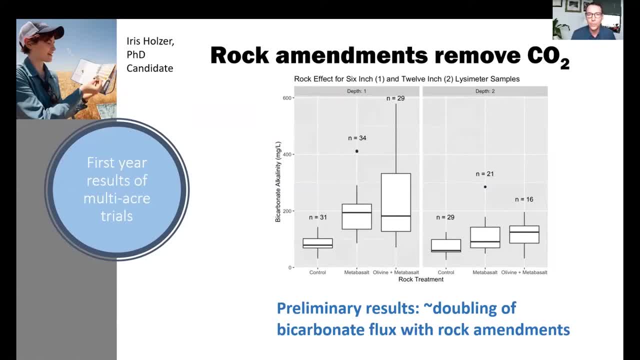 Rob Lemansky. drought in California, telling us that even under incredibly extreme climate of the future, enhanced weathering still has the capacity to more than double CO2 removal, again Rob Lemansky, In the form of bicarbonate which is not vulnerable to things like microbial decay. scaled up, this would be approximately one ton of CO2 removal per acre, which is the equivalent with what you might find in an acre of trees planted to remove carbon dioxide. 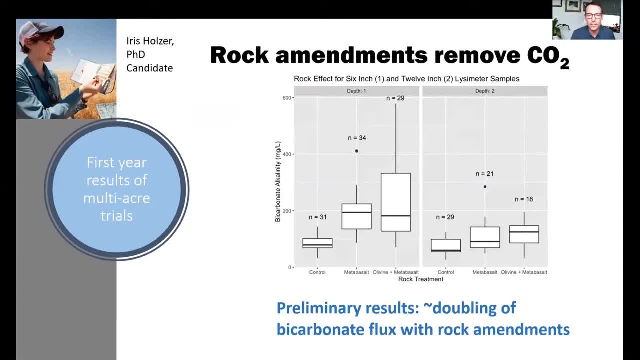 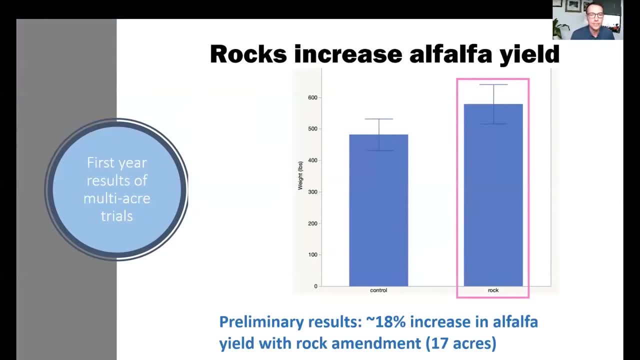 Rob Lemansky. The notable looks at exception here is that this is bicarbonate or inorganic carbon, as opposed to organic carbon, Rob Lemansky. In addition, we are, Rob Lemansky, Finding evidence in the first year of trials for enhanced yield in alfalfa. we are still going through data in corn and other crops, but our alfalfa yields have gone up around 18% across 17 acres and this is on real farms. 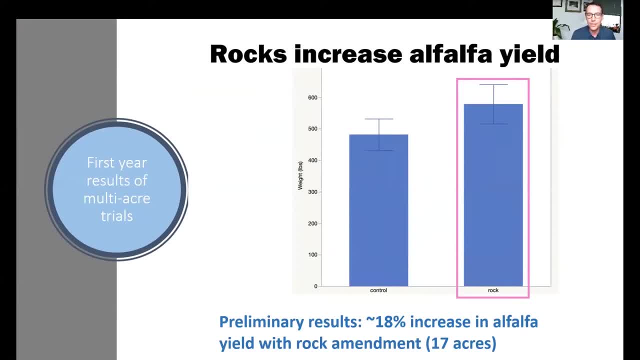 Rob Lemansky, Working with farmers throughout the central valley. we need to know if these results will hold. one year result is not enough to draw any kind of conclusions, but it is compelling to see that yield is enhanced with rock dust. Rob Lemansky. This is consistent with what has been found in relatively small settings in greenhouse environments in the past and is likely a product of some of the micronutrients that are released from the rock minerals, as well as pH changes and perhaps even some water holding capacity changes, which we are exploring. 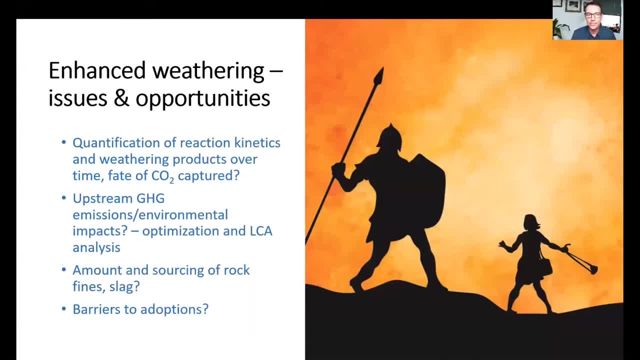 Rob Lemansky. There are many issues and opportunities in front of us still to understand how enhanced weathering can scale. there is still a heck of a lot of Rob Lemansky Science that needs to take place in terms of understanding predictive analytics of the rate of weathering reactions and the fate of CO2.. 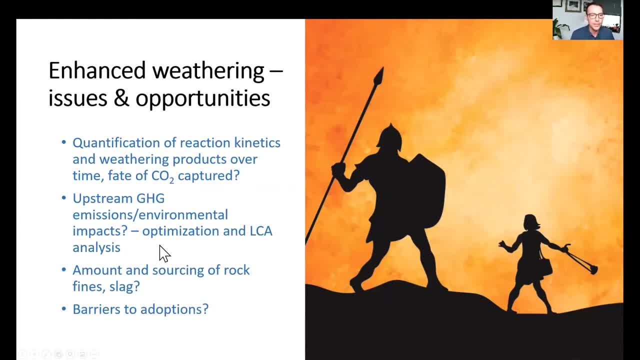 Rob Lemansky. We are also exploring the life cycle of the material, including mining, Rob Lemansky, Including transportation and application, and how that can chew into some of the greenhouse gas benefits. Rob Lemansky And we are performing some optimization analysis in terms of economics in greenhouse gases in the project. but this 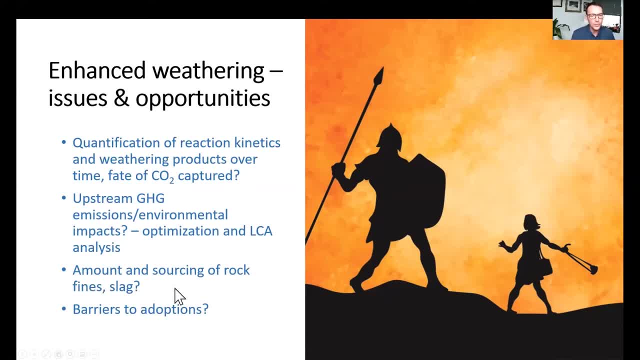 Rob Lemansky Is a huge area that needs a lot more attention. also, there are questions about the amount of rock dust that is available, and there's compelling evidence that there is enough rock dust, Rob Lemansky That has already accumulated over time to get us to billions of tons of CO2 removal on the planet if deployed on earth, croplands and a future where slag and 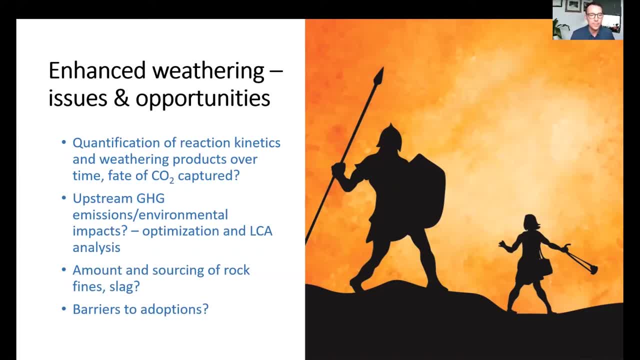 Rob Lemansky. Concrete manufacturing byproducts, as well as demolition, could be used for enhanced weathering to avoid, Rob Lemansky, The need for mining operations. but there are still incredible barriers to adoption, and some of those are price point barriers that our farmers are facing. 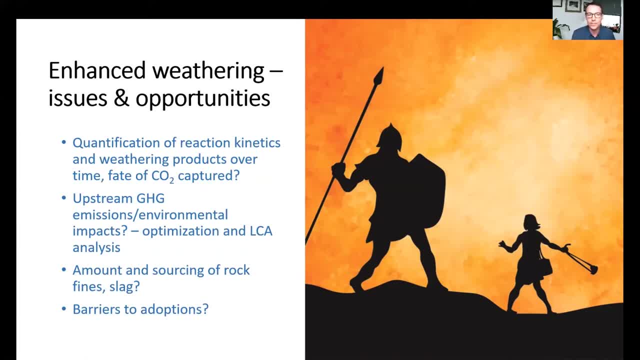 Rob Lemansky. Currently we estimate that it's anywhere between 60 to $200 per ton of CO2 removed, so still need to get that price point down to something that's more on the order of $100 per ton of CO2.. 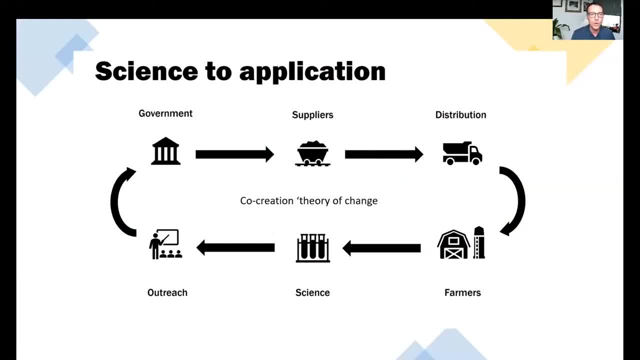 Rob Lemansky. Also, science to application is a huge part of our project and I won't get into that now. perhaps in the Q amp a, Rob Lemansky, This can be discussed. but our theory of change means including suppliers, government distribution, farmers, science and outreach together in our ecosystem model. 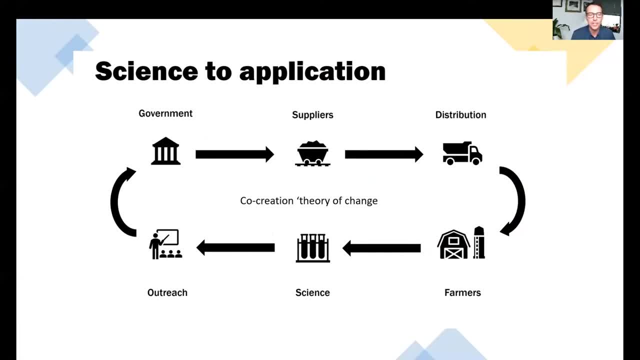 Rob Lemansky, Our model of change to really understand the barriers to adoption and how to overcome them as quickly as possible. so our project is, by design, one where co creation involves Rob Lemansky, The application of the amendments in our understanding of where the science needs to meet the real world. 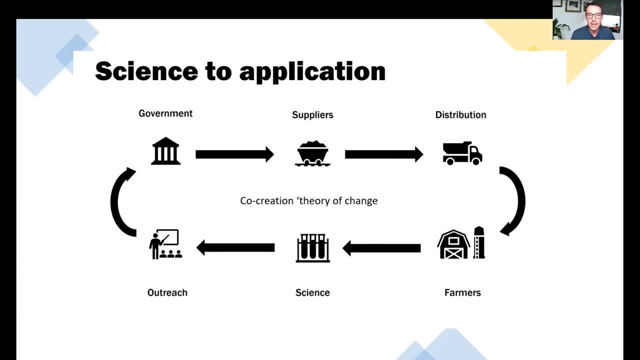 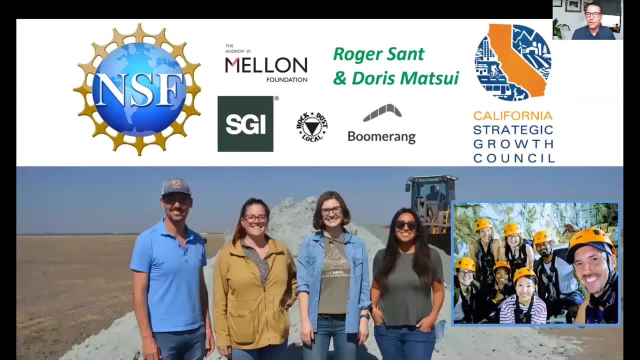 Rob Lemansky In terms of what farmers are experiencing and how to bring the price points down, Rob Lemansky, So thank you so much for this brief overview. I look forward to the outcome of the question and answer period and I hope you have a terrific panel discussion. 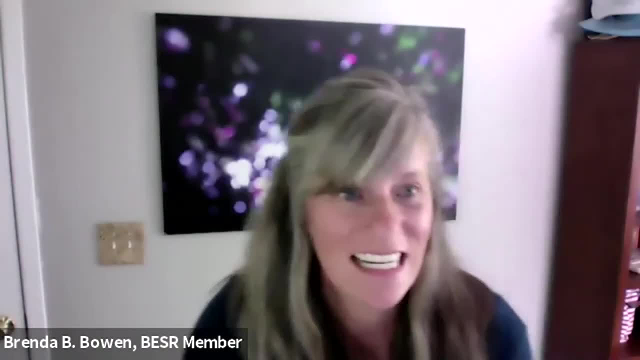 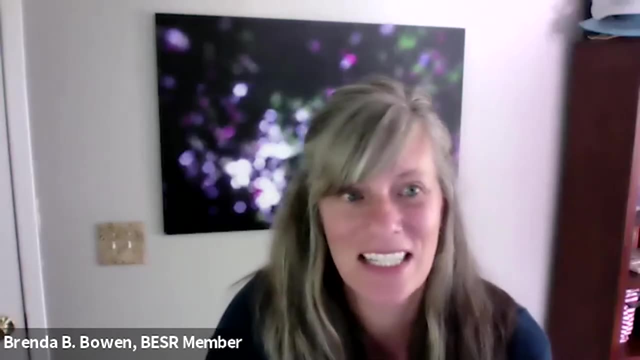 Rebecca Sandefur. All right, Rebecca Sandefur. Thank you, Rebecca Sandefur Ben, for that great presentation and for recording it for us today. we'll miss having them on the on the panel, but look forward to a conversation. 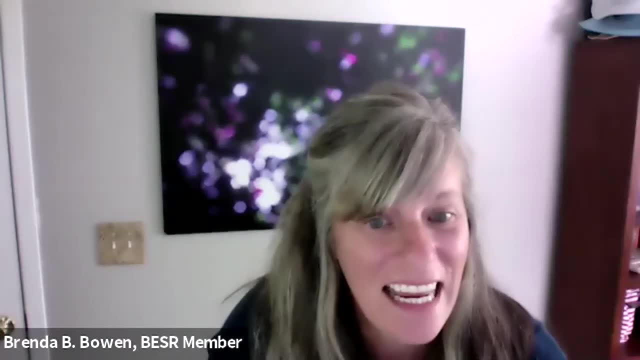 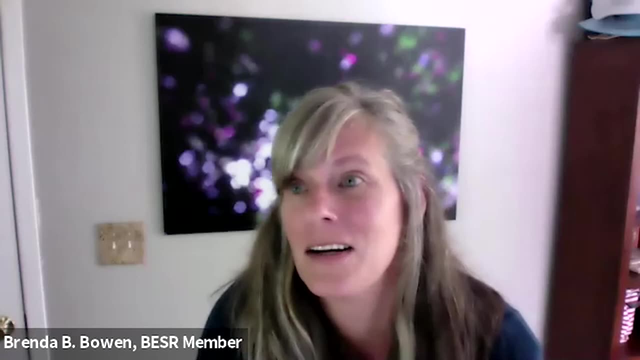 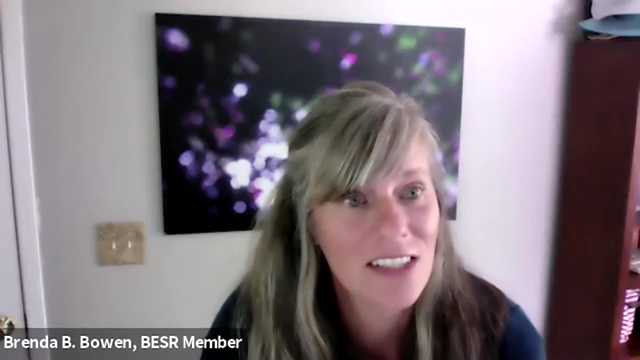 Rebecca Sandefur With everybody after a quick break. just want to thank Nicole and Rebecca and Ben for their excellent presentations and for being here with us today. Rebecca Sandefur, We will take a not quite 15 minute break now and come back at five past the hour for our panel discussion, so please rejoin us. 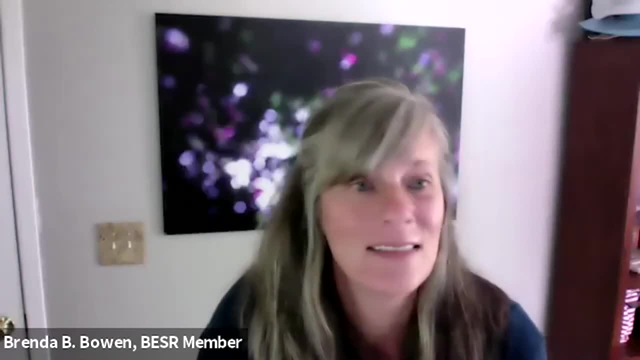 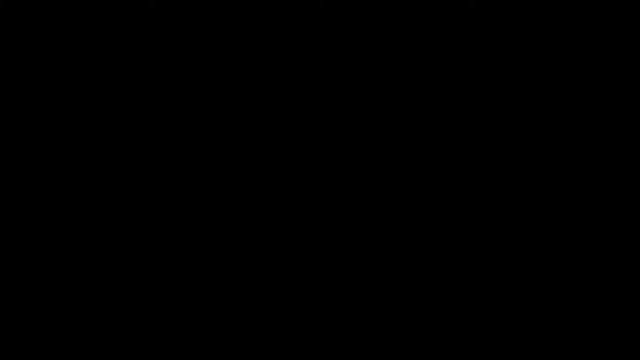 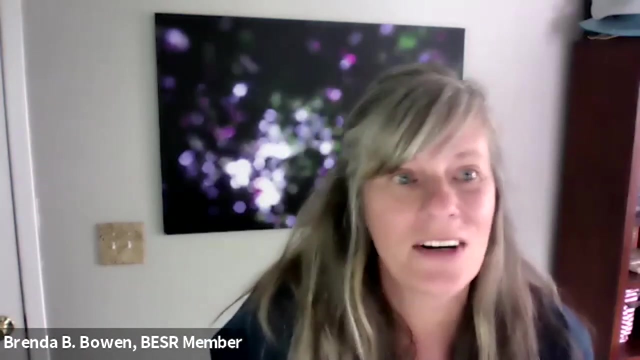 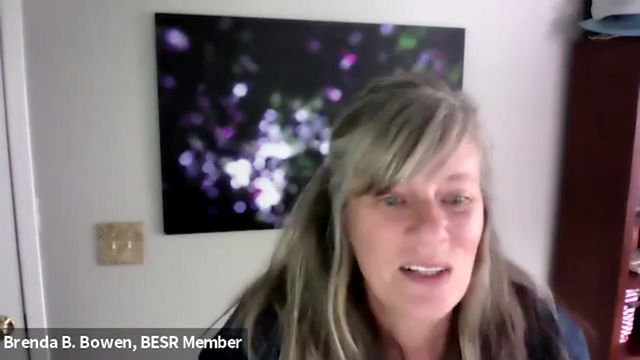 Rebecca Sandefur, At 205 Eastern time, and please come with your with your questions, for all of our panelists and we'll look forward to a great discussion. thank you, Rebecca Sandefur. Hello, welcome back, everybody. we hope you were able to join us for our presentations earlier today by Nicole Saunders, Rebecca Hernandez and Ben Fulton. Nicole and Rebecca will now come back for a panel discussion and we'll be joined by 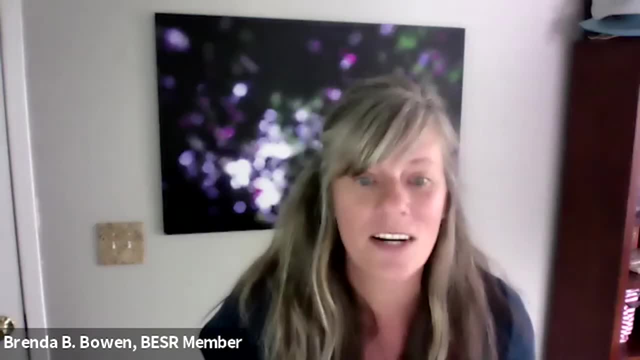 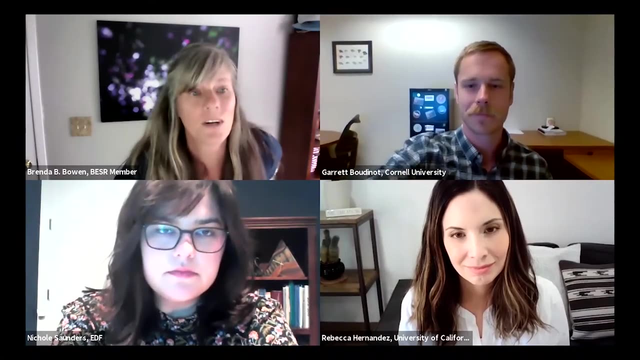 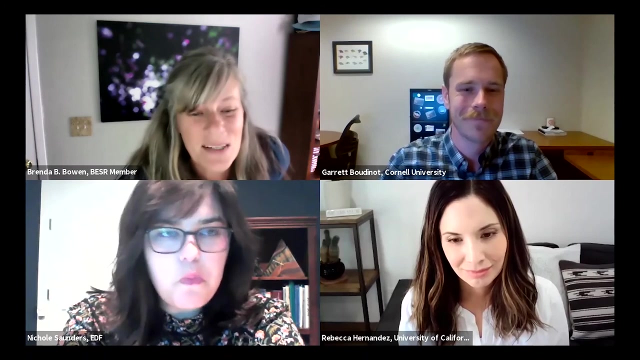 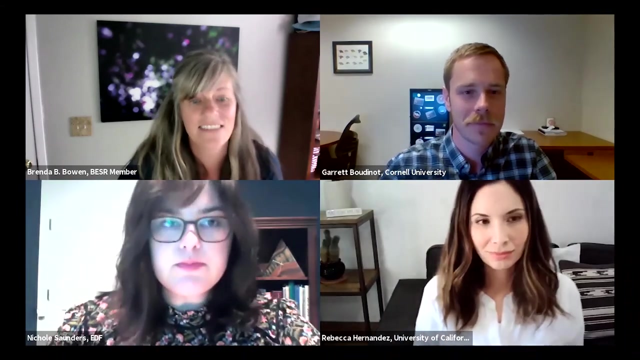 Rebecca Sandefur. Garrett Buddha know, a research associate with cornell's department of ecology and evolutionary biology and the College of agriculture and life sciences, who works on the enhanced weathering project with Ben Garrett, Rebecca Sandefur, And also works as with Ben Garrett. also works as a Community science fellow with ag use, thriving earth exchange and serves as a science advisor at climate music. Garrett, thank you for jumping in to join our panel. 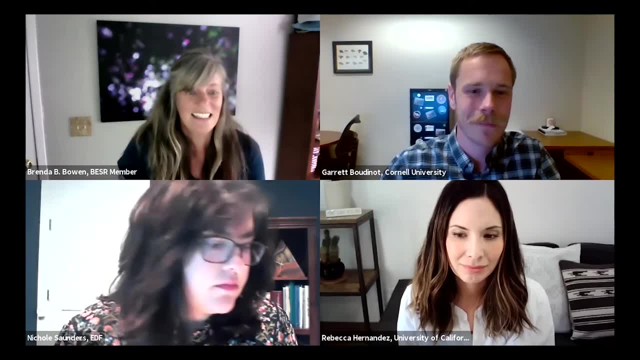 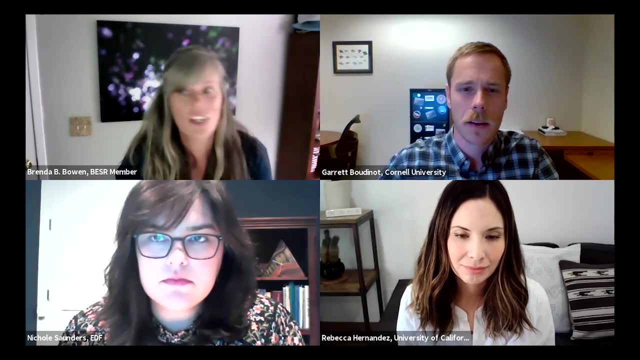 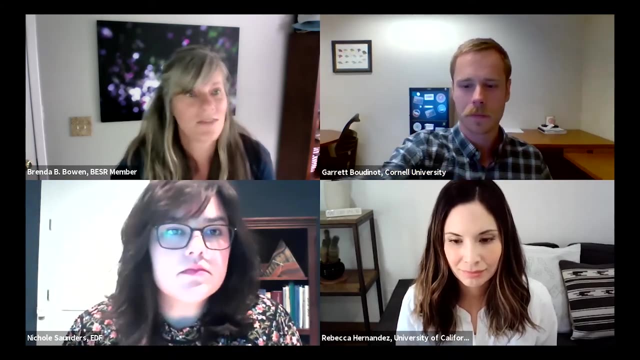 Rebecca Sandefur. Thank you, Rebecca Sandefur. We really appreciate your participation today, Rebecca Sandefur, So for those of you joining us in the audience, please feel free to put your questions into the Q amp a box and at the bottom of the screen, and we will intersperse those questions with questions from our visa board members. 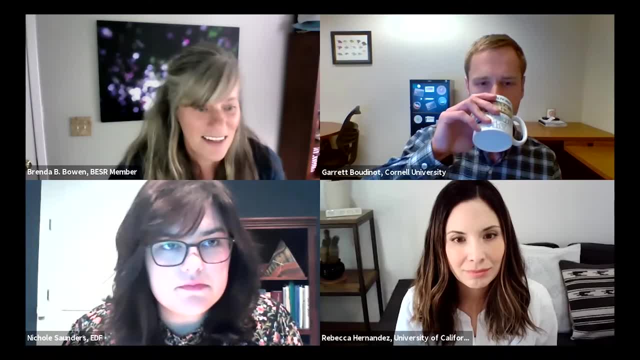 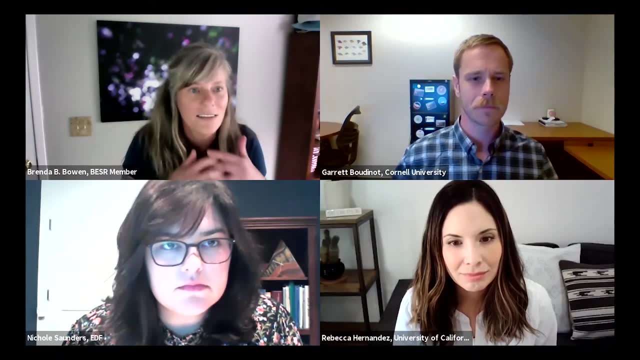 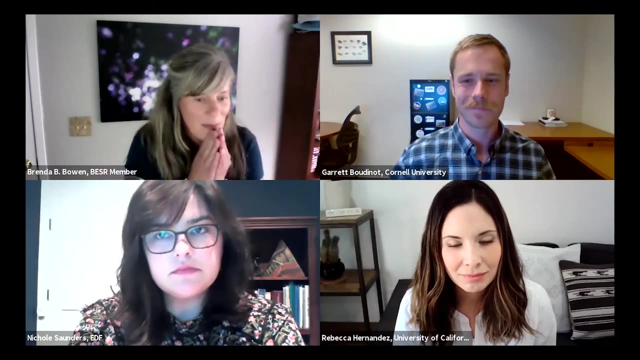 Rebecca Sandefur. And so, to start off, Rebecca Sandefur, i'm, you know, really excited to be able to have this discussion today at this. Rebecca Sandefur, Intersection of of water, land, subsurface rock processes. and think about how we're sort of communicating across these different disciplines as we work towards this energy transition. 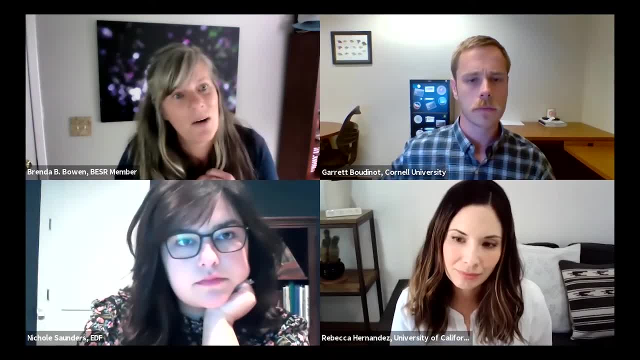 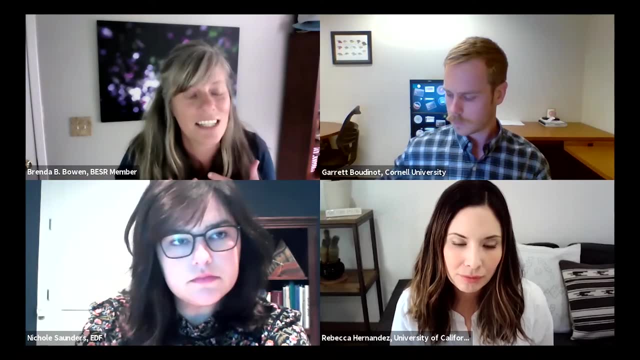 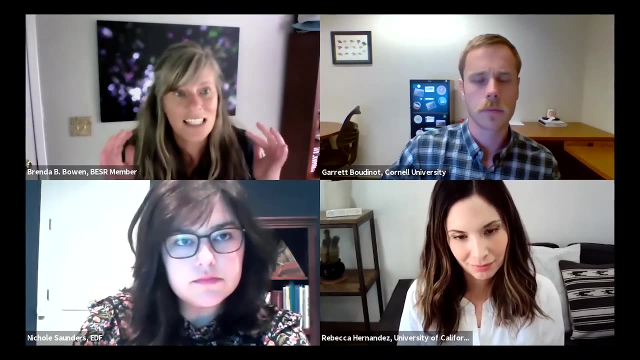 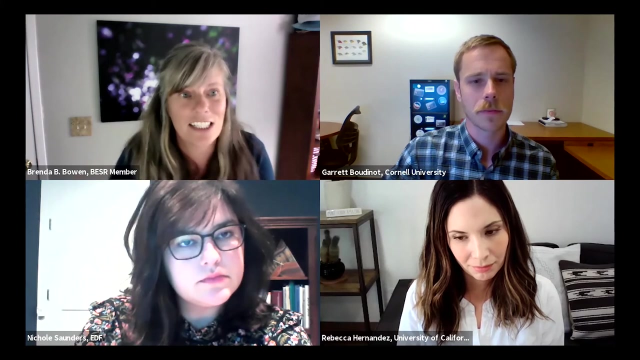 Rebecca Sandefur, And so i'm interested in hearing from our our speakers today about what you see that's working in creating the space for these really sort of interdisciplinary conversations. or we're talking about things and rock, subsurface weathering to Rebecca Sandefur, land and environmental justice to water, and where you see sort of the strengths in creating the opportunities for these sort of cross sector interdisciplinary 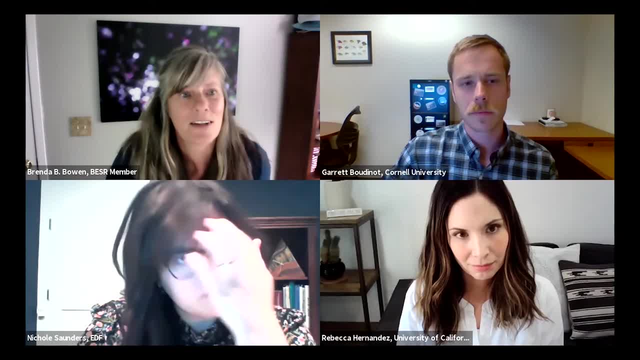 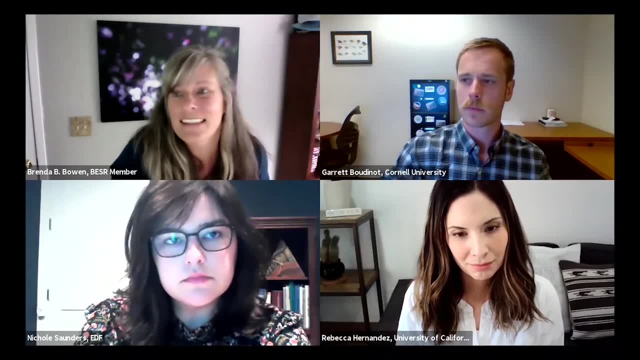 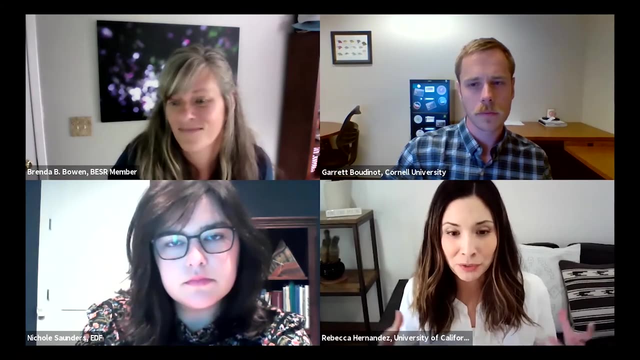 Rebecca Sandefur- conversations and where we're doing where those conversations are happening. and I guess, Rebecca, maybe can we. can I direct that one to you, Rebecca Sandefur? Sure, yeah, Rebecca Sandefur, I think that that you know. basically, what you're asking is where. 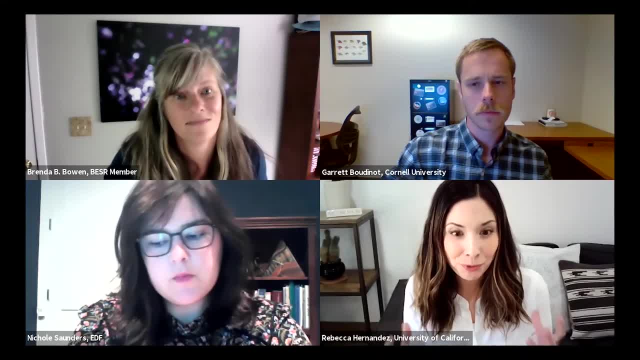 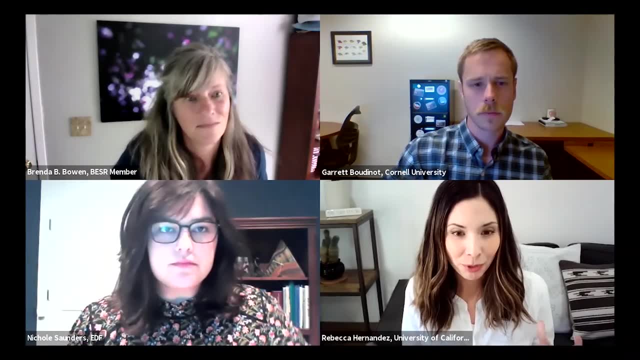 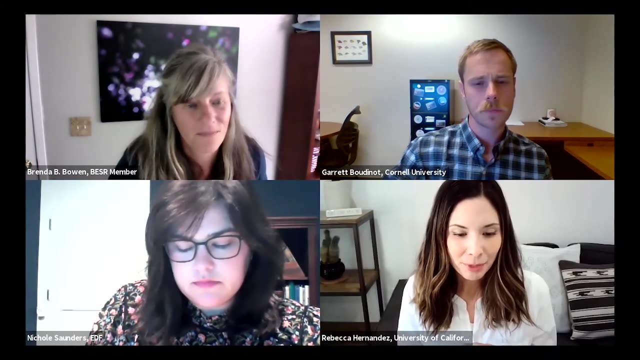 Rebecca Sandefur. You know where's this Rebecca Sandefur going to be developed most effectively, and I think that that is at the Rebecca Sandefur, Really where, where lots of different groups come together. the one thing i've noticed in my research is that it takes an entire knowledge system. 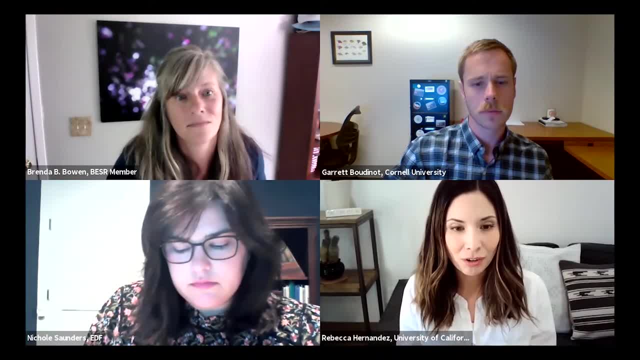 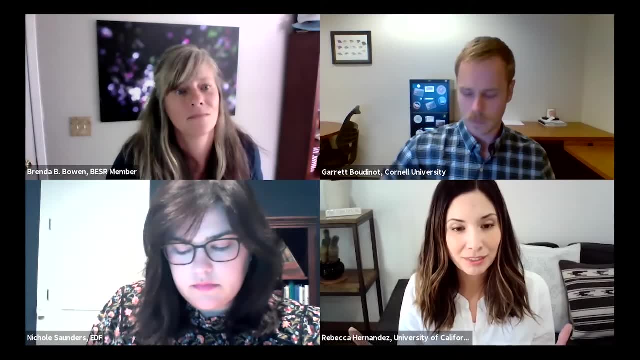 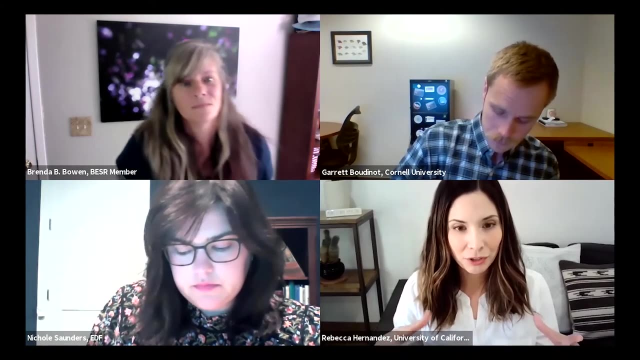 Rebecca Sandefur, To really shed light on all of the outcomes of a particular technology, both the positive, Rebecca Sandefur ones and the negative ones. and so you know making sure, when you are working on a technology, that you're incorporating the voices. 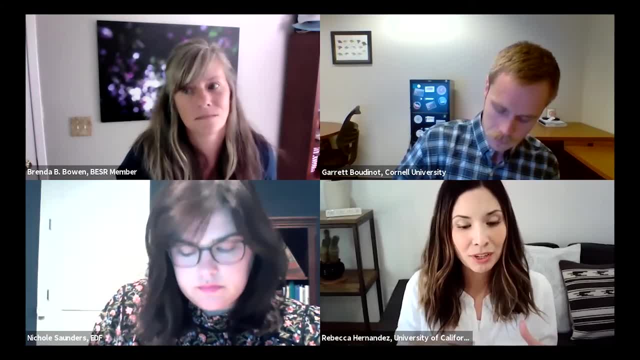 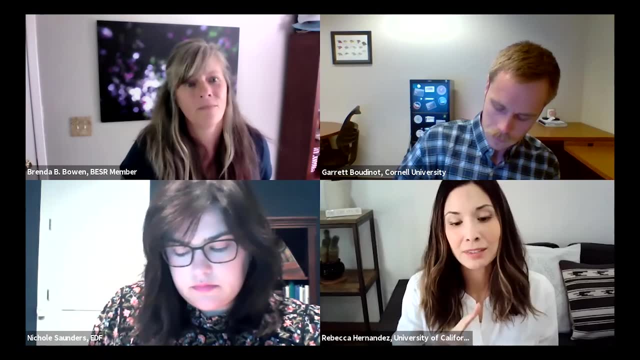 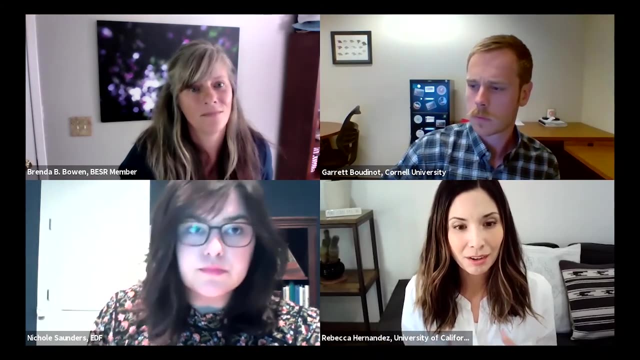 Rebecca Sandefur, The data from all of the groups involved, spanning multiple sectors, you know, not non governmental groups- government, industry, academia. I feel like that's really Rebecca Sandefur. that's really where a lot of Rebecca Sandefur Innovation can happen, especially when thinking about how to. 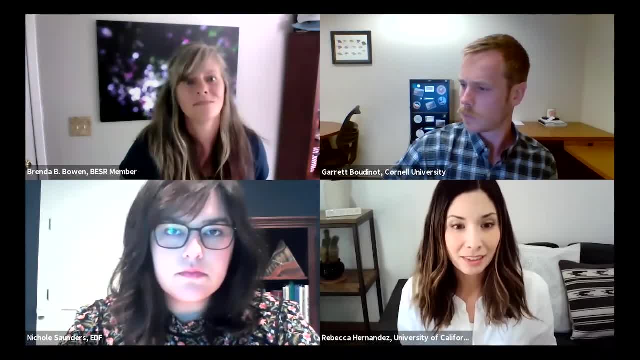 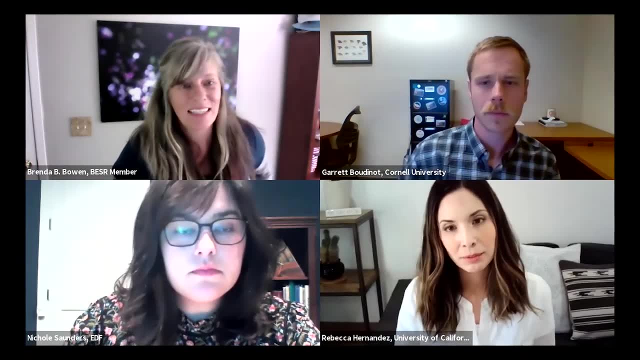 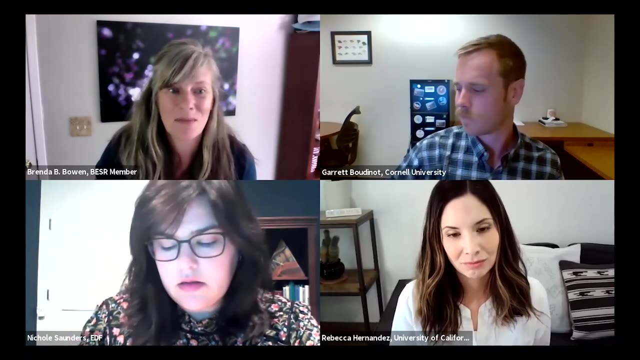 Rebecca Sandefur produce beneficial outcomes that outweigh the negative outcomes. Rebecca Sandefur, Thank you, Rebecca. Rebecca Sandefur, Nicole or Garrett, would either of you like to answer this question or we can. we can go on to one of the questions from our from our board. 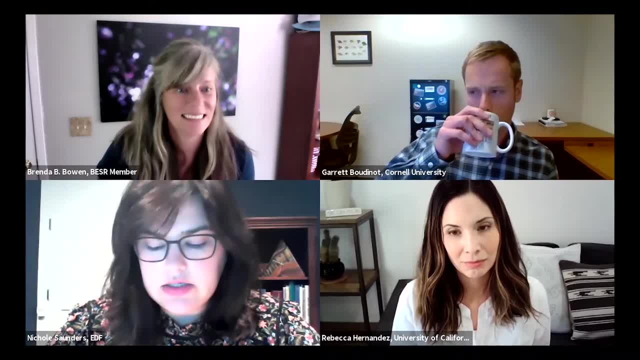 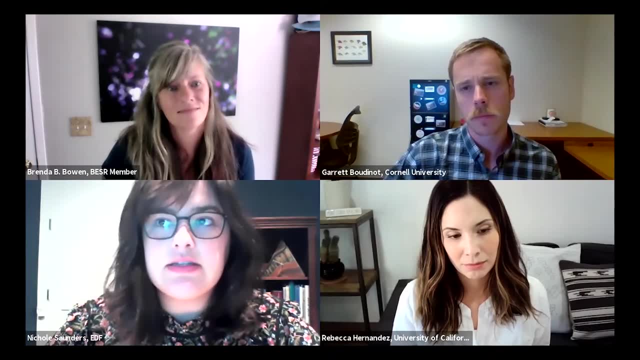 Nicole Coburn. I think this is Nicole- I can chime in quickly- and just I, Nicole Coburn. I liked, Nicole Coburn, The idea that you brought in the interval interdisciplinary and approaches to some of these challenges. one thing with the produce water in the oil and gas context is that 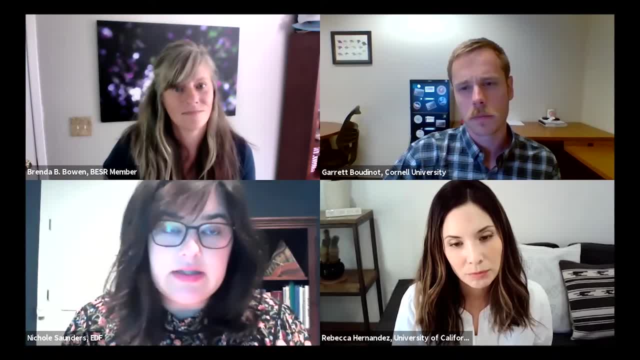 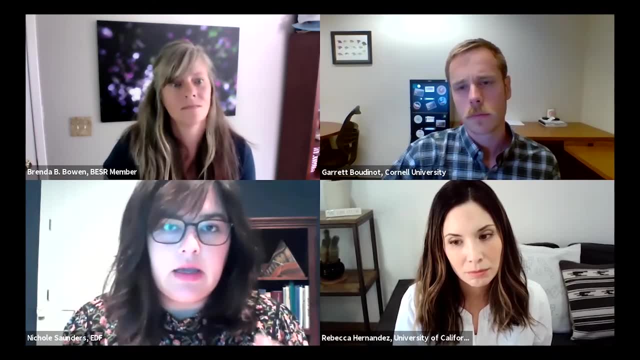 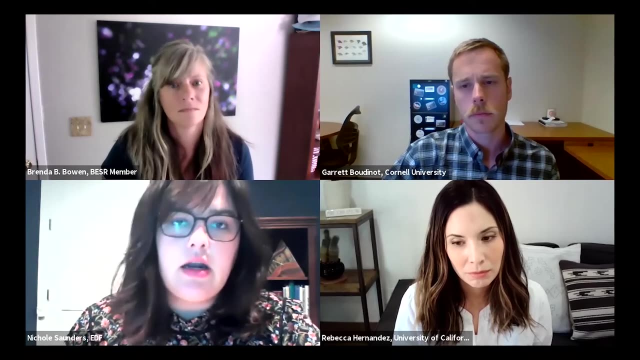 Nicole Coburn. we're only just now starting to see experts and entities and policymakers that are not traditionally involved with oil and gas decision making and oil and gas research chiming in on this challenge of looking to produce water and what the risks and- Nicole Coburn, Opportunities are. 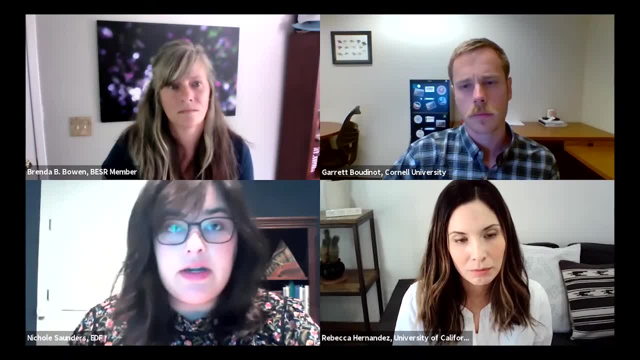 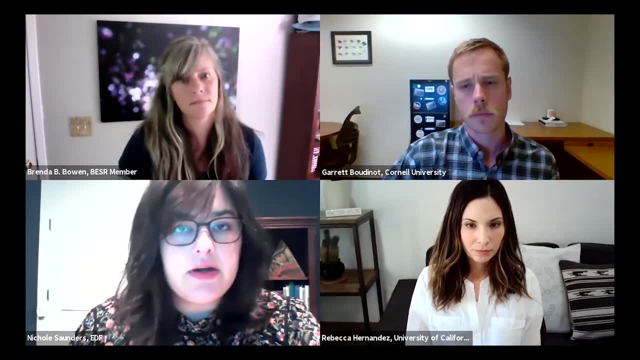 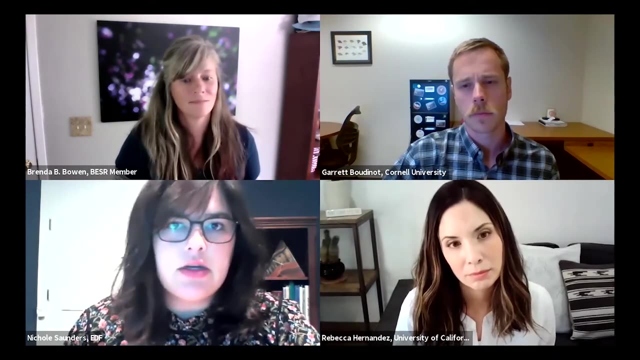 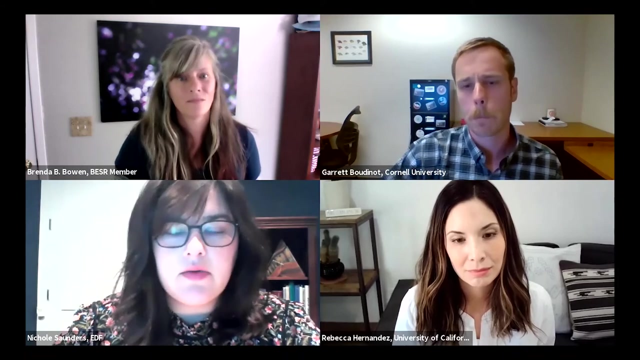 Nicole Coburn Are for its reuse. so things- everyone- from the impact of communities and end users outside of the oil and gas contacts to traditional water reuse experts that are bringing a different Nicole Coburn perspective and needed nuance and new thinking to this challenging raising. what questions need to be asked and answered to ensure that if that moves forward, it does so in a way that doesn't increase risk? 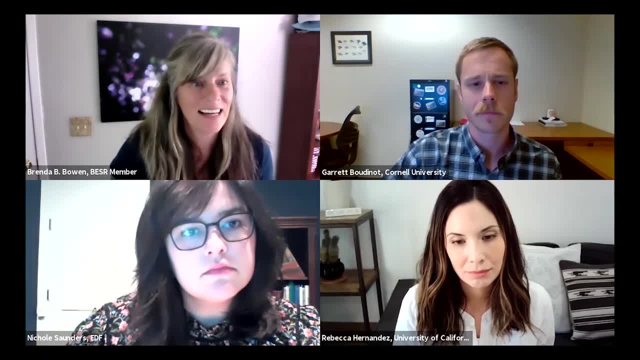 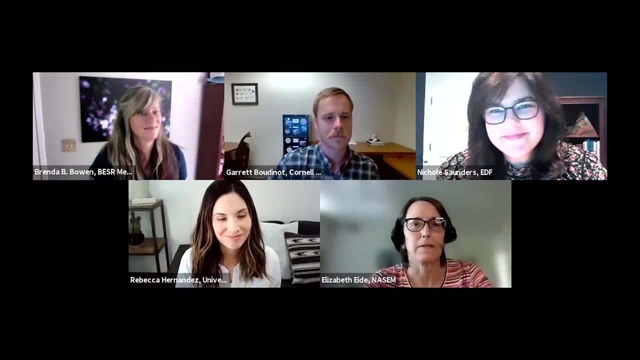 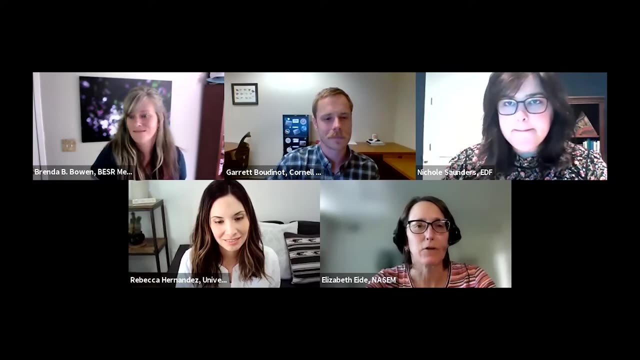 Rebecca Sandefur. Great Thank you, Nicole. Rebecca Sandefur would like to invite Elizabeth I to ask a question. Elizabeth A, Thanks a lot, Brenda. Hello everyone and my compliments to all three panelists. really great talks. I have a question actually i'd like to ask Nicole. Nicole, it's nice to see you again. 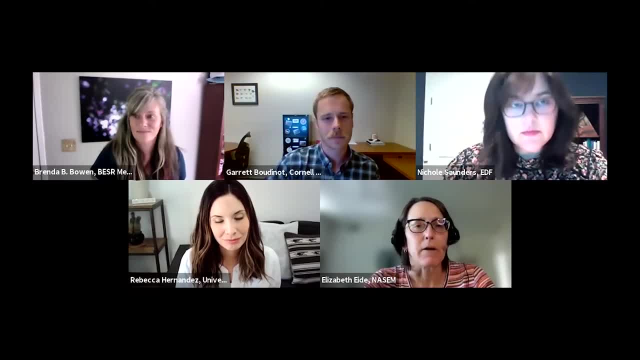 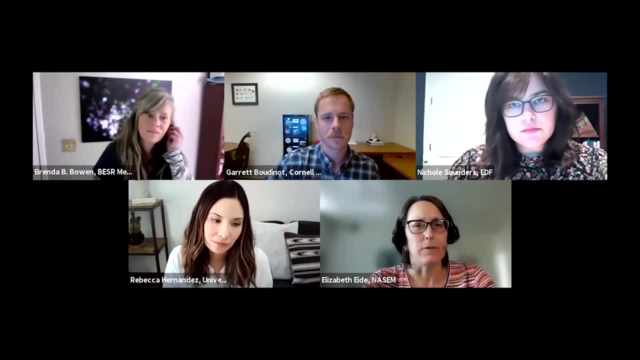 Elizabeth A Just in connection with you talked a bit about the fit for purpose aspect of the produce water and there's a degree of Elizabeth A of societal acceptance for some of the different applications- right, and I know the chemistry and exposure pathways and so forth. the different types of produce water or big issue and still need a lot, of, a lot of. 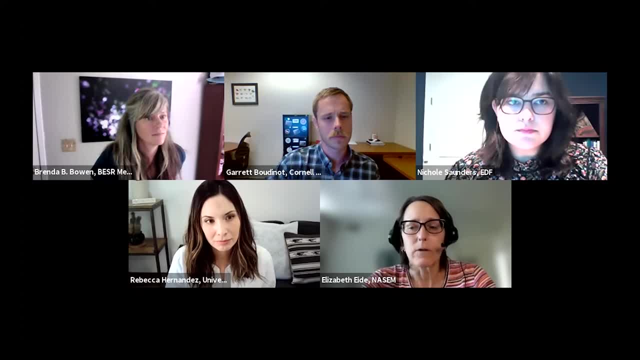 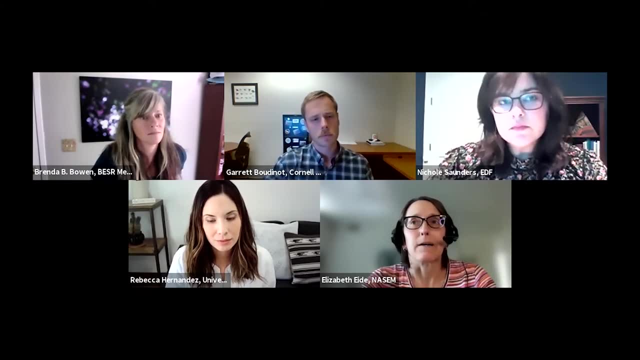 Elizabeth A Research in certain cases, certain parts of the country, but I wondered if you could talk a little bit about the volume challenge because there's a for any given purpose, Elizabeth A want to assure a consistent supply of the water and then a lot of places that that's been intermittent and 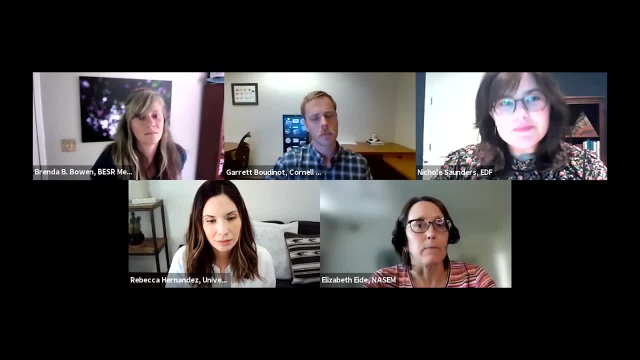 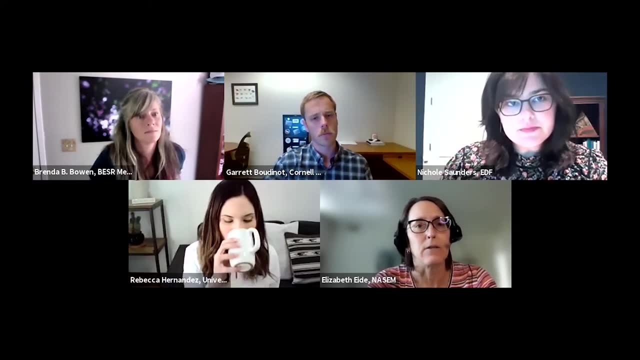 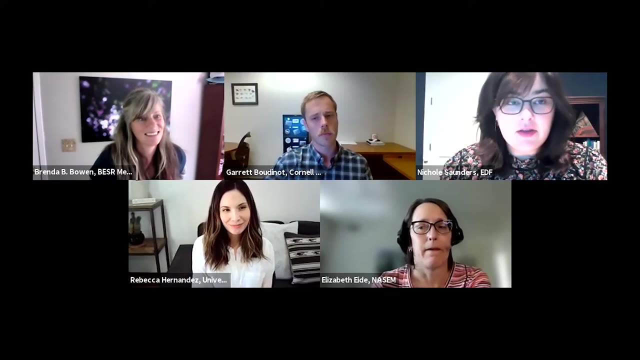 Elizabeth A, Particularly with this last year where the the industry has had some Elizabeth A swings, if you will, I wondered if you could talk a little bit about the quantity issue and and how it ties to the quality challenges there. Elizabeth A, that's a great question. Elizabeth hi, nice to see you as well and I thank you for the question. 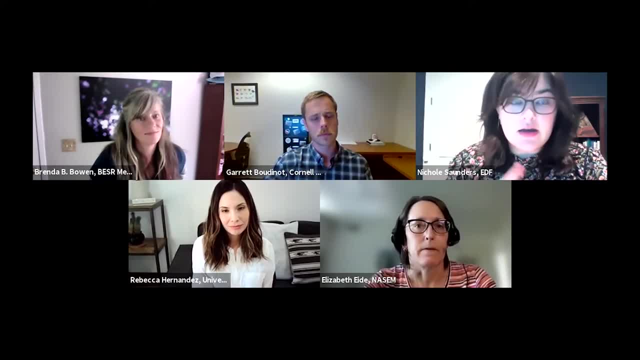 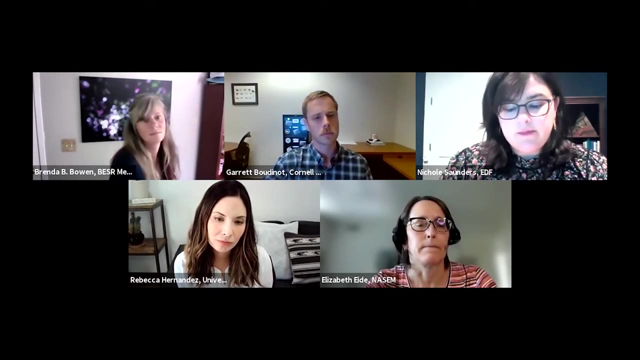 Elizabeth A I. there are some really great experts. I would first say on the quantity specifics of point directly to. maybe Bridget scanlon at Bureau of economic geology sees Elizabeth A published a lot of really fantastic Elizabeth A interesting research on this front. but generally speaking I think you raise an important point. that is the when you look at the reuse of a potential resource, how reliable is it? 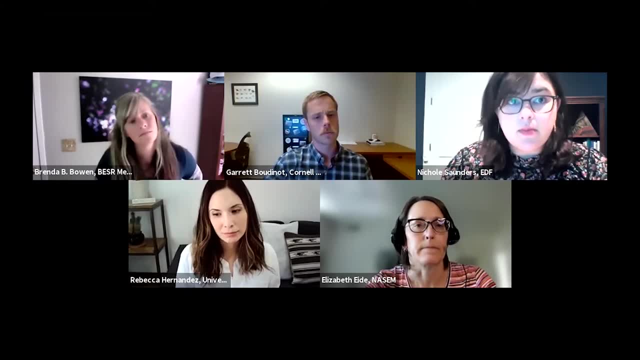 Elizabeth A. How consistent is it? are we going to have seasonal complications when we look at it? does it vary? and so all of those basic infrastructure and Elizabeth A Issues are really are important. when you think about produce water- and the volume is a challenge, you know, I think in some. 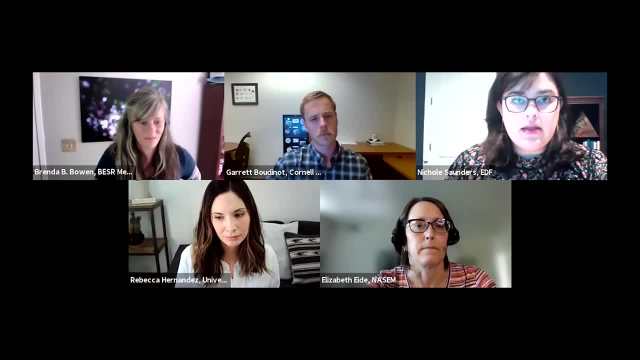 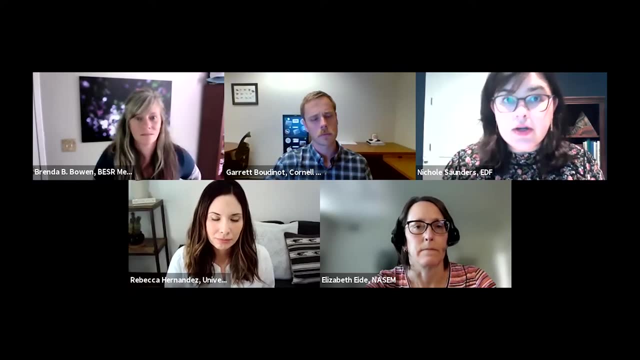 Elizabeth A Bridget studies out of the big, she's found that even if you were to put a large volume of this produce water to a certain use in a certain region, it's really not going to quench the thirst, maybe, of those uses, like an agricultural context and so 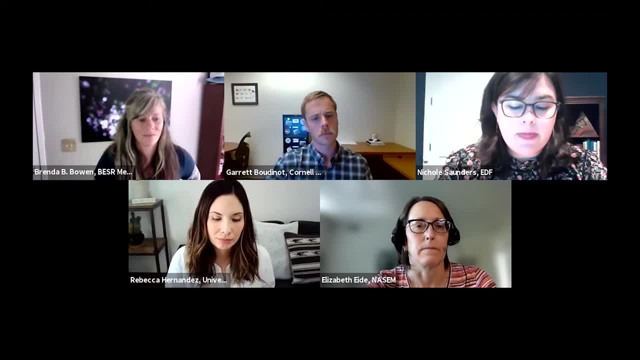 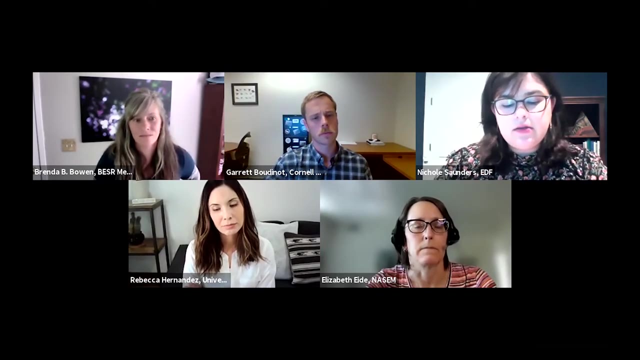 Elizabeth A. I think there is a challenge there and realistically thinking about from a volume perspective and the cost of treatment and the cost of Elizabeth A, Basically getting everything from one place to another. we all know that Elizabeth A The cost of using water period is very cost intensive. so thinking about that fit for purpose issue of in this place at this time is there an opportunity and 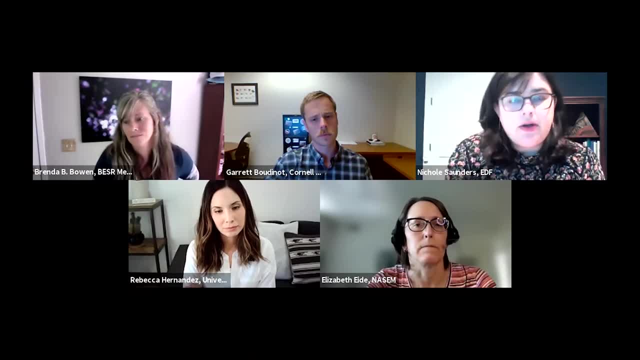 Elizabeth A. Perhaps the best and highest use of that water is to use it in oil and gas operations. stop using fresh water, Elizabeth A, and look for reliable disposal alternatives and allow the fresh water to be used in those regions for those other purposes. 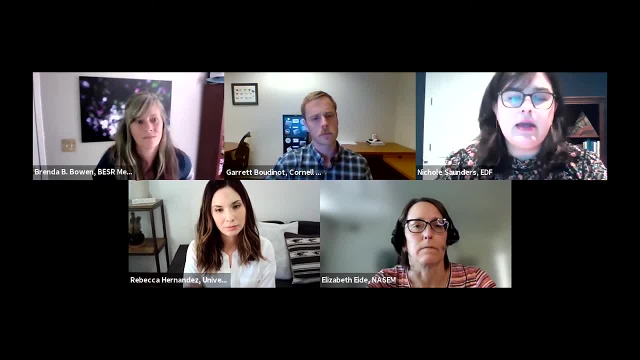 Elizabeth A And there may be some instances where it's worth the treatment to think about. but it's going to be Elizabeth A, Not a national application. it's definitely going to be heavily regional, if not very localized, I think, because of that volume, challenge and transportation and getting it where you need it. 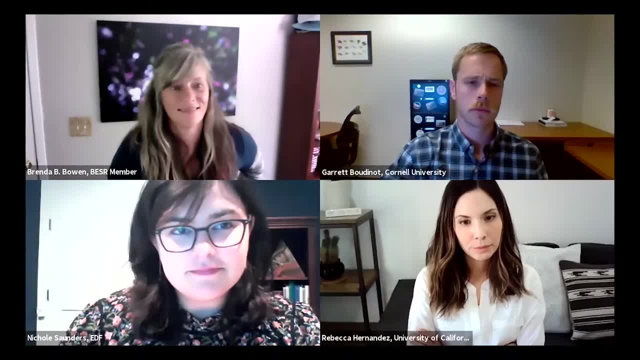 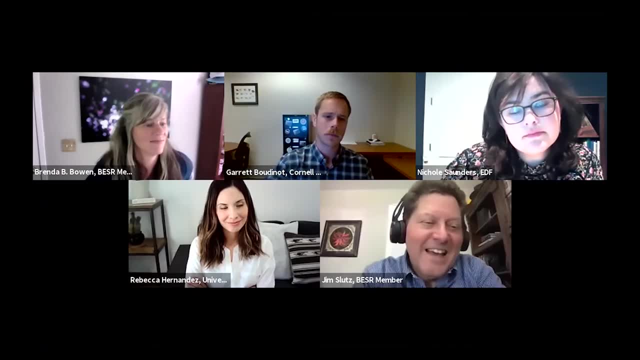 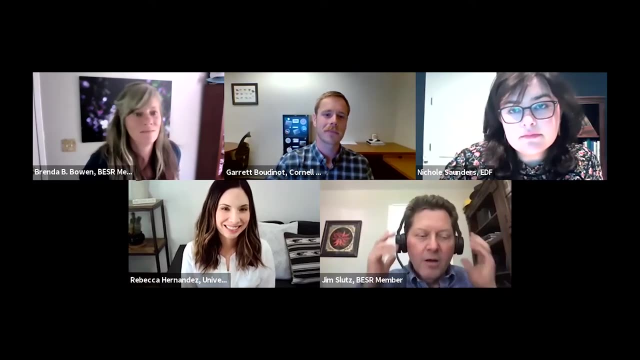 Elizabeth A Great. Thank you so much, Nicole. Nicole LiBaire- And i'll invite Jim to ask a question to sluice. Nicole LiBaire- Oh, we can't hear you, Jim. Jim Sluice- About now, Jim Sluice- yeah, okay, sorry about that. 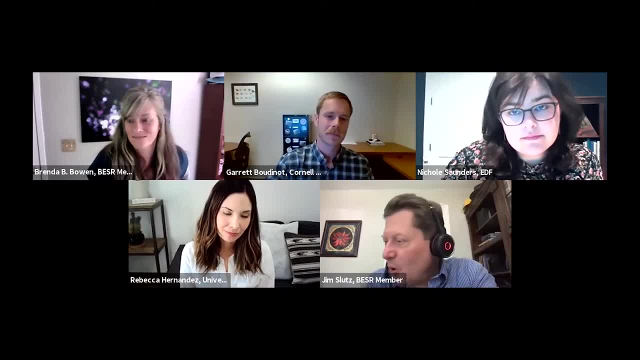 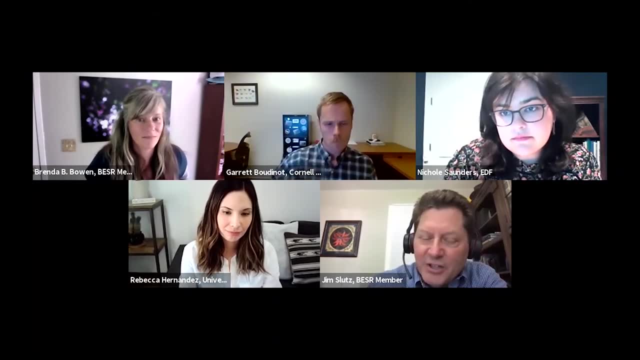 Jim Sluice- This is for Rebecca and it's really in the what's the two parter and looking at land use and different energy sources. the first is is more on whether you've looked at. yeah, I found it intriguing. I know that you're looking at very large scale solar. 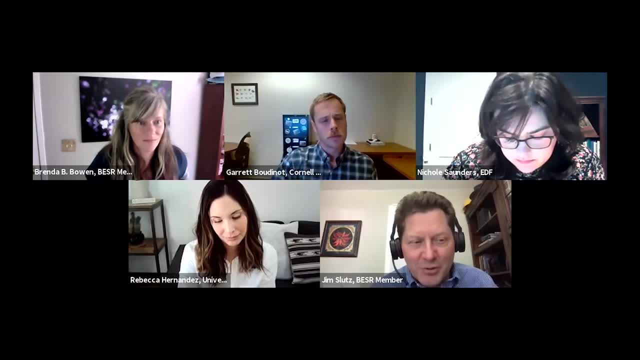 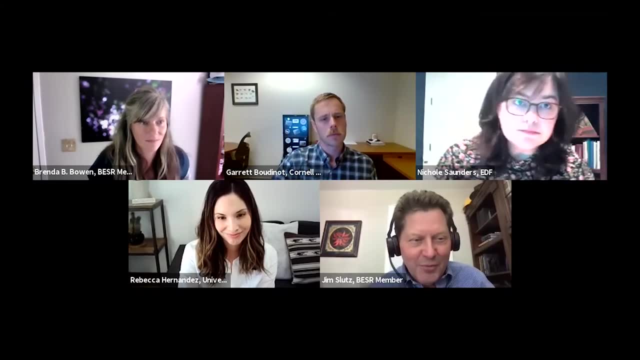 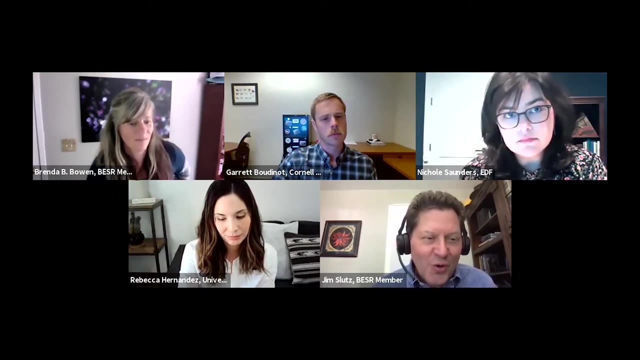 Jim Sluice- But when you look- you mentioned the free lunch being, if you put it on an existing building- Jim Sluice- One of the things- and this is because of personal experience- you come in go to put- like Jim Sluice- residential solar- there's a disincentive of oversizing your solar because of the way the net metering works and it would seem that if you could fix that- I don't know if you've analyzed any of that, but if you could fix that disincentive- disincentive so you would maximize the solar on on an individual roof- that that would have a collective benefit. 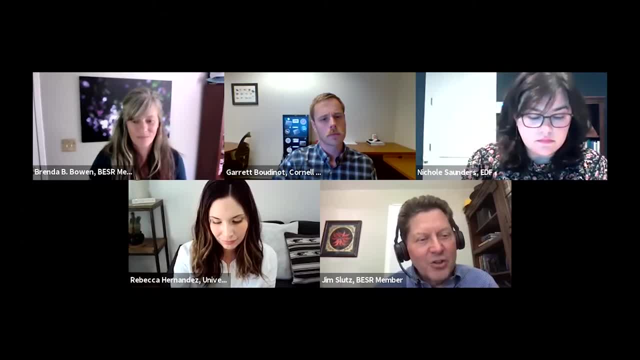 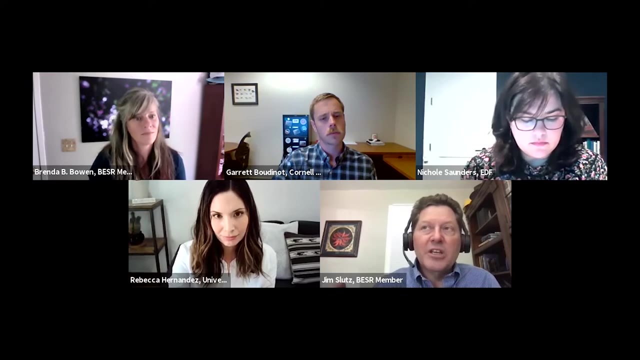 Jim Sluice- and Jim Sluice- Anyway. so that's part one. the other, Jim Sluice- Is looking at at different I in your. in one of your slides you showed land impact versus CO2.. Jim Sluice-, or economic or ecological impact and and so because the CO2 impact things like natural gas went out quite a far on the right on that. 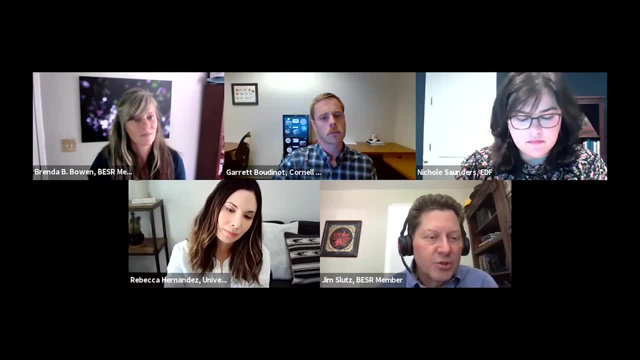 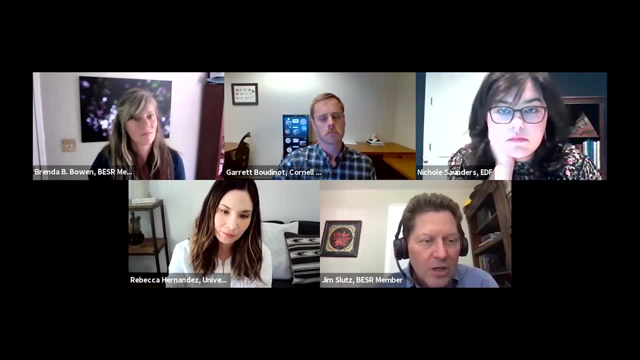 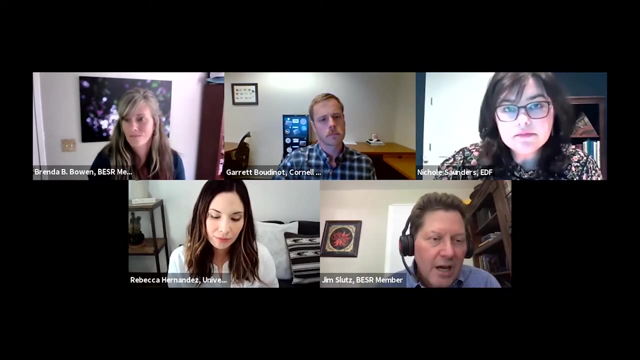 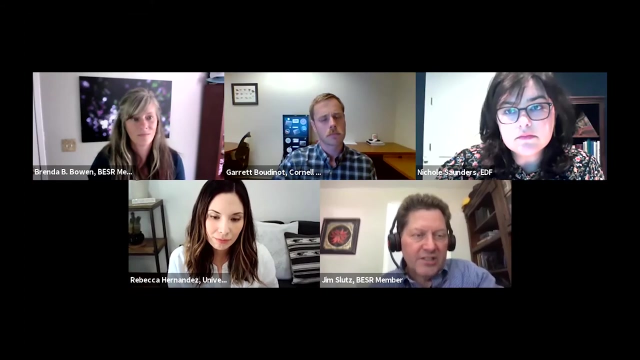 Jim Sluice- But have you, have you also looked at modeling? what would what if you were doing some level of of CC us with natural gas? have you looked at where, Jim Sluice- That would fall on the continuum sense most? most energy analysis is: hey, we're going to need some component of of at least of natural gas, in the future. in fact, some models say we actually in the near term have to increase natural gas use to meet energy needs. 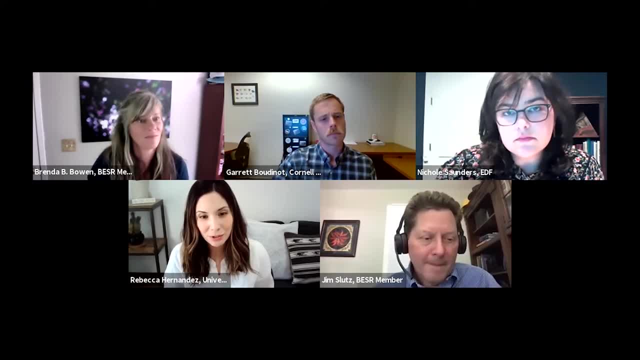 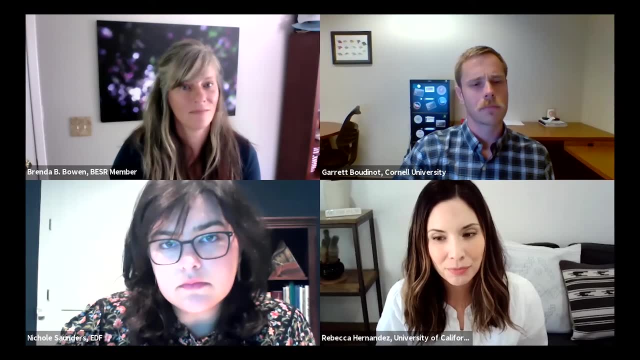 Michelle Magyar- Great question, thank you, Jim. to your first question on incentives: Michelle Magyar- I have to say Michelle Magyar- There are Michelle Magyar- A couple other Michelle Magyar- Excellent Michelle Magyar- Experts who are making. 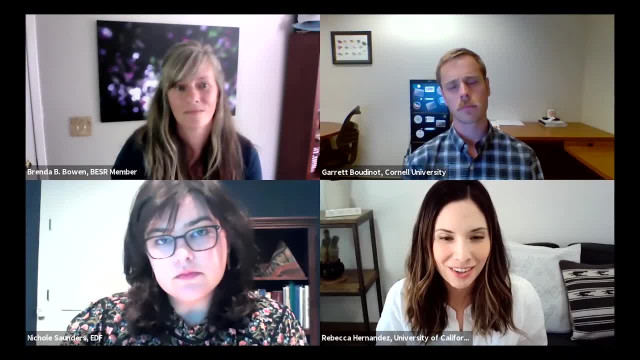 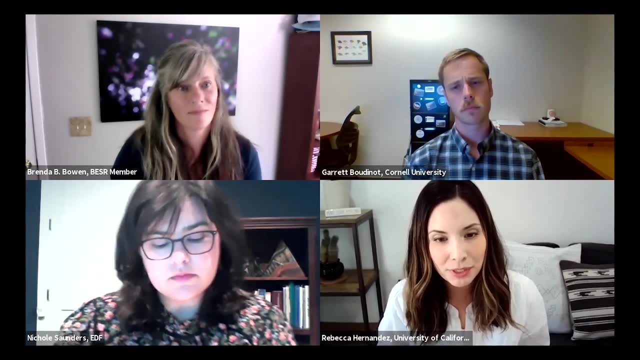 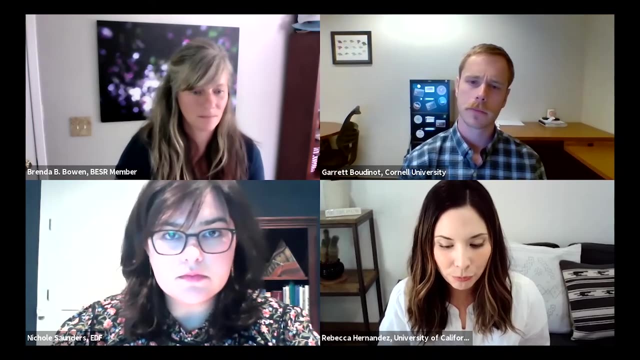 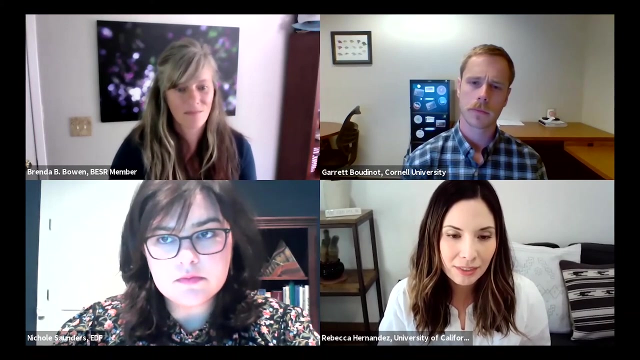 Michelle Magyar- A lot quicker, faster, better strides on that. on that particular topic, greer Ryan at the Center for biological diversity put out a really good report quantifying different incentives for low footprint. Michelle Magyar- renewables, solar energy in the US, and I think that really it's. it's clear that the the 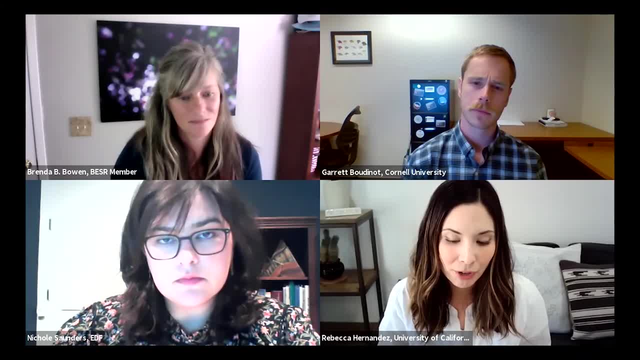 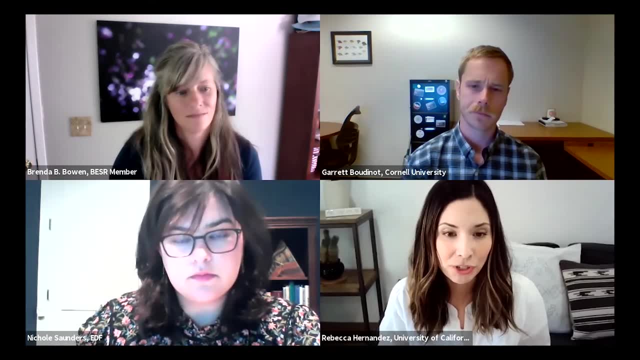 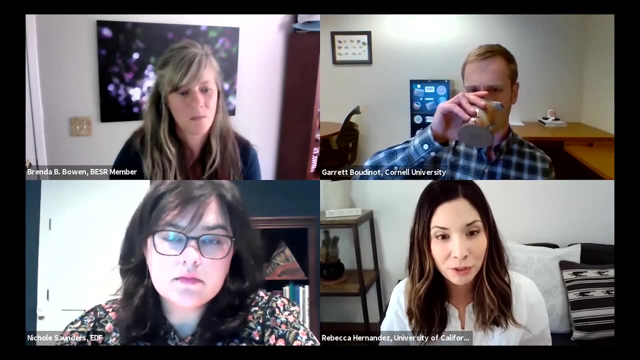 Michelle Magyar- incentives that we have in place- Michelle Magyar- are not matched to facilitate low footprint, low carbon energy development in the US, and this is this is problematic when we think about the fact that land use and land cover change is something that facilitates greenhouse gas emissions. 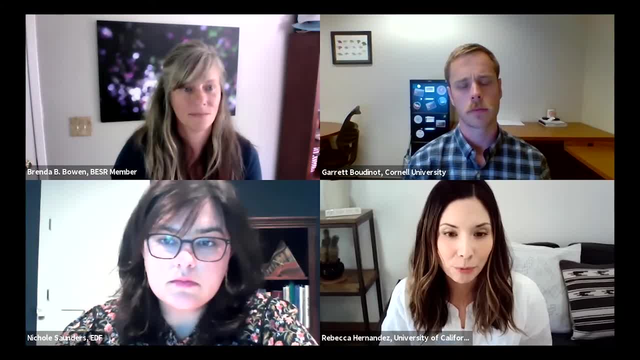 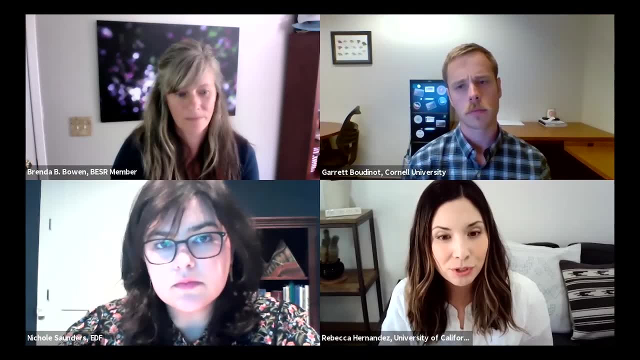 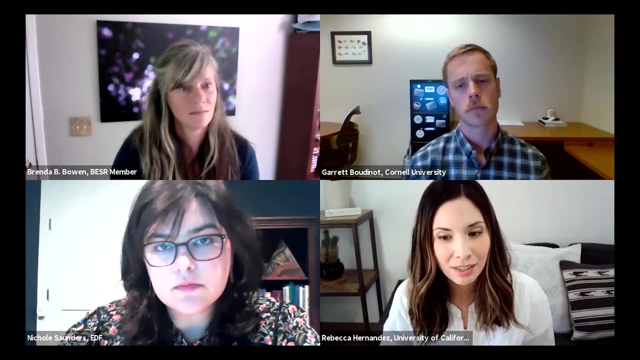 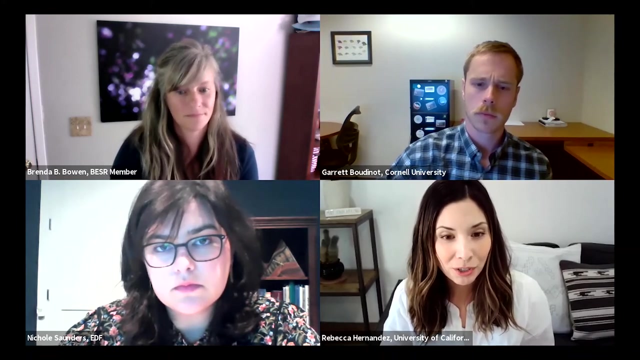 Michelle Magyar- And it it also reduces habitat for wildlife. so you know, what I like to tell Michelle Magyar- folks is that, Michelle Magyar- You know, one of the most impactful things you can do as an individual is to put solar on your rooftop or on your commercial building, because not only are you reducing emissions associated with just the lower CO2.. 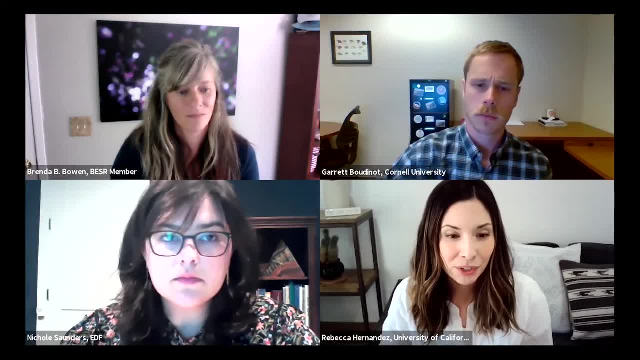 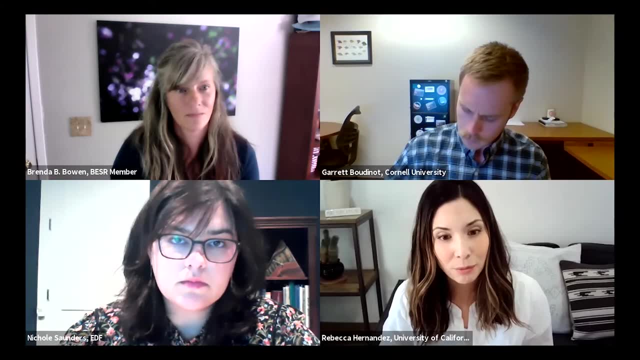 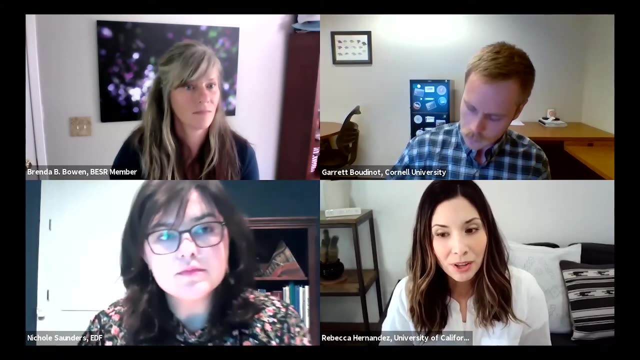 Michelle Magyar- Emissions associated with that technology compared to fossil fuels. you're also reducing emissions associated with the land use and land cover change that, Michelle Magyar- would have otherwise occurred if that renewable energy infrastructure was developed in a, say, natural area. so you know, this is. this is complicated and the 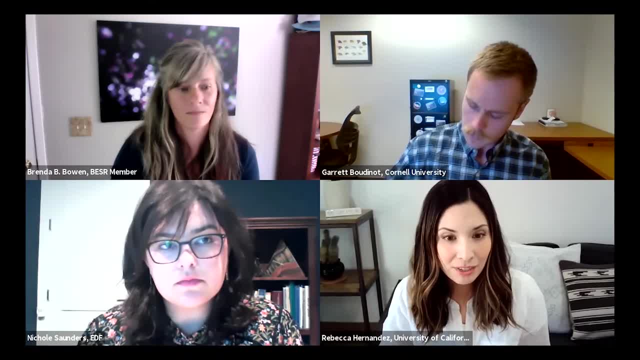 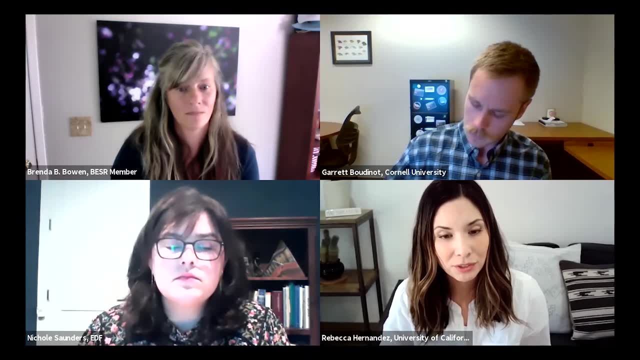 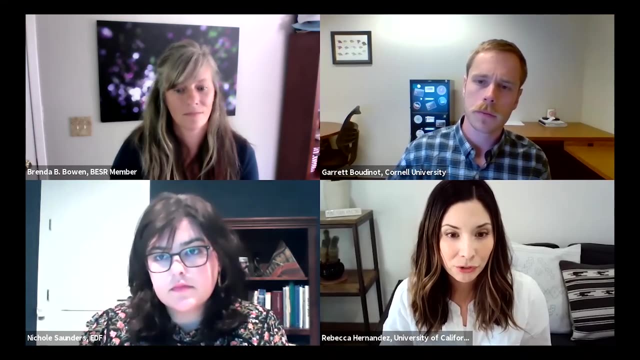 Michelle Magyar- The, like I said, the policies surrounding this understanding in the US today are not- are not well suited to Michelle Magyar- To engender an outcome for Michelle Magyar- A low footprint transition, and I think it's something that we really need to acknowledge and and. 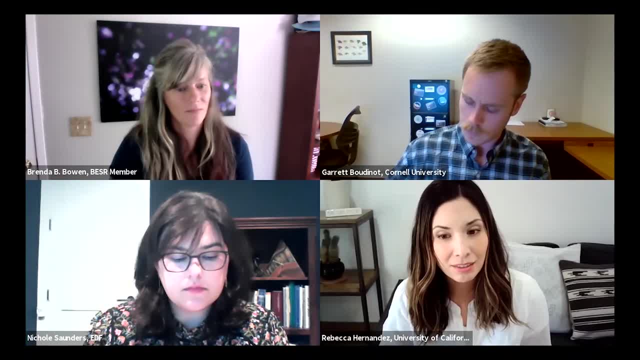 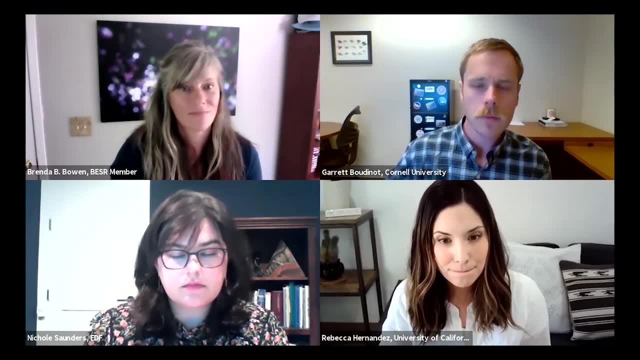 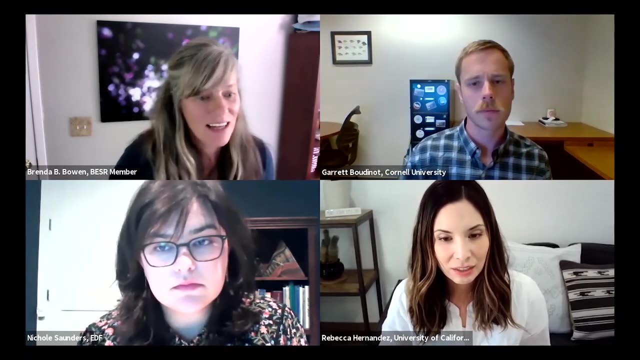 Michelle Magyar- Make sure that we're understanding the the, the consequences of that. Michelle Magyar- Down down down the road. Michelle Magyar- Thank you, Rebecca. Michelle Magyar- i'm going to jump in with a couple of questions from our. 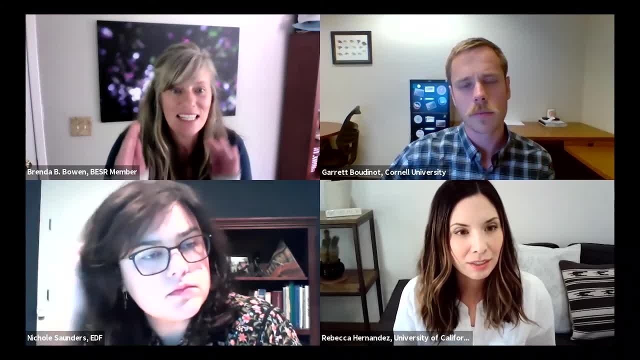 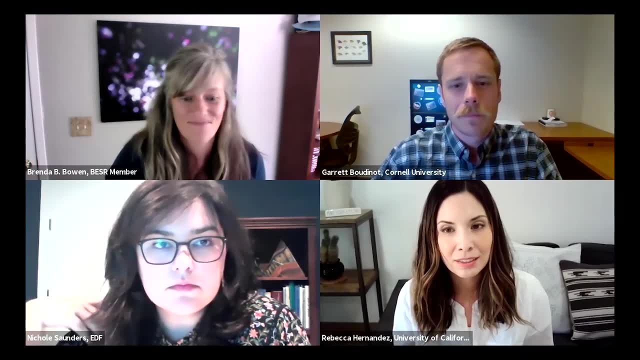 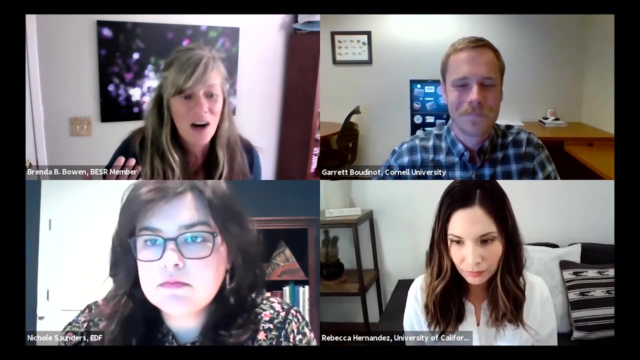 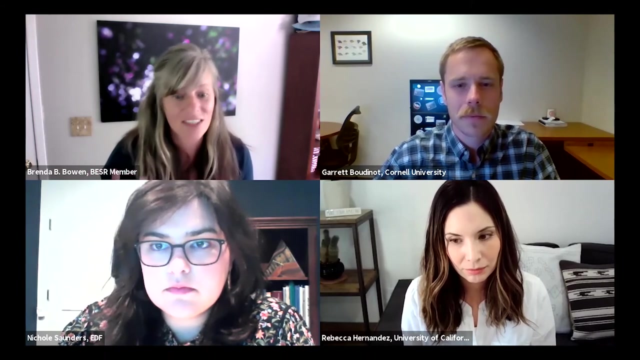 Michelle Magyar- attendees who had had several sort of detail specific questions for for Garrett, about the enhanced rock weathering, Michelle Magyar- Experiments, and so there were. there are a number of them that all sort of go through here. thinking about Michelle Magyar- How does this change the local pH of the soil environment and does that then change the nutrients of the produced crops? 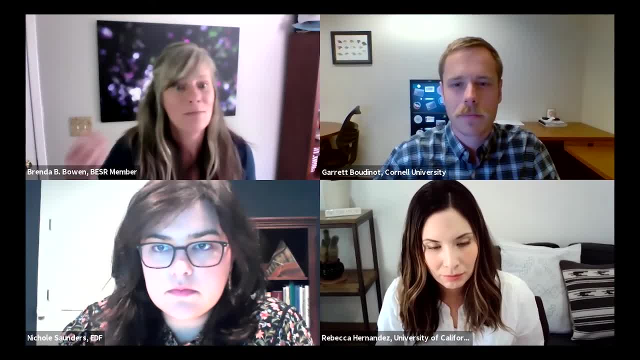 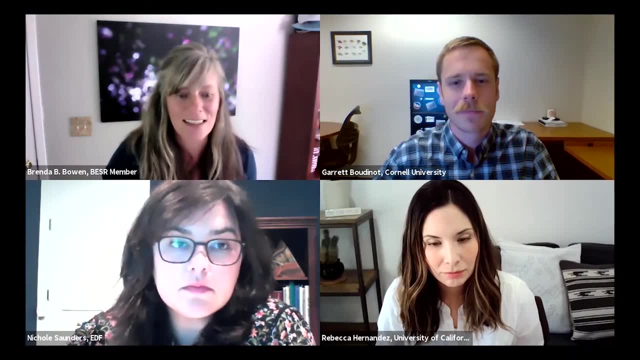 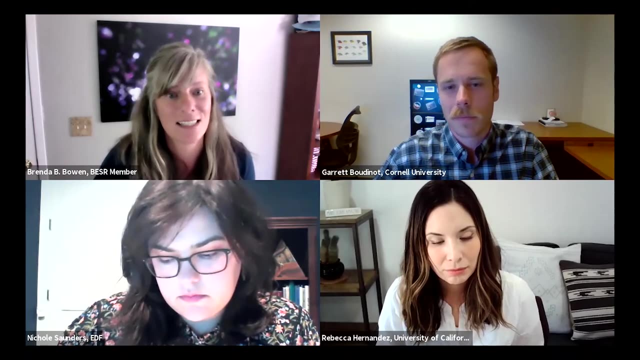 Michelle Magyar- And could that perhaps be a benefit, Michelle Magyar- For some biospecies that are that are being being farms and things like that. so those are sort of the first set of questions around around how it changes the pH, and perhaps there are- there are crops that could benefit from some of these, these enhanced weathering reactions. 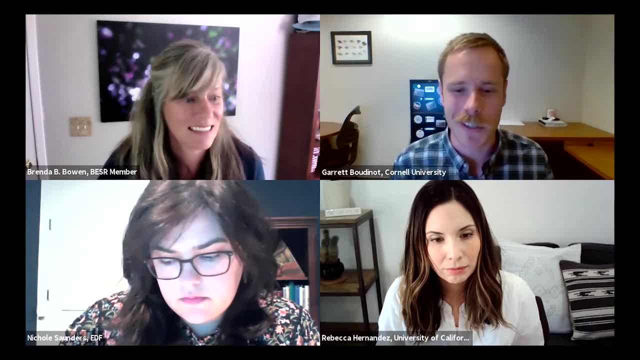 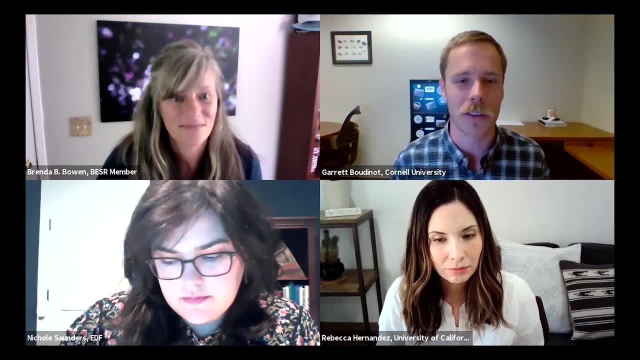 Garrett-. yeah, thanks for for bringing those up, Brenda. I saw those questions in the Q amp a and was really excited to see those- Garrett- have a chance to get in the weeds on how enhanced weathering works, Garrett- And I think those 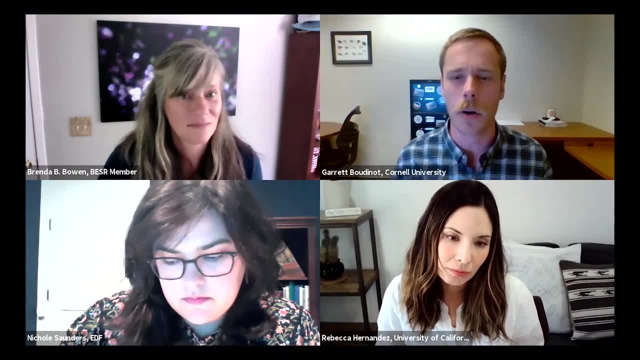 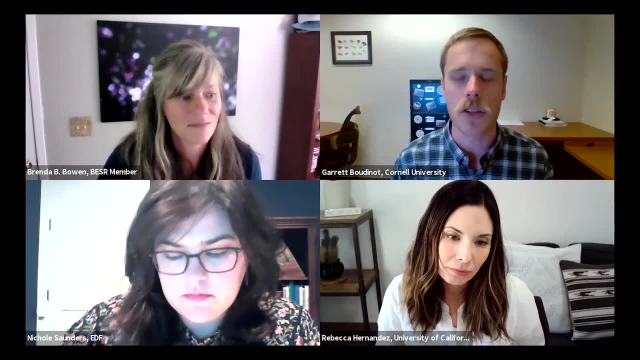 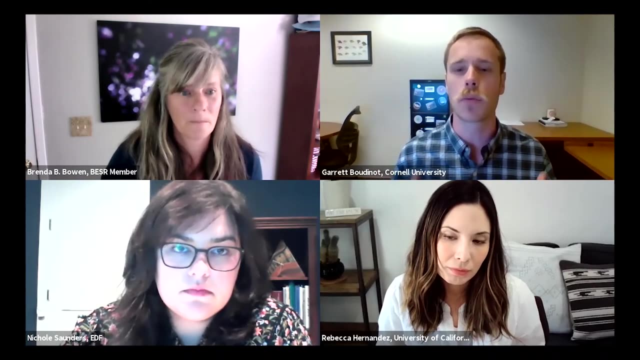 Garrett- Questions are spot on and to provide a little bit more detail of the chemistry behind enhanced weathering, it's actually based on a change in soil pH, Garrett- And so as those magnesium and calcium rich silicate rocks dissolve, they're releasing those positively charged magnesium or calcium ions. Garrett- What that does is that shifts the charge balance of the soil, poor waters changes the way that hydrogen species, Garrett- And ultimately it increases the pH. so that one one question hit the nail on the head: it does increase the pH of the soil and from an agronomic perspective that's actually really advantageous. so a lot of the world soils are actually over acidic. Garrett- And when soils are very acidic, it means that nutrients are more likely to leach away from the soils and it increases the bioavailability of toxic metals. Garrett- And so any strategy that we can use to increase the pH of soils actually has a number of benefits for overall agronomy, including. 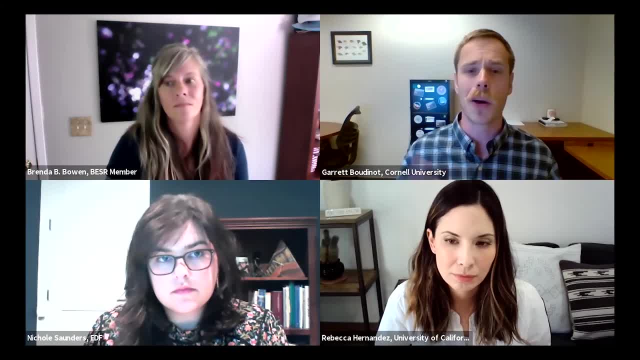 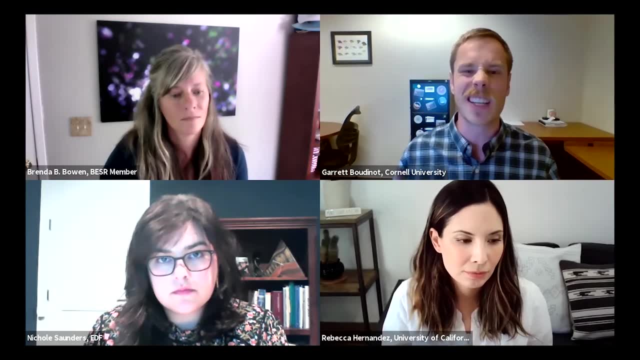 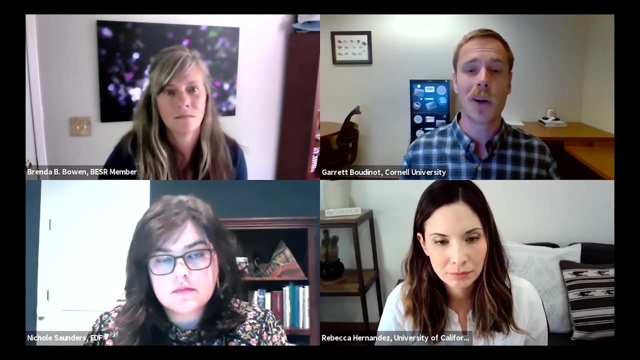 Garrett- Improved nutrient retention, and so there's a number of soils, particularly in the tropical regions of the of the planet, where soil productivity is limited- Garrett- Because of the acidity, and so if we could deploy enhanced weathering and some of those areas, we would have incredible benefits for soil. 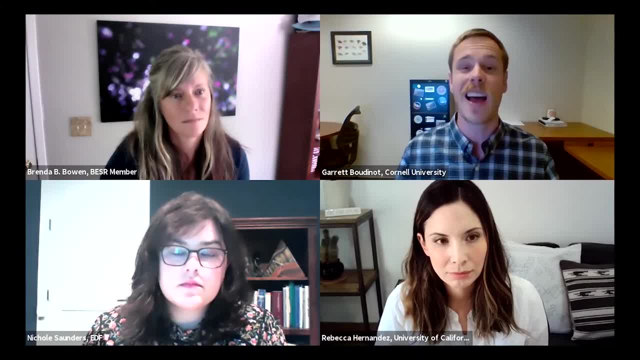 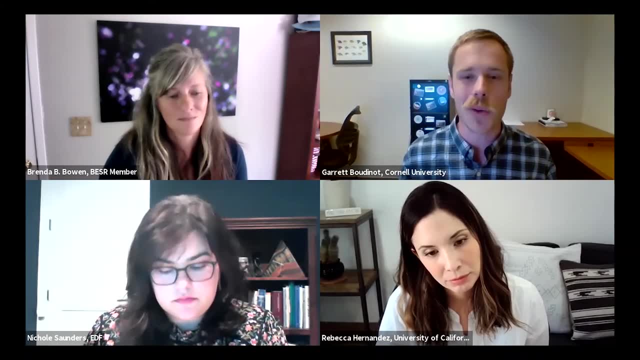 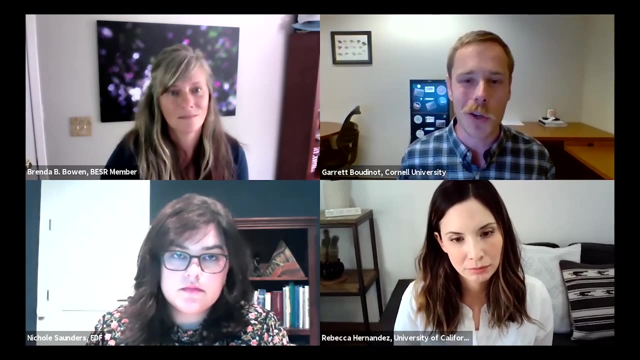 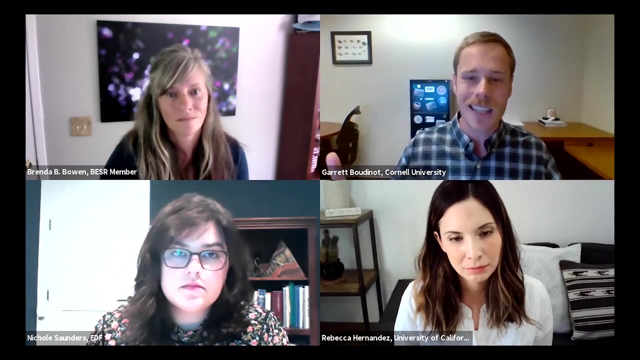 Garrett- Health, and thus human health, human nutrition, as well as mitigating global climate change. Garrett- And farmers already use one practice that's very similar to enhanced weathering to increase the pH, and that's called liming. they add calcium carbonate- Garrett- To soils to do that same thing: increase the pH. unfortunately, when it's a calcium carbonate, that process releases CO2. so when we replace that with a calcium silicate, it reverses the 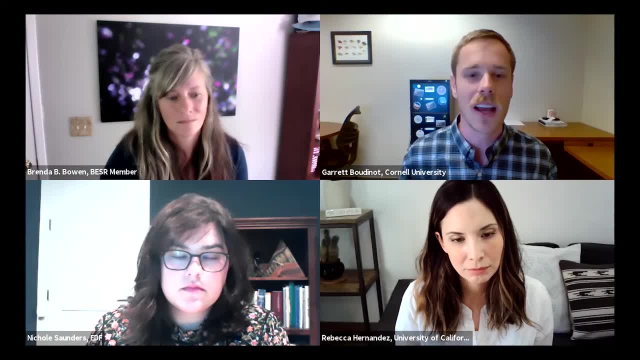 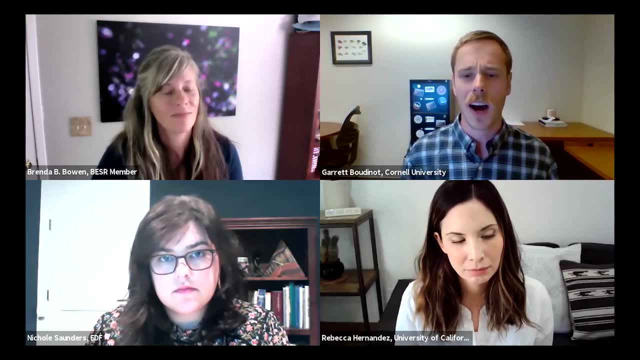 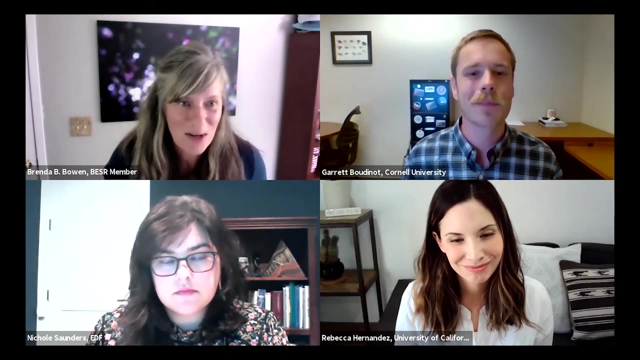 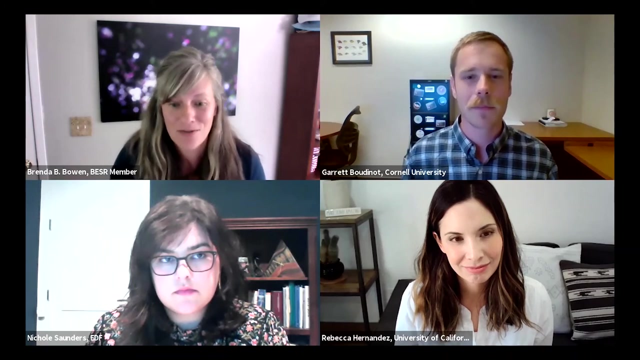 Garrett- The direction of carbon speciation and encourages that by carbonate production that draws down CO2. so that was a great question and, and hopefully Brenda did that, answer the big one there. Brenda Becker- yeah, there's a couple more details i'll follow up with here. there was a question about will. has coal ash been tried as a potential source for that and do does this perhaps? 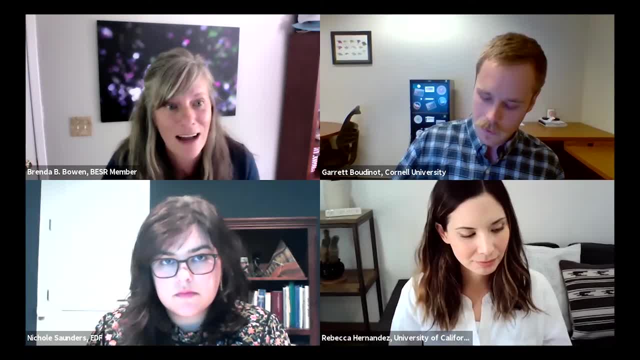 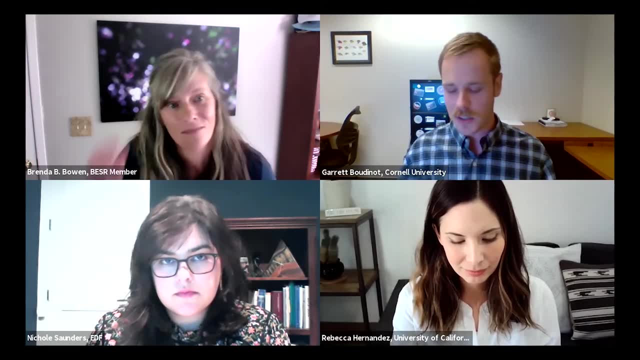 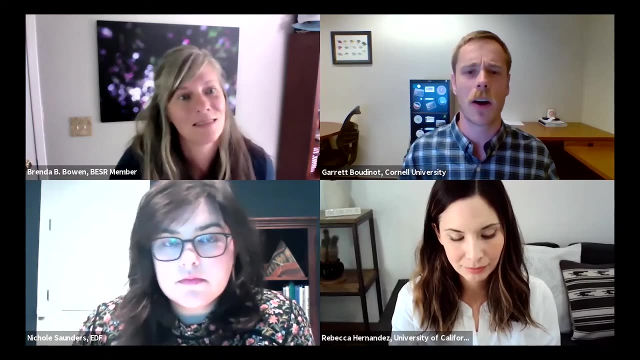 Brenda Becker- change calcification. Brenda Becker- In the soil over time, you know this, this change in pH and these changed reactions. Garrett- yeah, great questions. and kind of gets the front end and the back end of enhanced weathering. so I, yeah, I saw the coal ash question. I also saw someone asked about potentially using mine tailings. 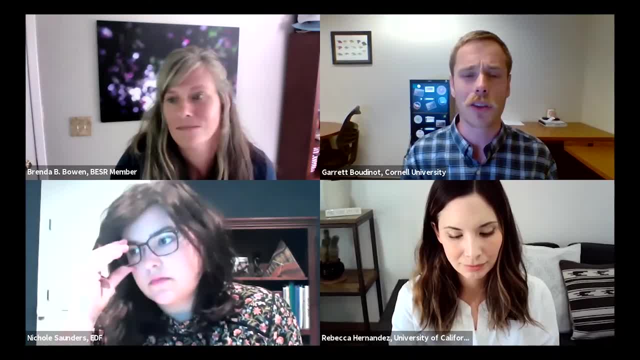 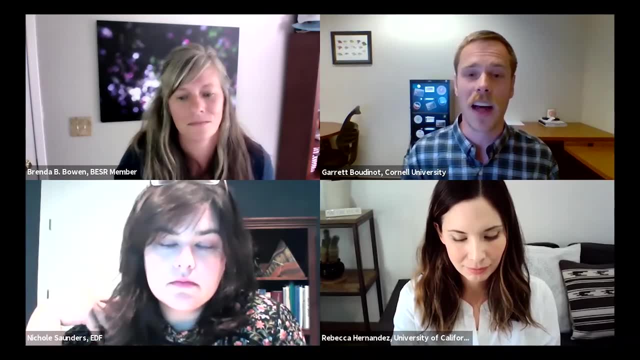 Garrett- As a source and those are spot on. so actually a lot of the rock dust that we're already using and deploying in the field are byproducts of mining Garrett- That are already ground to a really good particle size for this process and they have that ideal chemistry. 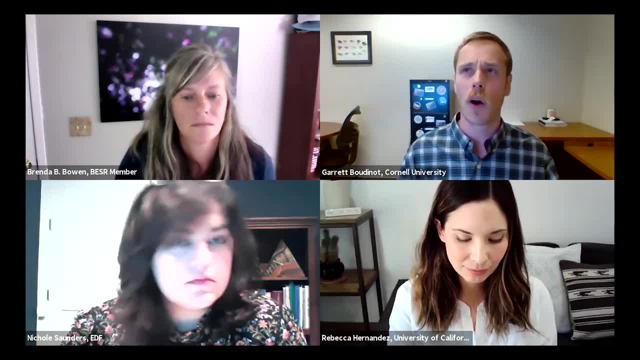 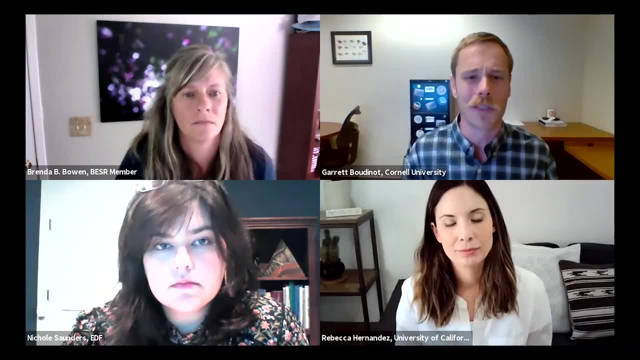 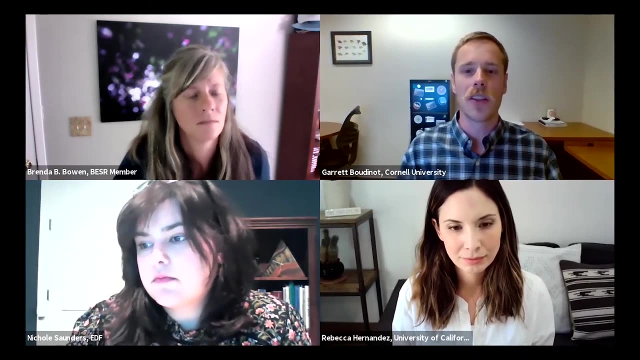 Garrett- And you know thinking about how can we address resource priorities and mitigate climate change while also reducing adverse environmental impacts, kind of the goal of this panel, that's, you know, in enhanced weathering is at the intersection of all of those goals, because the the global mining industry, 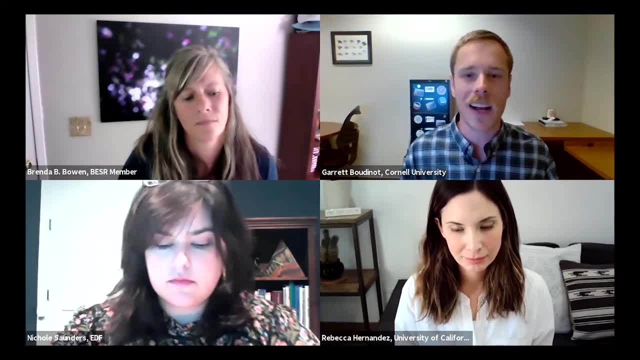 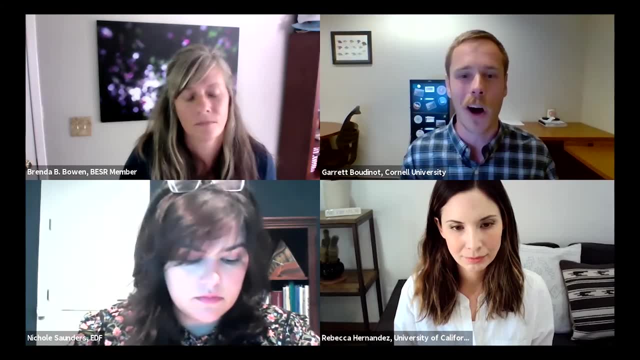 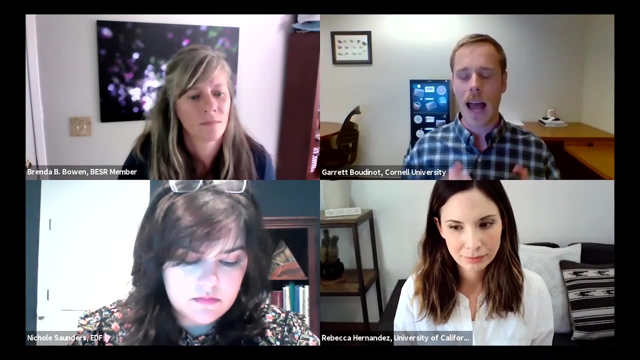 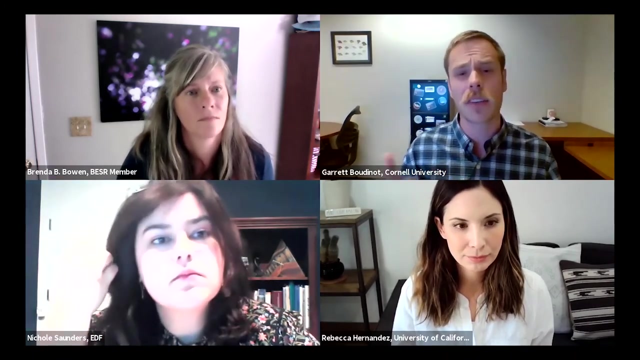 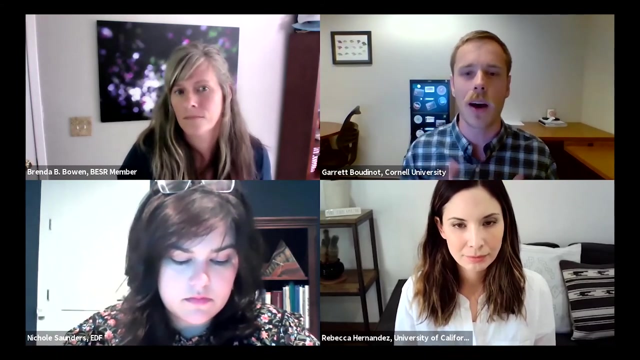 Garrett- produces an enormous amount Garrett- Of waste that we're finding has the ideal chemistry to be deployed not only to minimize environmental quality negative impacts, but actually have positive impacts on the global climate. so, Garrett- Absolutely. there are other industrial waste products- coal, ash, cement, kiln dust, things- that also have calcium, magnesium and an ideal chemistry for enhanced weathering. but what's important with a lot of these materials is that we not only 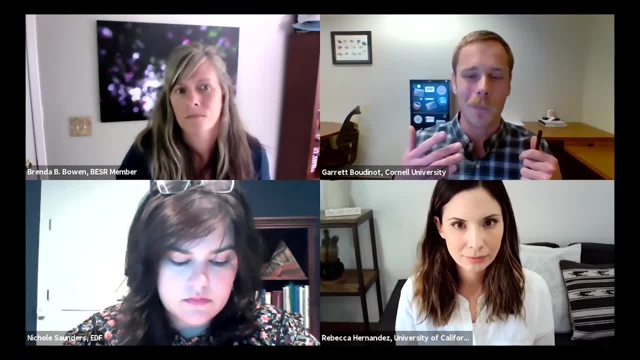 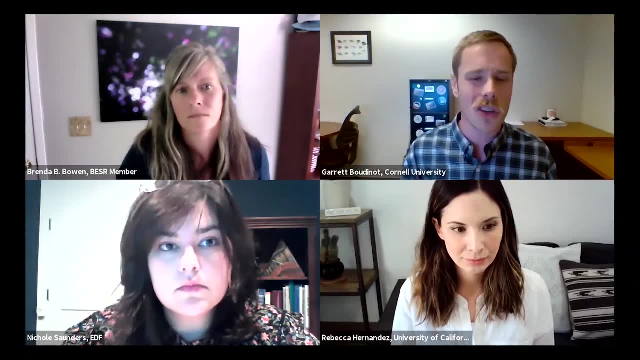 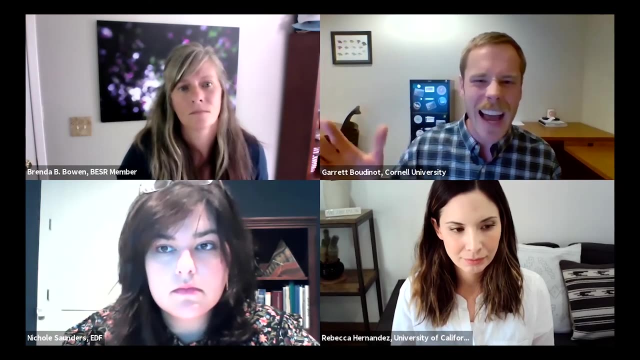 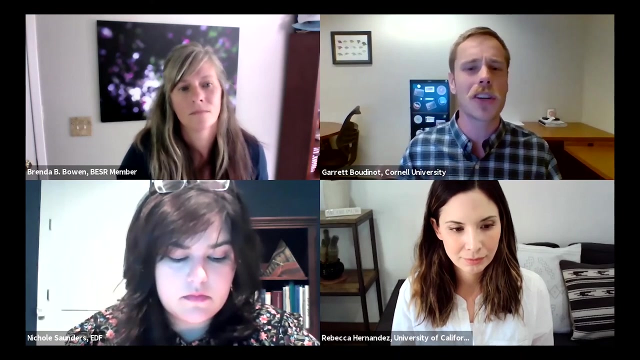 Garrett- think of what's the calcium and magnesium, those those Garrett- positively charged ions that drive enhanced weathering, but also what's the concentration of potentially harmful trace elements, trace metals, and so, Garrett- In the literature you'll see some really high estimates of how much carbon dioxide enhanced weathering can bring down, and then you'll see the material they chose was something that also has high levels of chromium and nickel and things. 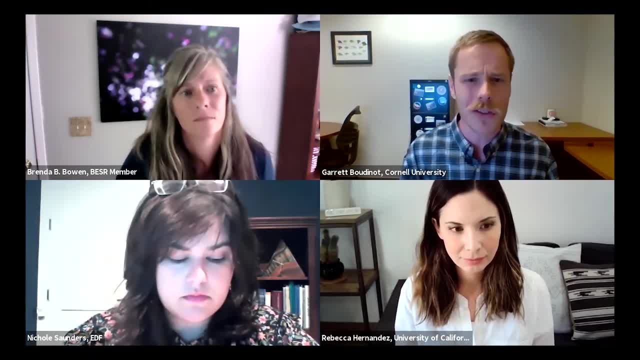 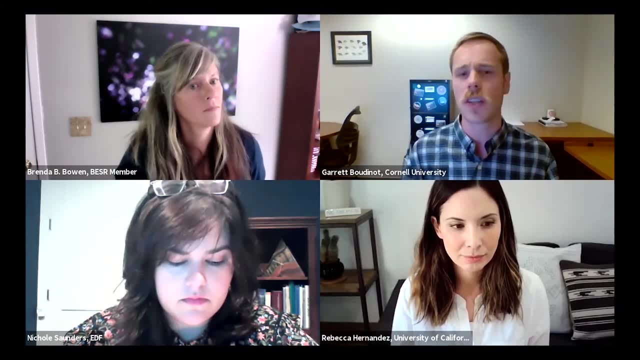 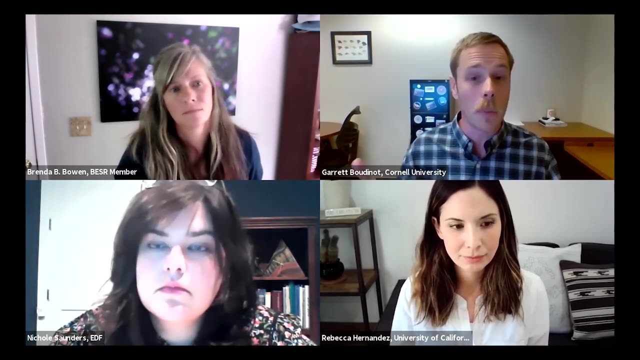 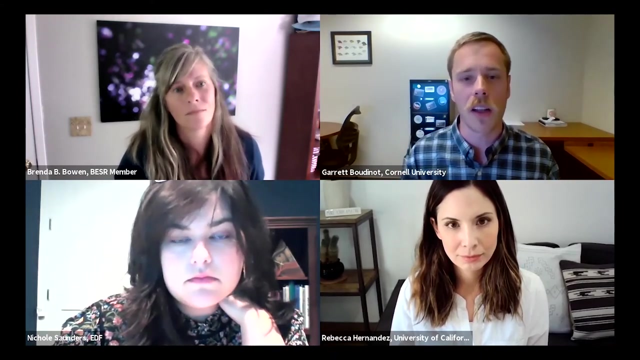 Garrett- That we really wouldn't want in our global agricultural soils, and so this goes into- I mean, life cycle analysis has been used a number of times today. this definitely goes into that life cycle assessment, Garrett-, of enhanced weathering, of what are the costs in terms of the availability of materials and their potential negative impacts on soils. but then what are the benefits that we could have for the climate and when we know that there are plenty of materials available? 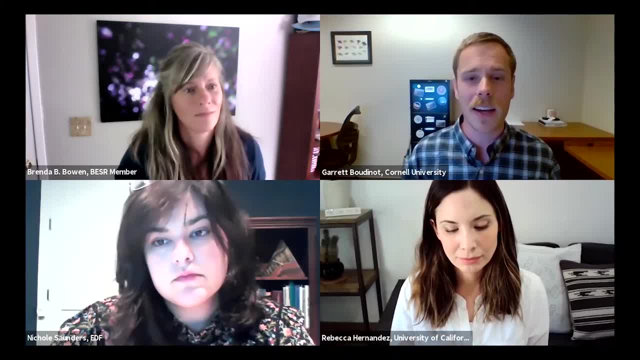 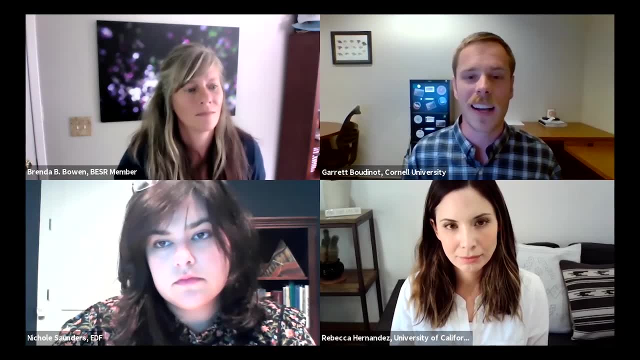 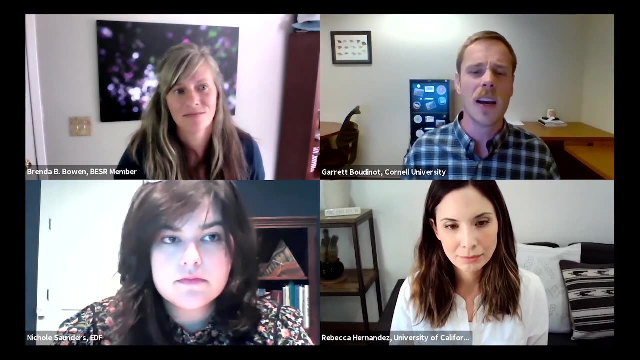 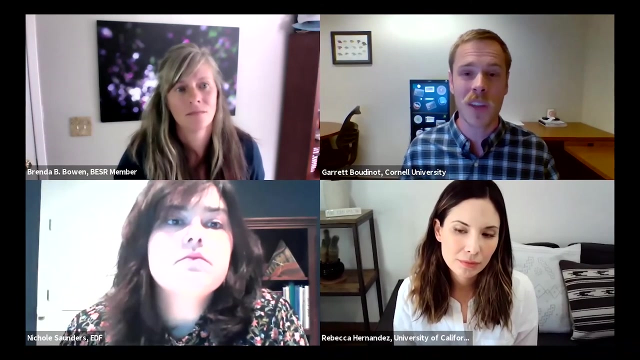 Garrett- that don't have those negative Garrett- impacts from chromium and nickel and other heavy metals but can provide the ideal chemistry for enhanced weathering- just to put numbers on it, if that helps Garrett-. So some studies have have suggested that globally we need somewhere around 10 to 30 billion tons of rock material for global enhanced weathering. there's over 40 billion tons of existing mine. 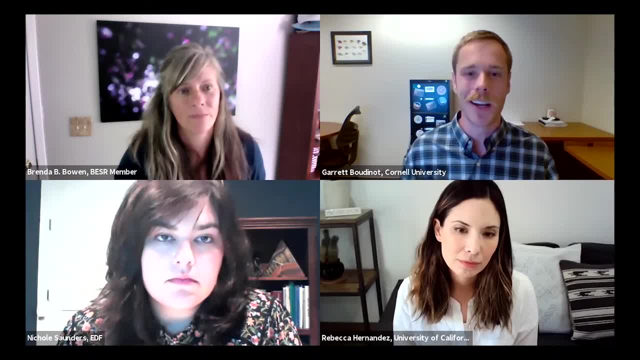 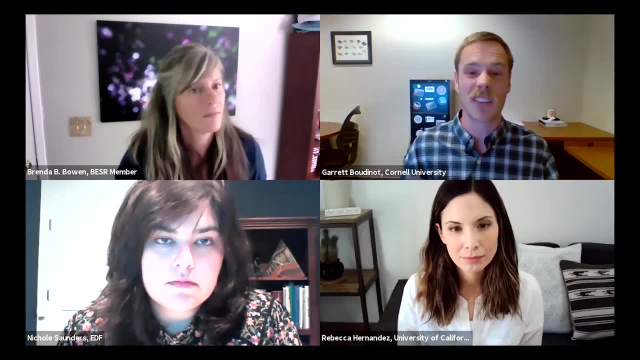 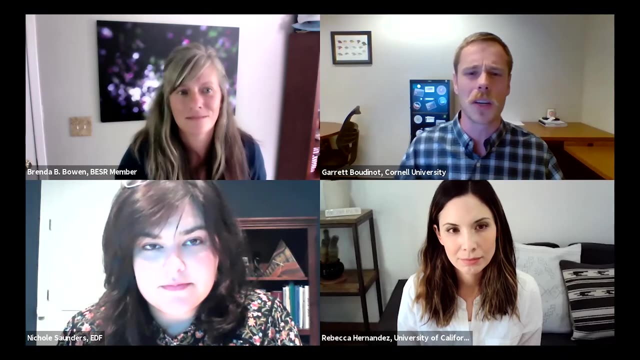 Garrett- tailings. Garrett- Just from metal and or in the US alone. so the US has tons of material just sitting around waiting to be used for a process like this, and again it could have a lot of benefits, Garrett- Briefly i'll mention that calcification- because that that can be confusing- been talked about by carbonate. then, going to carbonate, 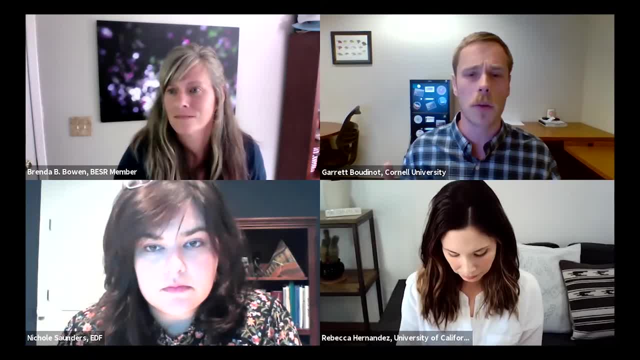 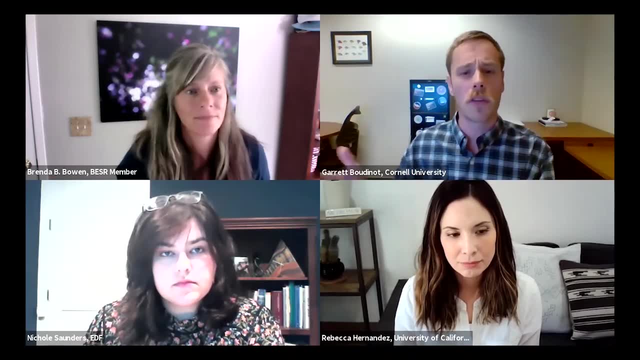 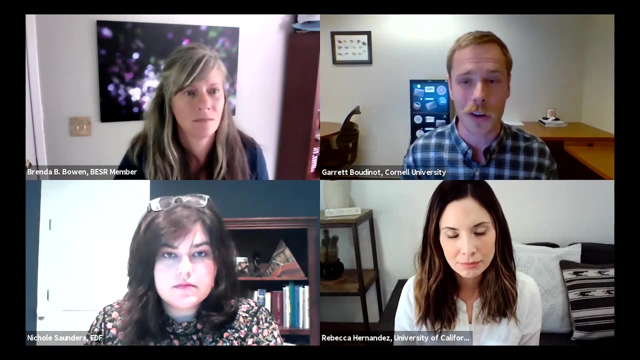 Garrett- What we're finding is that in a lot of soils, the majority of carbon, or the majority of the fate of carbon from enhanced weathering, is actually by carbonate, Garrett- And the overall fate of that is to the oceans, where in the oceans, it might either buffer ocean acidification- another really important climate benefit of enhanced weathering- or precipitate eventually into calcium carbonate. 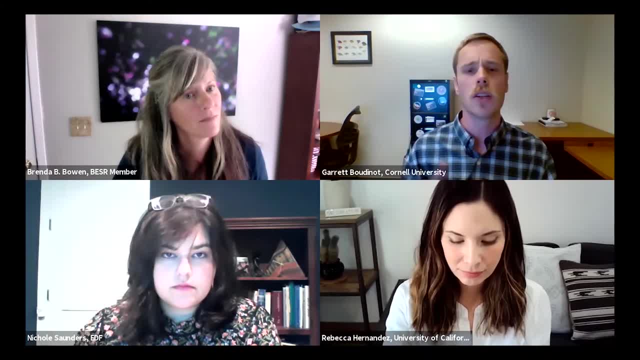 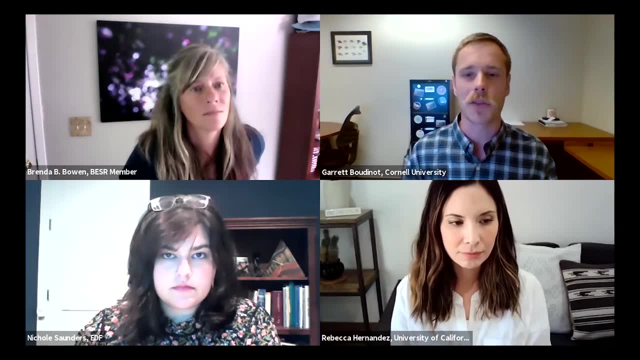 Garrett- So certainly it can happen in soils and it depends on the soil physical structure, soil pH and climate. but we're not seeing negative impacts from soil calcification. and again, primarily we're seeing Garrett- So certainly it can happen in soils and it depends on the soil physical structure, soil pH and climate. but we're not seeing negative impacts from soil calcification and again, primarily we're seeing 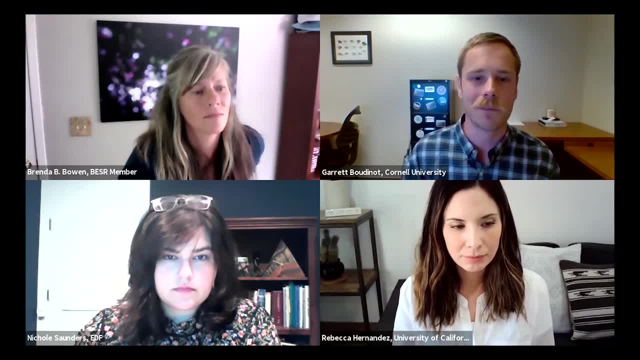 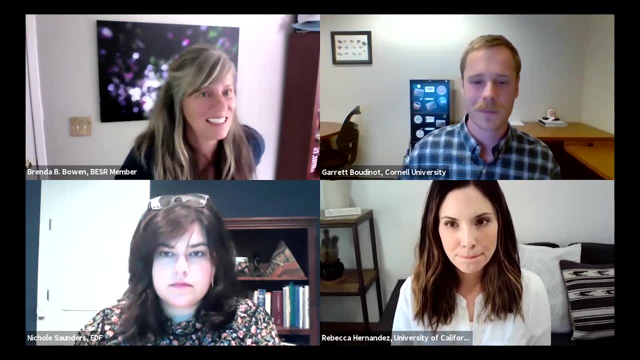 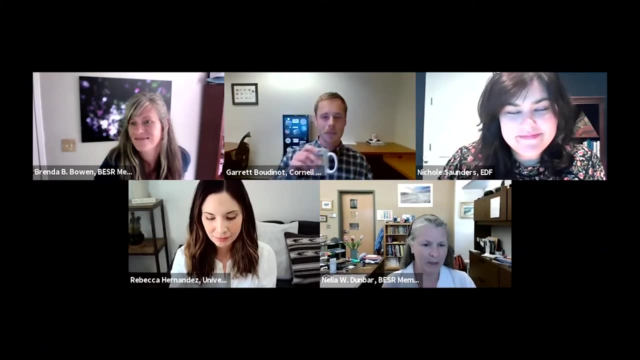 Garrett- Even having further positive climate impacts in the ocean. Thank you, Amelia, let's go to your question. Okay, thanks, so so my questions for Nicole and Nicole. i'm based in New Mexico, so of course, produced water is something I think about a lot. 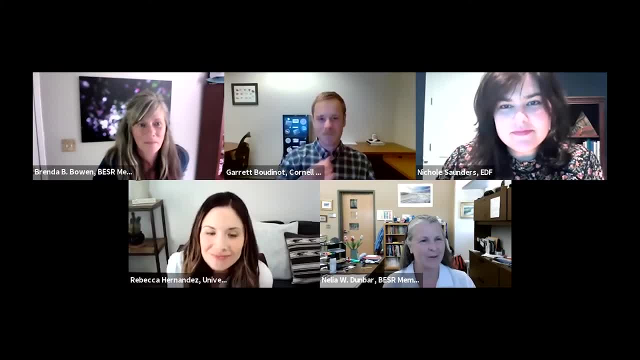 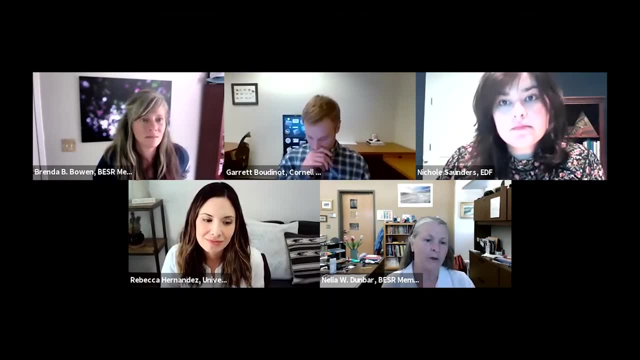 And I really enjoyed your talk and one of the things that kind of caught my attention that I hadn't really thought about before Is when you mentioned the, The, The, The Geochemical variability in composition of produced water regionally across the United States, and it made me realize that I probably need to start thinking about in New Mexico whether Permian Basin produced water is geochemically different than San Juan Basin. 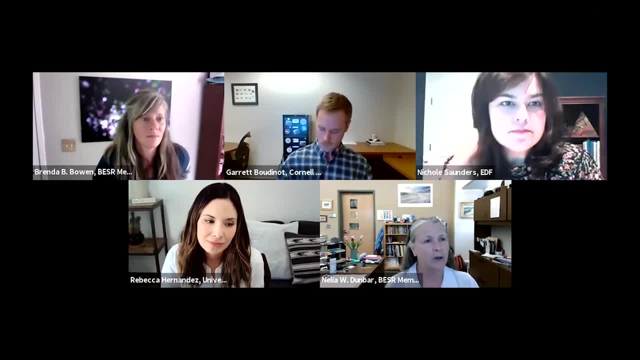 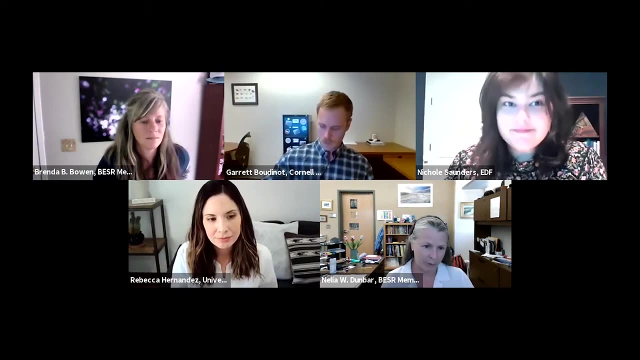 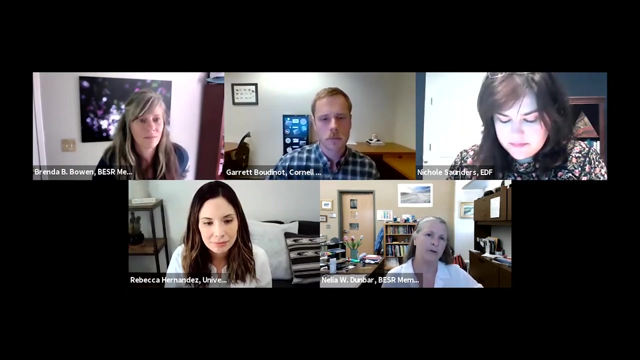 So i'm curious just to delve into that a little bit more, and the questions I had are: i'm assuming that, depending on the- you know the unit that the produce water is coming from, even within one region, you may May get variability and produced water and i'm curious about how the regional variability across the USA would vary compared to. 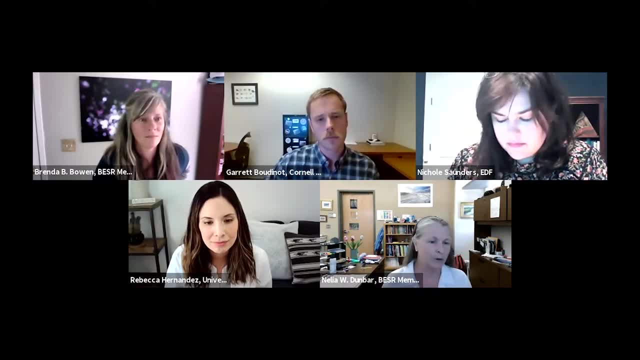 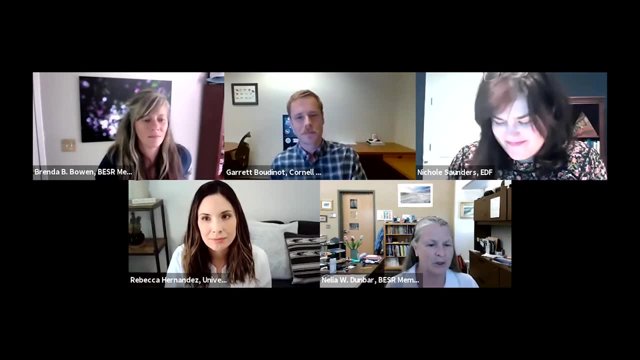 The geochemical variation and produce water within, say, New Mexico. and then also, it's kind of a big question if you could just point me in the direction of a place where I could discover some of that for myself, that would be great, Great question. and so the first thing is that I wanted 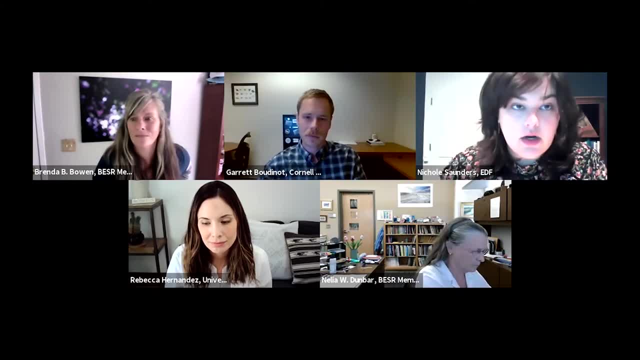 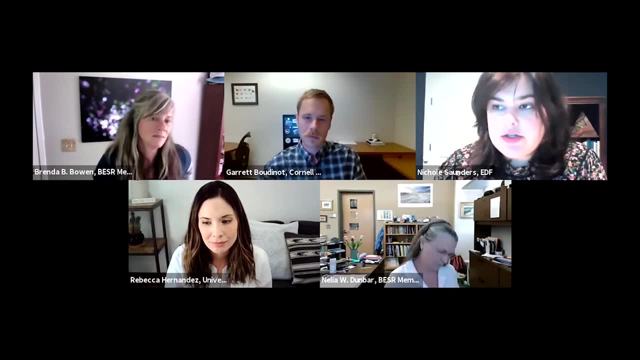 The scientists on staff. that actually was the author of one of our publications. her name is Dr Cole Danforth. we have partnered with a couple of different researchers and there is- There is- there's probably some research that's really interesting to you. that would have been done on DJ basin water in Colorado, but their findings could raise some questions that may be something that you'd want to look at on New Mexico waters generally. 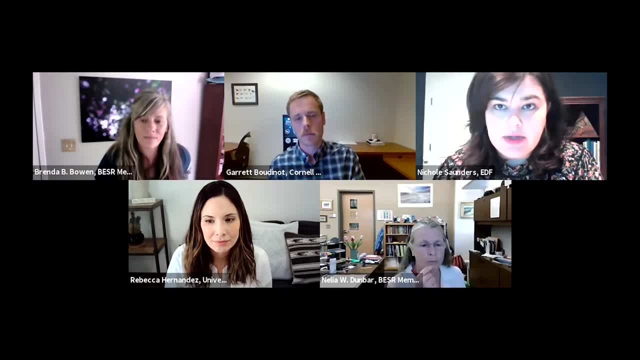 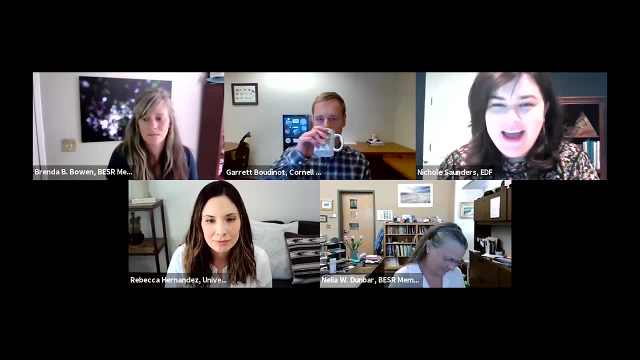 And I want. I will get you those paper citations. if you want to shoot me an email, i'm happy to actually send you the links to those rather than name them off the top of my head on a panel today. i'm not that good. And then the second question. I think you're. it's really spot on and you know it's hard to say we haven't done a comprehensive. 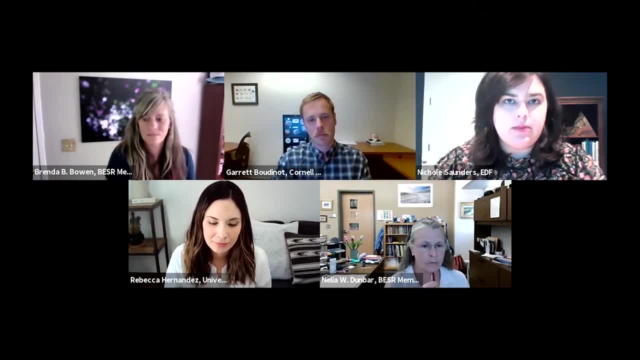 comparison. there are definitely some generalizations you can make, for example about the total dissolved solids that you might see from region to region. But I think that you will see, Even within New Mexico, the San Juan versus the Permian and even within the Permian, the Delaware versus the Midland, sub basins having very different. 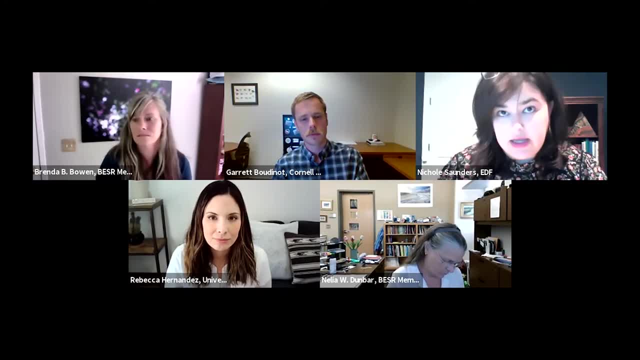 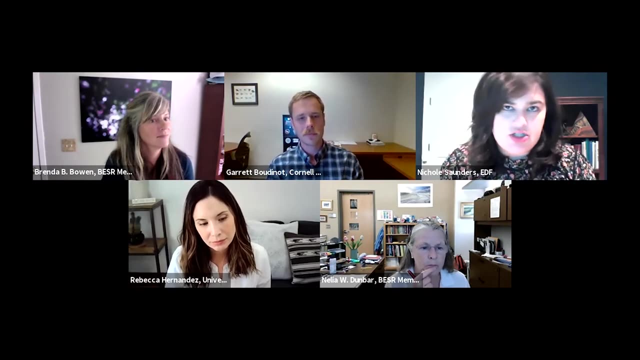 Produced waters. that will impact what we're targeting from a treatment system and what we're looking for in our regulatory system. and that's really challenging it because there's just not a lot of comprehensive, you know, using research, advanced research methods, more than just. 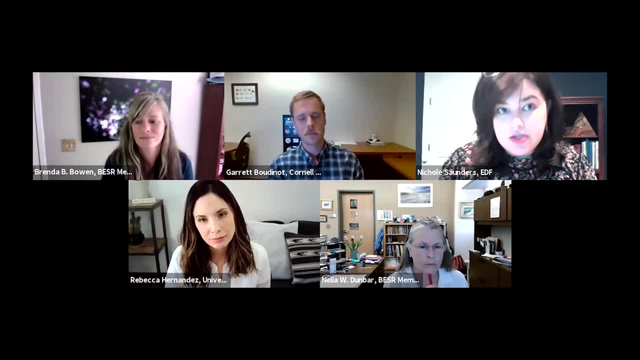 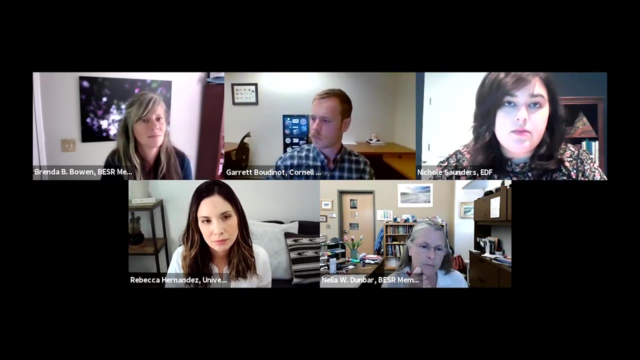 GCMS, More advanced non targeted analysis to characterize those waters. there's not a ton of that done on New Mexico water. same goes in in Texas, where we're also thinking about these questions, where I am. So so you do want to look region to region, and then we've also. there are also some really interesting studies that look. 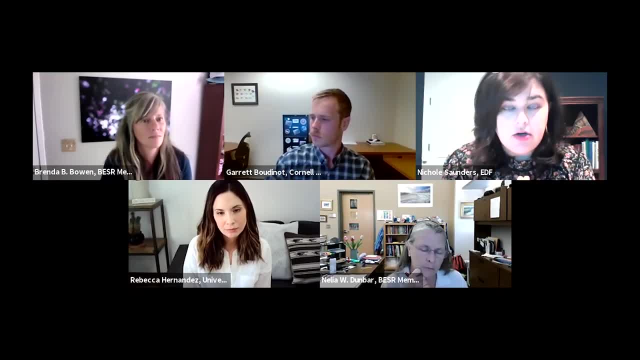 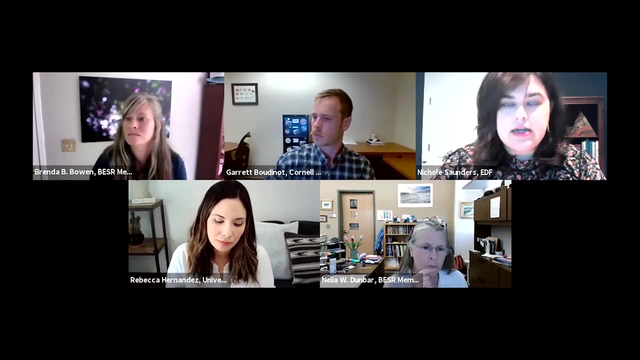 Over the lifespan of a well alone. so even if you take the geographical or geological considerations out of the picture and look at time alone, From day one where You've completed a well, obviously you're getting flow back and more fluids that you're using and chemicals you're using in that initial fracturing operation. but beyond that, when you look- 30, 60, 300, 900 days. 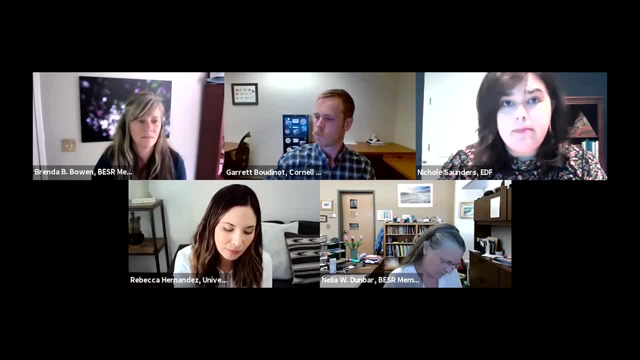 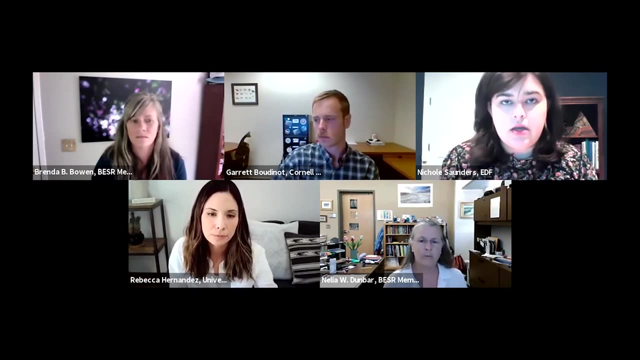 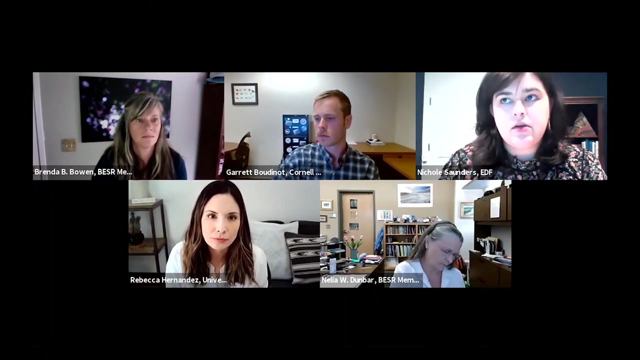 You do see some very interesting and impactful variation. so when we talk about reusing produce water in any given context, you know there's a lot of generalization about that term, but we really need to understand what specifically are we talking. Are we talking about day 30- produce water? are we talking about day 600? maybe the TDS changes, maybe trace organics change in a really important way, maybe a certain well has been. 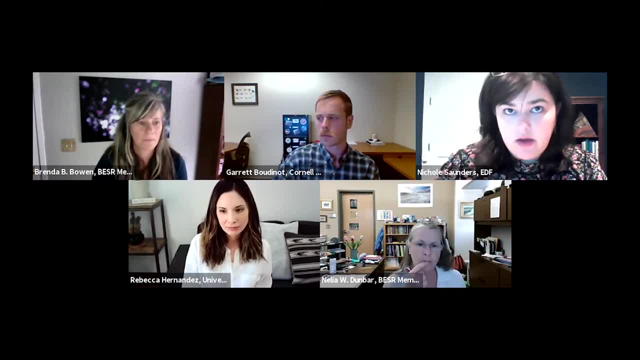 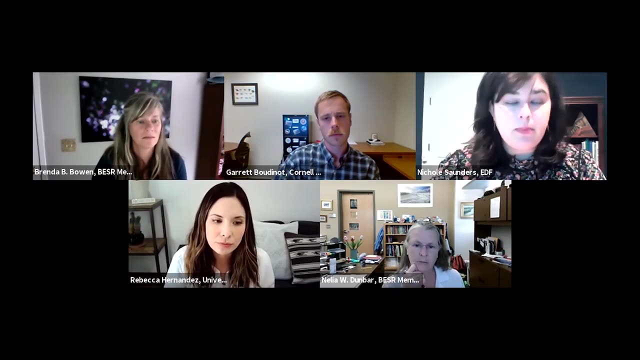 Up. you know they might have done maintenance on a well, they might have done some kind of operation on a well. the what was utilized in that process There could come back and show up in that produce water and if there's not a lot of conversation at the front end that we're expecting that or we're knowing we're going to see it, we may not be. 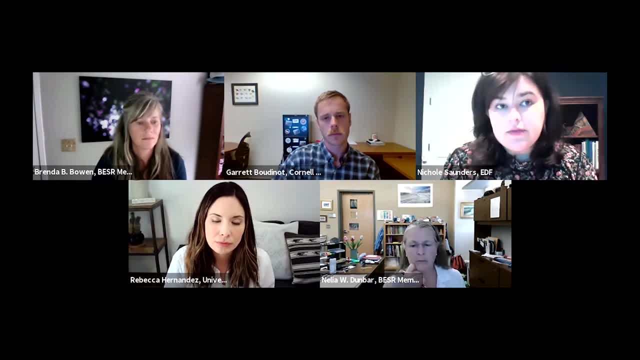 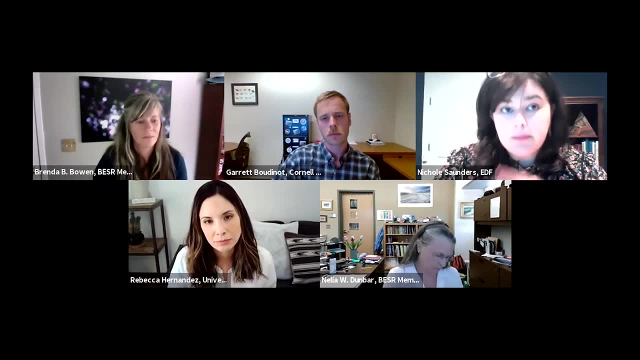 Prepared for that in the treatment receiver. so there's a lot of different things to consider back when it comes to the variability component, when when you think about developing reuse programs- and please don't forget to email me, i'm happy to make sure I get you whatever papers I know about. 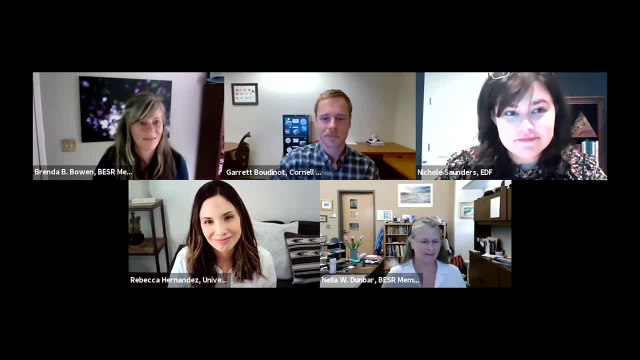 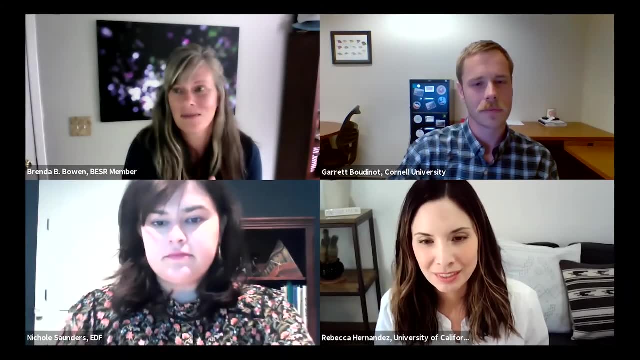 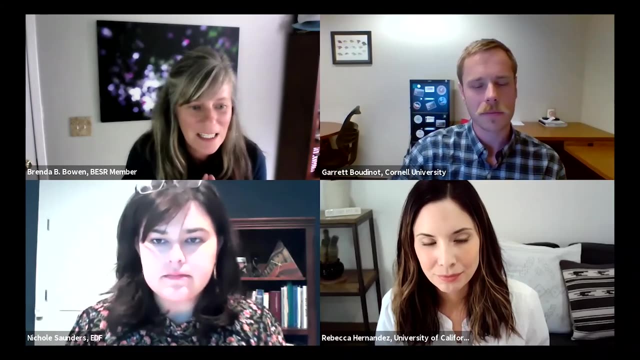 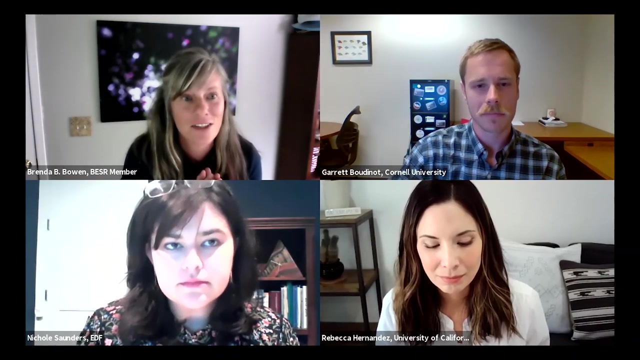 Great thanks a lot. I really appreciate your comments, sure Great. Thank you, Amelia and Nicole. here's another question from our from our participants for for Garrett, About sort of a sighting. so mine sites are often not around agricultural fields, so what are the transportation limits to truck the crushed rock to the agricultural land? 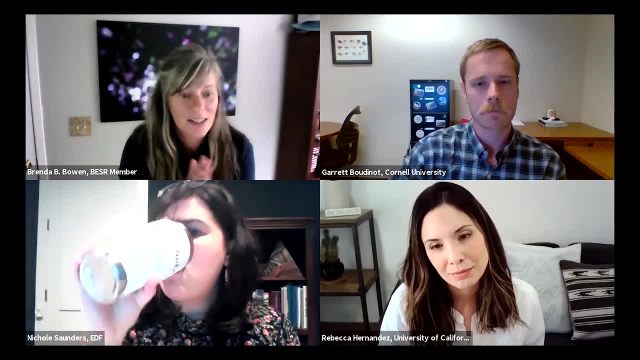 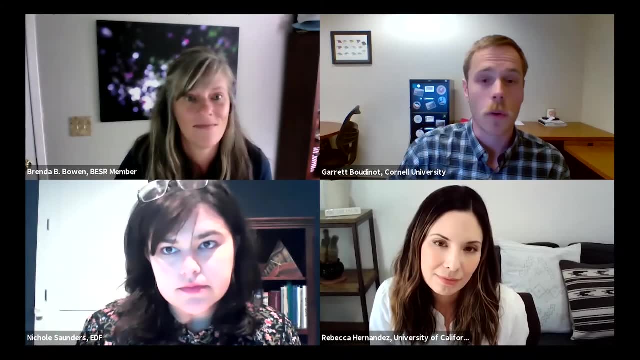 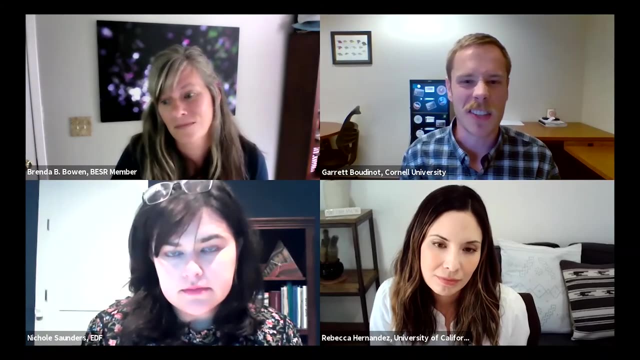 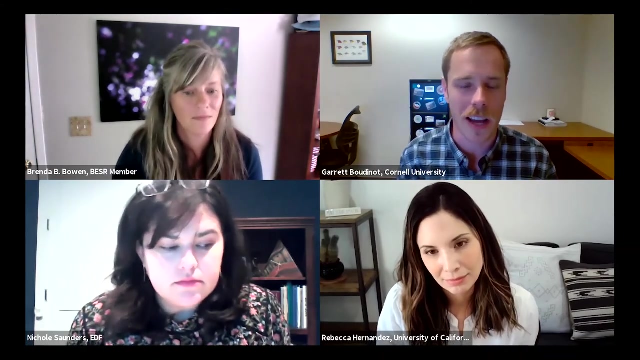 Does it have to be sort of large scale enough to see those significant impacts of carbon sequestration? and how does transportation link into that Great question? um, there are a surprisingly large number Of existing mine operations that do have a lot of the ideal chemistry for enhanced weathering across the country and across the globe. 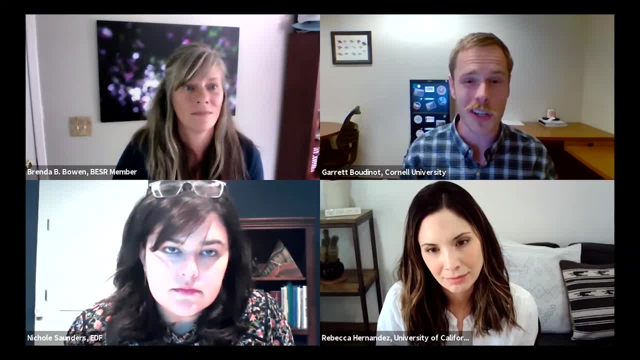 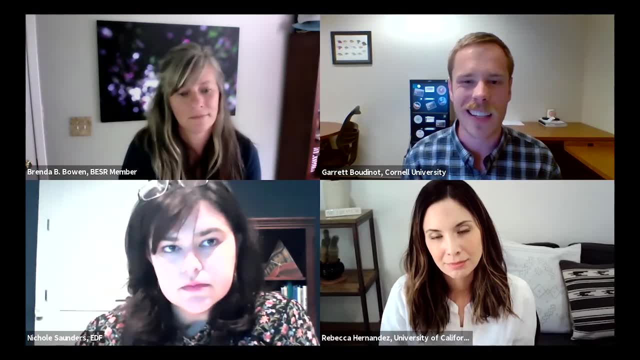 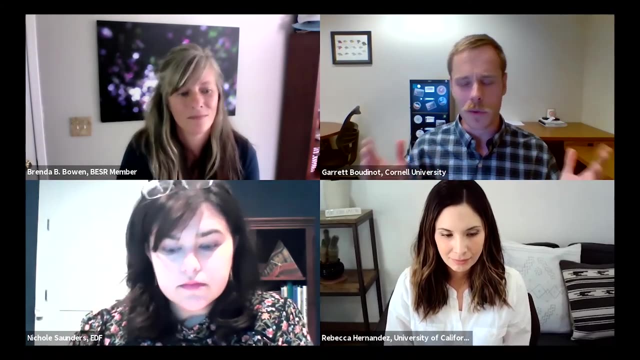 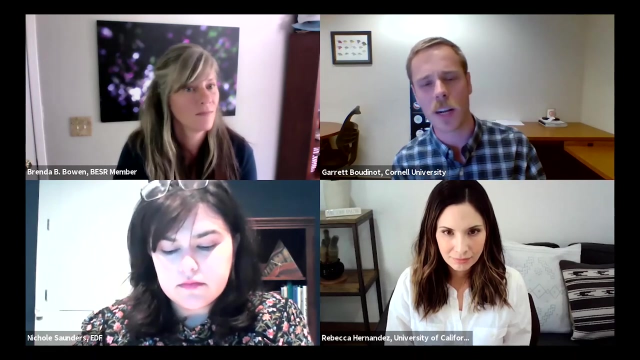 And so we're not thinking about having to ship things across the country to reach on the, the ideal farm candidates, although certainly shipping is something that needs to be done and needs to be optimized and commercially viable And, and you know when, when you mentioned the scale of the, the farm or the size of the farm, if that matters, one of the things we're really excited about with enhanced Enhanced weathering is its ability to scale to all farm sizes, so this isn't something that only large farm operations would be able to take advantage of. if you've got the equipment to apply fertilizer Or a line to your to your croplands, you can take advantage of. 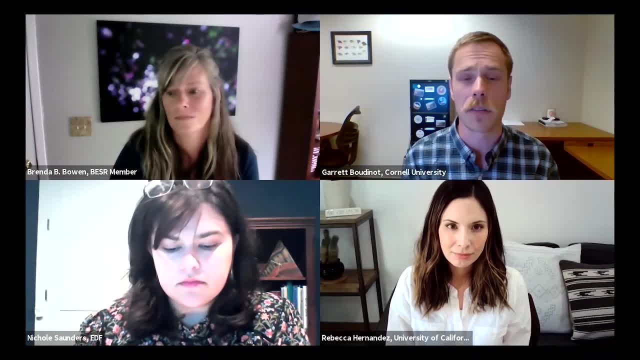 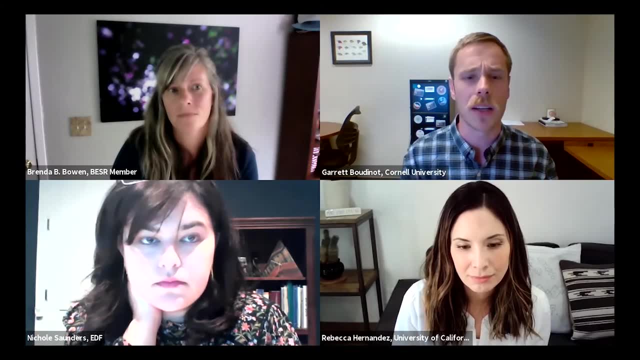 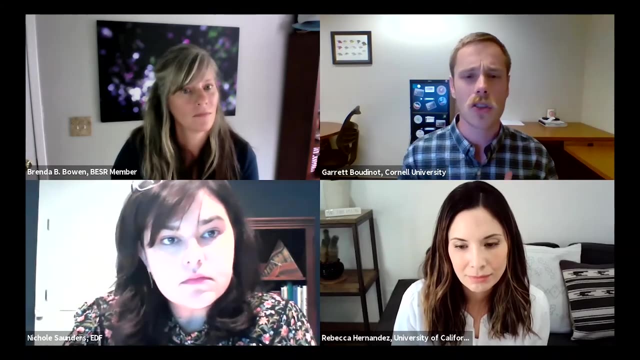 Enhanced weathering, get those agronomic and carbon benefits. but Ben alluded to this whole process a little bit When he mentioned the costs as something that needs to be optimized and is currently a barrier, And so for a lot- and it gets to this question- that's certainly the cost of transporting the materials, of acquiring and transporting the materials. 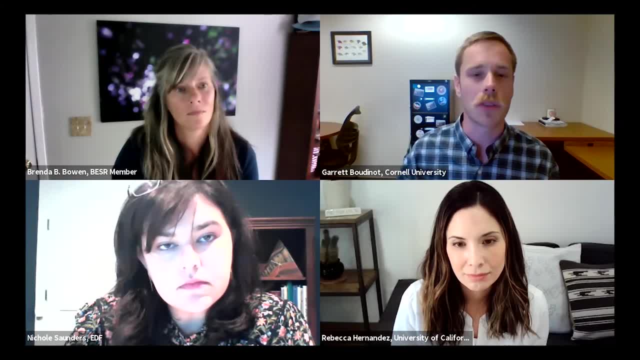 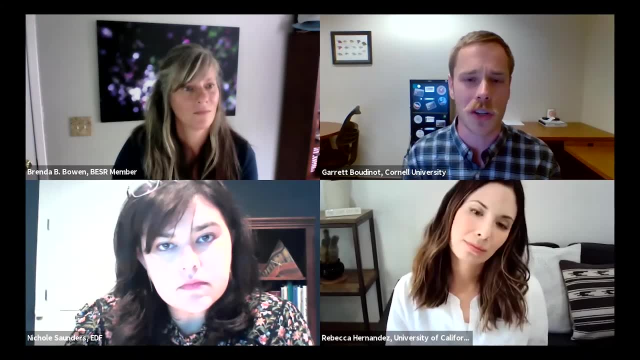 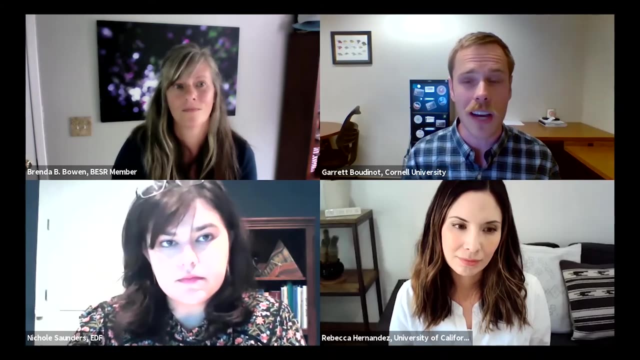 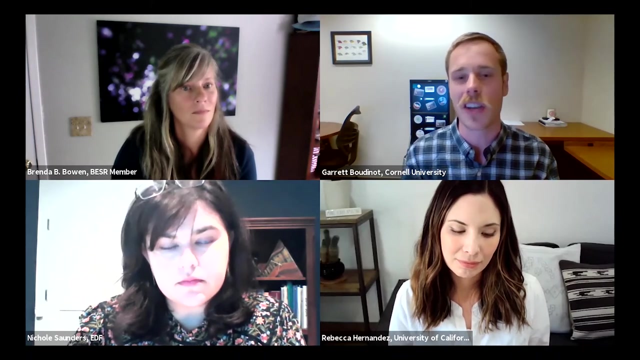 Do need to be offset by the cost of the carbon credits that the farmers might get. So we're really excited about enhanced weathering and other carbon sequestration and cropland options As a way to increase the economic viability of america's agricultural sector. but the economic benefits from carbon sequestration need to match the necessary inputs. 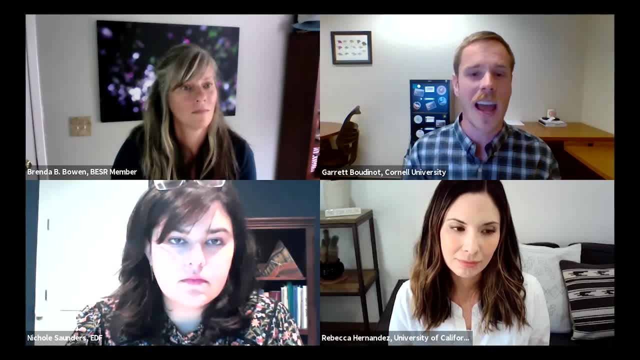 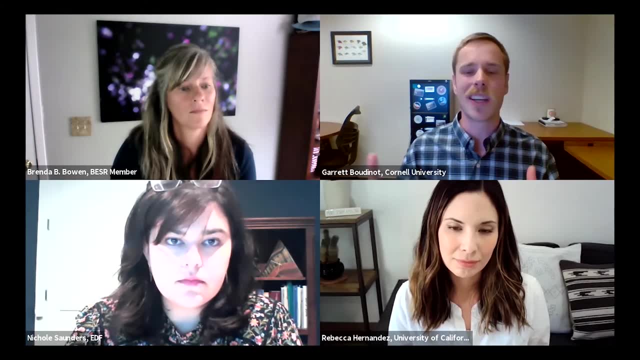 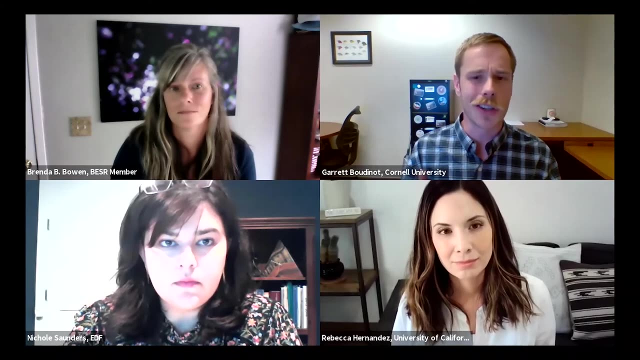 That farmers need, both on the acquiring materials and the management and verification side of things. and so there, there are certainly ways that we can Get farms of all sizes, wherever they are the material. the question is: does the do the costs? 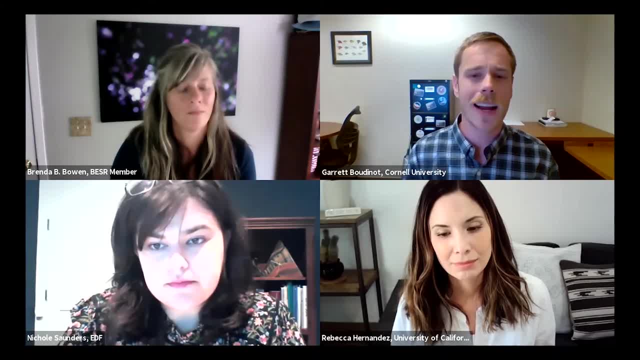 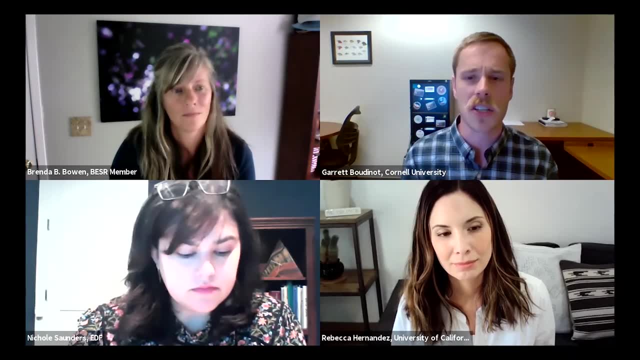 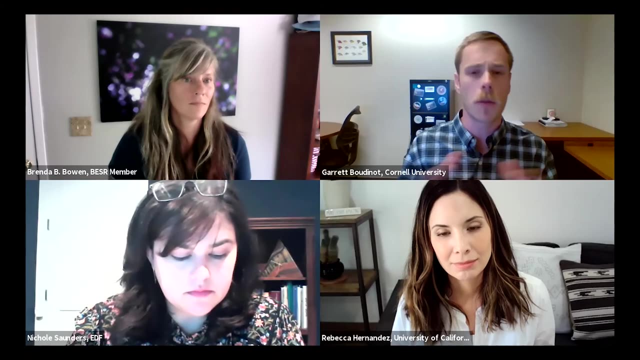 match the benefits or do the benefits outweigh the costs, and I think there's also some creative. Brian was talking about this. you know market and policy changes that need to happen on. I know that cooperatives are things that farmers use currently just small farm operations used to stay economically viable. 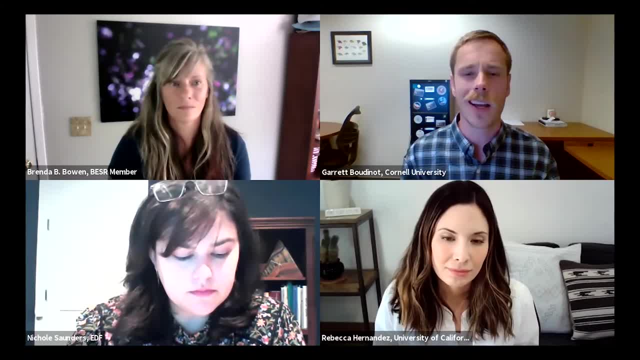 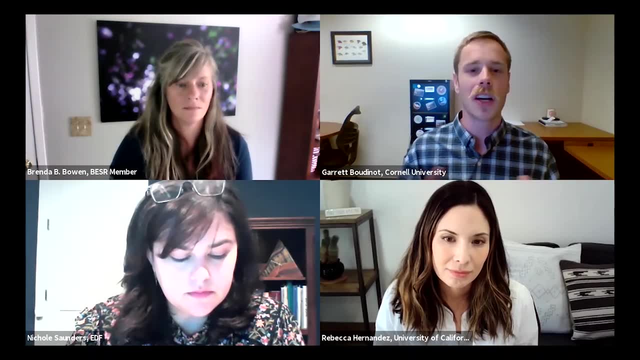 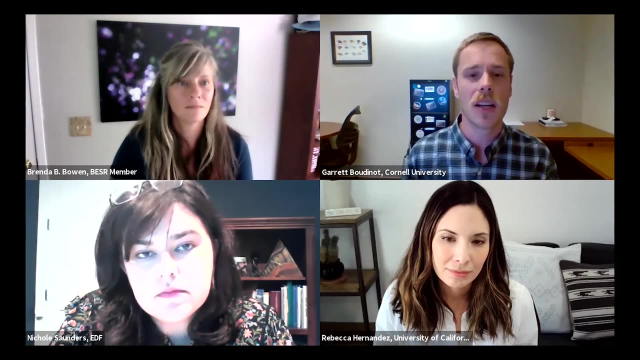 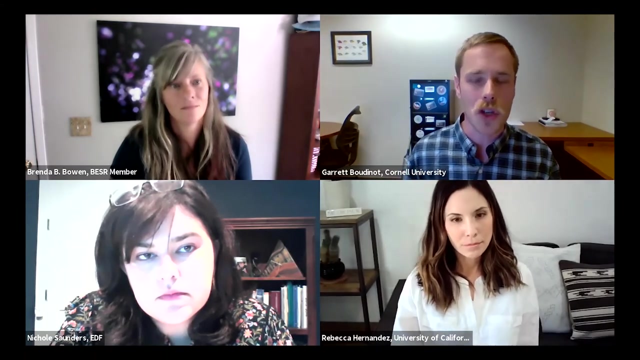 With these large farm operations, and we're envisioning how farmers could have Carbon cooperation so that they could cost, share some of the the needed inputs or acquire enough of these materials that need to be shipped To get elsewhere. and the last thing i'll say is been talking a lot about economic costs. there are, of course, carbon costs with transporting, and so wherever the these materials come from and go, 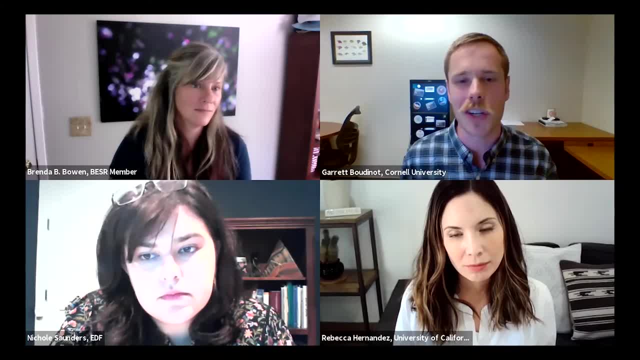 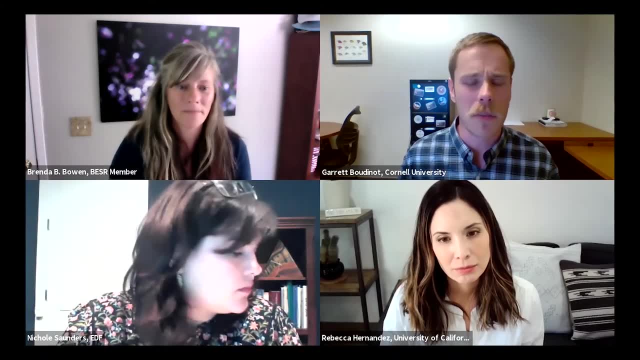 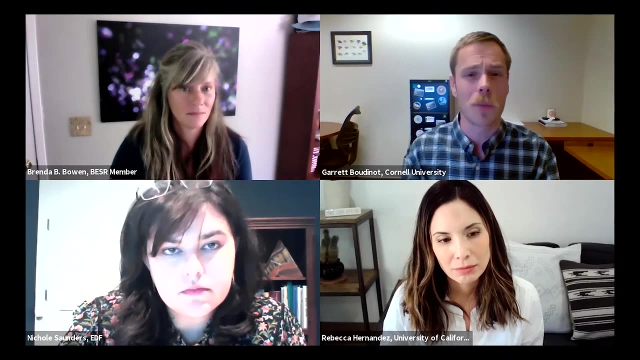 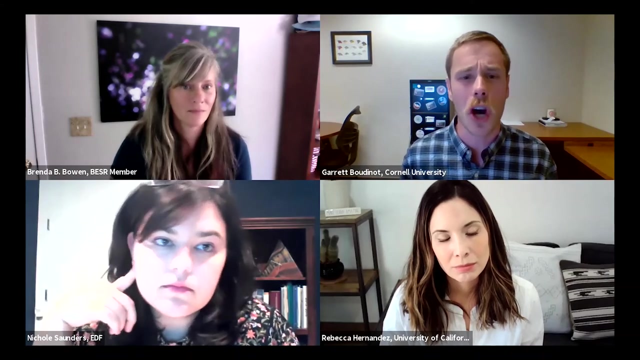 To. we need to make sure that the emissions from that transportation are lower than the carbon that we're sequestering. some existing models suggest that for many regions we could easily get to a place where we're emitting 10 to 30% of the carbon we're sequestering. so we're still sequestering a large, you know the cost benefit. that still says this is a huge carbon benefit. 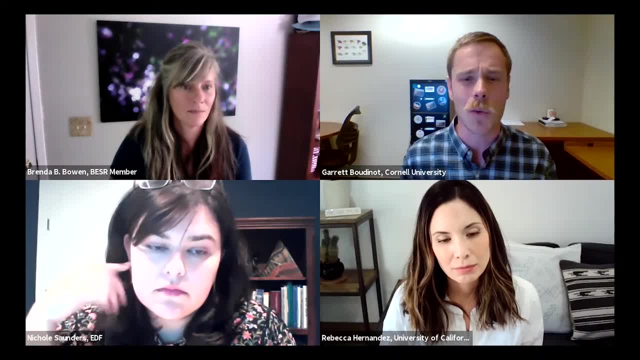 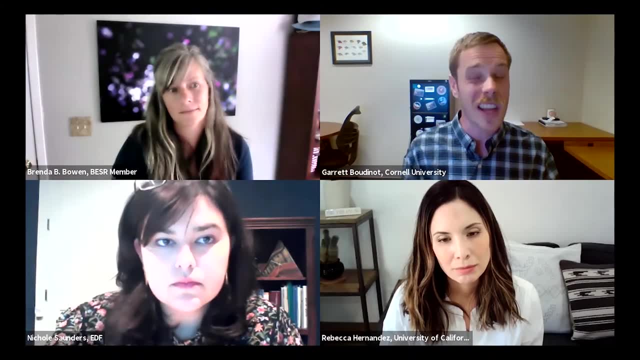 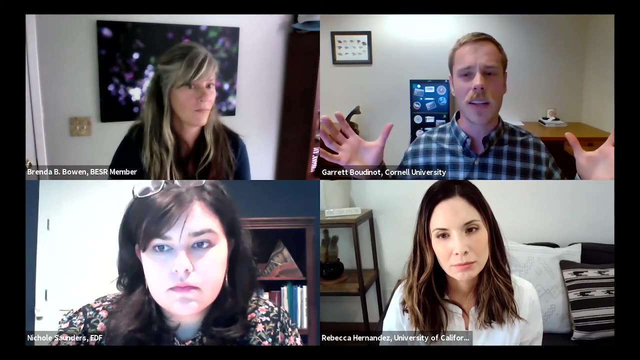 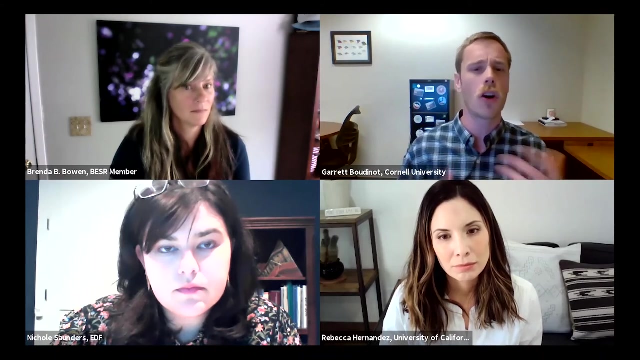 And we're in the early stages of developing enhanced weathering, And so i'm optimistic that, as again we look at those new, those other industrial materials and ways to safely use those, optimize the ways that farmers can form cooperatives and share and and stock pile a lot of these materials so that they could use rail instead of roads, for example. these are all creative ways that the market can move. 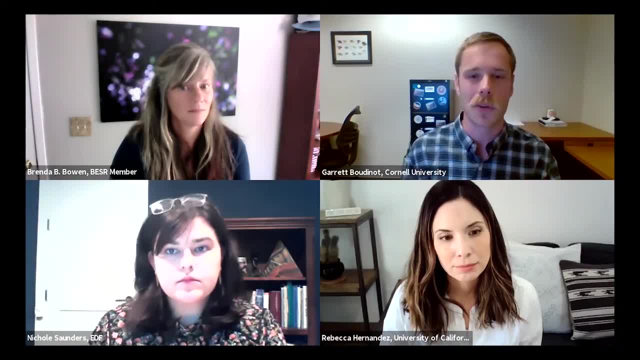 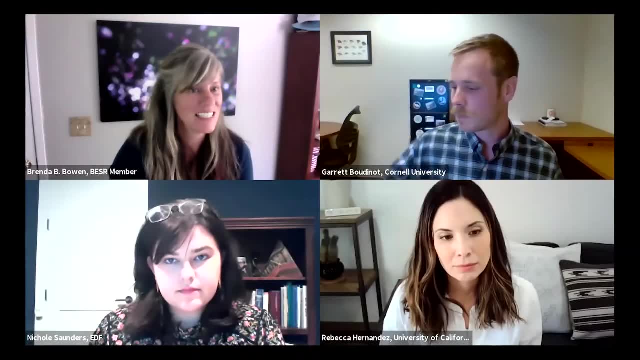 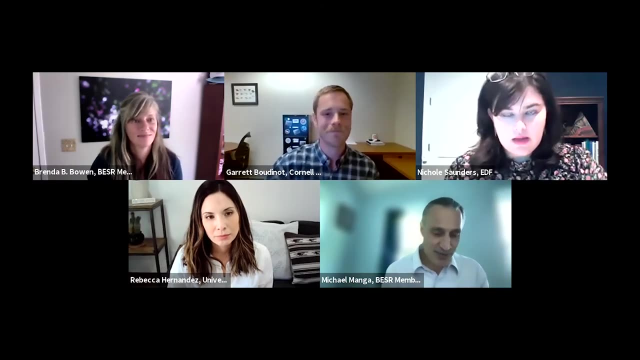 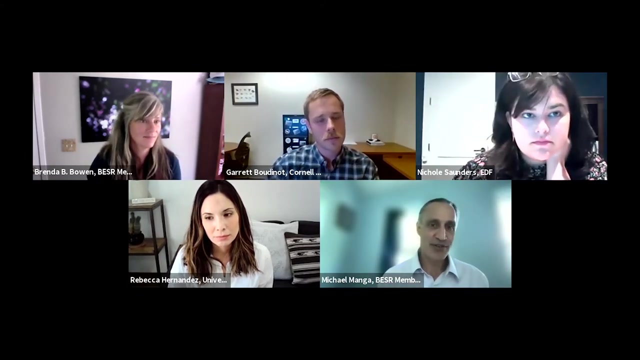 So that we can address this issue of getting the materials to the farmers safely and effectively. Great, Thank you, Michael. invite you to ask a question. Thank you to all the presenters that have so many great questions, so many questions based on your presentations. but maybe to start with Garrett: is there a limit to how much rock you can put on a unit of land before you accumulate too much? 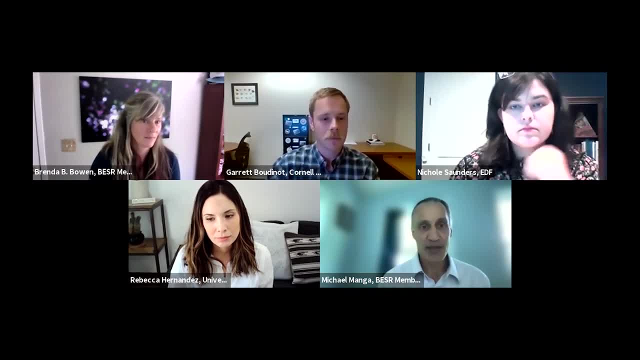 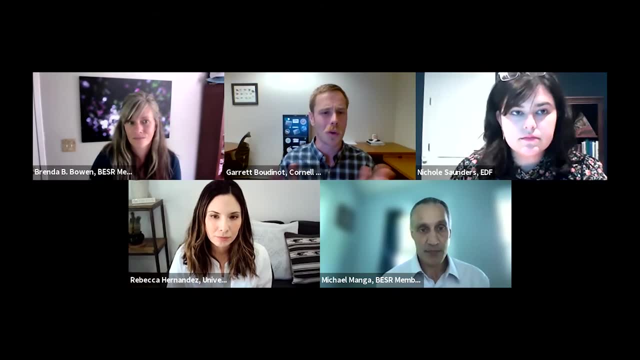 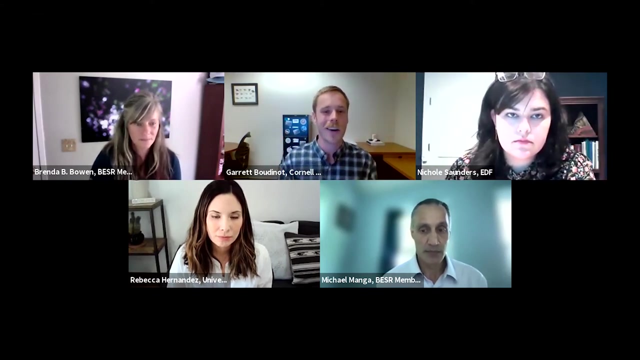 Other byproducts, for example clay or silica? Great question. The studies at the field scale are rather limited. so the working lands innovation Center is really currently the largest field deploy trial system in the world and we're still in our early phases. but some existing trials in the mesocosm or pop scale can shine some light on this. 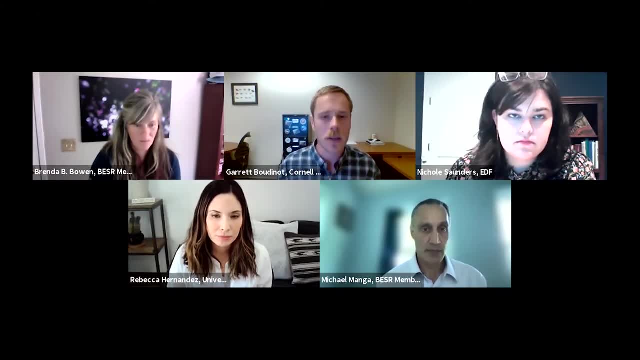 we're seeing that there is an upper limit to how much rock material can be applied to soils before The soil becomes so basic or the pH increases so high that you're no longer effectively dissolving the material. It turns out, though, that the amount of rock dust that would be needed to generate that high of pH is pretty exorbitant, on its upwards of 50 tons per acre- really high. what we apply is generally about 20 tons per acre, but we're going to be trying with up to 40 tons per acre, so 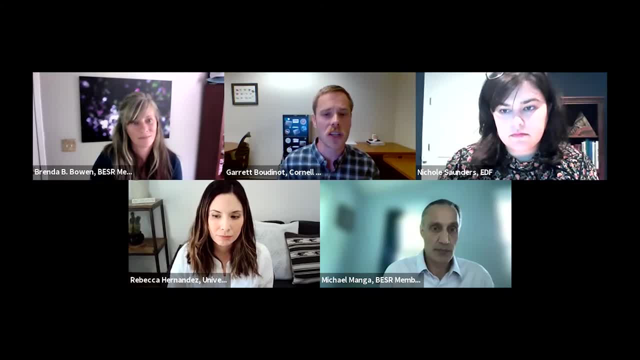 So all of this is to say that is an open question. and when Ben says there's still a large gap between theory and deployment, that optimized amount of maximizing agronomic and carbon benefits with respect to the amount of rock that we apply, that's at the forefront of the research we're doing. 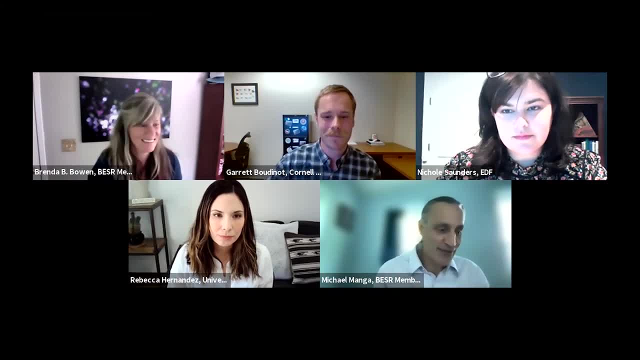 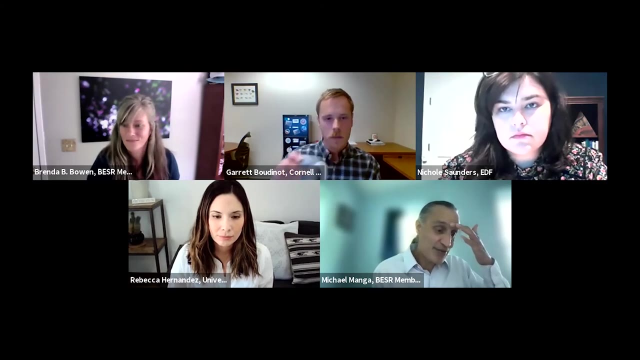 And I can ask the second question. yeah, go ahead. For Nicole, I was really struck when you showed the map of where produce waters are Coming from, where waters are being produced and where studies of what to do with that produce water been undertaken, and it seemed like there was a great correlation between how dry setting wise and whether people have been exploring using produced waters. 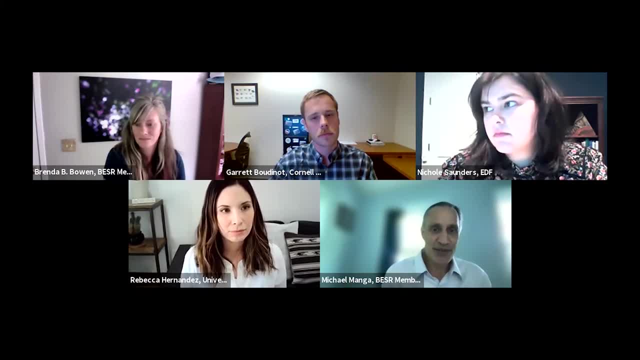 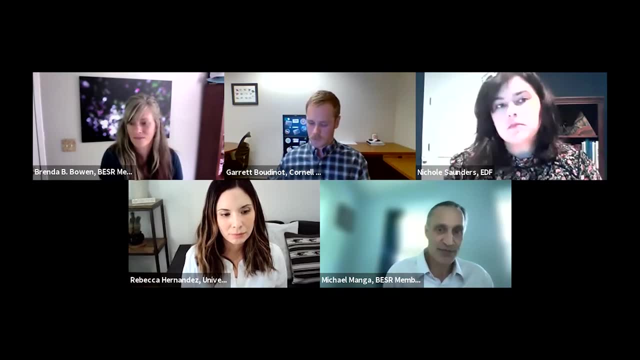 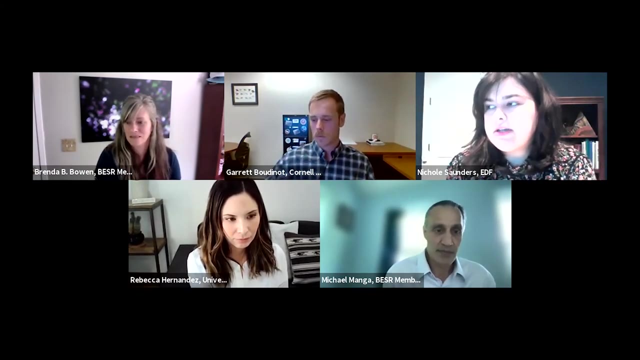 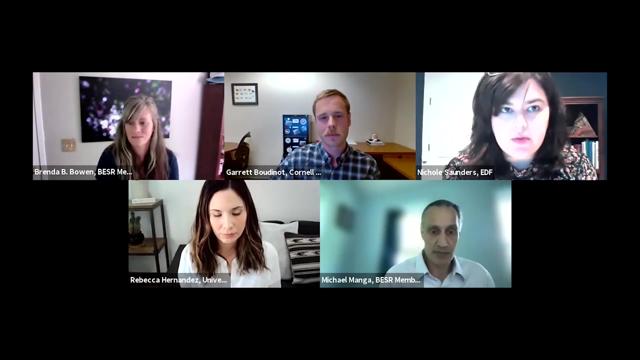 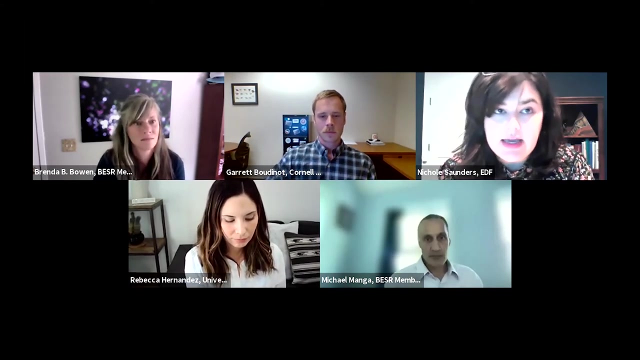 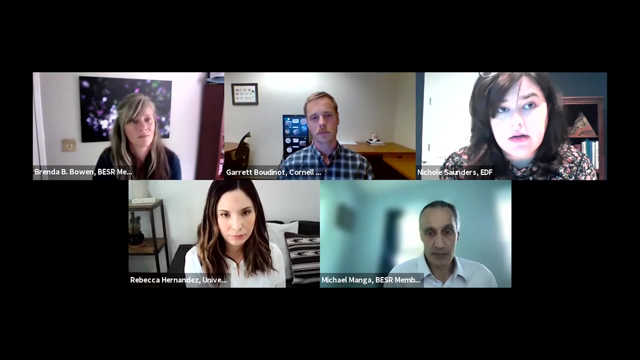 Is there a reason why California and Texas have not been exploring, have not take undertaken as many studies about produce waters? is there an expectation that production will decrease over time? No, I you know. I think one point to make is that the We were looking at studies of produce water specifically that did advanced chemical characterization of produce water. so that's not to say that there haven't been different types of studies on produce water, maybe for oil filled purposes or other places. 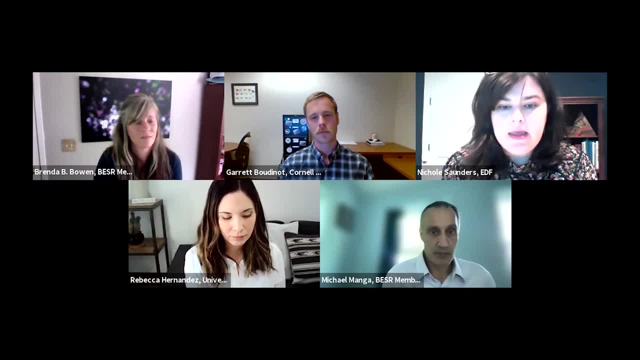 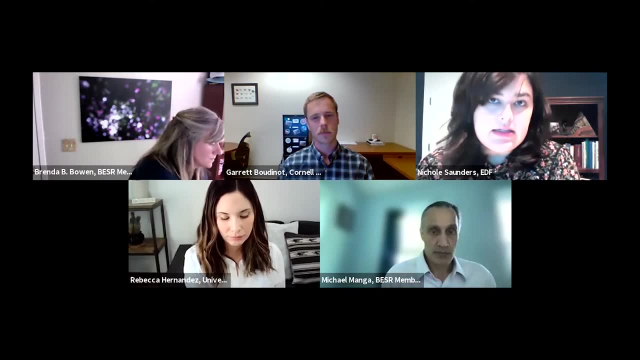 First and foremost is the first thing I think I want to say In response to that. the other is that economics is a major driver in this, in this issue. so in Texas, for example, produce water is predominantly, probably more than 90%. it's hard to know the exact amounts right now- reinjected. 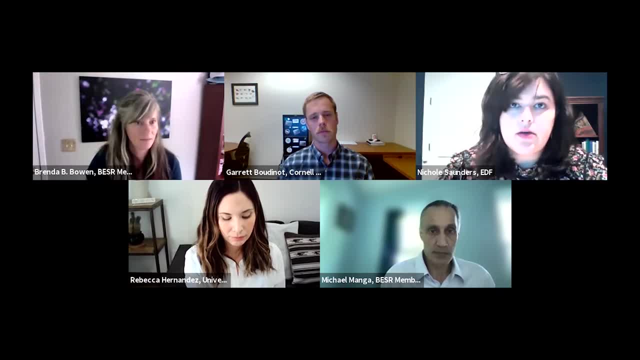 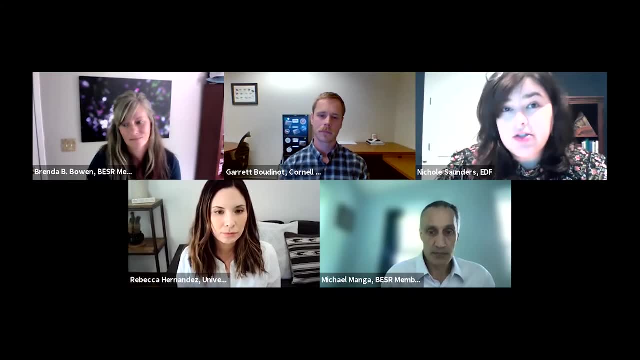 Some of that is for just reinjection for disposal. some of that is also technically a form of reuse through reinjection for enhanced oil recovery. so Large volume and you nationally- about 45%- I think was the last statistics I saw a produce water is reinjected for enhanced oil recovery. so in that sense it is reused in some places. 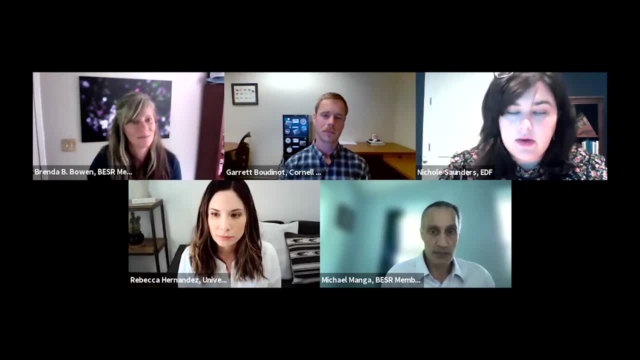 And the other thing to know with Texas is that disposal wells are widely available and a low cost alternative for underground and injection and management of this waste stream and, from the perspective of a Scientifically based environmental group that worries a lot about public health and exposure risk, and where those walls are constructed adequately at the moment, they do reduce exposure risk from the management of a really, really complex often. 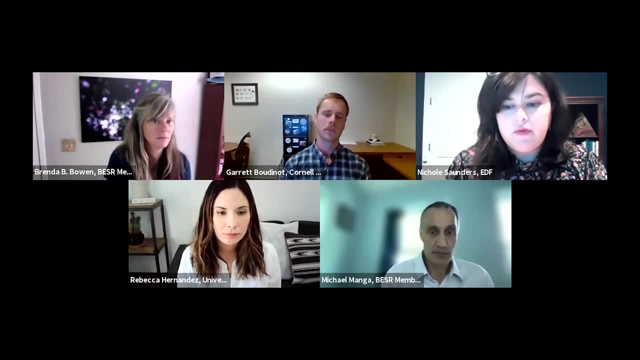 Toxic waste stream, and so when we think about moving outside of the oil field, there's there's both an economic consideration of the amount of treatment that you would need to do To treat this water to meet a standard that Really has not yet to be really comprehensively set to address what we're concerned about and produce water. that number just at a basic economic. 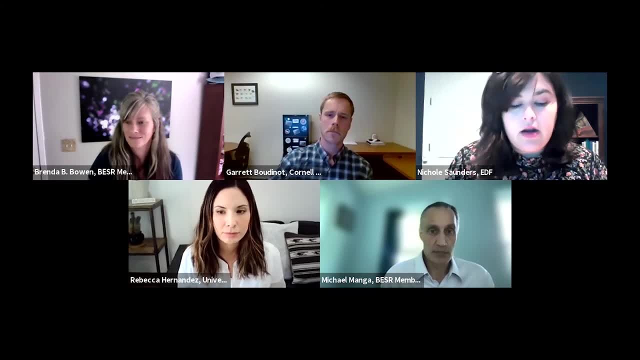 needs needs to be competitive with what your alternative is and then also your risk management decision. so in Texas, for example- I think we're just now starting to see that really ramp up- there's a consortium beginning to Look at treatment of produce water for alternative options that we're going to answer. ask some of these hard questions. 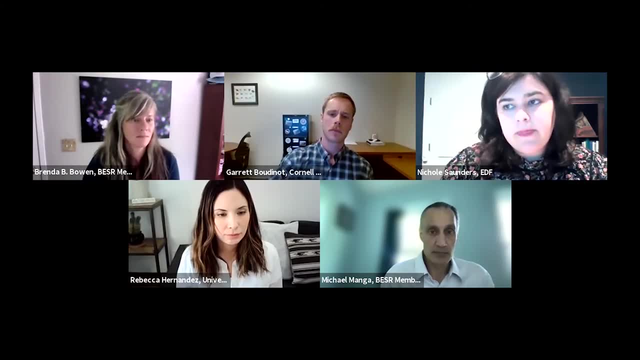 But we haven't seen that yet. just basically from an economic standpoint in California, unless familiar comprehensively with what they've done across the state there are. there is a small region of California where produce water from steam filled operations that are not hydraulically fractured in the current river valley are used. 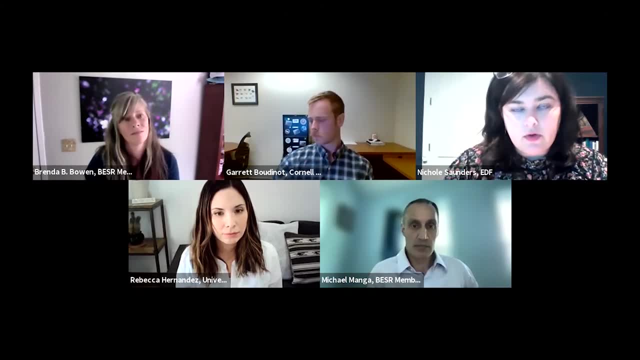 In the irrigation system for crops, including food crops. in that valley there's a food safety panel that is doing an ongoing study of the safety of that practice in looking at Comprehensive characterization of the water itself that's being used in an analysis of. 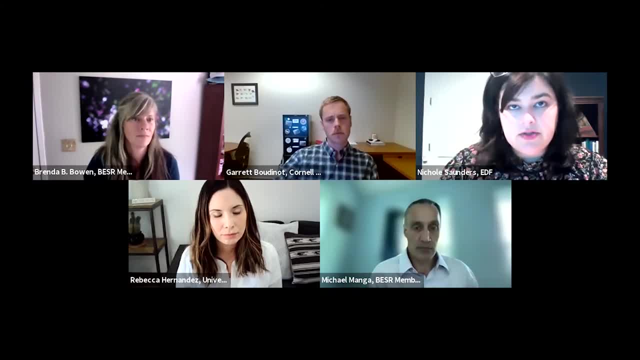 The fruit and other issues, and to look at public health impacts from consuming foods that are watered with produce water. that's a very, very specific kind of a niche area where that's happening. it's not happening anywhere else in the country And that's due to a number of different factors, but there's a lot of interesting research on that. with the food, if you think, if you research. 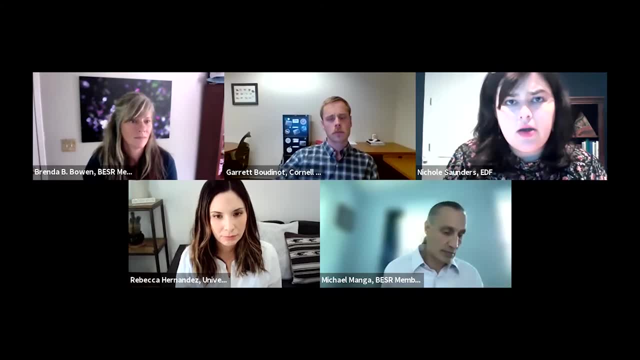 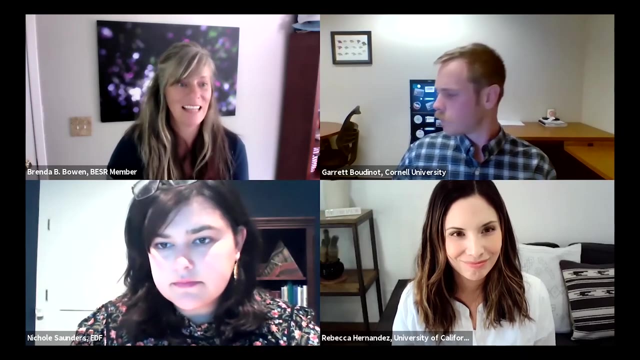 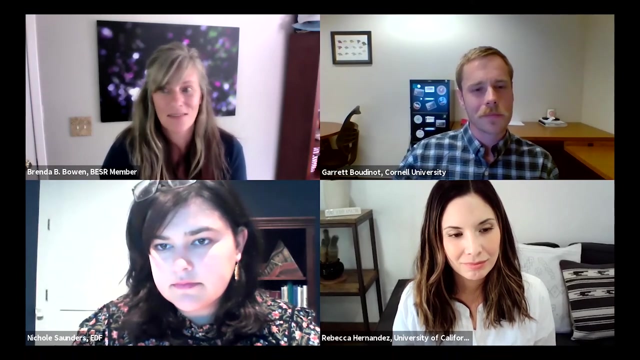 The food safety panel on the California Coelho irrigation water district. those things would come up and you would see what's going on in California there. Great Thank you, Nicole. we'll go to a couple of questions for Rebecca next. One question from the from the audience, was about the impact for increased solar on heat island effects, urban heat island effects. 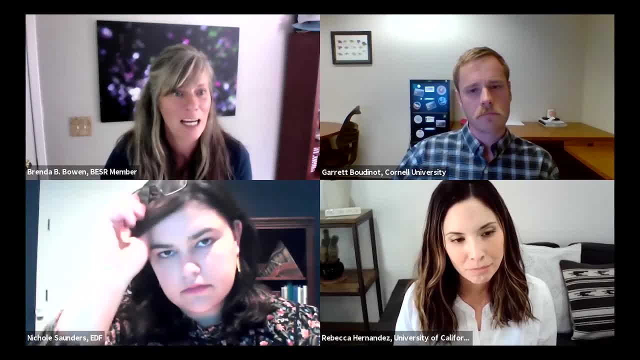 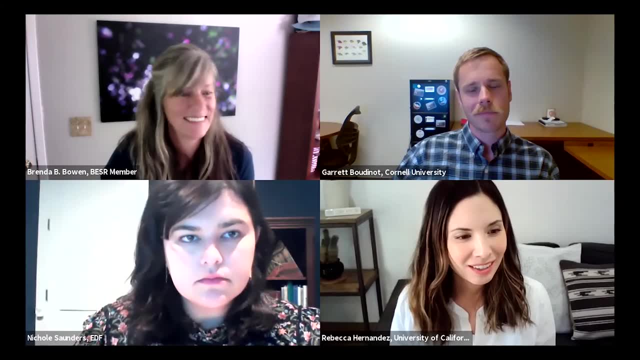 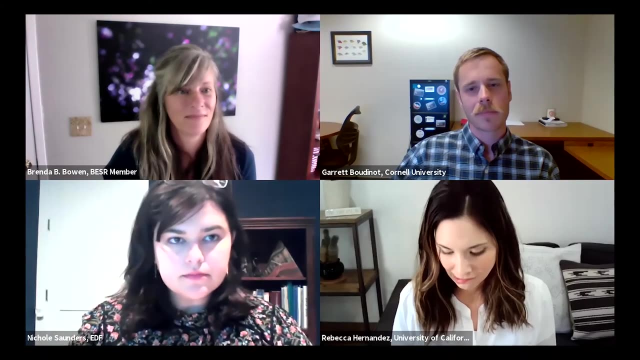 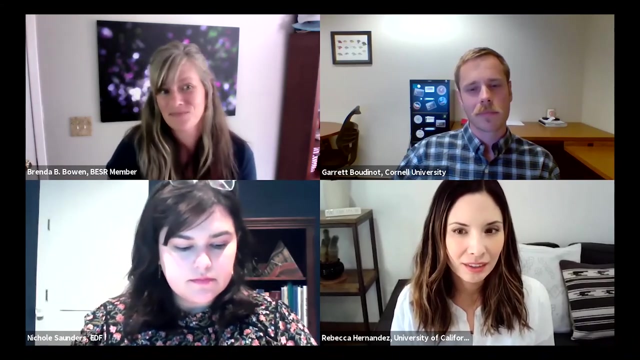 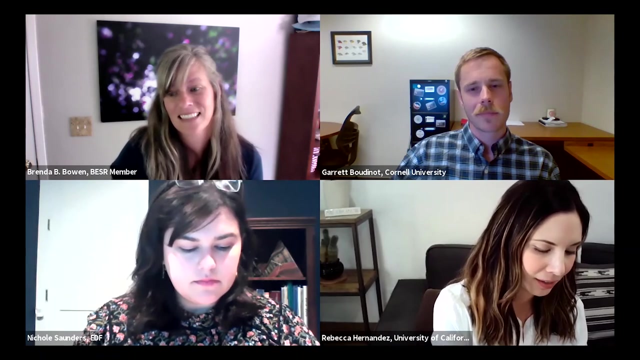 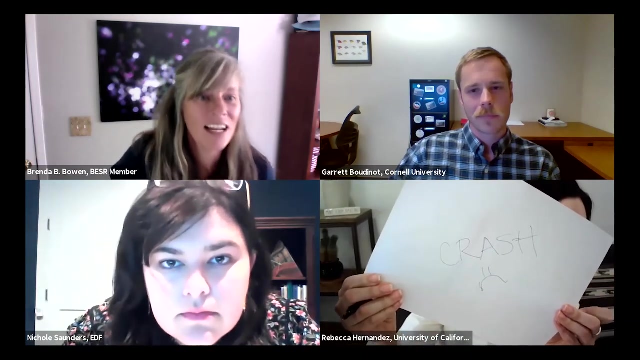 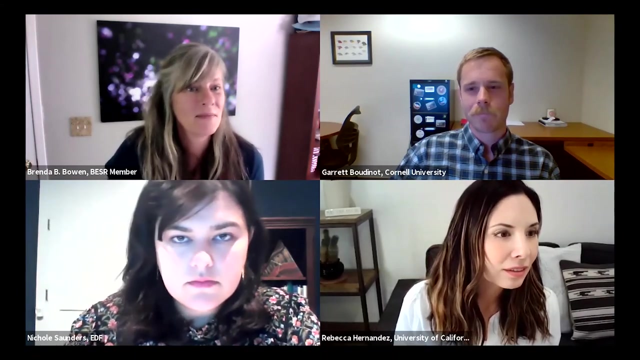 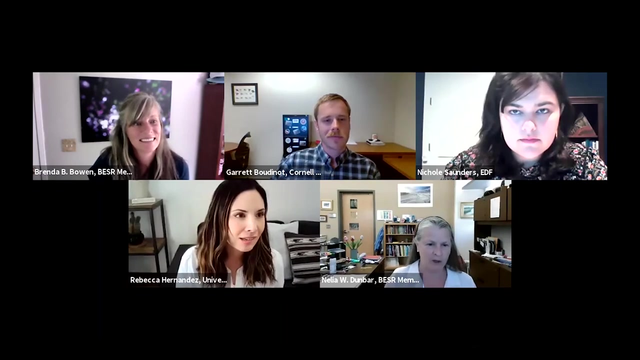 urban heat island effects and what we see in that area. I think you're still muted. you're not able to unmute. Eric, can you help Rebecca unmute? Oh no, a crash, that's no good. um, Amelia, yeah, I had a question for Rebecca, but because she's crashed, I have a question for Garrett. 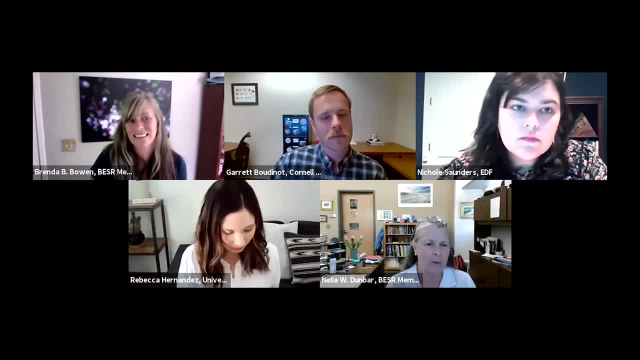 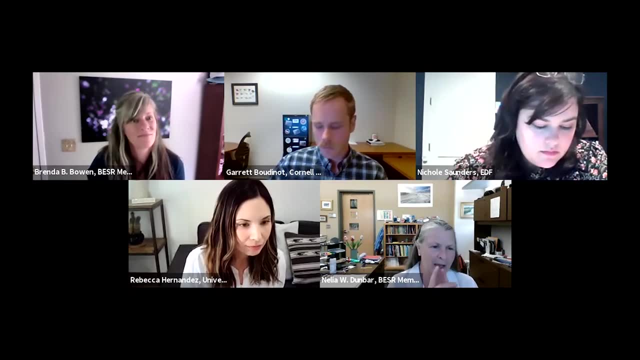 i'm Garrett. i'm curious, a little kind of a follow up on what Michael asked um you You add rock dust to agricultural fields and it. I think most you may not be able to answer this because it looked like the time scales that the experiments so far. we're pretty short, but what i'm curious is: 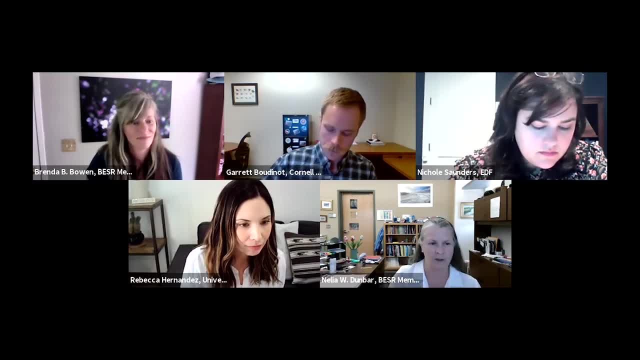 What is the time scale? you know you add X amount of rock dust, 20 tons per acre camera. what number, he said. but and how? for how long does that geochemical reaction continue to completion? what's? what's the time frame? Great question, and 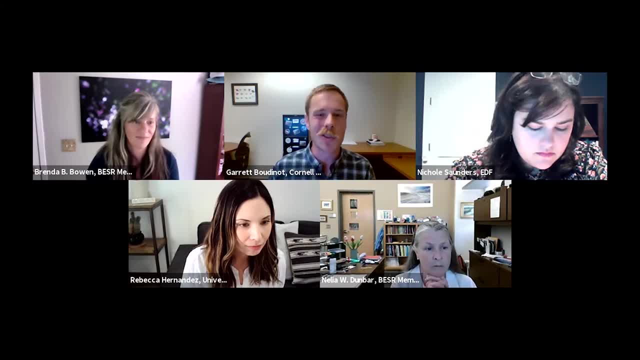 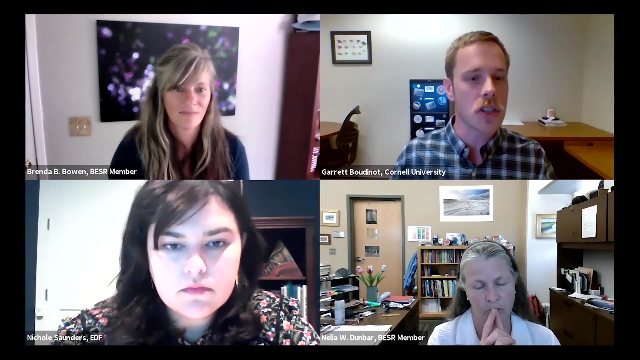 yeah, unfortunately, because this is a relatively new technology and new idea. we're still figuring that out. we're thinking this is an annual application and so this is something that farmers can apply every year. it's what we're doing in our trials, And it depends on the material or the the long term. fate and efficacy each year of enhanced weathering depends on the material. 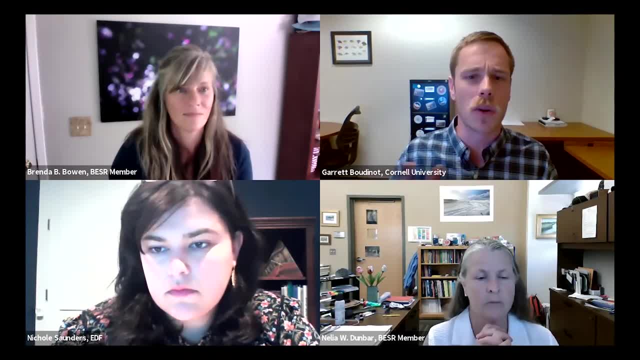 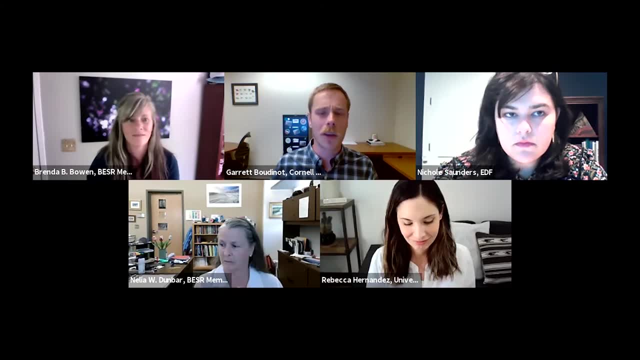 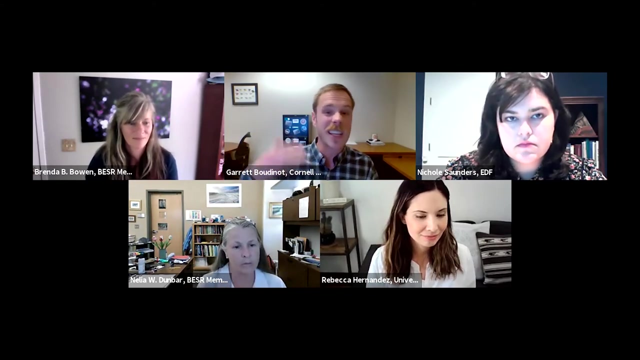 The grain size especially. So there was a question in the Q amp a of what's the ideal particle size material. all of these things are very much still being optimized and so Ultimately we want to increase the amount of dissolution that happens. so the more of these particles that you fully dissolve then, the more each year it's effective, and that is a function of temperature. 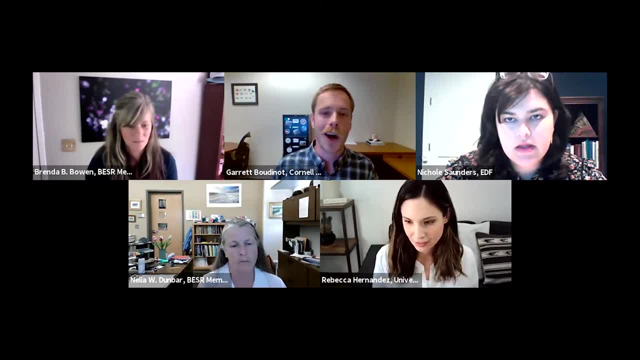 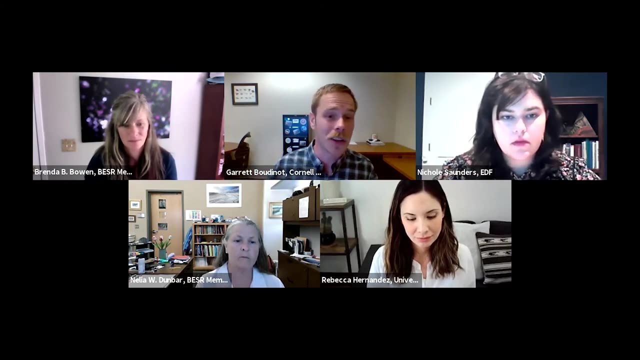 precipitation, And so we imagine that the best mineral to be to use for our trials in the palm of valley in California are going to be in the rate and practice there. it's going to be very different from the optimized practice that we have here in Ithaca, New York. But that's a great question. it's something that we're still optimizing, though we are relatively confident that doing this each year for for many years again, depending on this pH Of the soil and the climate, and this can generate the same agronomic and climate benefits. 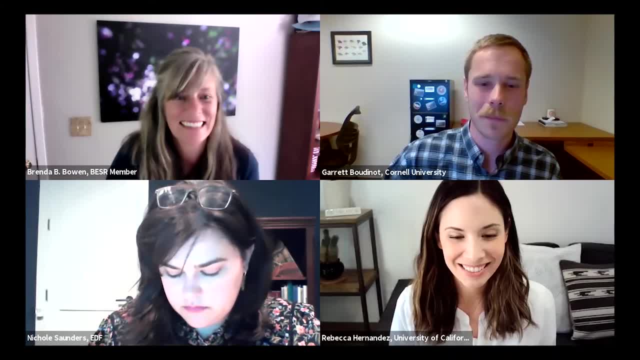 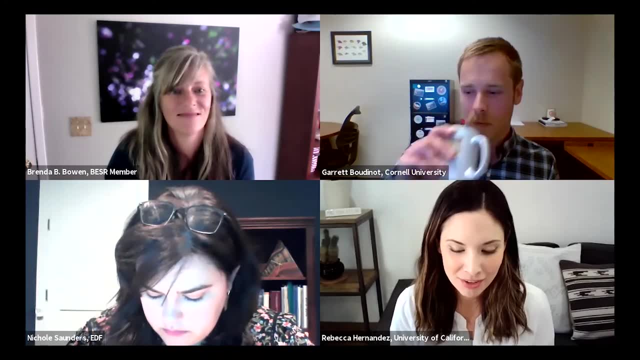 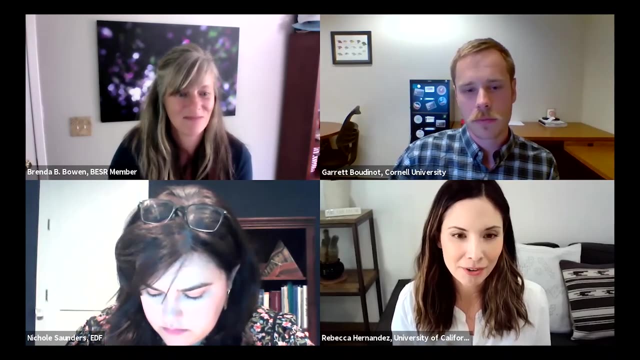 Okay, I think we have Rebecca back. yes, Yes, thank you. I had to shut down my zoom, it would not let me do anything. yeah, Thank you, The the well. I think I actually missed one of jim's question. he was asking about assessing. 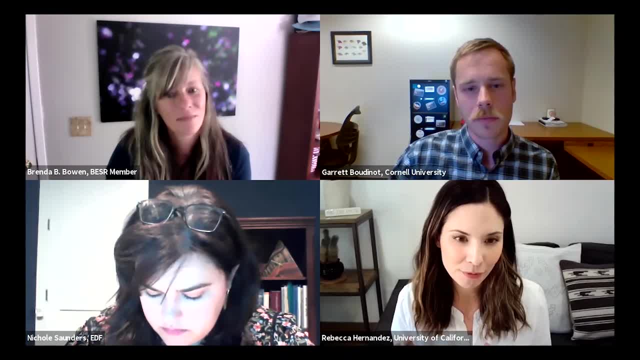 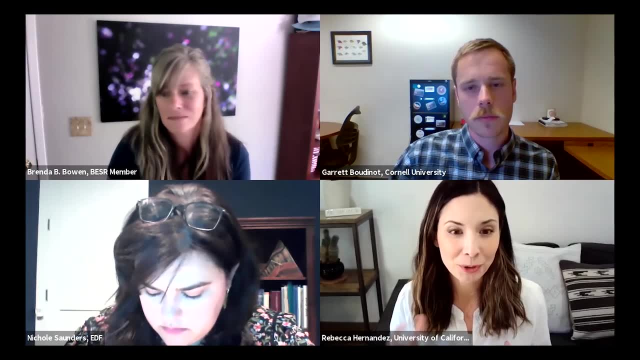 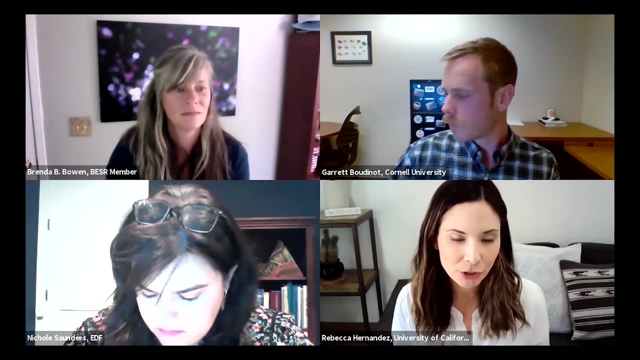 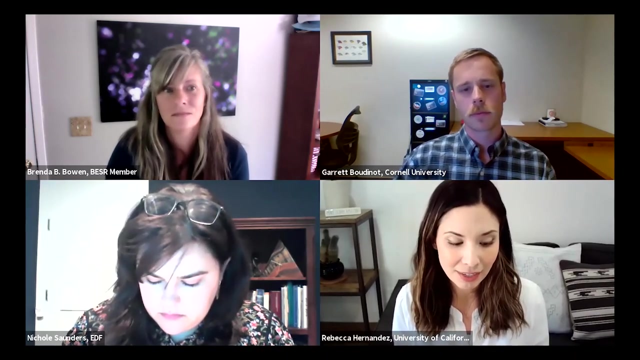 The footprint come by of CCS with natural gas? and to answer his question, no, our group has not done that analysis. it would be really neat to see To go from, you know, production and capture and transportation to injection and and quantify the the land footprint of that. 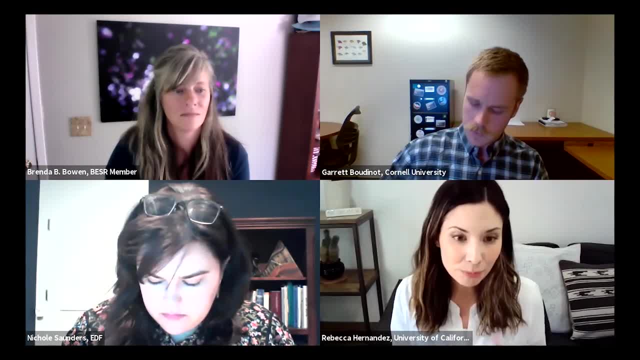 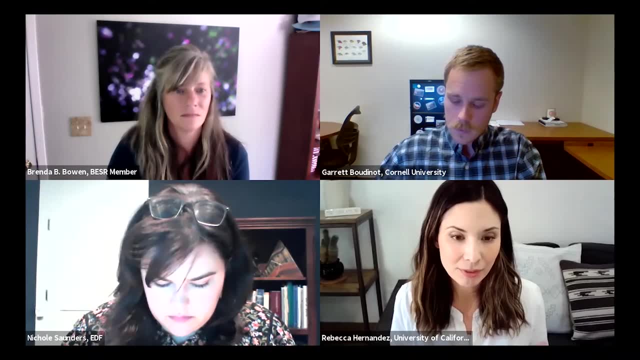 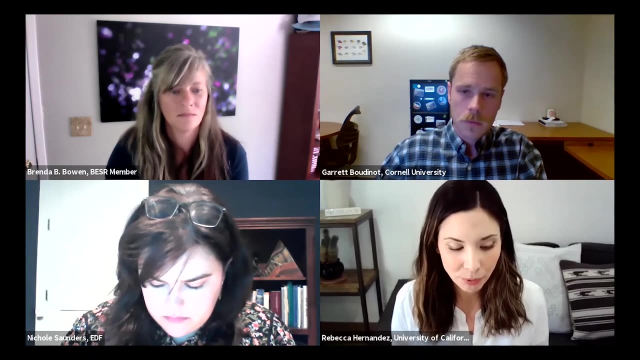 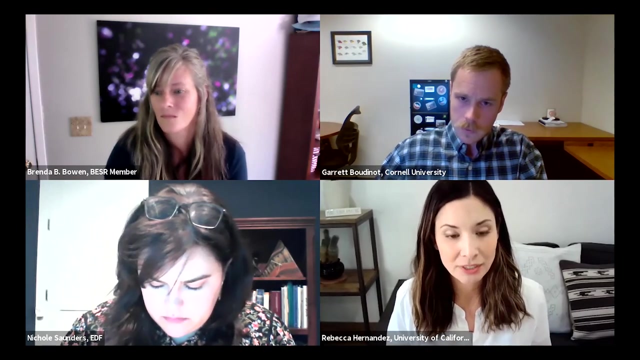 My guess is that a lot of that perhaps would be Comprised of footprint associated with with pipelines, as that's typically the case, for you know, the footprint of a natural gas power plant as a whole. but our group would definitely be poised to answer that question and certainly we're looking at other kind of gaps in the literature on footprint. 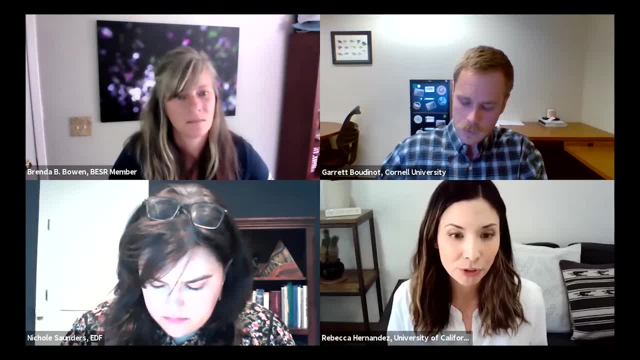 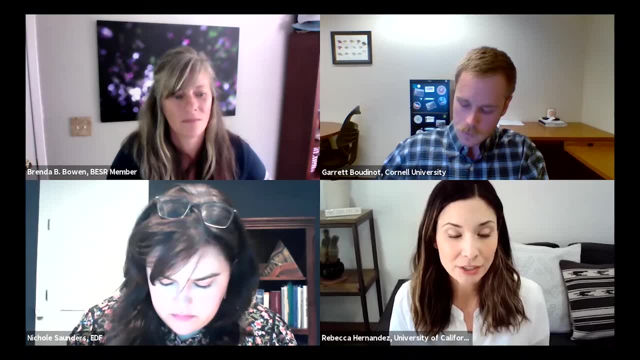 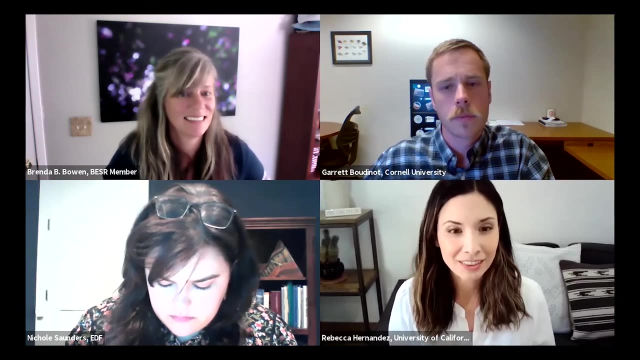 associated with energy infrastructure, like geothermal energy storage. those are Two areas that need That, need a lot more constraining in terms of the data that we have. and then the other question was on: oh, land surface temperatures or air temperatures? and there is there's, that's another really. 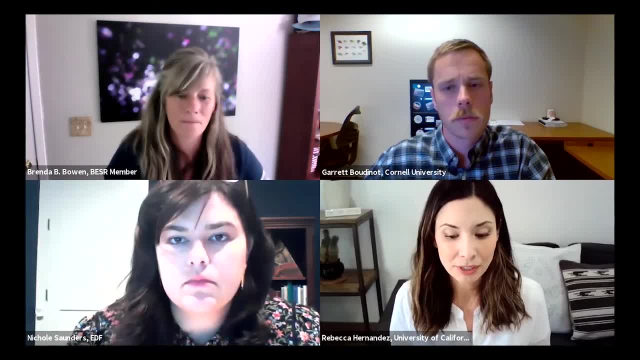 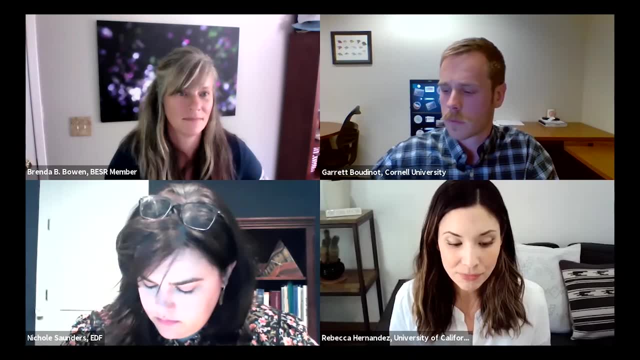 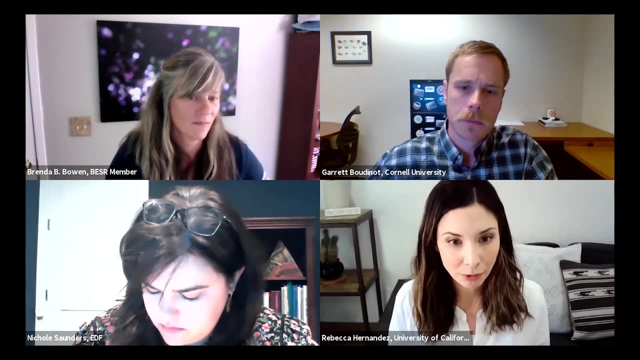 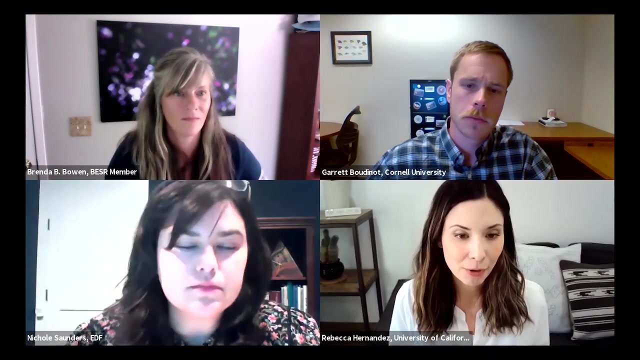 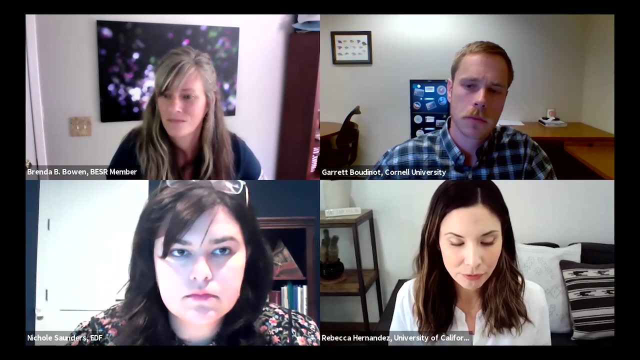 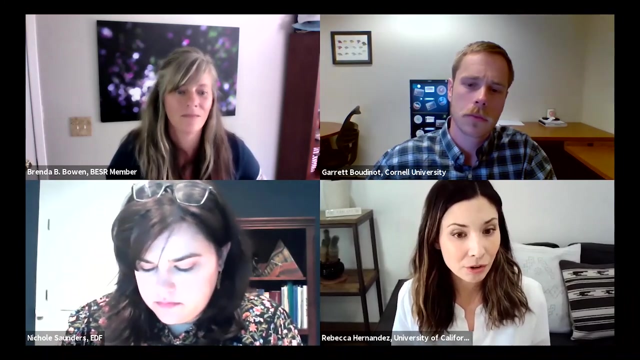 Important gap, I would say, in the literature that needs to be closed there. there there's consensus to date that that air temperature increases Within within solar parks, Particularly when you have ground mounted installations in, say, hot, semi arid climates. so we're looking at about three to four degrees increase in in in air temperature in a hot, semi arid environment and maybe two to five degrees in in, say, a cold, desert environment within an urban area. there's 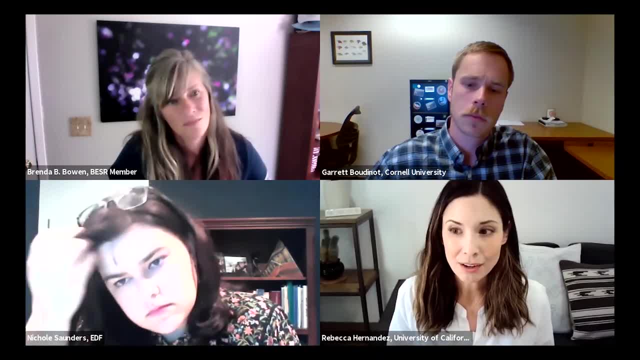 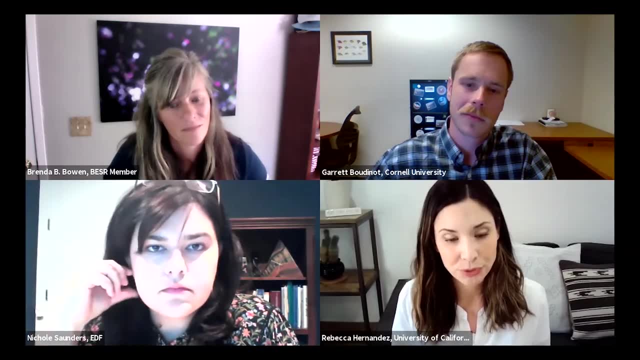 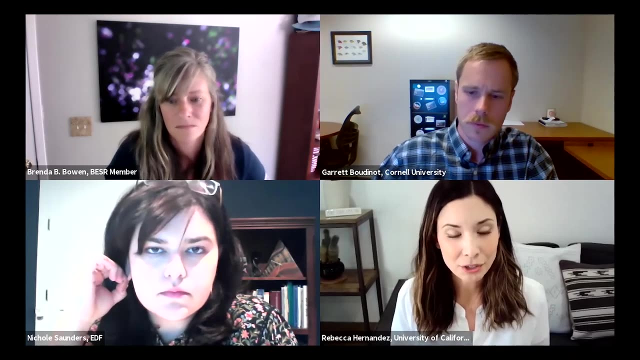 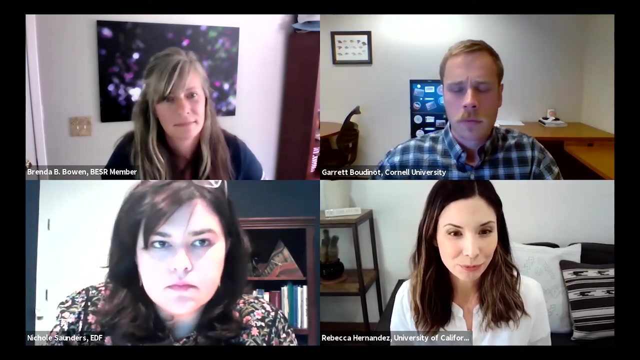 Increasing consensus, I would say that That Deployment in urban areas actually can serve to reduce The urban heat island effect, which is another one of these techno ecological outcomes that can really provide, you know, great benefits, not only just with that, but something that is really important to for parking lots, that that can provide a lot of important. 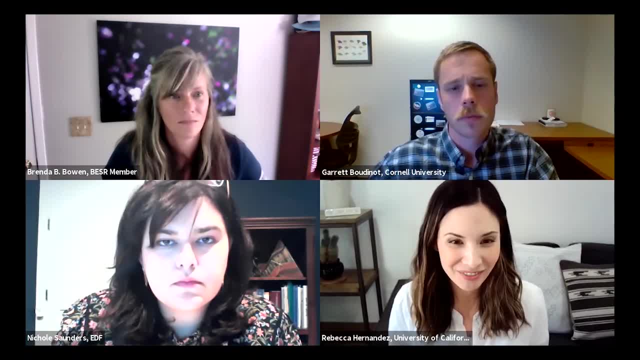 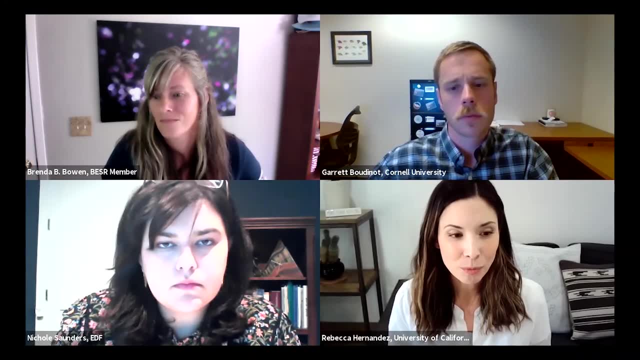 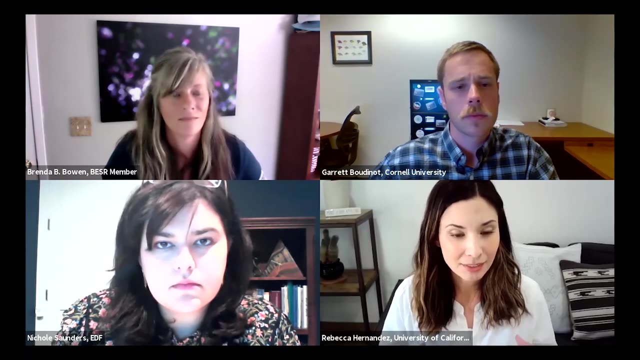 Services to people and In their cars when, when they get off of work or something, And and so there's a lot of work that needs to be done. one study that we're working on now is is exploring not only how solar energy development and arid lands impacts within 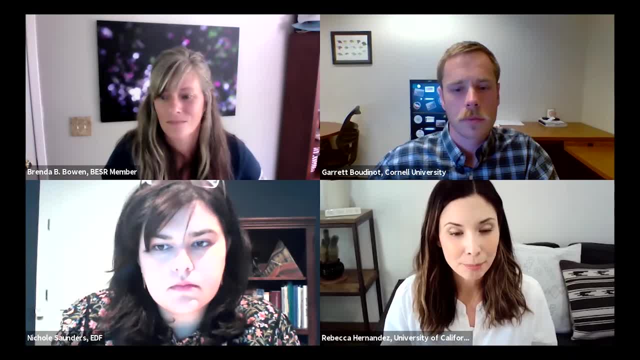 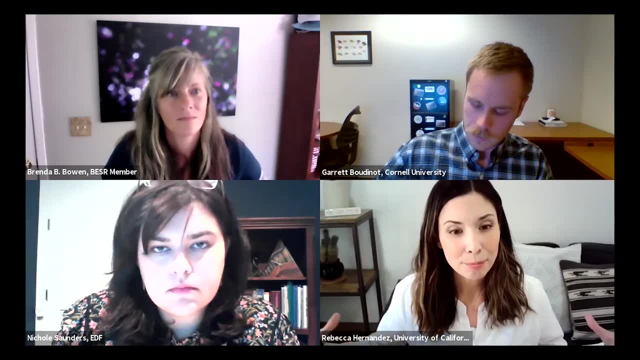 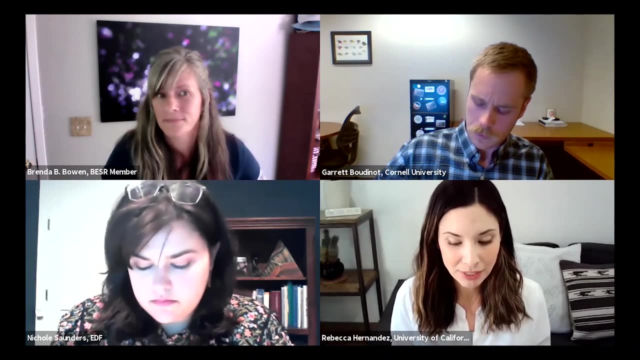 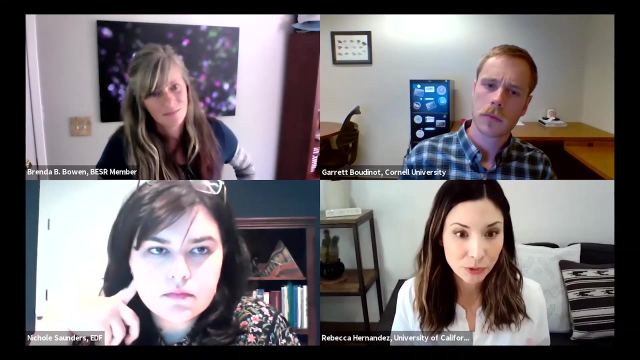 Within surface temperatures within the actual park, but beyond that. so what we're seeing is that there is a presence of a cool island that occurs beyond The the boundary of a Of a ground mounted installation up to 730 meters, so about 750 meters away from the solar park boundary. 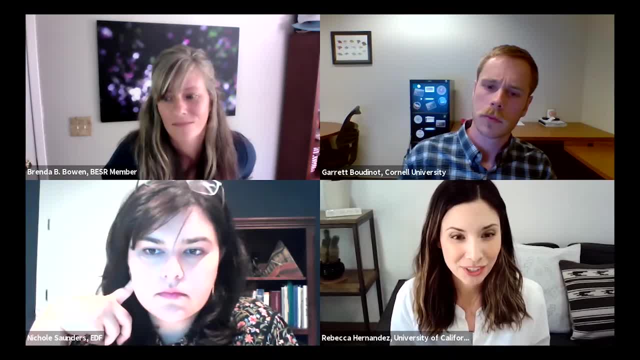 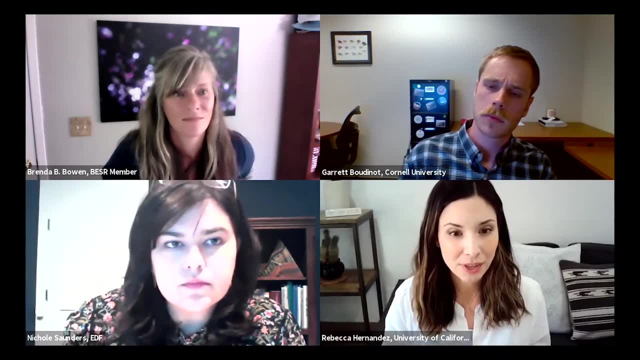 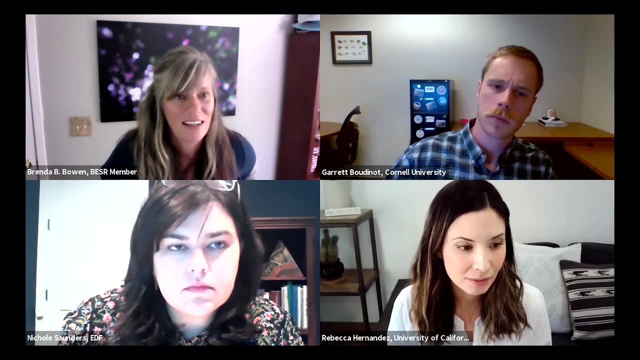 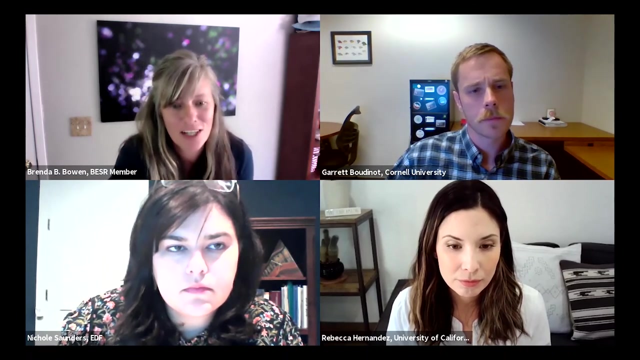 And so this is all sort of an area of active research and a really important consideration when you think about all of the Environmental cues that can be impacted from those Changes in both air temperature And land surface temperatures. And i'll ask a follow up question for you, Rebecca. we're interested in your comment on on how energy infrastructure 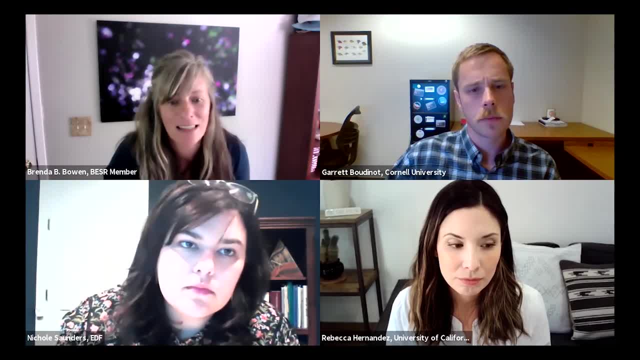 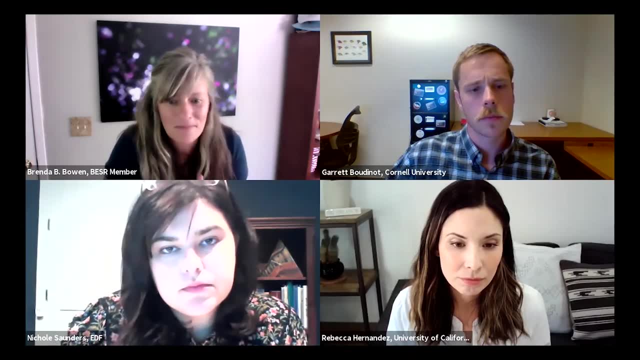 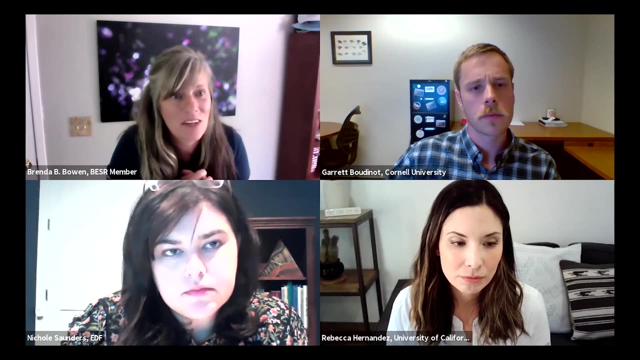 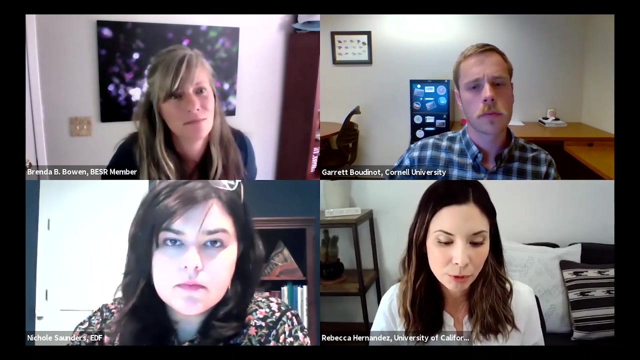 might impact and changing energy infrastructure might impact marginalized and indigenous communities, and wondered if you could say a bit more about you know how things like expanding renewable solar panel arrays might might impact communities, and either a positive or negative way. yeah sure, I think one of the most unfortunate side effects of renewable energy expansion, and perhaps one that 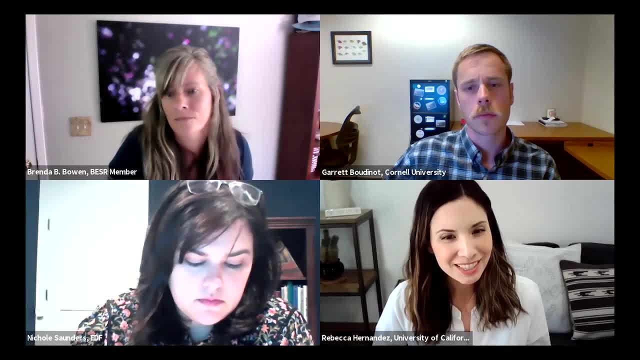 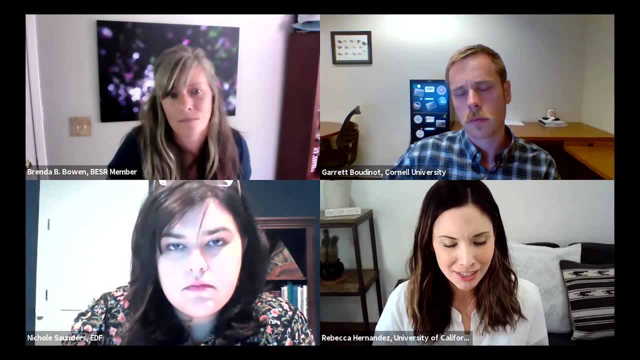 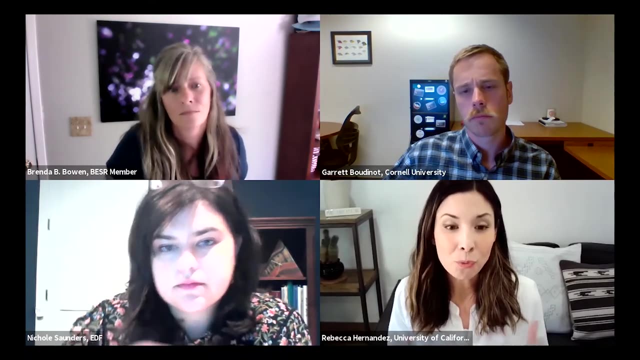 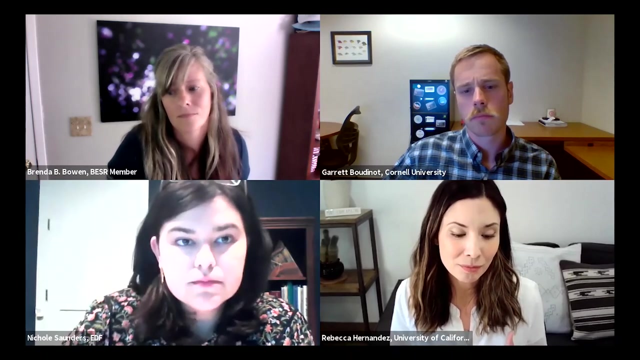 We don't often think about is that we don't really like to see Our renewable energy infrastructure. it's very industrial looking and refining that you know a lot of people. communities don't want to To see it in their view sheds and, and so the, the, the what happens is is that a lot of times, 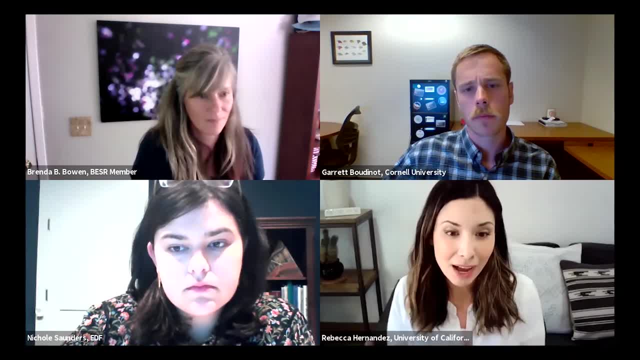 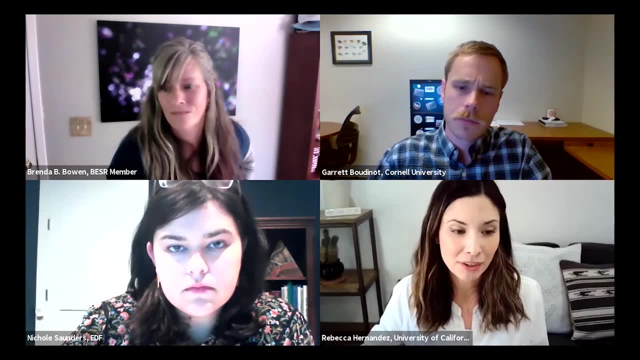 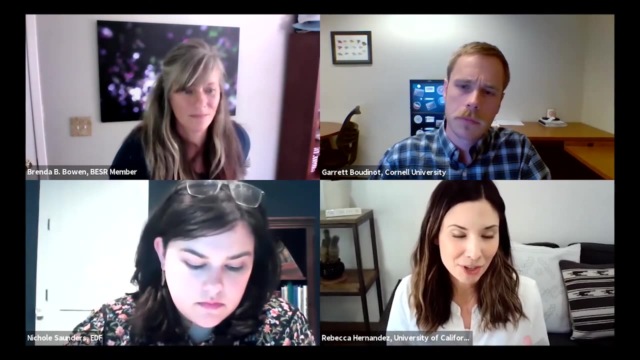 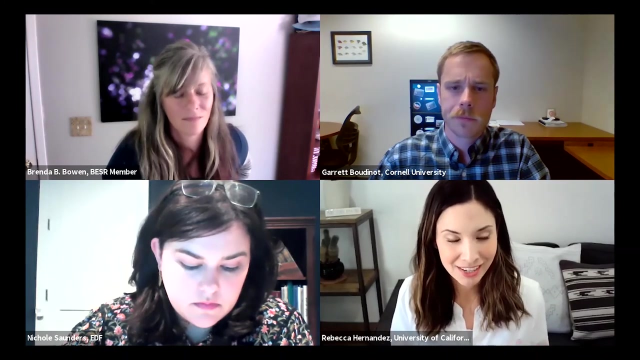 Our energy infrastructure gets what what we call outside it. they get installed into areas that are really really far from say, where the the credit for that particular power plant is given, And and and say: you know, maybe they're in the Silicon Valley and they're building 100 megawatt installation, but they're locating it in kern county, an area where Community voices are very disenfranchised and 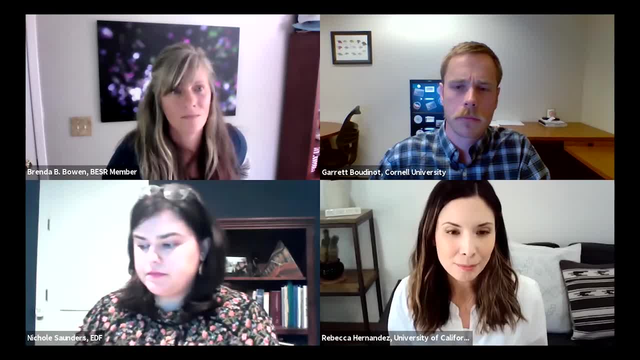 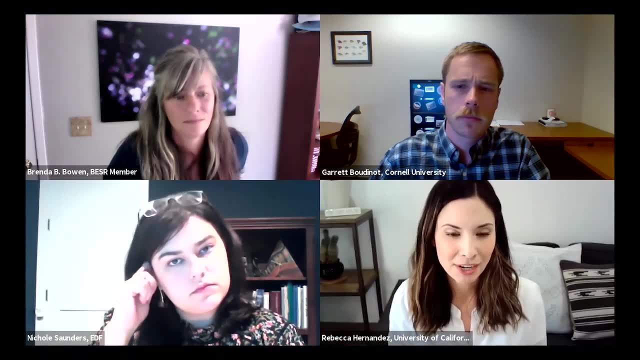 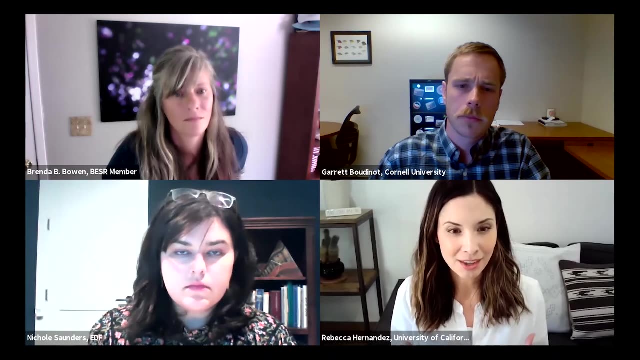 And people there are environmentally vulnerable, and so the important thing is to think about how we can kind of reframe our, our brain into thinking about how renewable energy infrastructure within our communities, within our cities, is something that maybe we can get used to you. maybe we can look at it as a 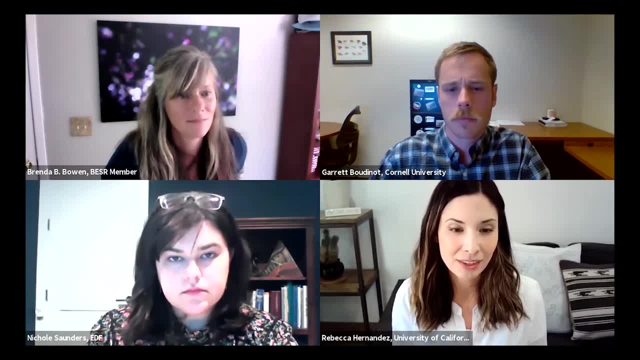 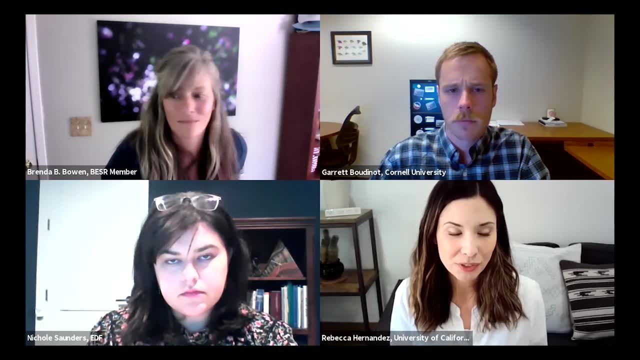 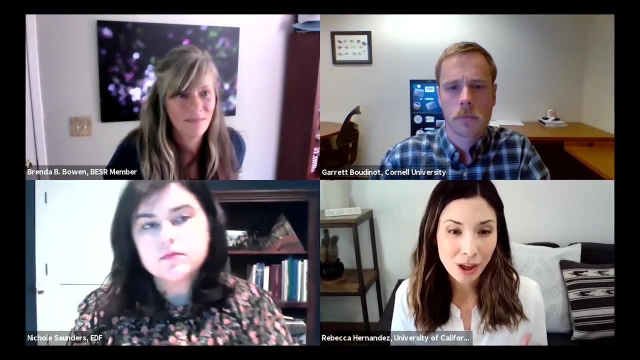 enhancement of the aesthetic value of the communities that we live in, because this is what will really underpin an increase in local energy, which will reduce transfer, transmission costs and associated loss of energy, and and so we're doing a lot of work on that front. looking at the 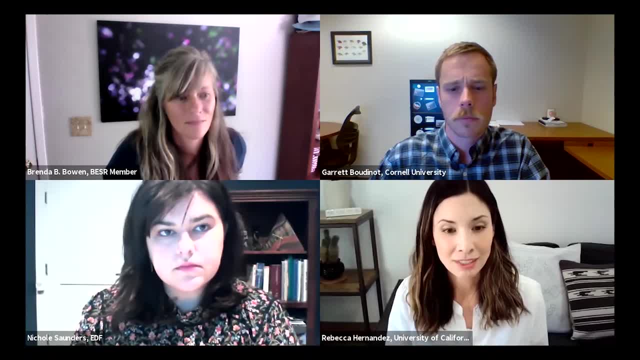 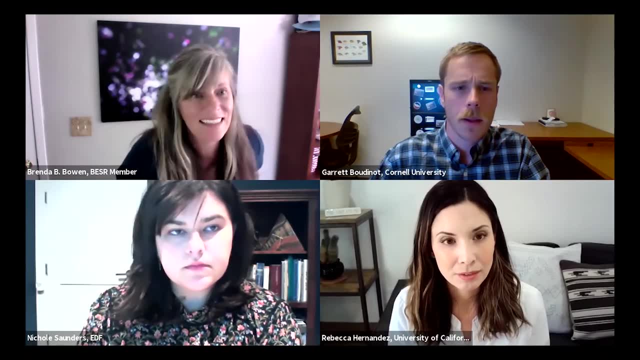 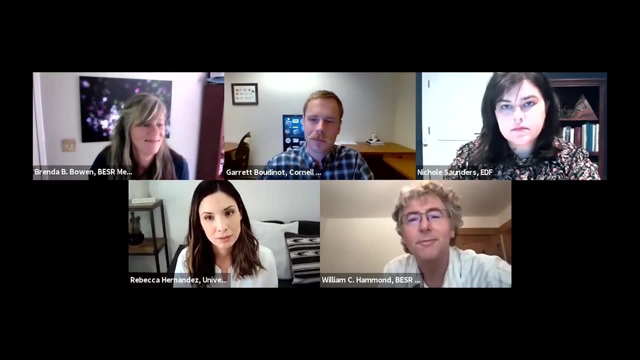 How to facilitate local energy and prevent what we're calling outside in on marginalized communities. Thank you, I think we have time for one last question. i'll invite bill Hammond, another user board member, to ask a question. Hello, thanks, Rebecca. I had one more question about one of your slides. you showed some on water, solar. 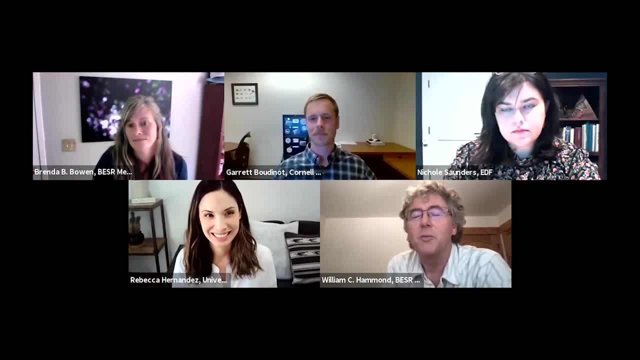 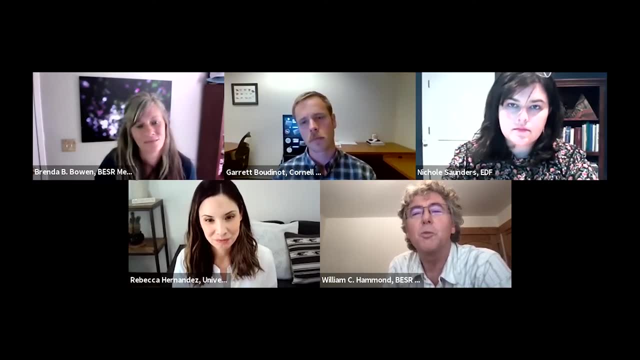 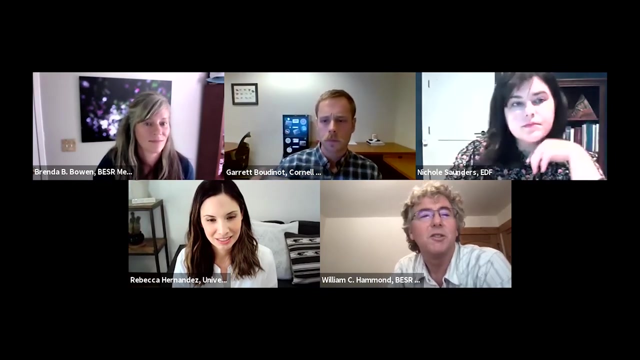 Floating there in a pond and that started me thinking and i'm wondering sort of: what are the limits on that? and- and we have a lot of ocean that can be covered with solar panels- what if That were utilized to the Max, and what are the limits on that? is it, is it the transmission, or is it the effect on wildlife, or is it the expense or the harsh conditions? could you say a couple of things about that? sure, this is such a great topic right now. 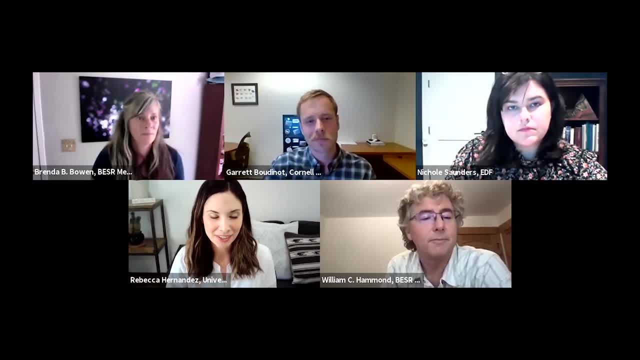 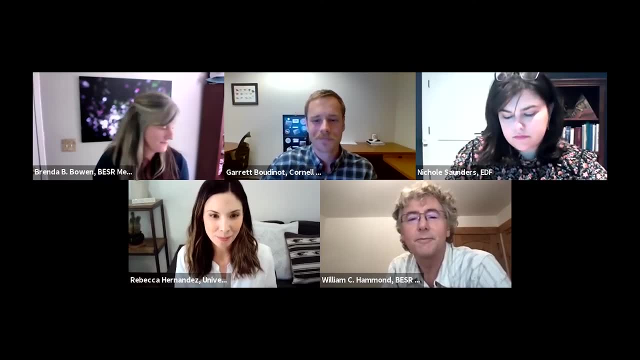 In renewable energy. there it, what started as sort of this niche boutique market of solar just within the past year has just completely proliferated. you know, on the industry side and in the academic side we currently have a grant with the. do we looking at for particular? 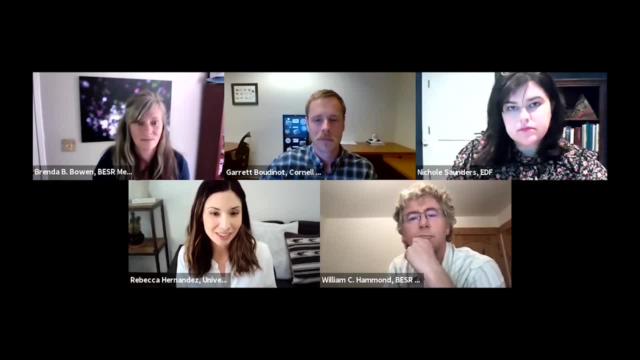 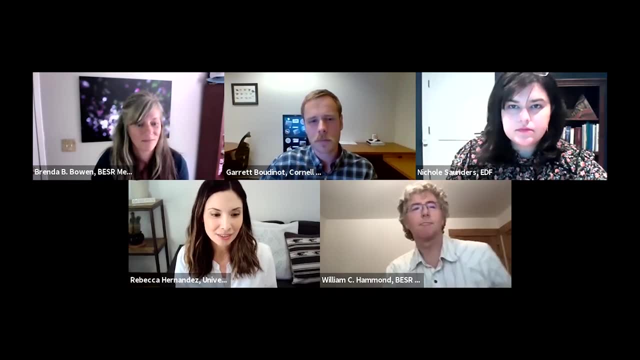 For specific installations in the US and the really amazing thing about them is that they're they're so diverse. One is the water treatment facility, one is the first floating photovoltaic array and for me and day, i'm sorry- in Napa, which is located at a winery called for me and day, and then to our stormwater, runoff reservoirs and Florida. 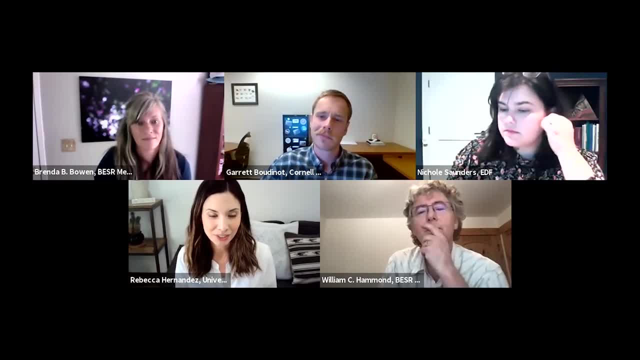 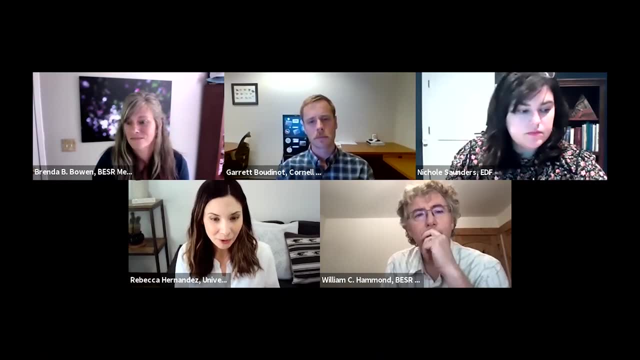 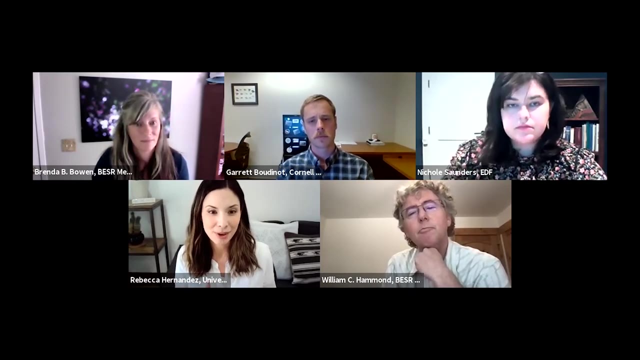 Now, what are the barriers to development? well, that's something that we're actually working on. right now, we don't know a lot about what the Performance outcomes will be. there's there's considerations about the soiling, specifically how birds might impact performance when you have water and sun combined. this is, you know, exactly what people add to. 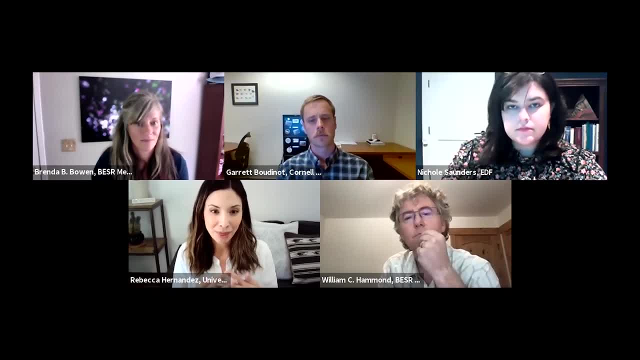 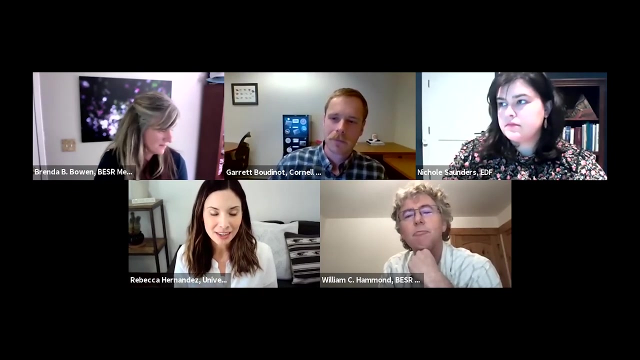 Create weathering experiment. so it's essentially this sped up weathering experiment on PV which has implications for end of life considerations for the solar energy industry, And then there's impacts on wildlife and impacts on potentially impacts on water, and so we're we're learning as fast as we can, while development is also kind of racing forward, and but the one thing that we've we've noticed in the field is that 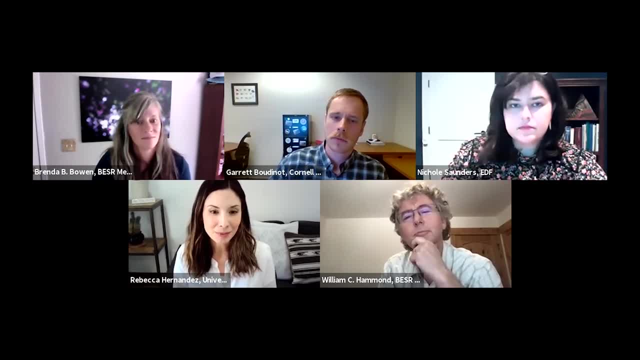 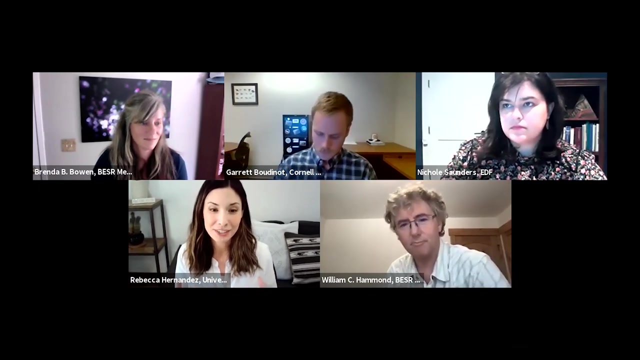 The birds seem to be very Acceptable, accepting of using the floating solar infrastructure. They use it to dry their feathers and to hunt, which surprised a lot of ornithologist when we showed that at a meeting. So there's just. it's just a huge sort of open space that our frontier, I would say, in energy ecology, and we're learning as fast as we can. 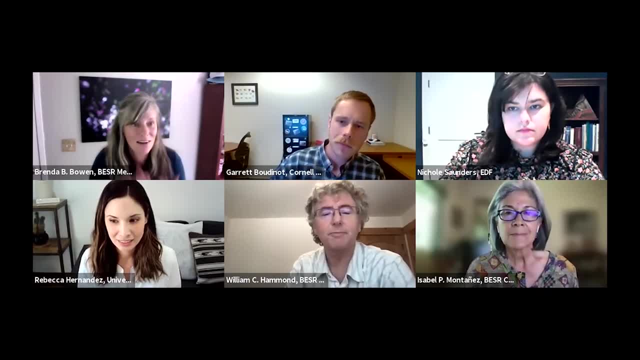 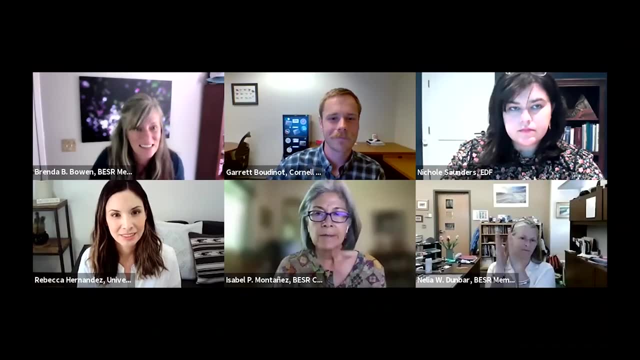 Thank you. i'd like to wrap this part of our meeting up with a big thank you to each of our speakers and panelists, And, Garrett, Thank you for joining in for our panel discussion. this is really a fascinating and interesting discussion. that just demonstrates the 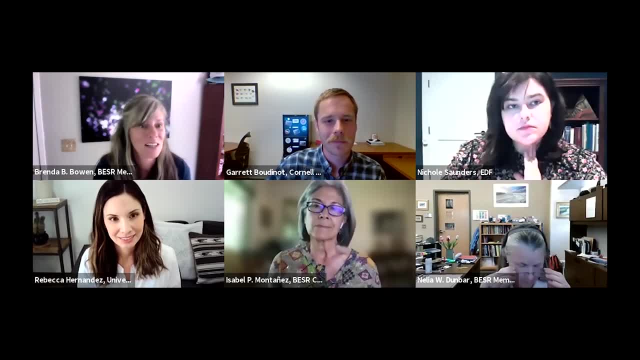 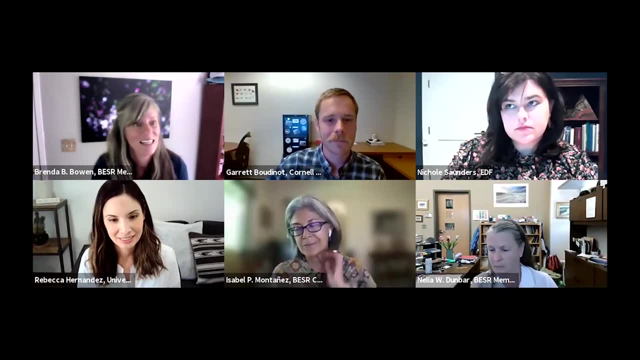 The areas of research that are poised to be worked on as we think about the energy transition and all of the links between water and ecosystems and land use, and justice, and And the work of the earth science community within that space. so thank you so much for your, for your engagement and presentations, and I will pass it back to Isabel, our board chair. 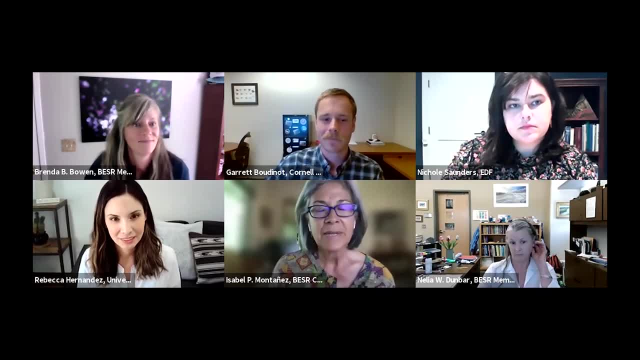 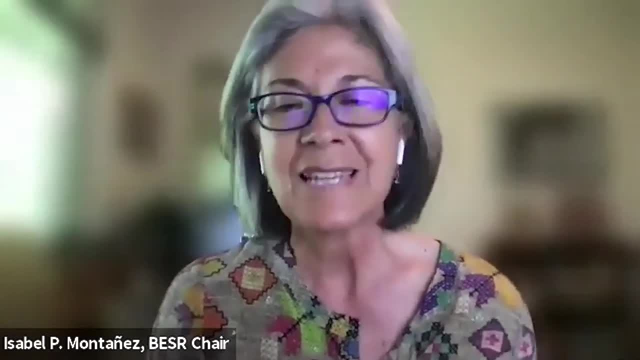 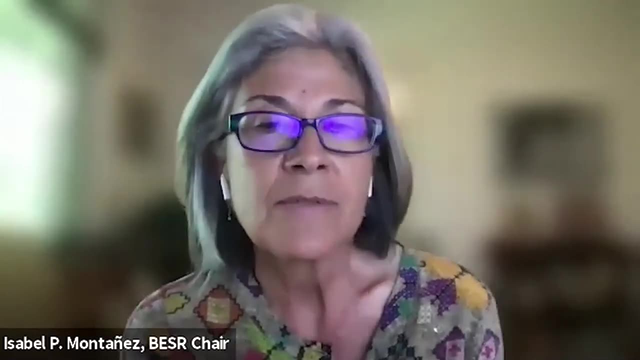 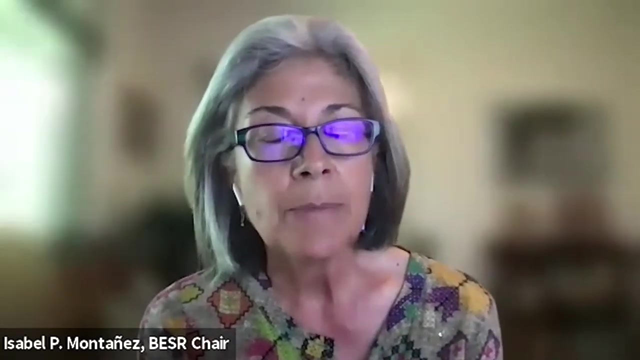 For a final synthesis. Thank you, Brenda. Thank you to all our panelists or speakers, and including Brian Anderson, who I don't think is still with us, and for all of your questions. So I would like to just Provide a brief synthesis of what I think we've heard today: where some emerging opportunities, the challenges and and where Beezer, for instance, might be available to contribute. 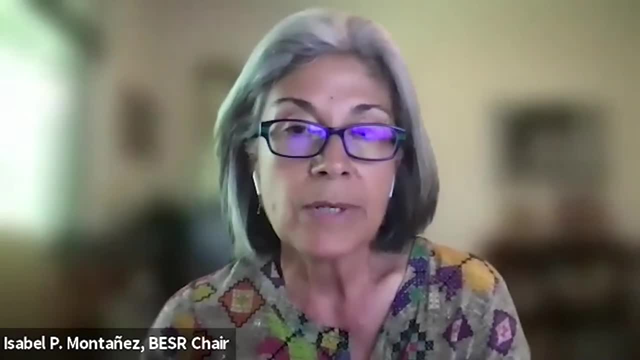 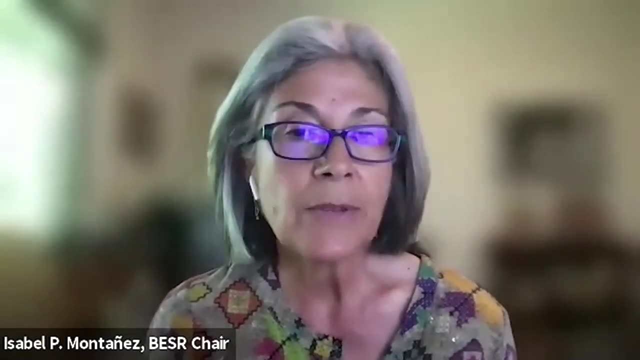 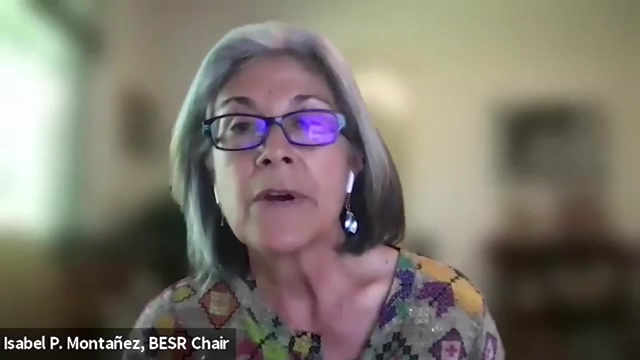 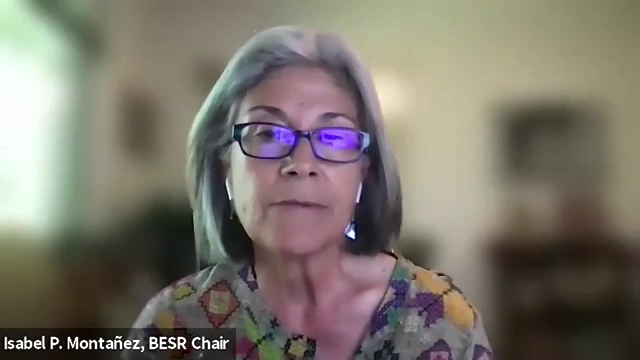 So we heard today That the future of energy systems in the US is one of decarbonized energy. with the current administration setting the goals to eliminate emissions from power plants By 2035 and net zero emissions across all sectors by 2050. and to accomplish these goals, it's clear we need a very aggressive pathway forward with optimal solutions if we're going to reach that net zero economy, carbon economy- by 2050.. 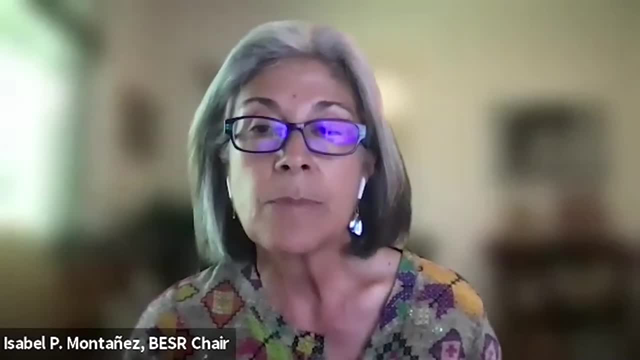 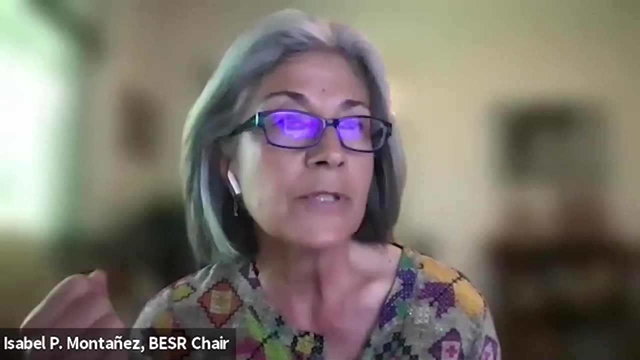 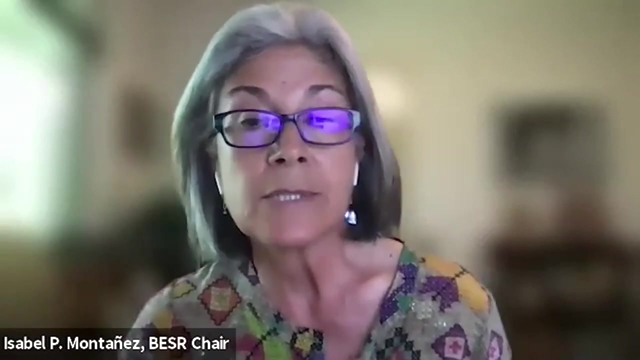 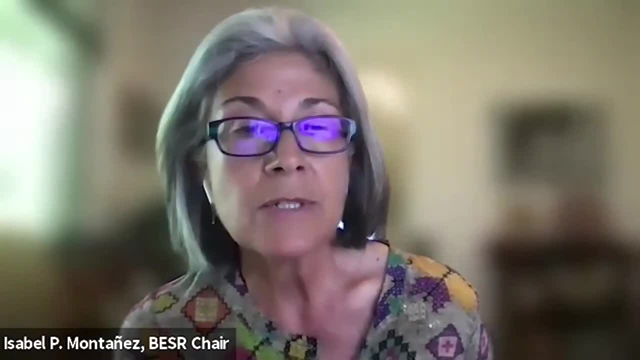 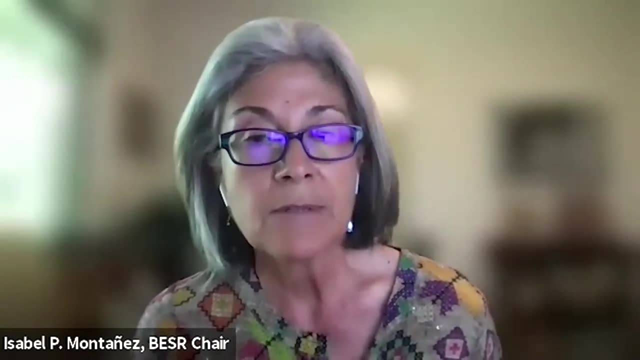 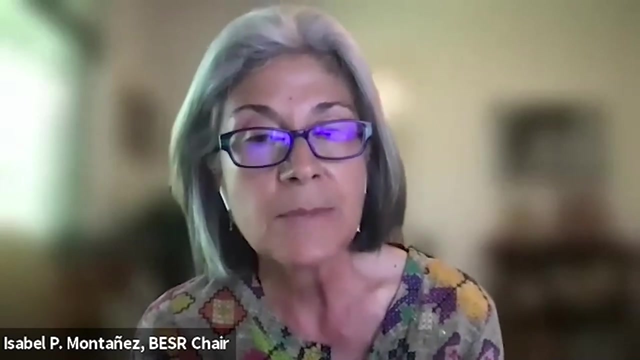 So we heard from all of our speakers both exciting opportunities and major challenges and defining the pathway forward with optimal solutions, with much focus on earth Resource sustainability and minimizing environmental impacts. So Most of the changes will require, as Becca Hernandez said, entire knowledge systems spanning. 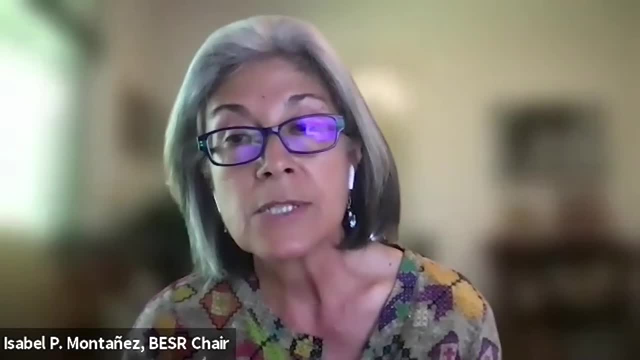 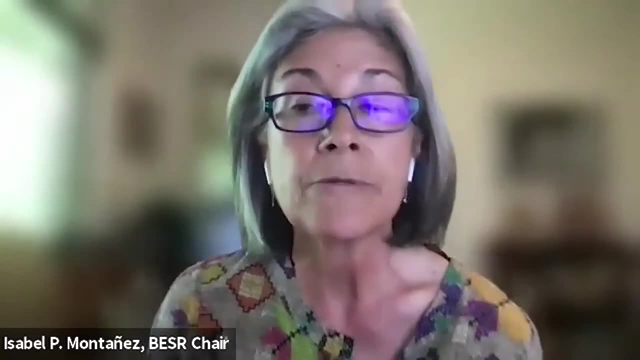 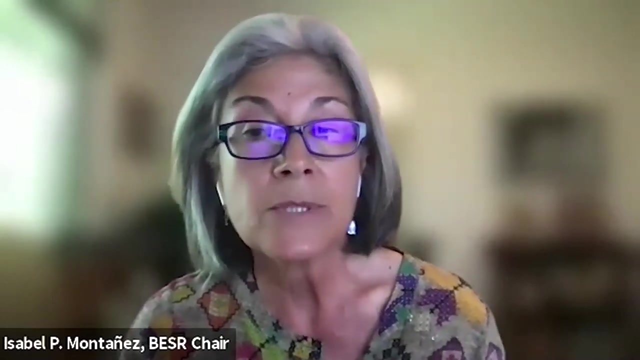 multiple sectors, including the stakeholders, policy and decision makers, regulators, researchers, among others, And we heard that alternative energy sources will provide only about 50% of the carbon or CO2 savings. Thus, we'll need carbon removal methods and carbon storage opportunities, both of which. 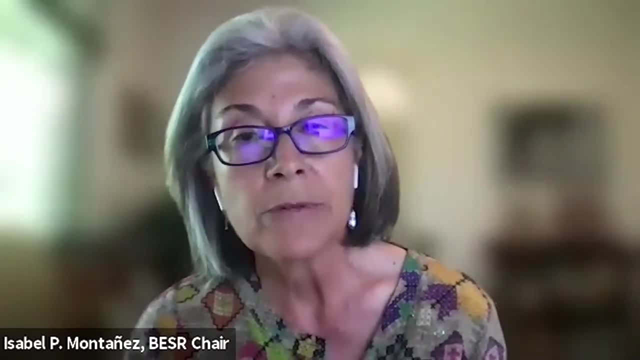 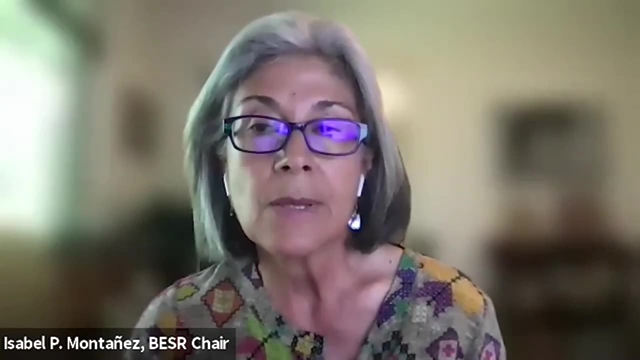 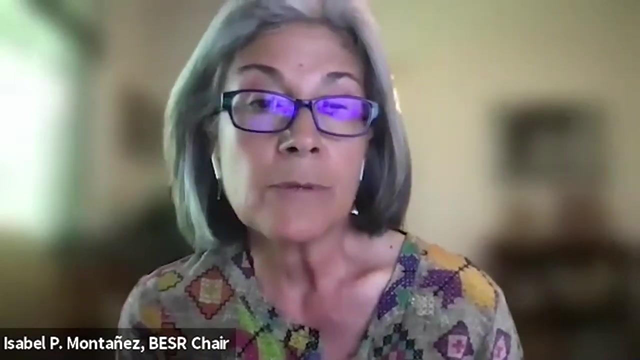 will be critical once we hit about 60% carbon decrease. We heard about the need for methane sequestration technologies that are just about coming on board, And we heard about transformational CCS technologies such as new polymers and biosorbent materials. 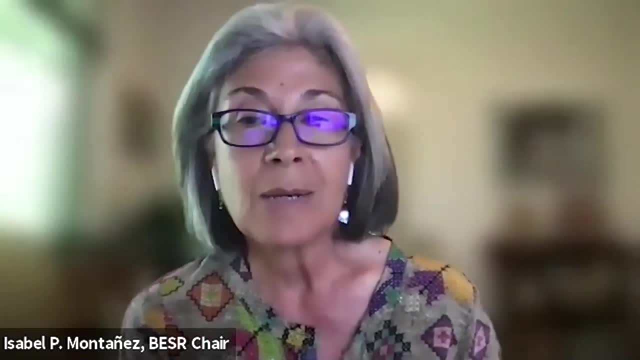 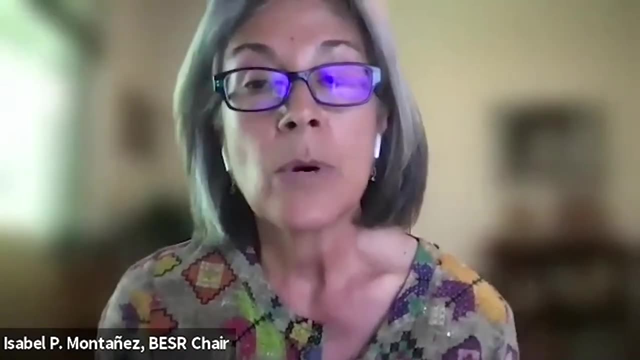 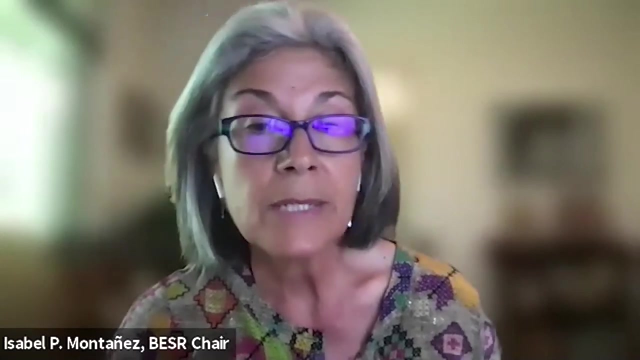 for direct capture of CO2, even with a benefit of byproduct of blue hydrogen. But there are challenges to this carbon. Where are we going to store it? in a subsurface, Where it is sequestered safely and permanently? And, obviously, another key need, how will we drive down the costs of carbon capture? 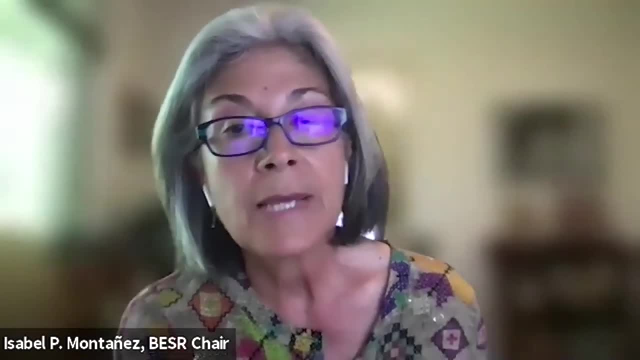 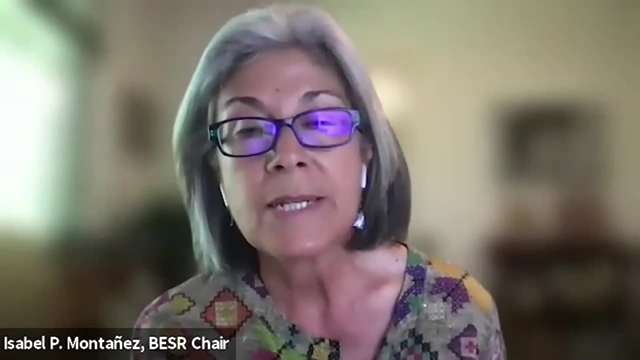 as Brian discussed with us, Ben Houghton and Garrett Abudanet introduced us to direct carbon capture that does not require fossil-based, fossil fuel-based energy And obviously, from a lot of the questions, I think there was a lot of interest in that. 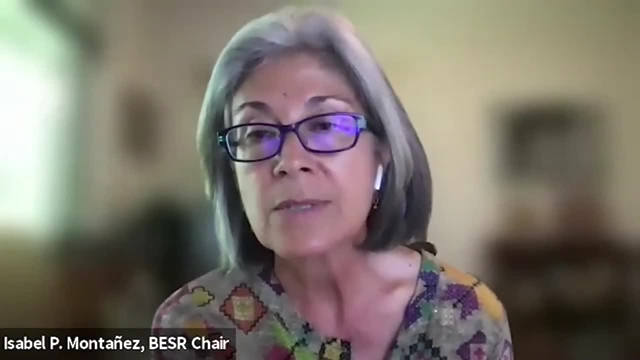 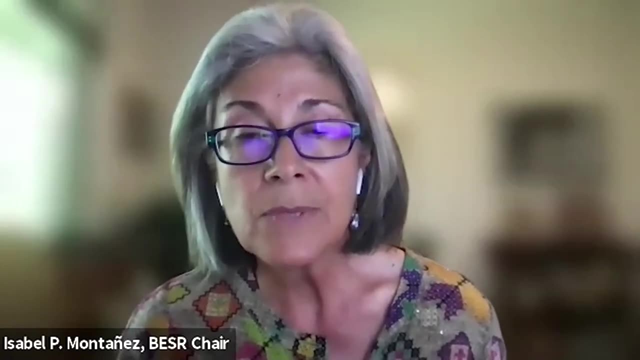 This has the potential on a global scale of 2 to 5 billion tons of CO2 removal, but clearly the gap between the potential and deployment is very large, And they shared with us their findings from their Workings Land Innovation Center, where 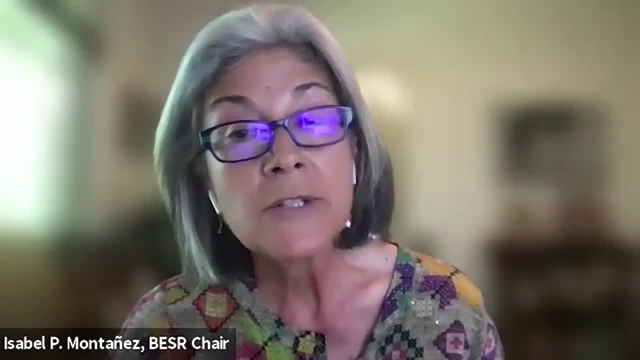 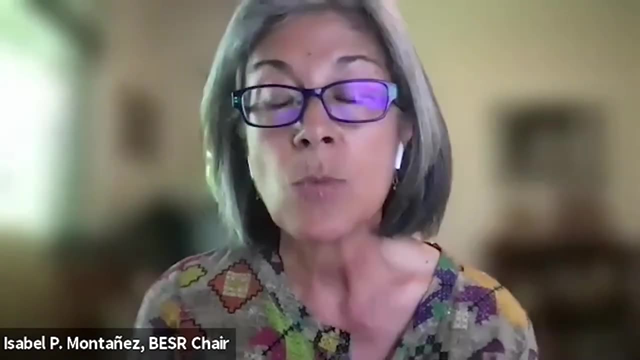 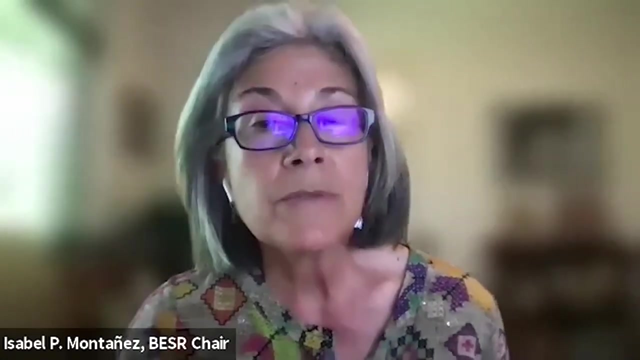 they're testing on a fairly large scale the potential of soil amendments to diverse croplands and rangeland, certainly showing us the potential as well as the co-benefits regarding the ecosystems and biomass yield. But, as with all of these emerging energy technologies, these efforts require much more research. 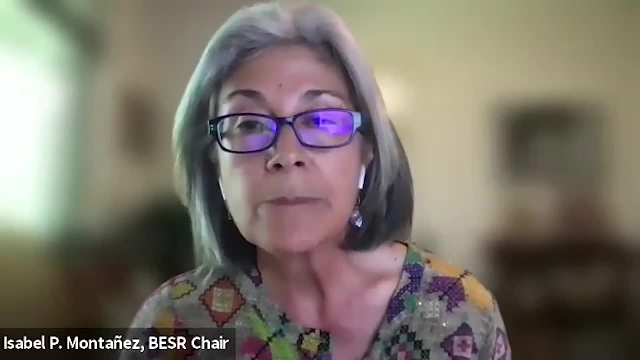 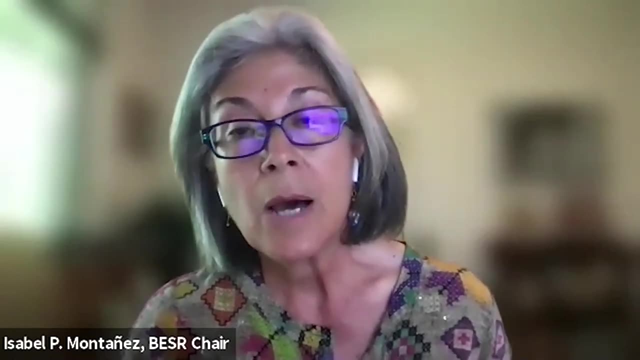 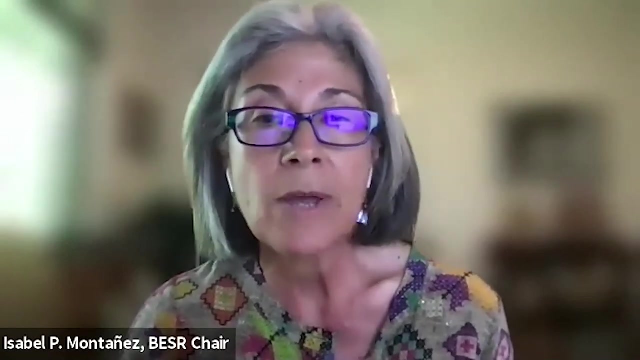 more research to understand the life cycle of carbon capture, that is, the predictive rates of carbon capture, cost of availability of the necessary materials, upstream greenhouse gas and emissions and environmental impacts. and then the incredible barriers to adoption of enhanced weathering, in particular price point issues. 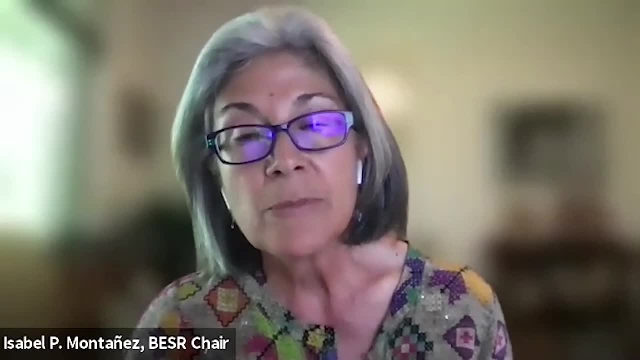 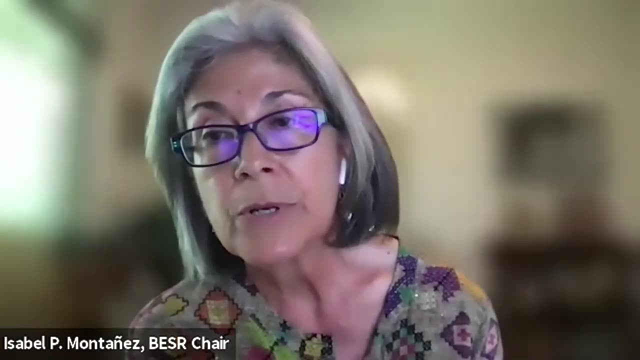 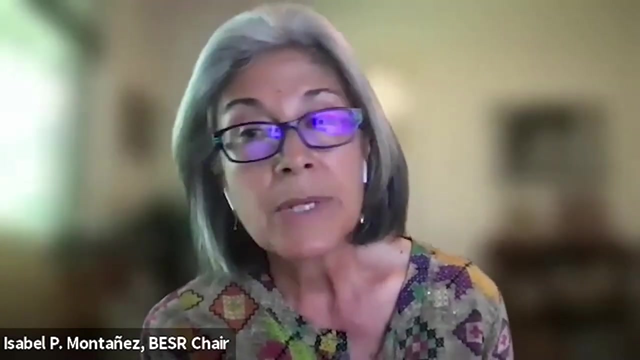 Once again, it requires the collaboration of the suppliers, the government, the farmers, the environmentalists, among others. Nicole Saunders shared with us the opportunity, The opportunity for reuse of produced water. management that has been conventionally reinjected into the subsurface but, with climate change and associated other impacts, has the potential. 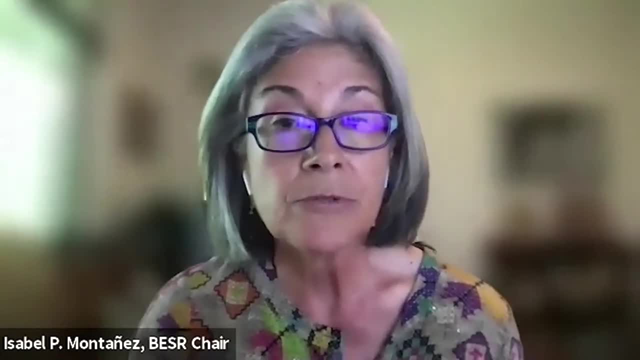 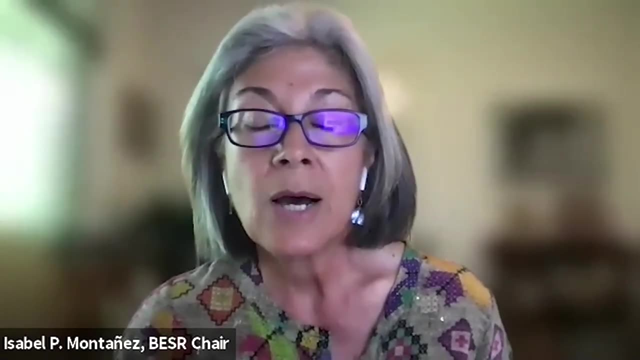 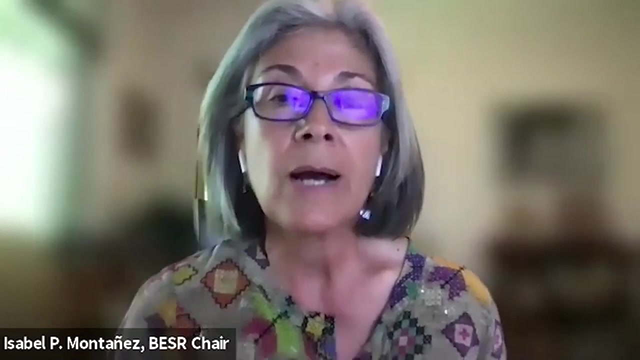 for land applications, industry use and potential for drinking water. But she too has told us these opportunities are met with regulatory and protection gaps, and talked to us about all of those issues, including infrastructure ones, And we all appreciate the need for. renewable energy sources That will be a substantial and necessary component of the US future energy portfolio. But, as Becca Hernandez indicated, energy sources use land, so much so that energy development in the US is now the largest driver of land use and land cover change. 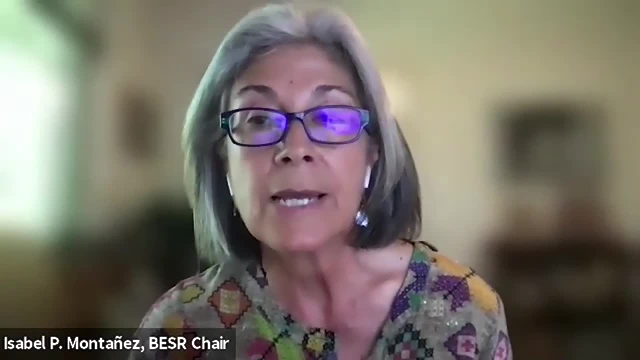 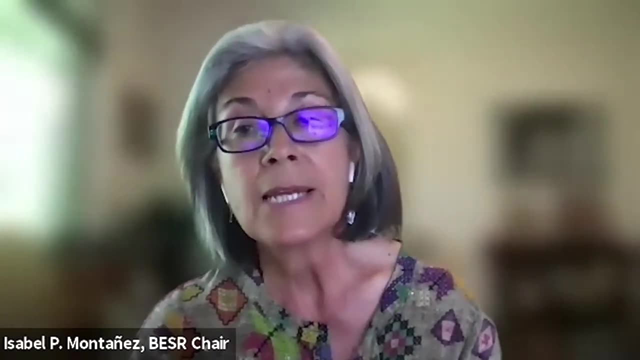 So a key question is: how will we meet our future energy needs and strategies while protecting a sizable amount of land for food protection and sustainability and maintaining the environment? Thank you, Thank you, MS. I would say that first is this: I think you're right, and that's just one of the single ones that I think that I am. 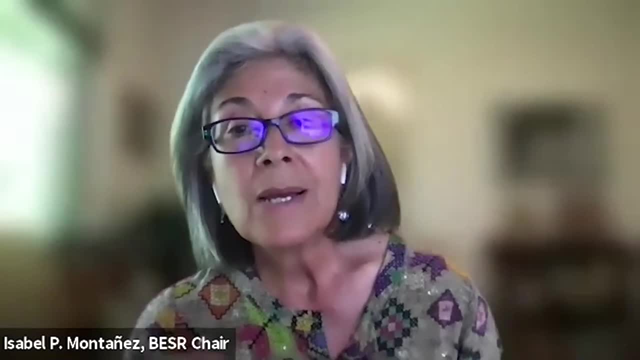 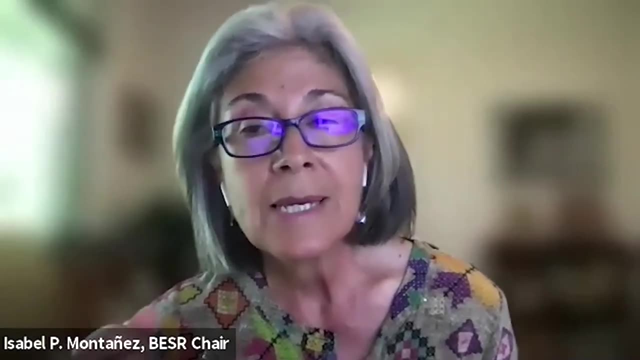 going to be talking about This is in terms of the development impacts on the environment, on the energy for getting ballooning habitats, for ecosystem services, And I think it's really interesting that we heard that when solar energy, for instance, which can have a very large land footprint, is integrated in existing infrastructure locally. 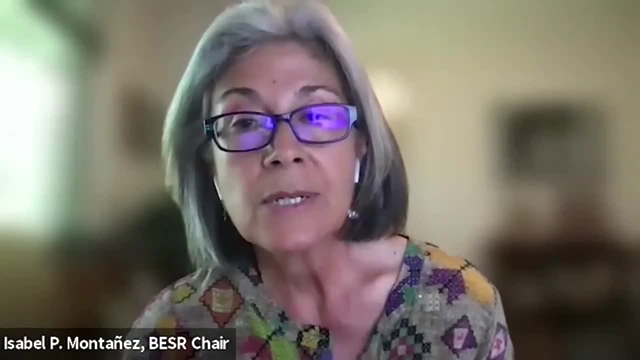 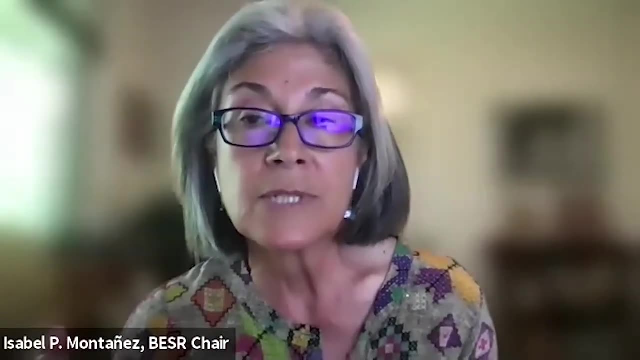 can incur zero additional land use and land cover changes, And she spoke to us of how different new installation strategies maximize techno-ecological energies. We heard from our panelists and comments by our guests that solar energy is closely related to the environment, And she also said that solar energy could actually help the environment in which it. 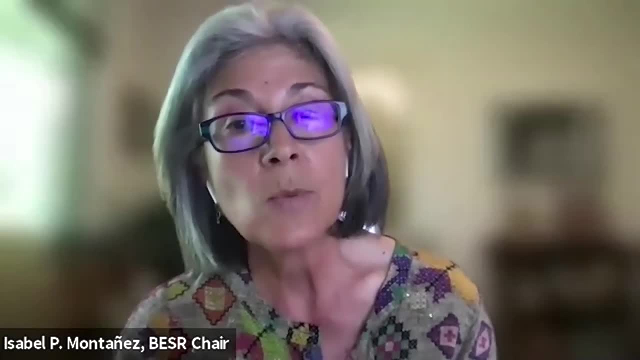 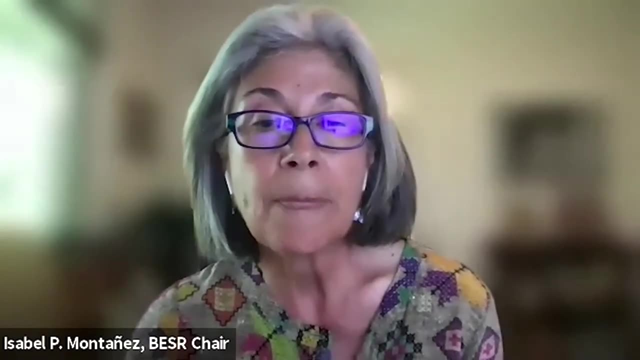 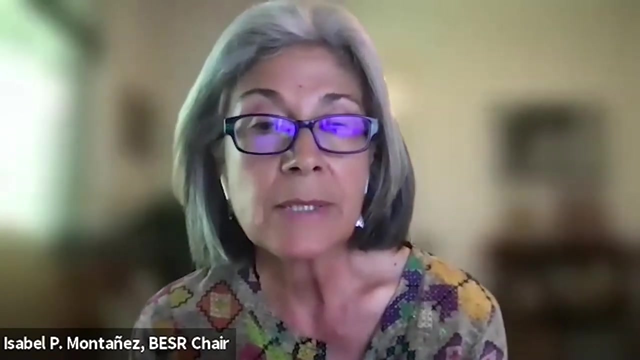 is located. So thank you to all the partners that shared Ms that. solar and wind renewables, reuse of wastewater streams- all involve challenges in seasonal variability and will require seasonal energy storage. research And the sustainability of critical minerals and rare earth elements is a major challenge we're facing. 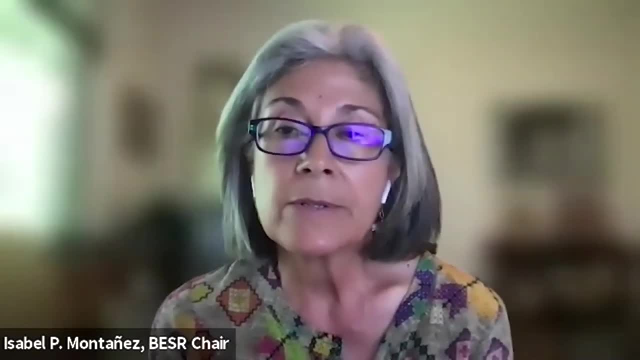 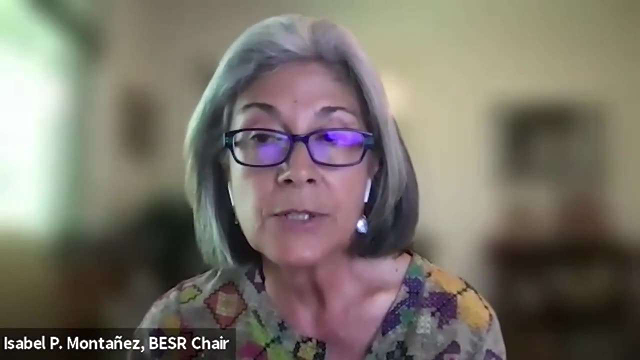 as the demand to produce many of these critical minerals or materials that are needed for carbon capture and sequestration and renewable energy is increasing and anticipated to continue to do so in the future. So, to conclude, I come back to two common themes we heard today. 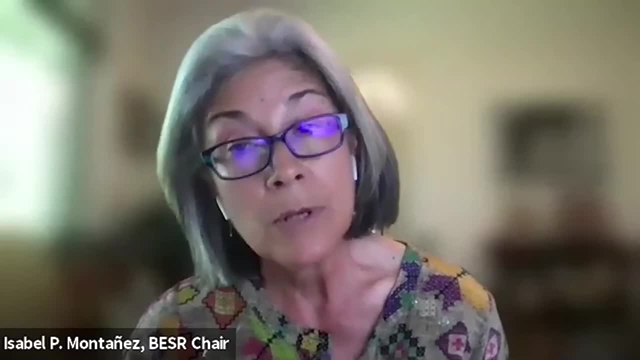 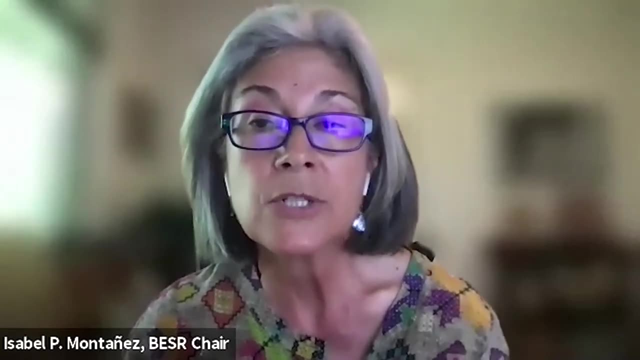 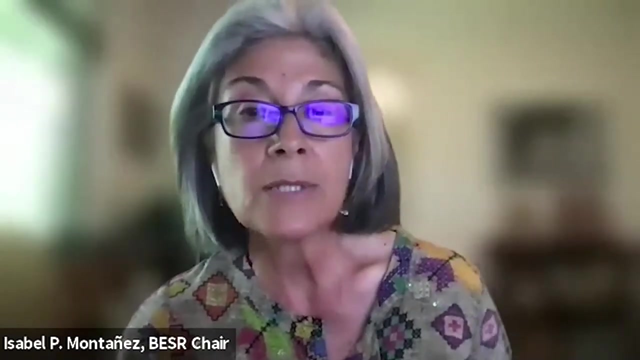 That is, that developing and applying these solutions, and others that were not discussed today, requires a full-scale knowledge system, one that holistically considers the life cycle of the technologies, and one that involves those players that produce the science and technology, those who will develop an aggressive energy policy. 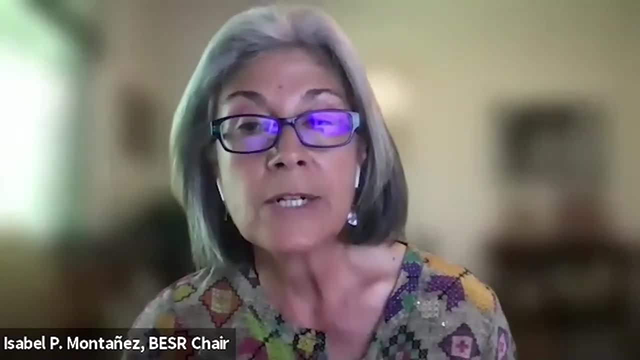 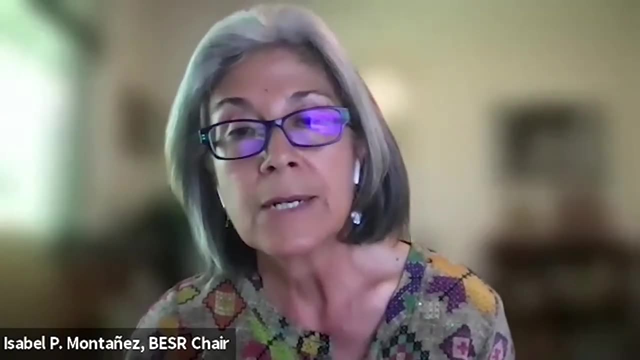 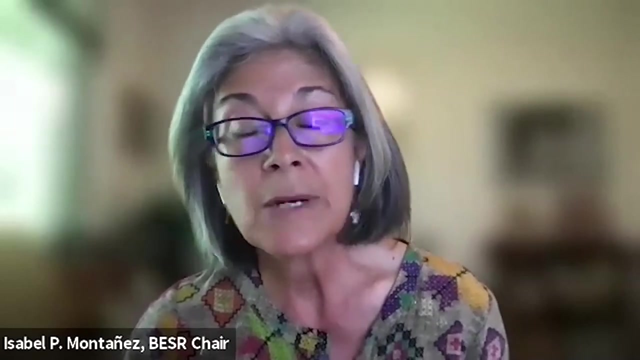 and regulation portfolio, as well as market strategies, actions and the stakeholders who will be impacted both positively and negatively by the emerging energy technologies. So I'd like to thank again Brian Anderson, Nicole Saunders, Rebecca Hernandez, Ben Holton and Garrett Abuno.